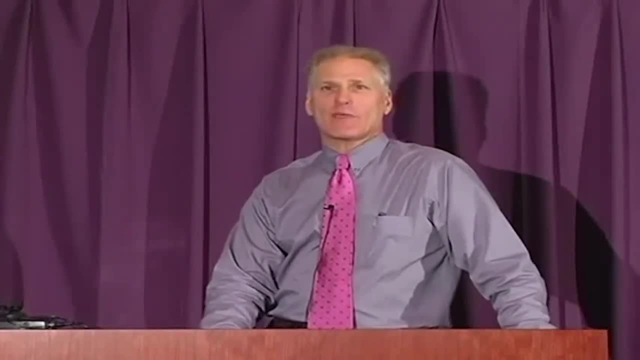 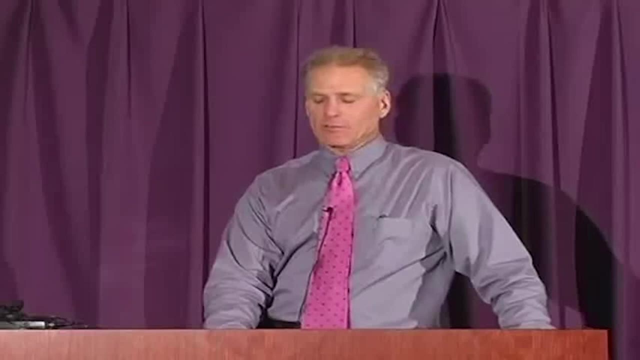 This is where we started. This was the first exploration that we made, because we found that our systems in-house were very inadequate. When we compared our vacuum system to a vacuum system, it was very inadequate. It was a vacuum foaming system and I'll use quotes on that. It was basically a vacuum pump and compare it to industrial guidelines. 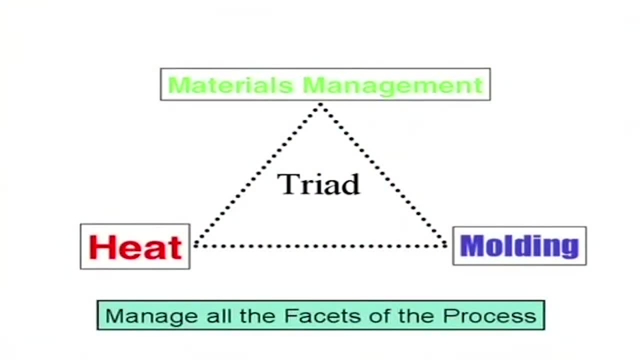 Again this comes into our triad. We've looked at materials management. We've looked at the heating aspect. Our material is now at molding temperature. How do we now take that material and use some kind of a physical force on that softened material to form it into the shape that we want? 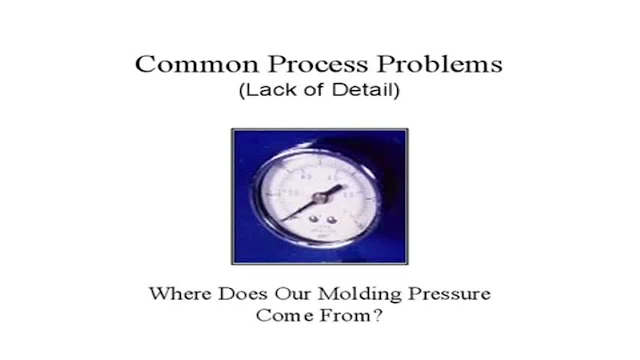 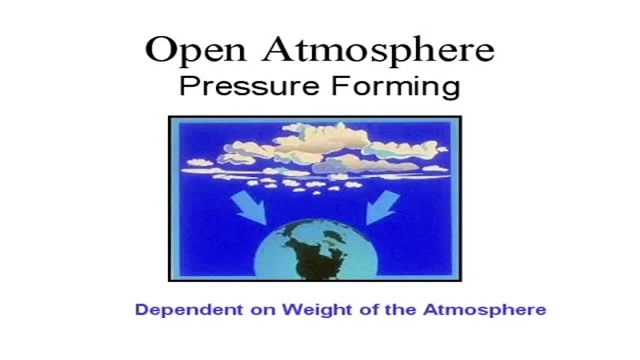 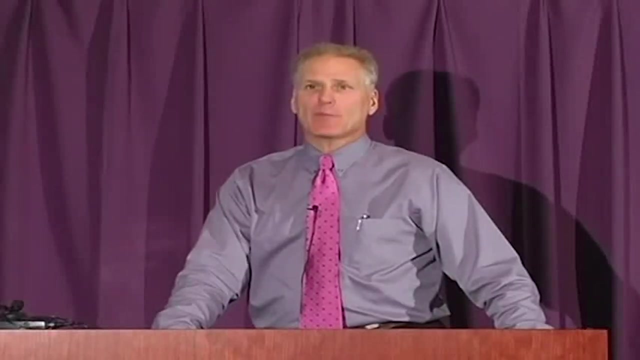 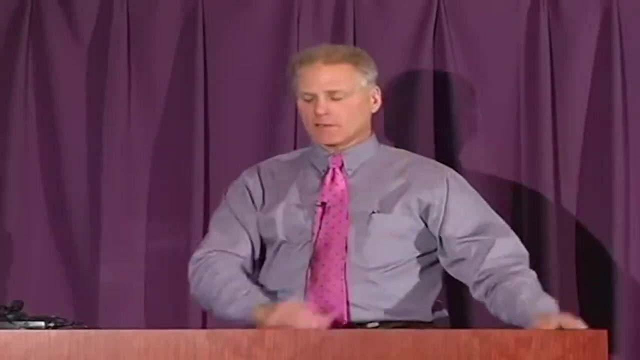 Where does our molding pressure come from? Common process, Common processing problems? Lack of detail, Lack of capturing that intimate shape that we need to hold componentry in the plastic We do use open atmosphere forming. It's just the weight of the atmosphere directly pushing on the plastic as we create a vacuum differential through the application of low pressure or vacuum pressure underneath the plastic. that creates the movement of that plastic against the positive muster. 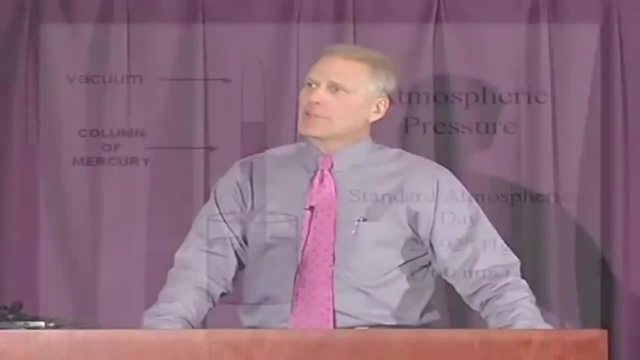 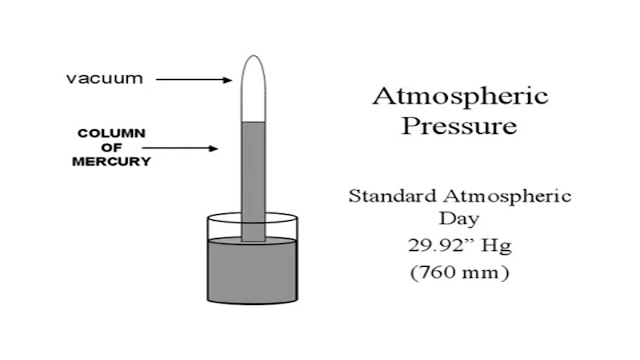 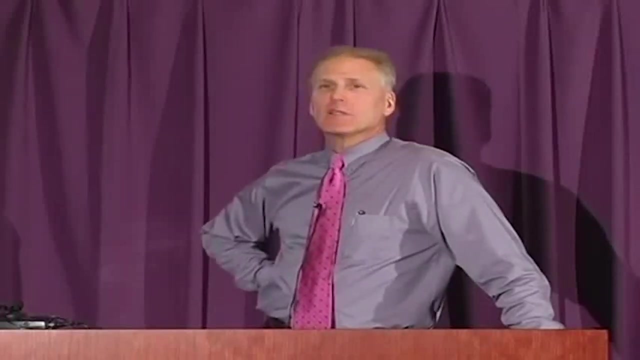 Now we do measure that vacuum in inches of mercury. It could be in millimeters of mercury, Either way, And that's a very more or less. that's an odd way to measure pressure. We're measuring inches of mercury. We're measuring millimeters of mercury. 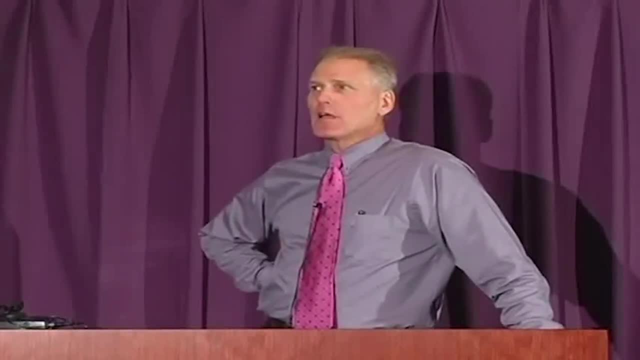 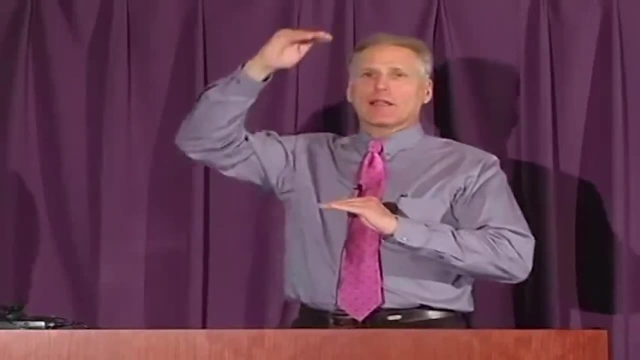 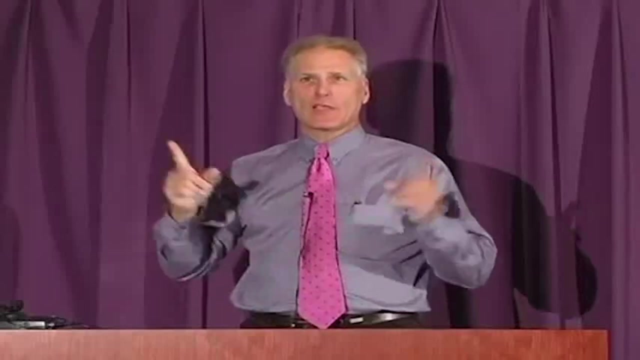 One standard atmospheric day has a pressure of 29.92 inches of mercury, or 760 millimeters of mercury. We're measuring. We're measuring the length of a column within a glass tube that's held in a bath of mercury. We're using a length measurement to measure pressure. 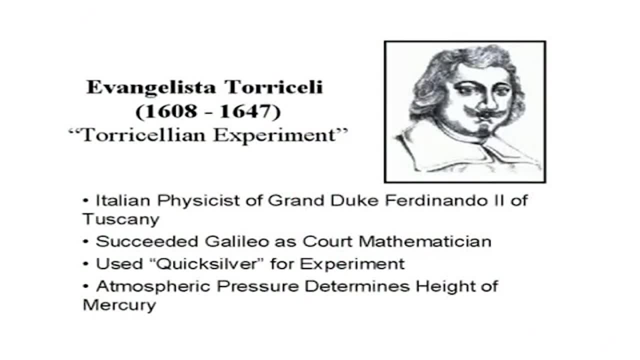 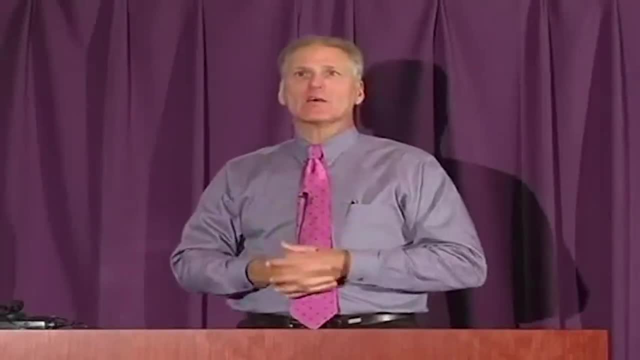 Very unusual unit of pressure. We use that unit of measure primarily because Evangelista Torricelli, making the Torricellian experiment, was the person that came up with that very basic barometer- Mercury or quicksilver as they called it- in a tube that was immersed into a bath of mercury or quicksilver. 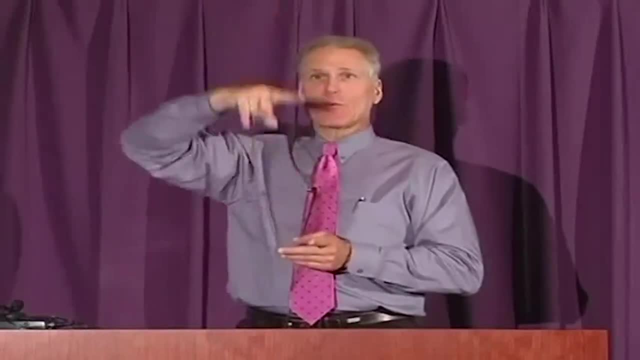 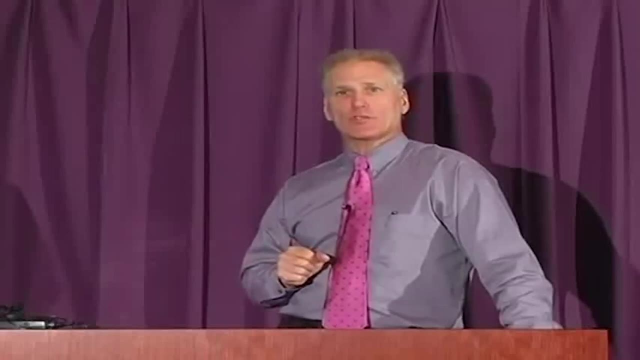 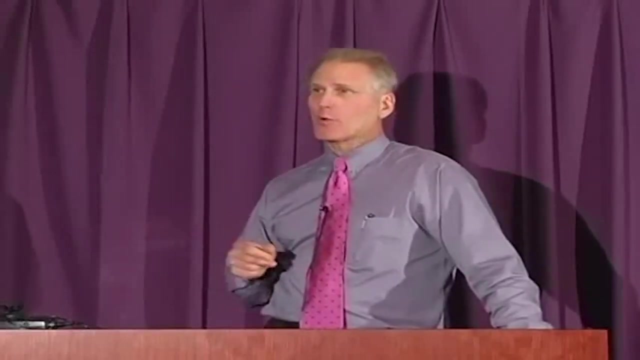 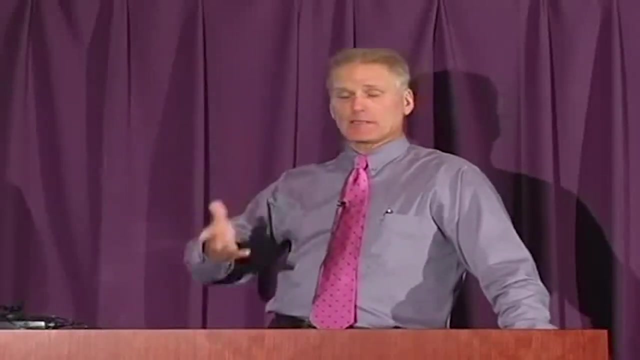 And depending on, Depending on the weight of the atmosphere, would basically raise or lower that mercury column and that's why, to this day, we still measure our atmospheric pressure in a linear measurement rather than pounds per square inch or the metric equivalent. The reason that we have that fluctuation from a barometric standpoint. you go home and hear your weatherman saying the weather, the barometric pressure, is rising or lowering. It all depends on how much, How much, water vapor, is in the air. H2O is a much lighter gas than oxygen, because there's two hydrogen atoms in it- H2O rather than pure oxygen- So the atmosphere becomes lighter. So as you have more vapor in air, you have a low pressure system, which sometimes means we're going to get rain. 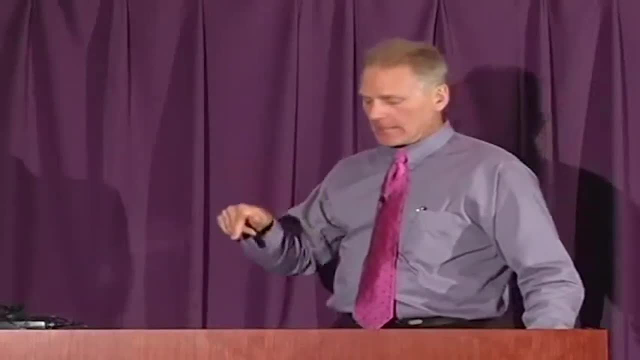 So when the weather man is saying your barometer is decreasing likelihood of rain is because the pressure is decreasing because of the higher water Freeze. Cumulus δ found a near average. so Re FA Matthew Roberts were also reading. Did you guys see it before? 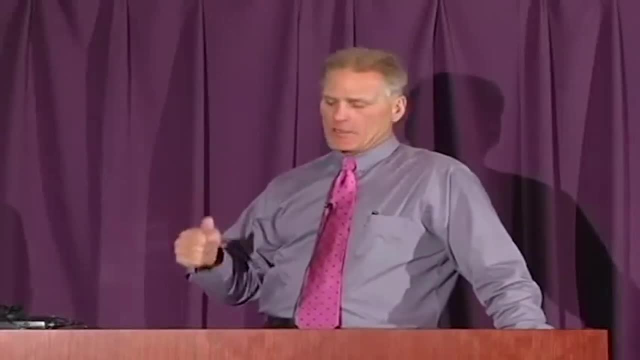 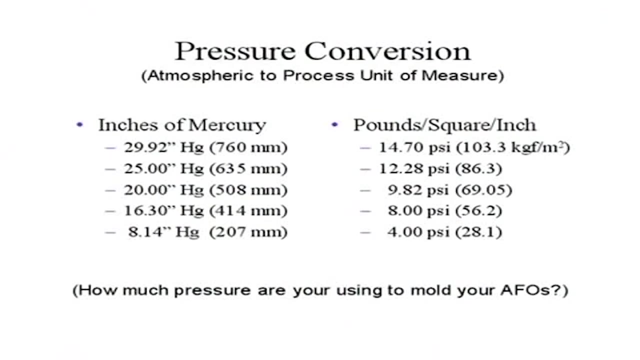 Yes, Uh, huh. Yeah, I could have seen, But back to不過, Yeah, I would especially have. Little does No worries. Eight, Oh, content within the atmosphere In terms of our process. units of measure. 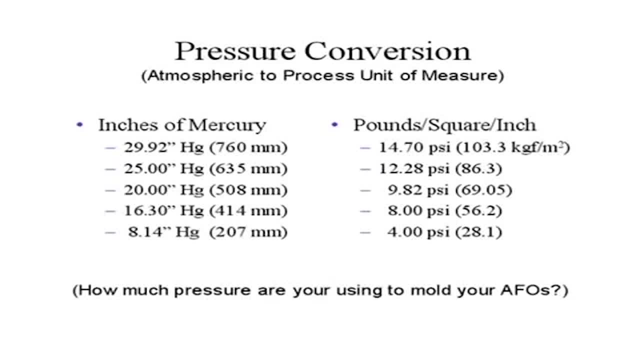 we can do a pressure conversion, switching that linear measurement to pounds per square inch. So if we were to say how much pressure we're using to mold our AFOs at one standard atmospheric day, which is 29.92 inches of mercury, 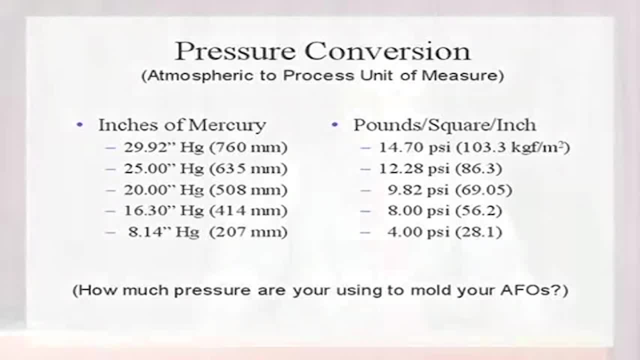 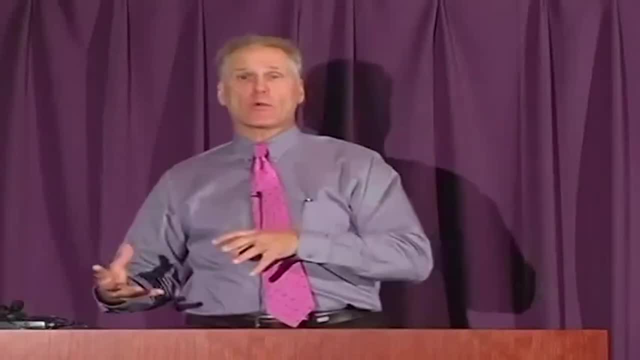 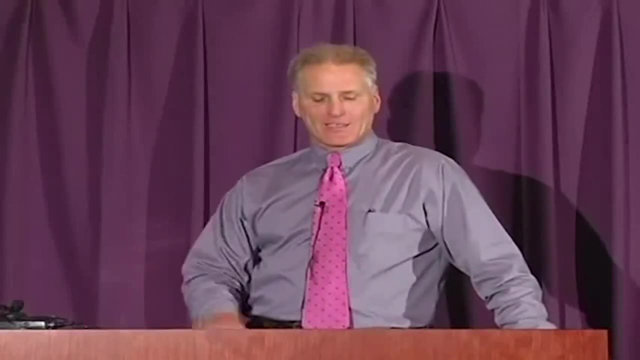 we could say that we're using 14.7 pounds per square inch. It's a very small amount of pressure, Nothing in comparison to that pressure vacuum forming when we talked about the plug assist back in the introduction of this program. Very low amount of pressure, so we have to be able to hopefully. 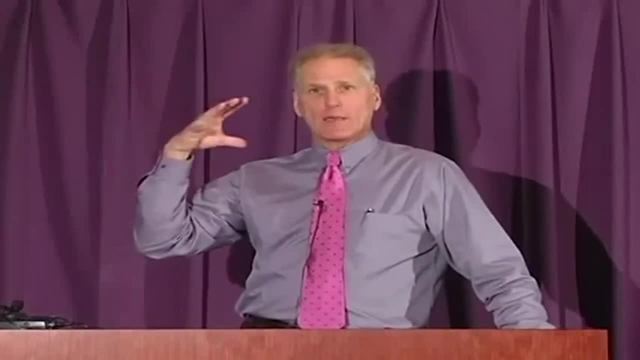 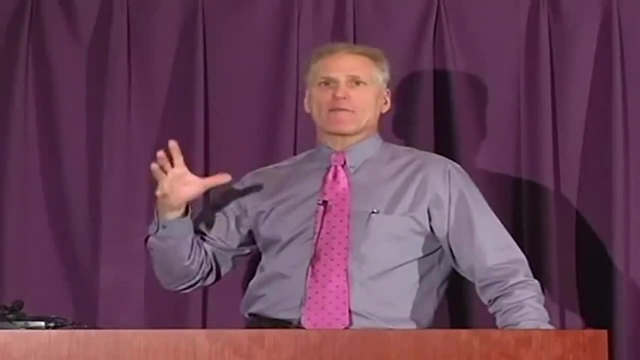 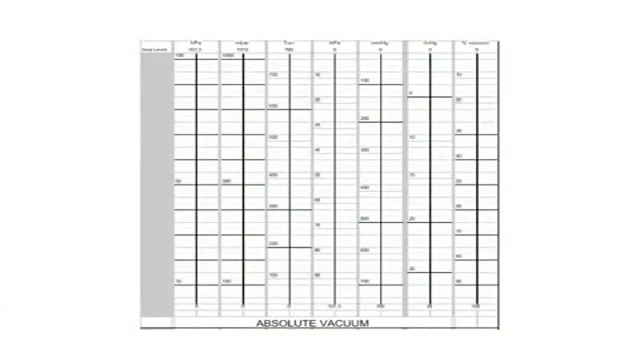 capture the full essence of the weight of the atmosphere when pushing onto our melt temperature plastic, And we can only do that by having an adequately designed vacuum thermoforming system. This was just another graph that I put up here that had KPA, millibars, TOR, TOR-SELI. 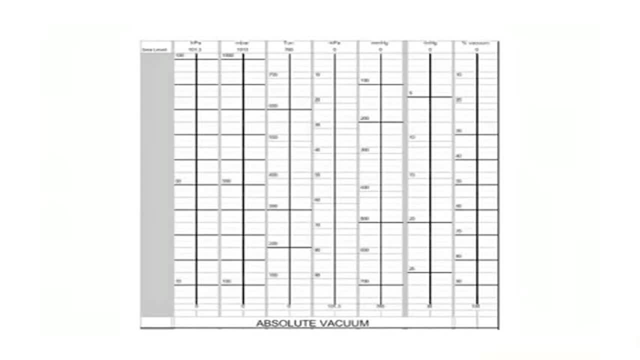 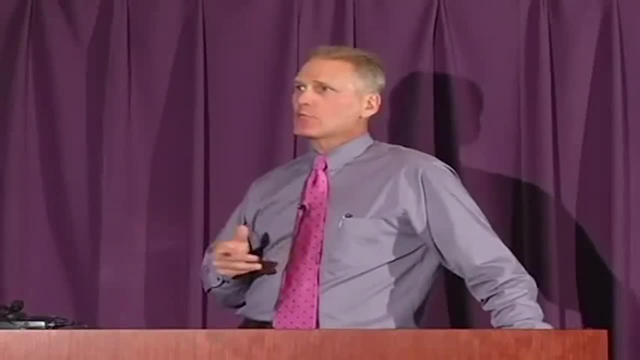 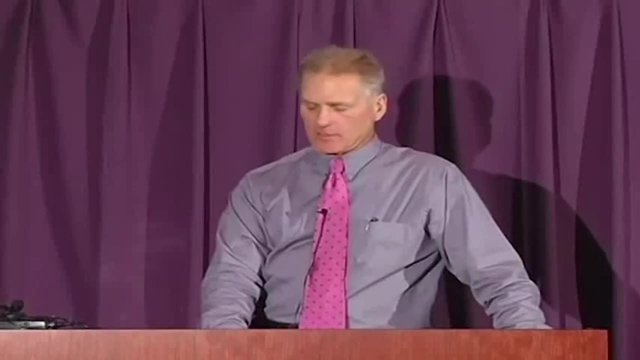 It's one unit of measure. It's using the scientific principles for vacuum: 760 millimeters, inches of mercury and, of course, percent vacuum. So basically, there's just different units of measure for measuring vacuum, depending on what your scientific principle or process is. 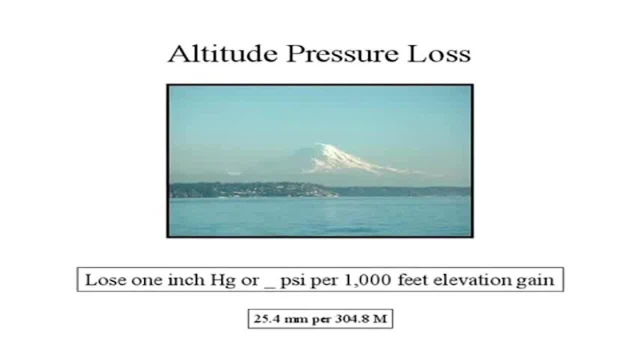 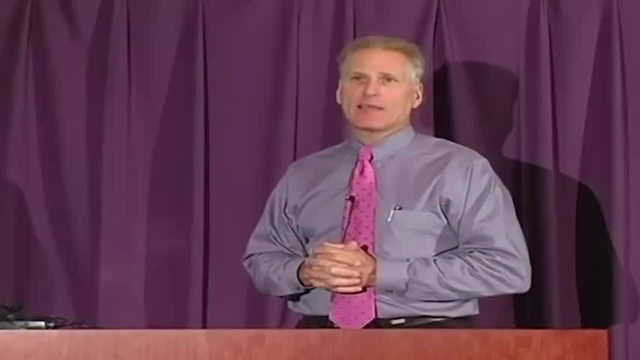 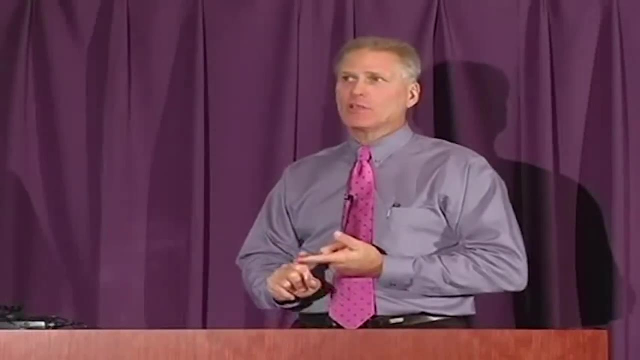 Thank you. Now we also have to remember that the elevation of our lab, the physical elevation of our lab, directly impacts the amount of pressure that we have available from the atmosphere to push on that plastic, onto our positive models, For every 1,000 gain in elevation. 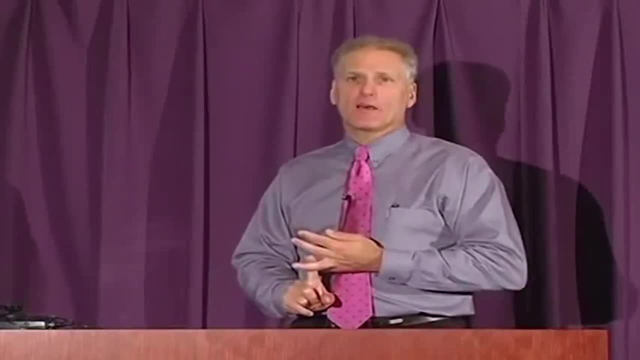 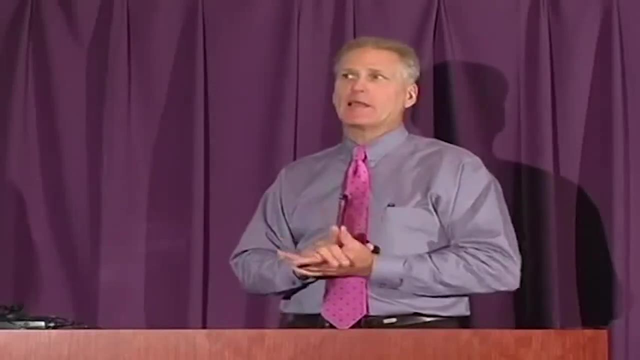 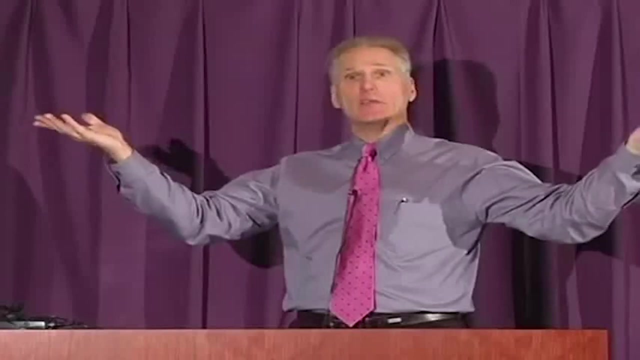 you lose one inch or a half PSI of molding pressure right One inch of mercury or half pound per square inch of pressure pushing on that plastic for every 1,000 feet, because obviously, as we go up in elevation the atmosphere isn't as thick, isn't as heavy. 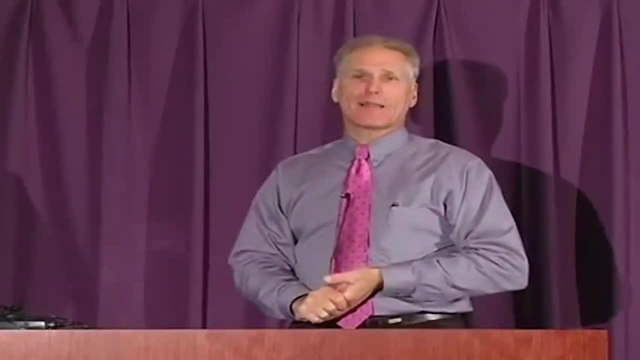 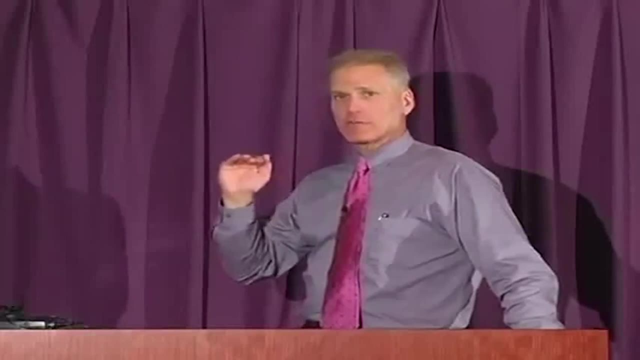 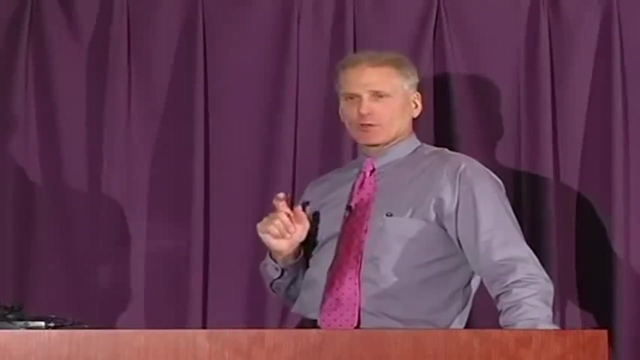 has not as much weight pushing on our plastic as we create that vacuum pressure differential. So if you're in Colorado Springs or a lab that's in the Rocky Mountains, remember that you might have some trouble for vacuum thermoforming unless you're following good guidelines of proper temperature of your plastic and then having 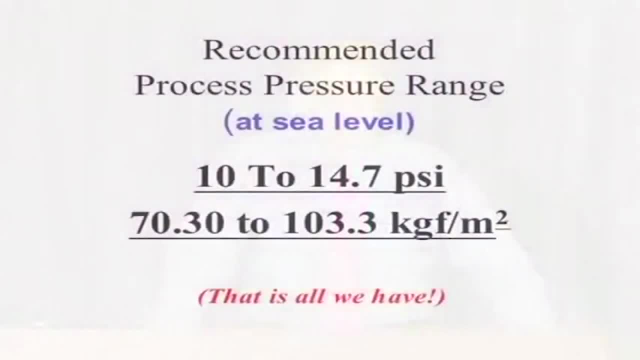 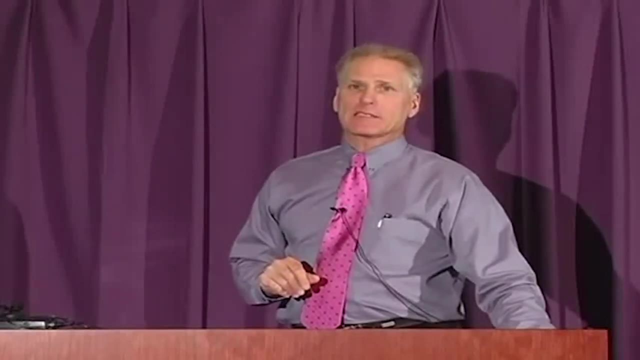 a very well-designed vacuum molding system. Now the recommended at sea level is 10 to 14.7.. Now 14.7 is typically the upper range, because that's the weight of the atmosphere. Now 10 is designated by the plastics engineers because they feel if your system drops below 10 PSI, they feel you will not have enough pressure to push that thick gauge plastic material into the intimacies of the mold. So there is a range, High and low. range: Low defined by the engineers, High defined by the actual weight of the atmosphere itself. 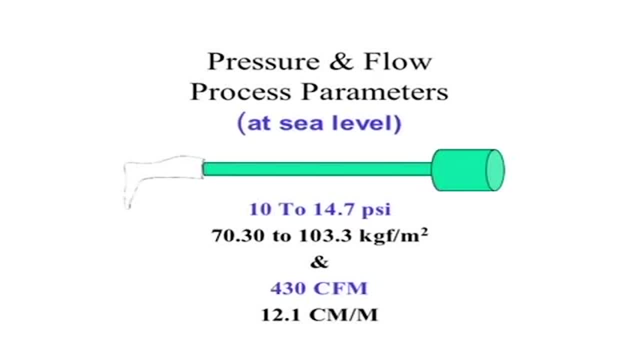 Then we throw on another component to it: flow. We want to be able to move that air as quickly as possible. We want to move that air out from underneath the plastic through our vacuum system as quickly as possible. That's the flow component. 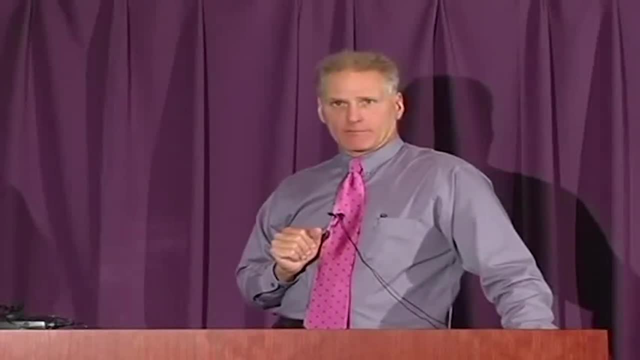 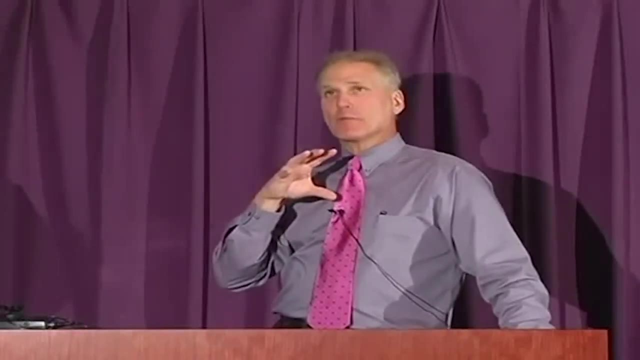 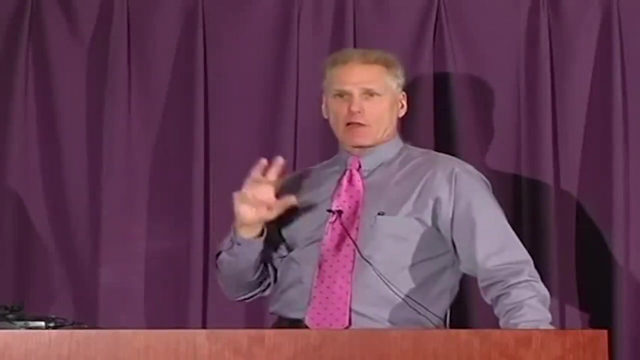 So the flow component is 430 cubic feet per minute And that is from a mathematical model That's specific to the type of volume- mold volumes- that we have in our field. Within the textbooks that I mentioned earlier- Dr Throne's books- there are mathematical formulas that let 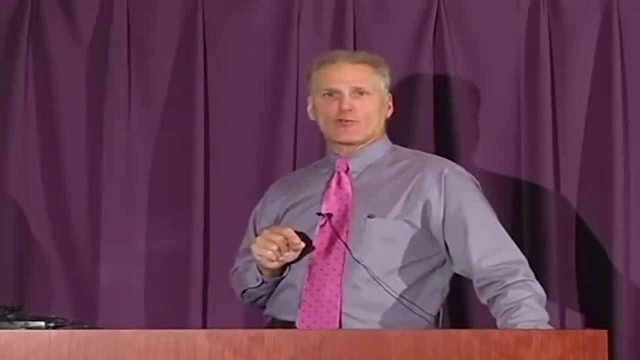 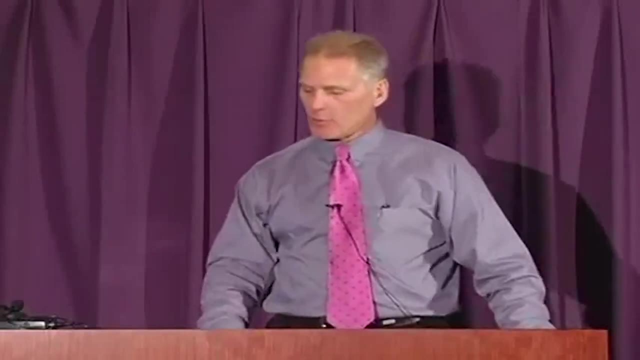 you determine how to maintain that. 430 cubic feet per minute, And that really is the minimum. Up from there would be better, but that's the minimum that you would want to have. And between that, 10 to 14 PSI of molding pressure. 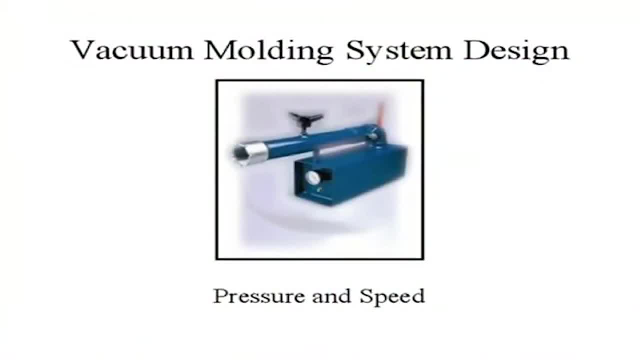 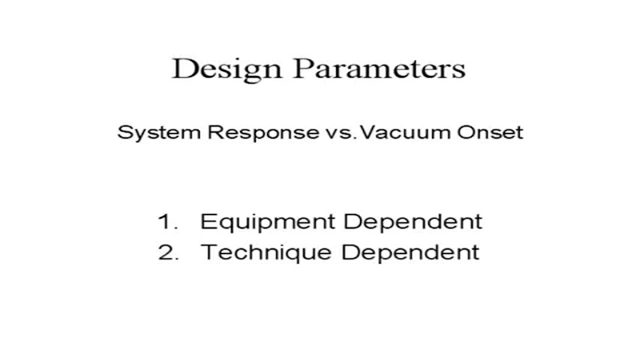 So this is where we get into our vacuum molding system. Our design parameters are based on two sets of criteria Based on your system response versus your vacuum onset, One's equipment dependent and one's technique dependent. Your system response is equipment dependent. In other words, it's how you design your system. so when you crack that valve, you have a very quick evacuation of the air from underneath your plastic, All dependent on your system: The vacuum that's generated by your vacuum pump and the flow you're actually able to correct through the piping and your surge tank within your system. 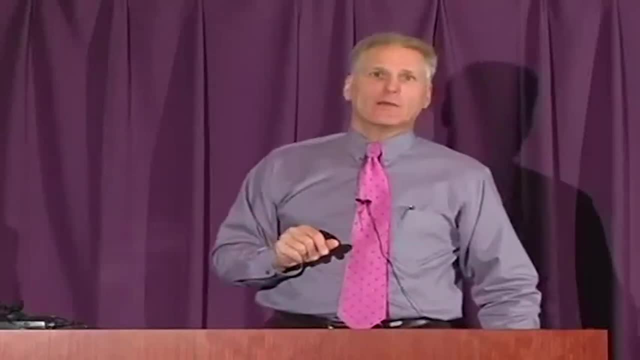 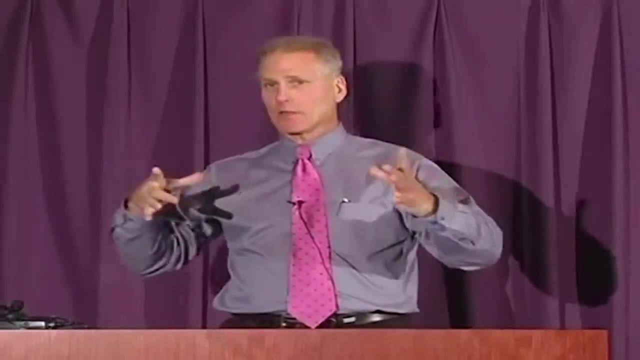 Now your vacuum onset is technique dependent And that's very critical in terms of when you sealed your plastic, how quick you put that onset Prosthetics. sometimes you want it a little bit slower when you're vacuum foaming that truncated cone, so you don't have 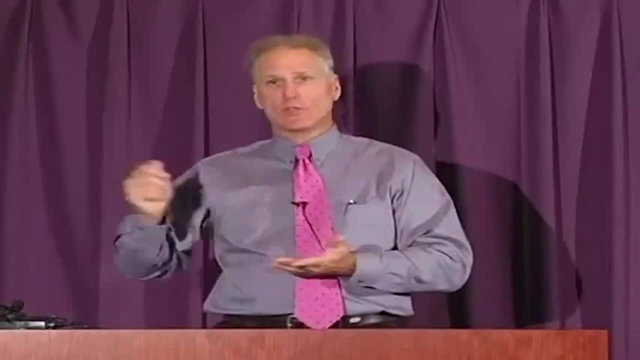 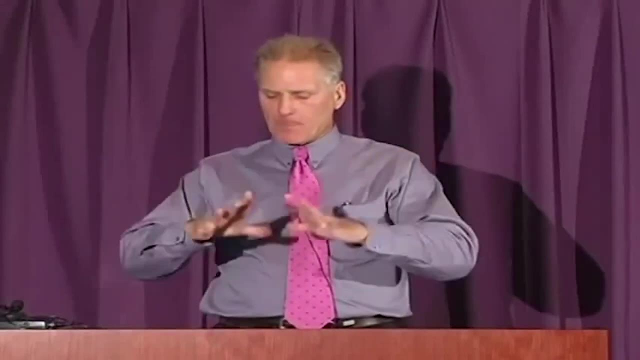 any seams that form When you're doing orthotics and have it sealed. you want to maybe do it a little bit quicker because you don't have to work. You can wait for that webbing that might form, or prevent that webbing that might form when you're manipulating the plastic. 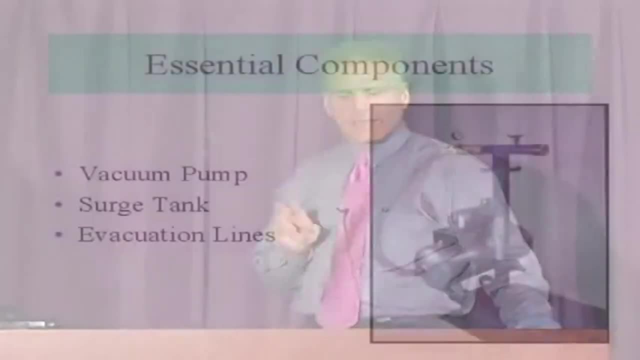 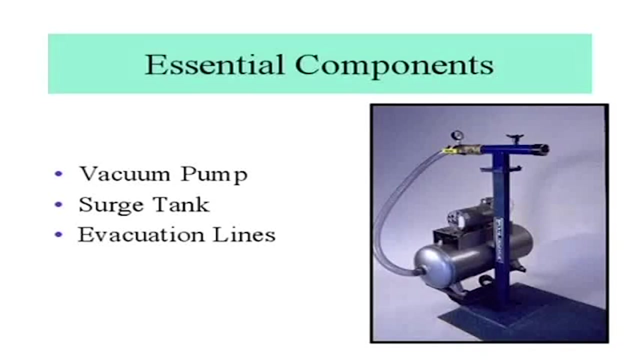 in to take the shape of your positive model. Now, the three essential components that you should have, absolutely have in your system is: a vacuum pump, obviously, because you have to generate the vacuum somehow. A surge tank, which many people don't have but you have to have. 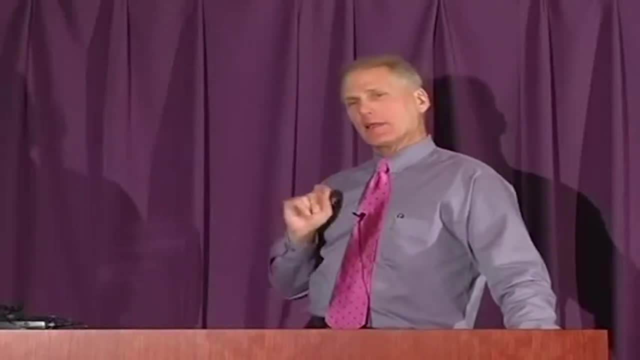 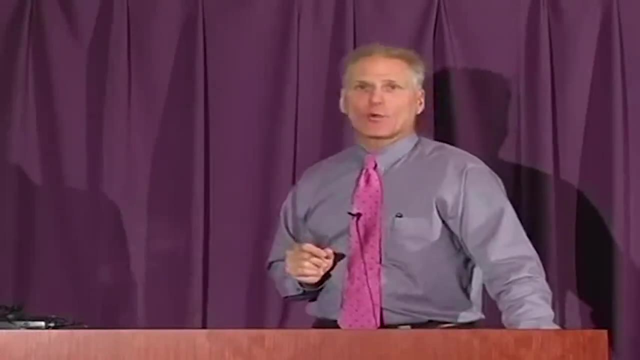 in your system. Look at any thermal forming textbook and that textbook will outline that you need a surge tank of a certain volume compared to your mold volume, And then your evacuation lines. If you have tiny little lines, you can have the world's best. 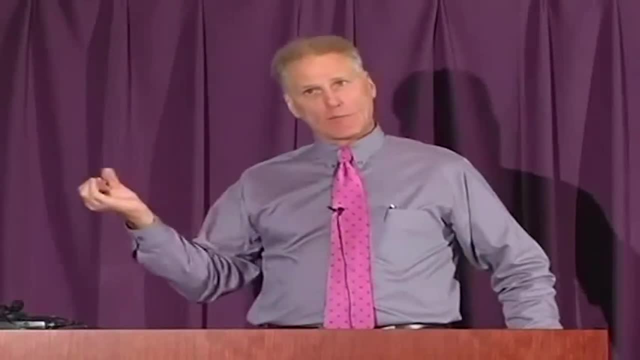 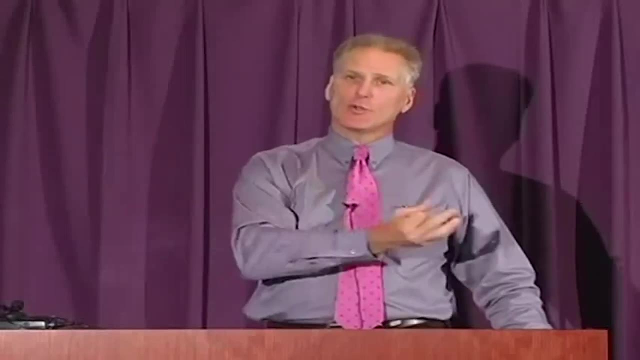 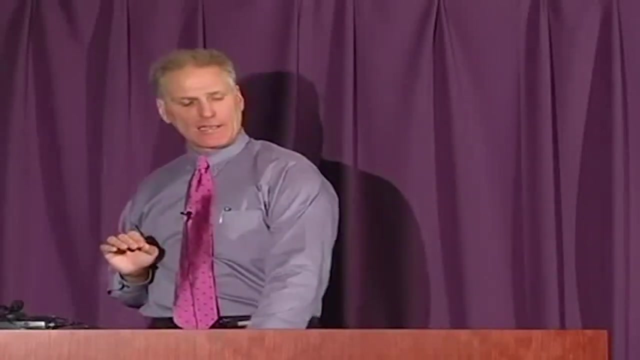 vacuum pump, You can have the world's biggest surge tank, But that little surge, that little evacuation line running from your positive model or your molding manifold to your evacuation tank can choke off your system. So you have to have an adequate, designed evacuation line as well. 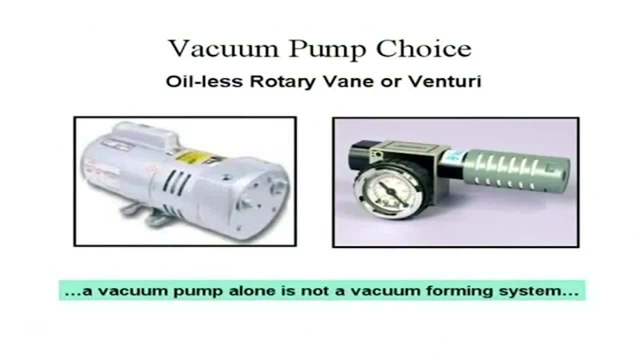 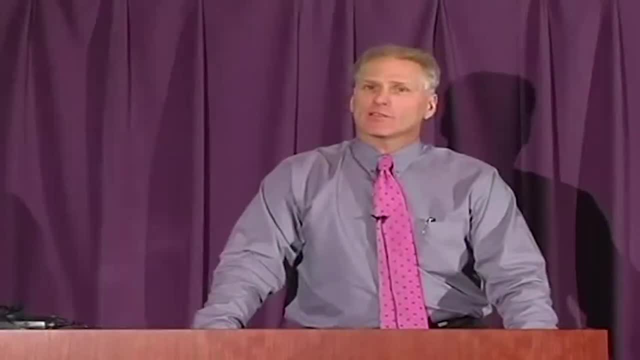 In terms of a vacuum pump, I like to say: a vacuum pump alone is not your thermal forming system. Yes, it will make a sucking noise, but it certainly is not a system. It might be the heart of your system, but it certainly isn't the 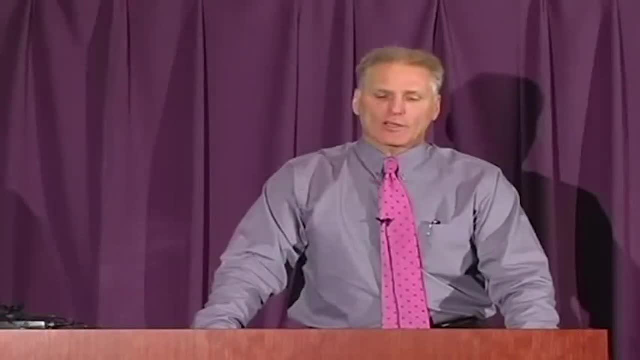 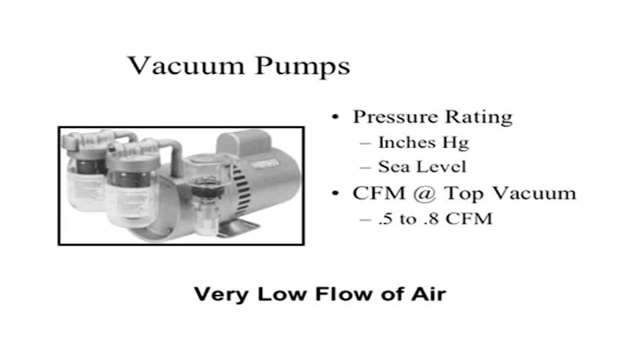 vacuum system alone. Many labs use an oil-less rotary vane pump. Some labs use a venturi pump. In terms of vacuum pumps, one of the inadequacies of the pumps is that they only create a very low flow of air, typically 0.5 to 0.8 cubic feet per minute. 0.5 to 0.8 cubic. 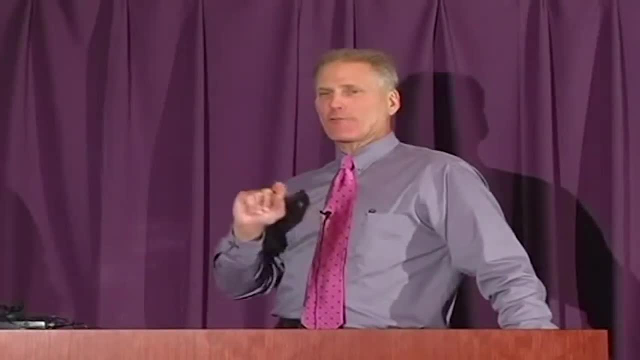 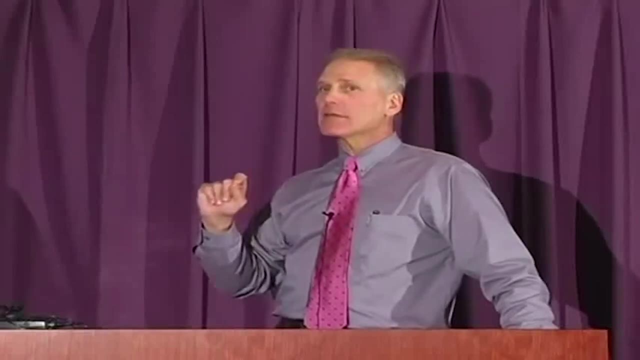 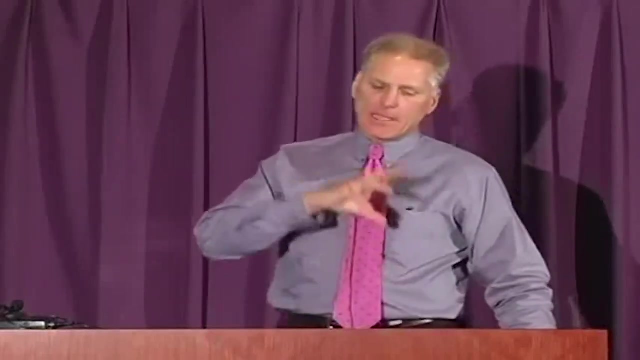 feet per minute. Remember I said that the standard for our field should be a minimum of 430 cubic feet per minute. That's why a vacuum pump by itself is a very inadequate system. It's only the heart of your system, not your vacuum system completely. 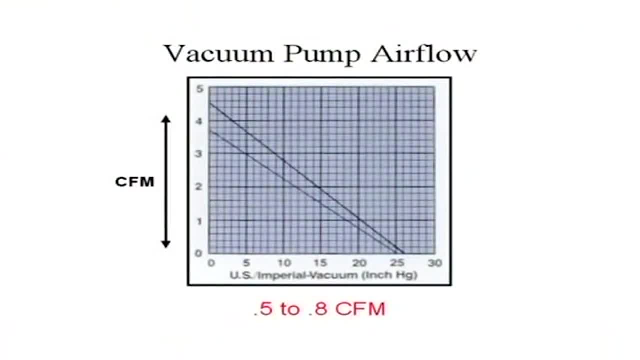 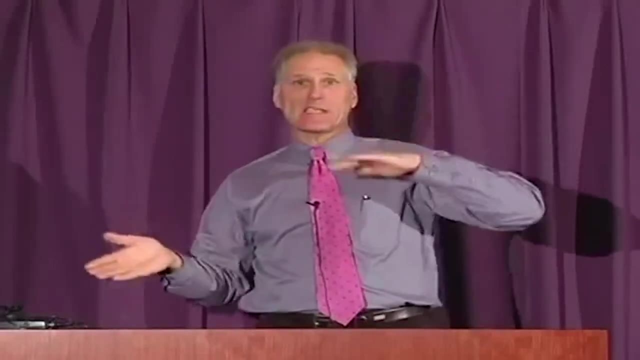 And then a vacuum pump, of course, can only draw so much. As it gets closer to that perfect vacuum, the flow of air slows down, So a vacuum pump at the higher range of vacuum actually becomes slower, So it doesn't have a consistent CFM across its whole spectrum of vacuum pressure. 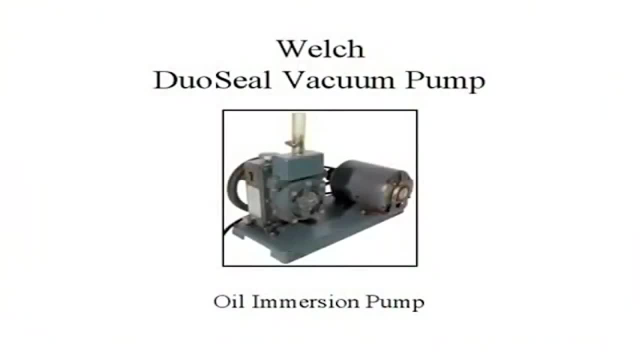 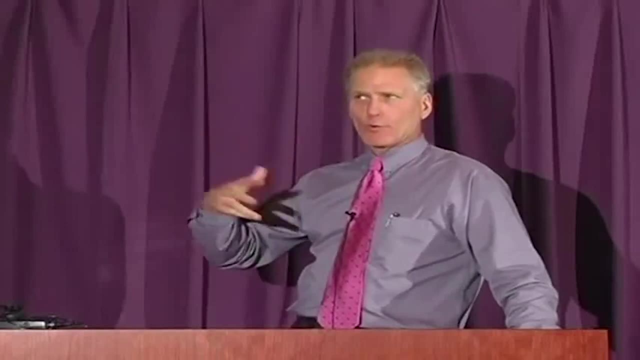 It decreases over time. The pump I like to use is a Welch DuoSeal vacuum pump. There's other companies that make them, but Welch is probably the best known of this oil immersion rotary vane pump, So it does have oil. The rotary vanes are immersed in an oil bag. 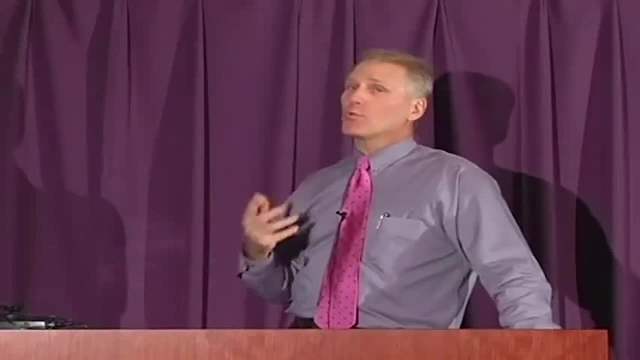 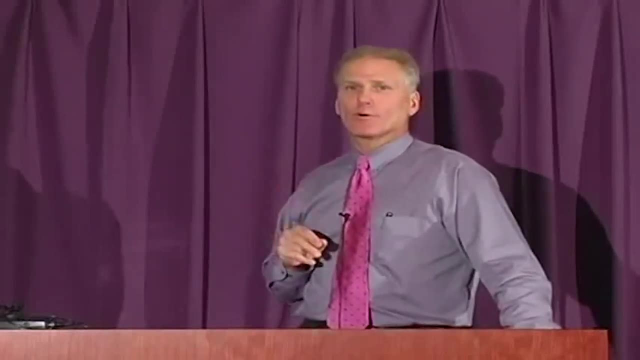 It's a very good pump. It's a very quiet pump and it will pull one atmosphere of pressure. That's why I like these pumps. Two reasons: One: they're quiet so I don't like noise in my lab. Number two: it will pull a full vacuum, a full atmosphere of pressure. Typically venturi pumps. they lose a little bit of efficiency because you're using a compressor to drive through the venturi to create the vacuum, So they will not pull one full atmosphere of pressure. And the rotary vane pumps even though they're low maintenance- two reasons I don't like. 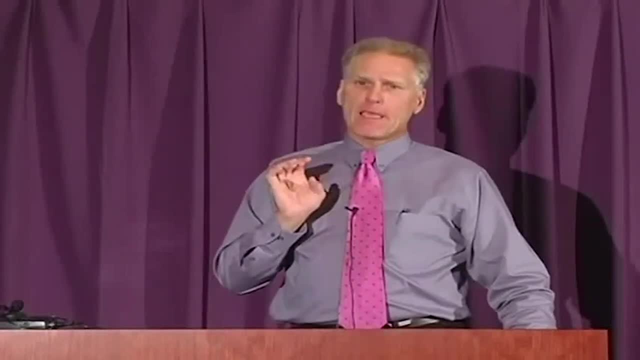 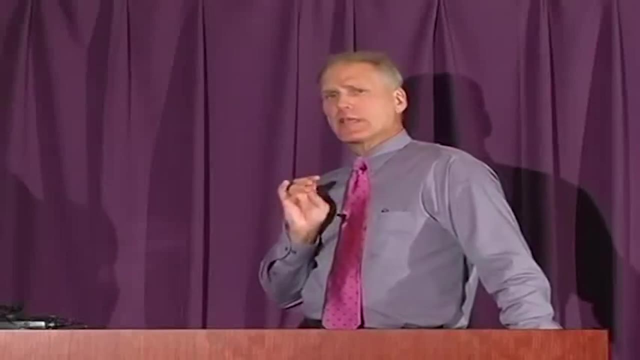 them. They're very noisy and I just don't like the amount of noise they make, and they have a lack of efficiency. They have a mechanical loss where they will not pull a full atmosphere of vacuum. Typically, you'll lose anywhere from one to two inches of mercury, and if your lab's at 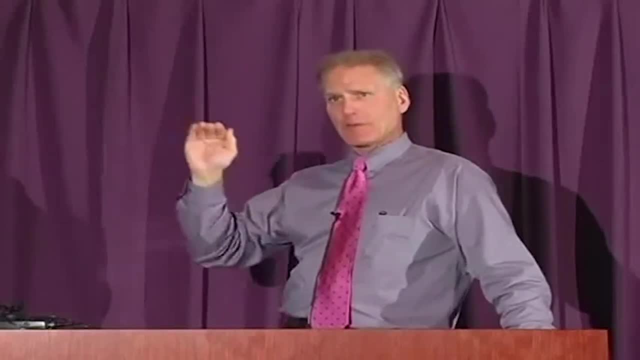 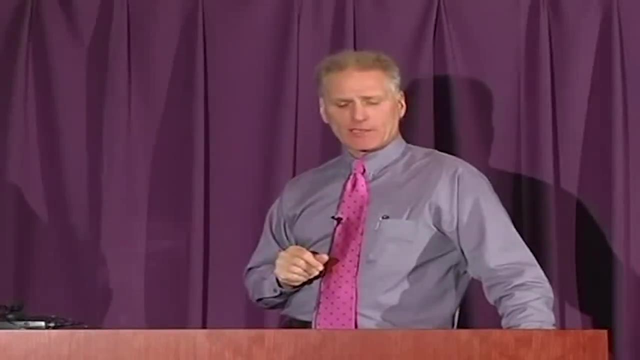 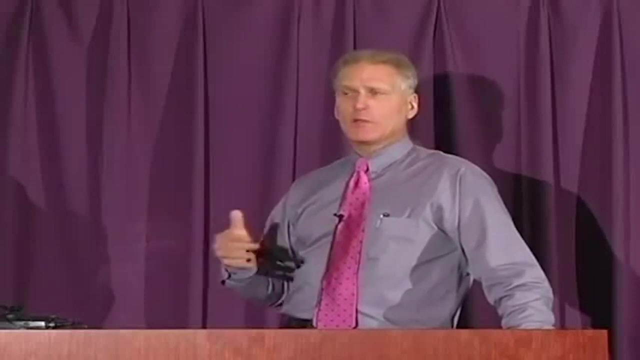 a higher level. losing that one or two inches of mercury can make a big difference in terms of having very good intimate thermal forming during your molding process. So I do like the vacuum pumps. They're very They're very durable. I think the one that I have is probably 35 years old and I picked it up in an equipment. 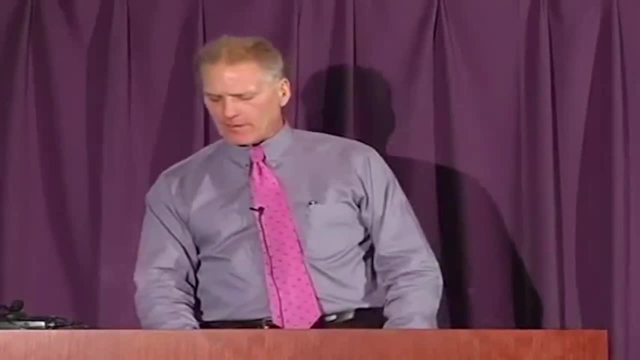 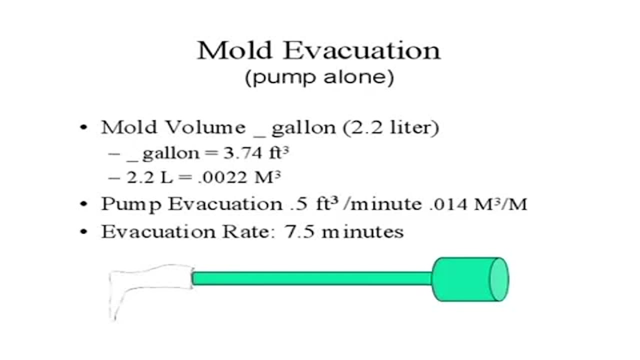 trade, but it's quiet and it will pull a full atmosphere of vacuum If you depended on your pump alone. we did this little mathematical exercise a couple years ago where we figured out what the average volume of the biggest positive model we would have in our lab, how much air we would trap under that plastic once we sealed it. 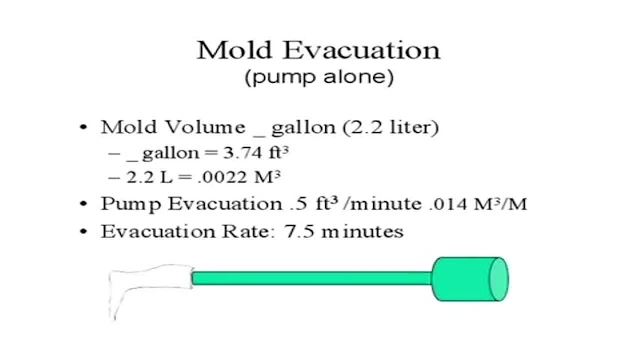 And then how much time it would take in order to evacuate all the air out from underneath that sealed plastic in order to reach the maximum vacuum pressure of the pump, And we found that evacuation rate would take seven and a half minutes, Right, Seven and a half minutes. 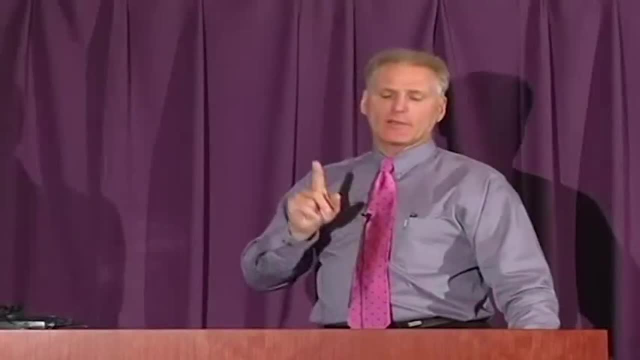 We did that mathematically, following the formulas in Dr Throne's book, and remember Dr Throne was the one that looked at one of our videotapes- one of my videotapes of our process- and said it should be done completely. 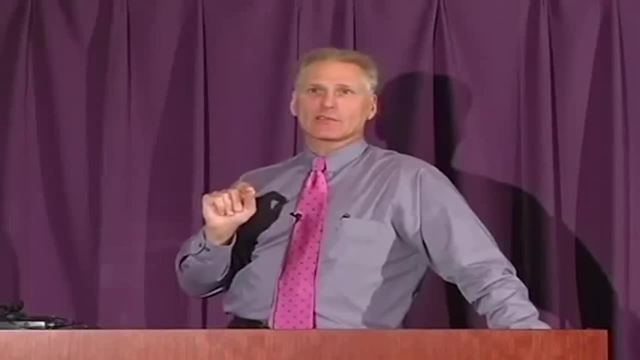 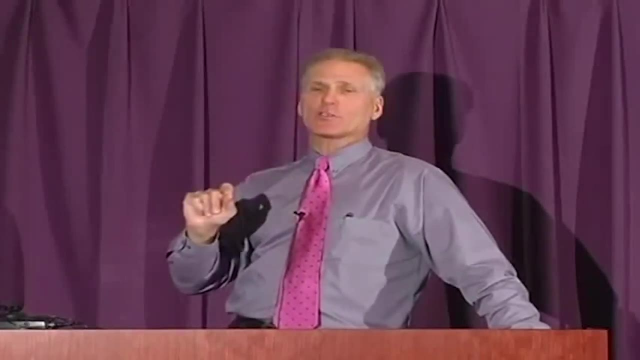 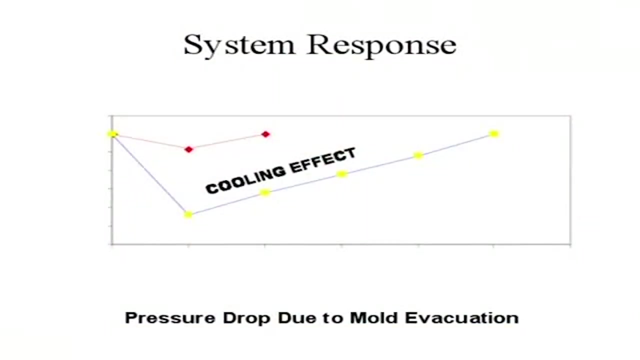 Dr Throne, Completely in 25 seconds, 25 seconds. So again, if you do not have a surge tank, big evacuation lines, you're not basically doing your production according to standard industrial guidelines. Your system response- how quickly you can evacuate the air- shows on this graph what 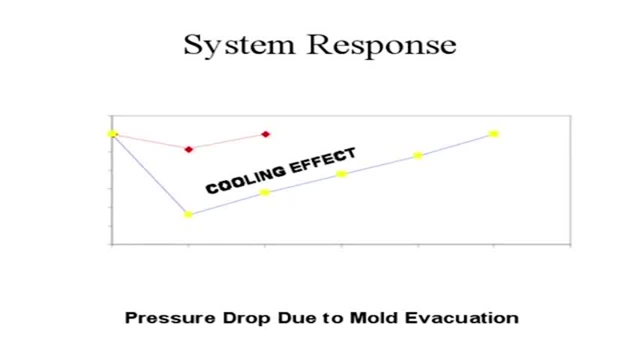 happens when you're using just a pump alone or if you have an adequately designed system. The blue line represents a pump alone. As soon as you crack the valve, pressure down, Pressure drops and then it keeps reaching that vacuum pressure and it'll go up to. 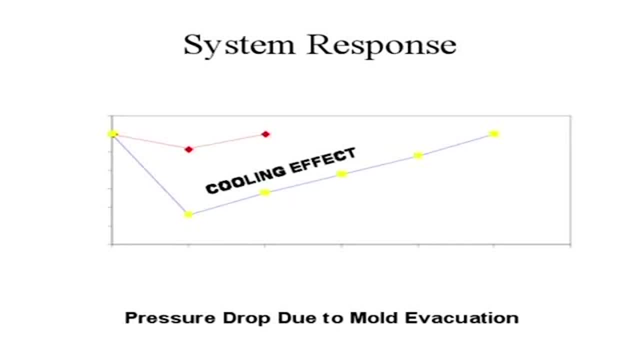 as I said, seven and a half minutes And this exercise was two and a half minutes In the red line. that's basically one with an adequate system. Within less than a minute it comes up to full pressure, vacuum pressure level that. 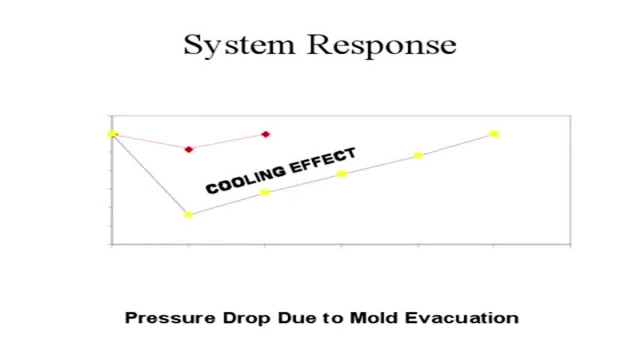 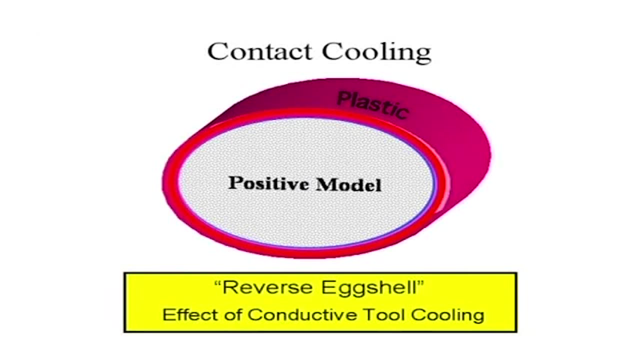 can be generated by your pump. Typically it's- I find it's- less than basically 15 seconds for the most part, Again, goes back to that whole concept of that reverse eggshell: The quicker You can put that plastic into your definitive shape, the better off you are. 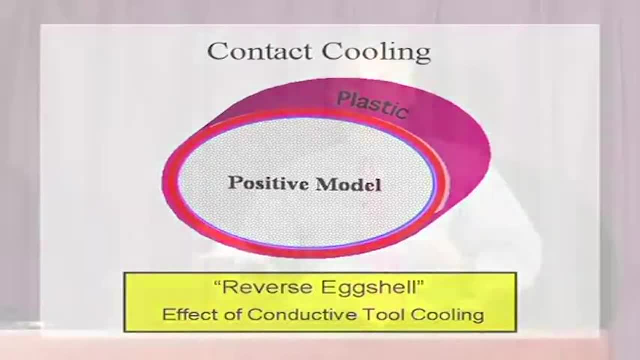 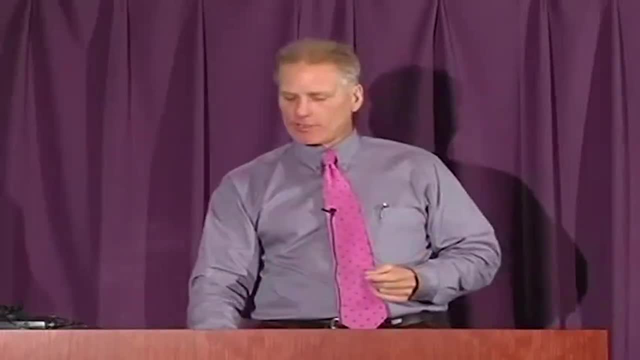 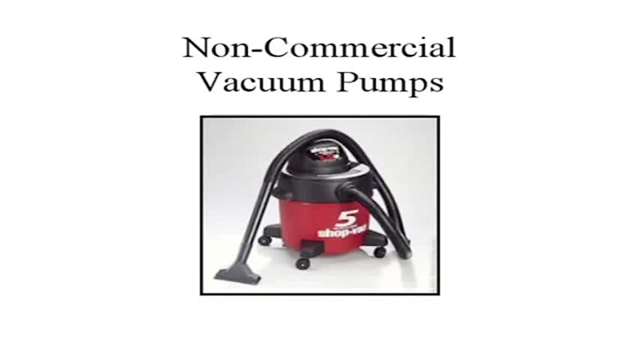 The longer it takes, the more of the likelihood that you're going to have that reverse eggshell with that inner layer. plastic that stiffens up is going to prevent the intimate molding of your plastic. I've seen some places use shop vacs: High volume, low pressure. 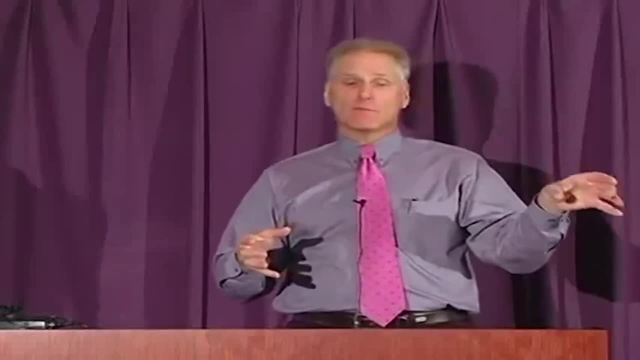 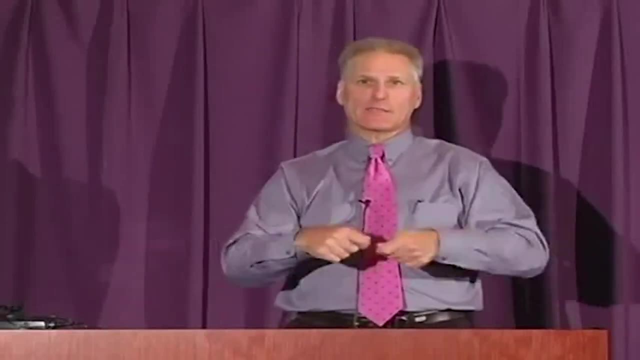 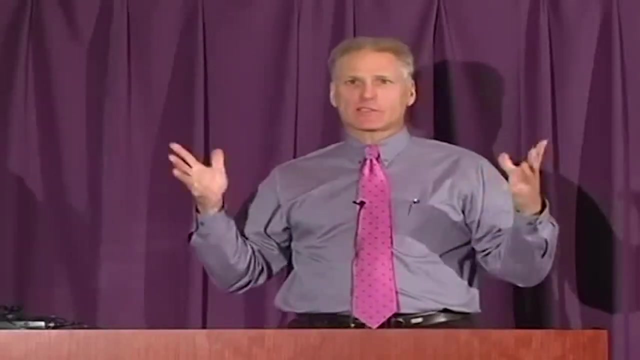 They're inadequate. I've seen some labs use a vacuum shop vac Okay, Along with a oil sorter, evade pump, all connected to the same pipes because they move a lot of air and have high pressure. That just gets too complicated. It's easy just to build a system from the beginning that's adequately designed for what. 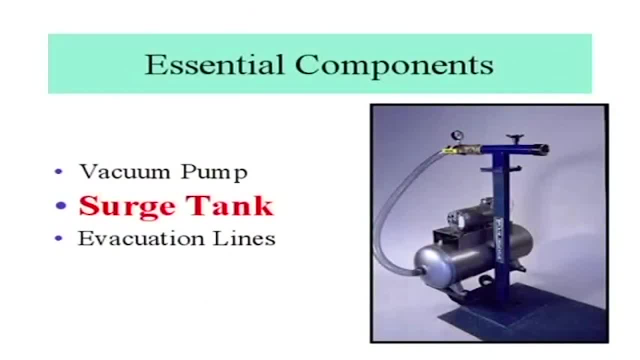 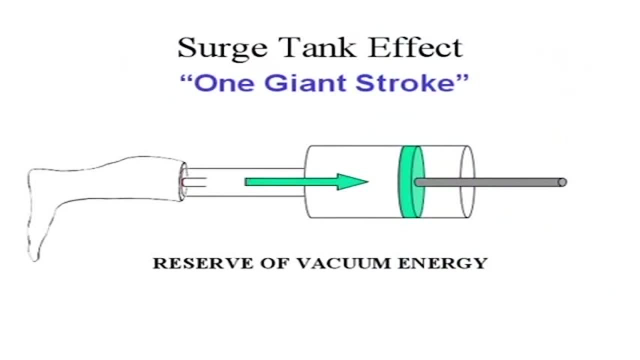 you want, And your essential components are a vacuum pump, a surge tank and, of course, your evacuation lines. We'll take a look at the surge tank first. Your surge tank is more or less a mimicking type of effect. It makes your system act like you have a giant single stroke pump. 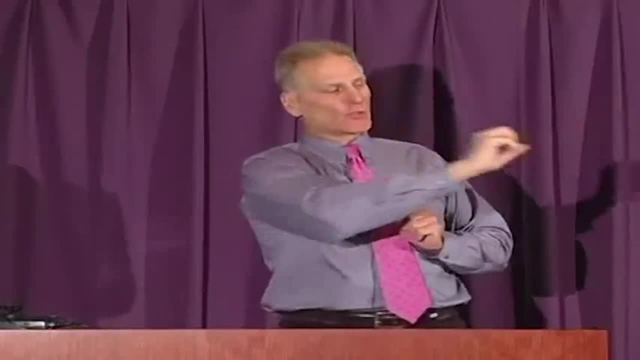 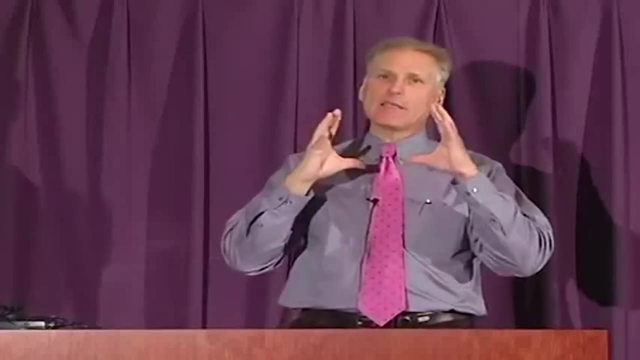 So that way there, if you flipped on that switch, that pump would just go whoosh and pump all that air out. That's what a surge tank is, Just like having a big piston sucking all that air out. It gives you that adequate reserve of vacuum energy. 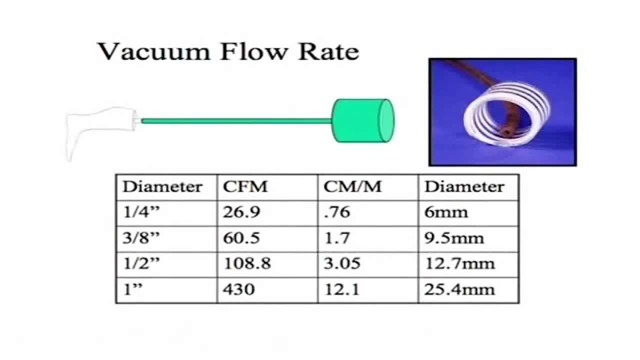 Your evacuation lines have to be of an adequate size. This shows lines at a quarter inch, three eighths half inch and one inch. Okay, At one atmosphere of pressure, which would be 29.92 inches of vacuum pressure a quarter. 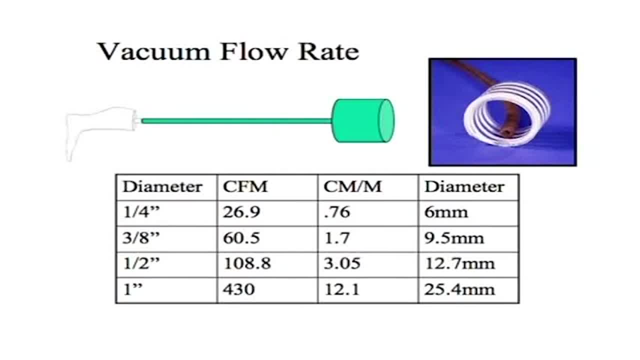 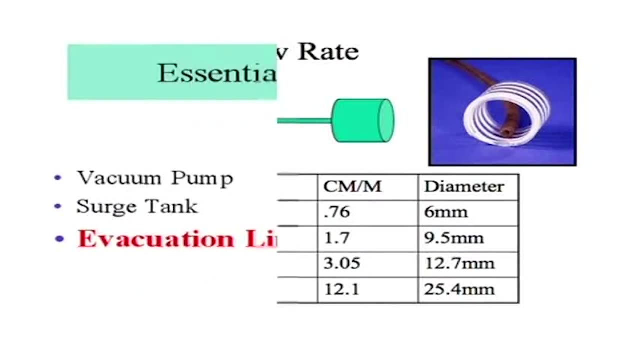 inch line will only move 26.9 cubic feet per minute. Our minimum is 430 cubic feet, which is a one inch diameter line which should run from your molding manifold to your surge tank. That's the smallest you should run. Bigger than that is fine, but that's the smallest that you should run. 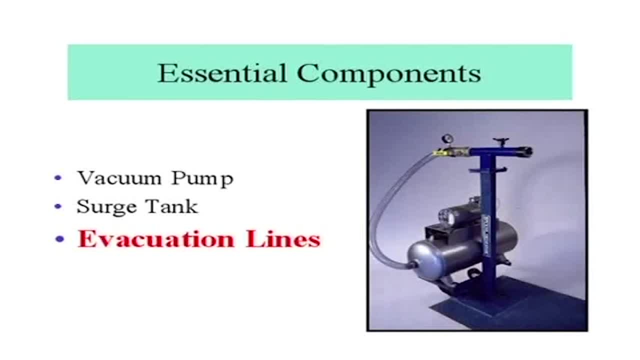 If you have a small line running from From that molding manifold down to your surge tank, this basically acts as a choke. A small line, as we talked about, that quarter inch line, will just not give you the flow that you need to evacuate the air from underneath your sealed plastic within that 25 seconds. 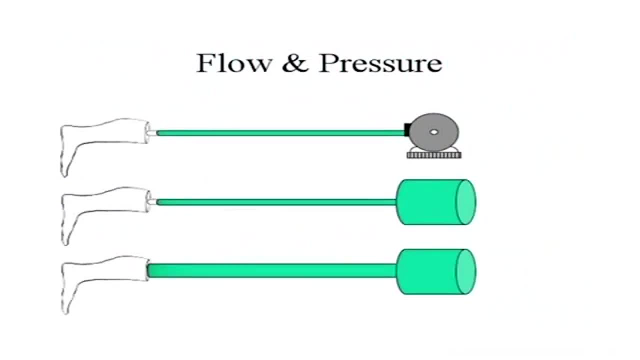 You have to have a good sized line. This is what I- This is a sketch I put together. that's representative of what I see in the field. Sometimes, a small line running to the surge tank, Running directly to your vacuum pump. That's not a system. Small line running to your surge tank still an adequate system. I see that mistake done quite often in labs. Well, they will have a surge tank, but very small lines. The reason that's done is most tanks are made to a pressure standard. 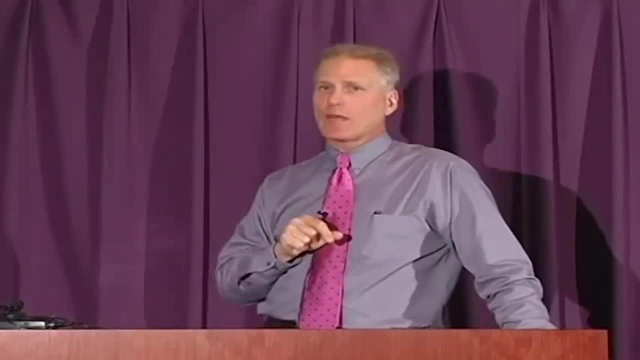 Their biggest outlet might be 3 eighths of an inch. Three eighths of an inch will not move enough air, especially after you screw in a barb fitting in there and have a line on it. It's just too small. 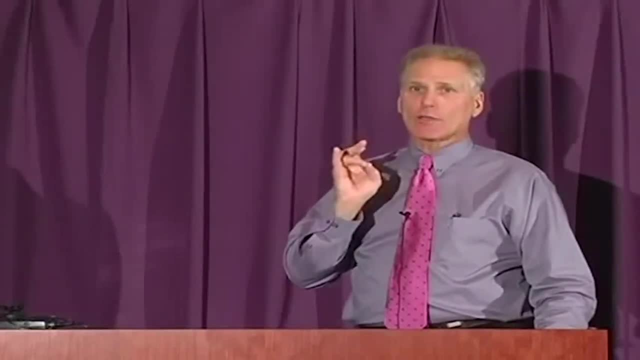 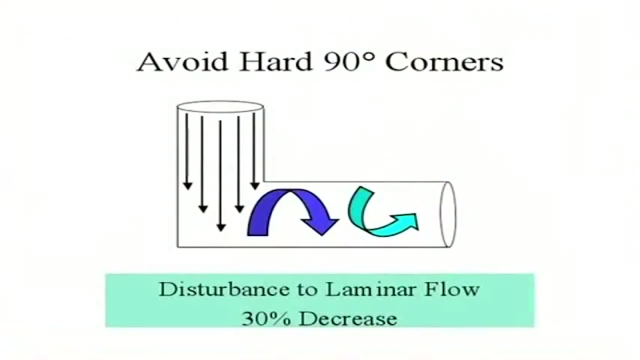 You have to have a vacuum pump, Vacuum tank that has at least a one inch outlet on it so you can use adequate line. And that's the schematic on the bottom Big evacuation line going to your surge tank. Try to avoid 90 degree corners. 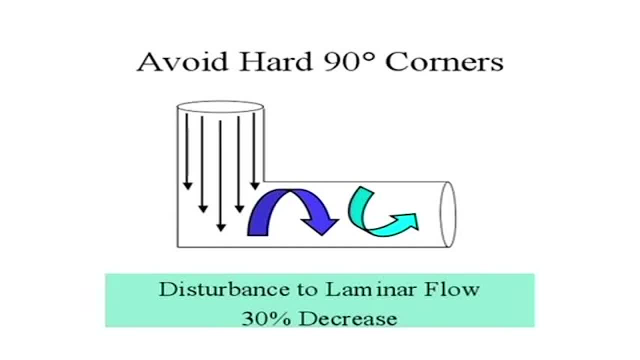 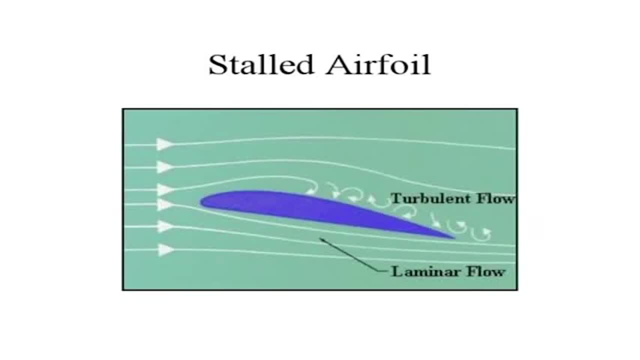 They basically disturb the laminar flow by 30%. It just slows down the flow of air within your lines. It's all based on that: laminar flow versus turbulent flow, Look like an airfoil on an airplane- and it just slows the flow of air within your lines. 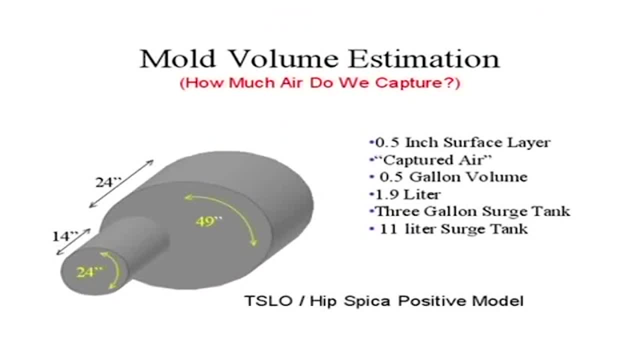 In terms of our mold volume. We looked at what would be the largest TLSO that we would have in our lab, which would be a TLSO hip spica positive model with a 49 inch diameter. We found that we would evacuate probably a half inch of air off the top of that total. 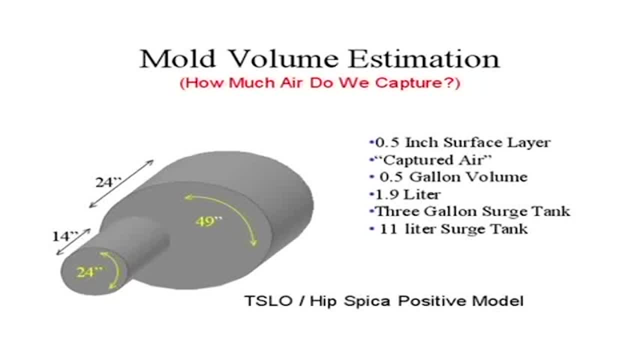 area. So we felt that a three- about two and a half to three gallon surge tank was what we wanted to have as a minimum Right. So a three and a half gallons to three gallons is adequate for almost anything that you would have coming to labs. 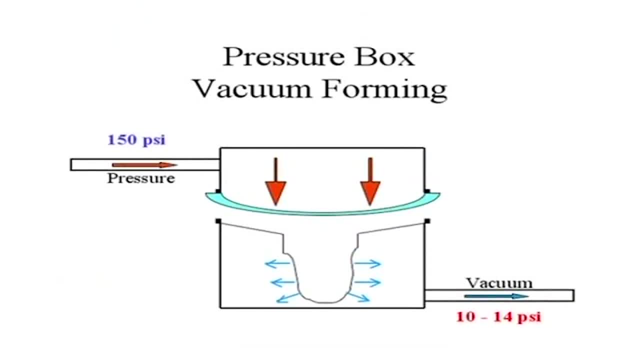 It's not a big tank by any means. As I said, on the industrial side many times they're using pressure on one side of the plastic and vacuum on the other side, because they find that vacuum alone many times is inadequate. So that's why they use compressed air. 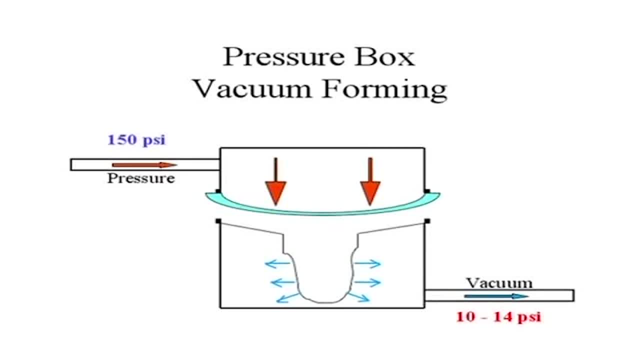 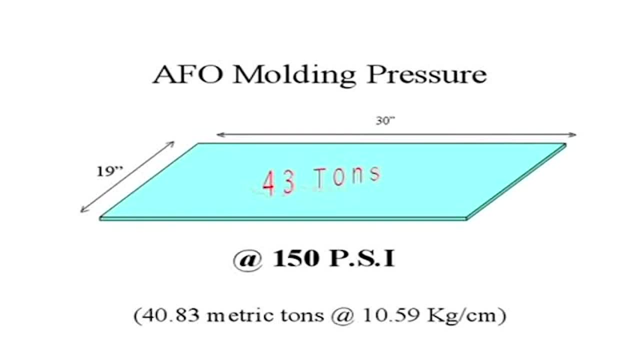 They use compressed air, high pressure, 150 PSI on one side of the plastic but still draw with vacuum on the other side. All we have is vacuum Differential. Differential might be up to 10 times 15 PSI versus 150 PSI per square inch. 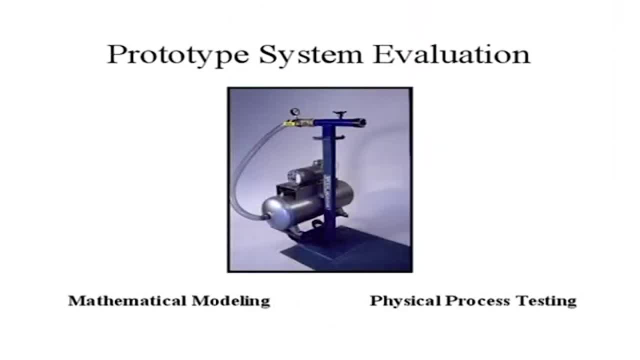 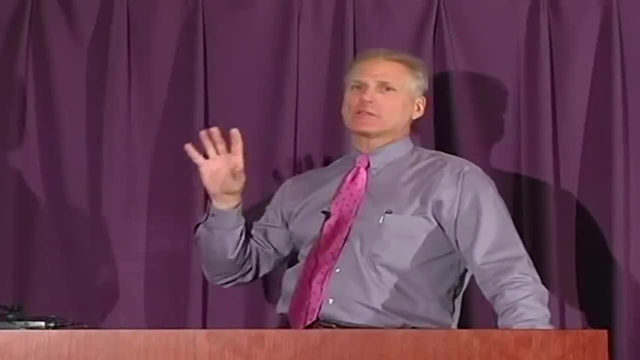 Huge differential from the industrial side to what we're doing In terms of looking at a prototype system we put together because when we started looking at our systems there was nobody in the field internationally that was creating thermal vacuum forming systems that were designed specifically to industrial standards. 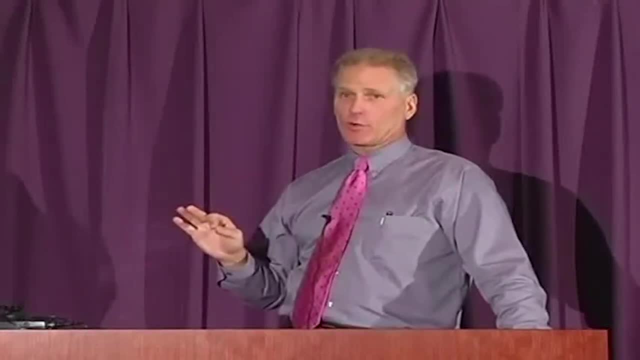 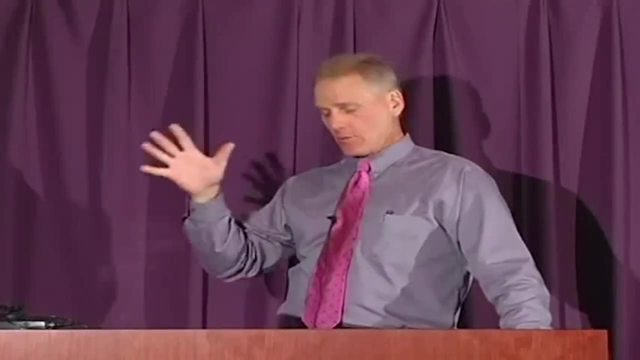 We were the first ones to do that. as a company, We typically don't build equipment, but we had to at this point in time and we initially built these prototypes for our own internal use at first. Then, when we conducted these lectures, ironically, regionally folks- practitioners- started to 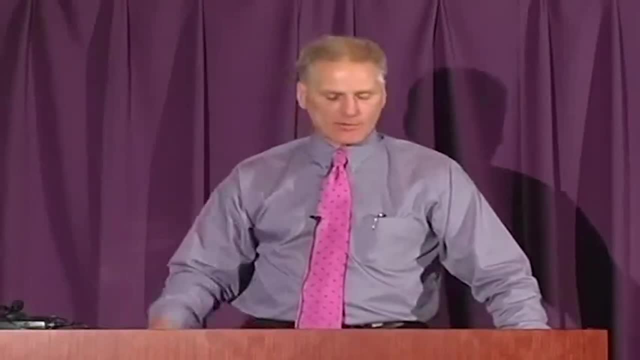 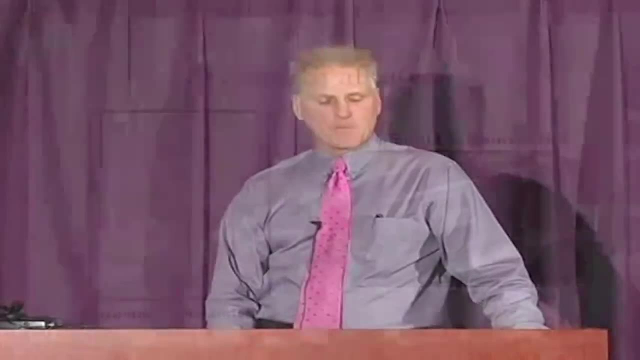 ask us: why don't you just produce the equipment? so that's how we got into the equipment side of it besides the componentry that we made. So we went through our mathematical modeling, Then we went through our physical process testing. We did produce a full mathematical model. 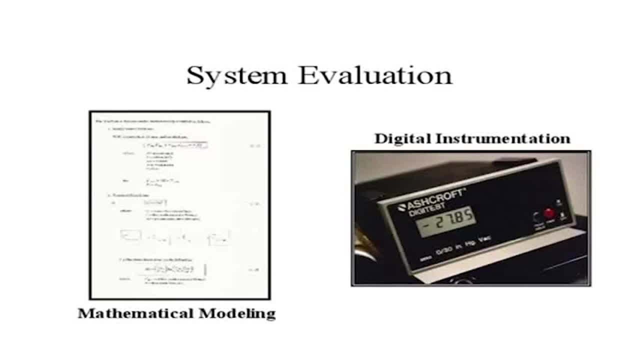 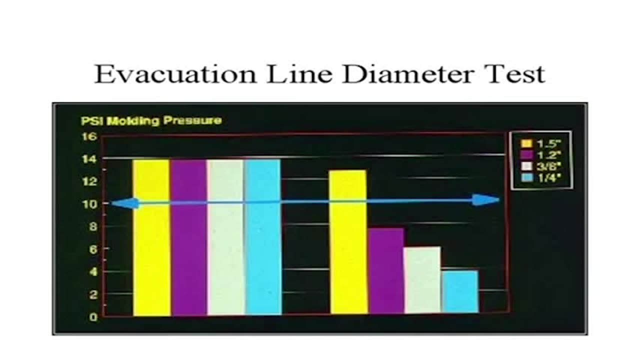 Based on the formulas that were in Jim Throne's book. We then had a custom digital vacuum gauge made that would hold to two decimal places and record basically the drops in vacuum pressure In some of the testing we did. I won't go through everything, but I'll go through this. 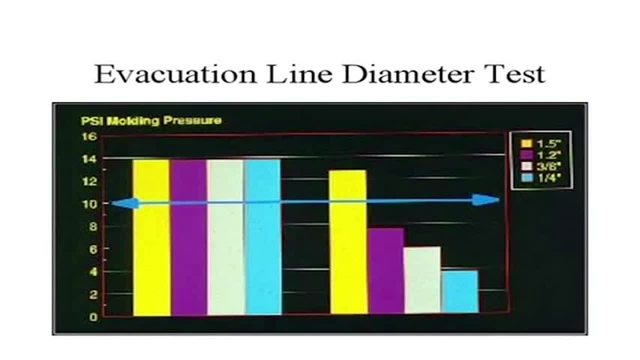 one. This was a test to show the drop in pressure within your system dynamically when you cracked your valve in order to conduct a thermal forming test. We did it at Long Beach Lines at quarter inch and then half inch, three-eighths inch and a half, one inch actually. 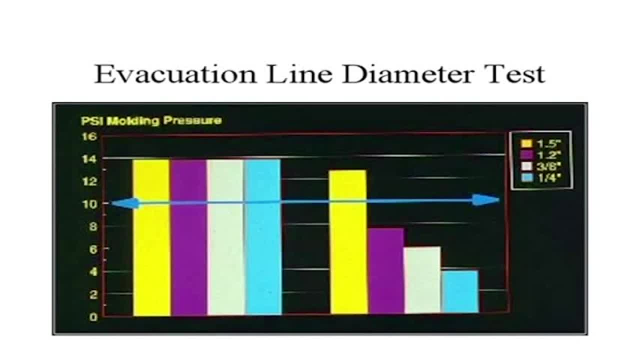 And then the blue arrow across is the 10 psi minimum. So when we cracked the valve, basically the only system that worked is when we had an inch and a half line. The half inch, three-eighths and quarter inch all dropped below that 10 psi minimum. 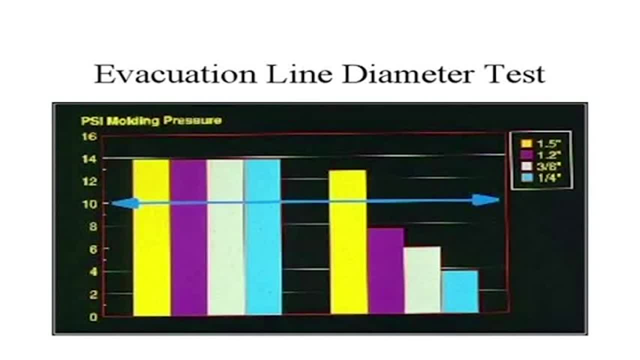 That means for a certain amount of thermal forming process. that dip in pressure from system response put us below the 10 psi minimum That's recommended by the polymer engineers in order to have adequate thermal forming. So that was one test we did in our system. 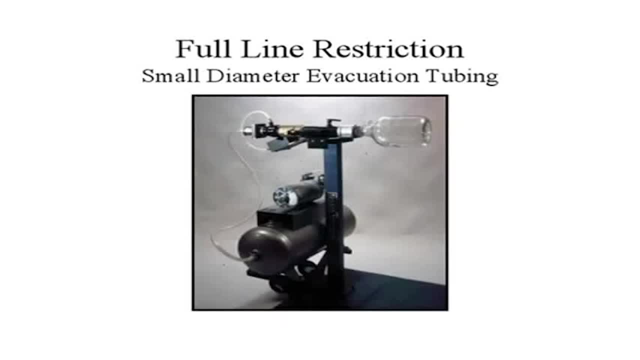 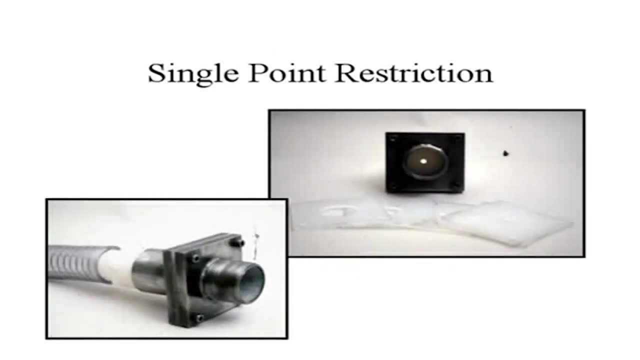 We ran standard size mold, We changed the evacuation lines running from the surge tank down to our molding manifold And then we also tested, basically, point blockage, putting a baffle system in with little holes, basically at the same size diameter as the line, so we could show single point blockage. 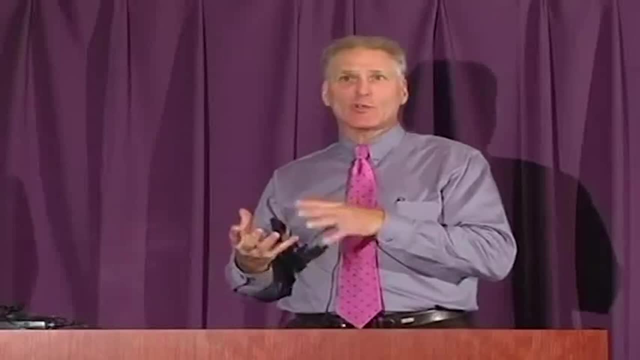 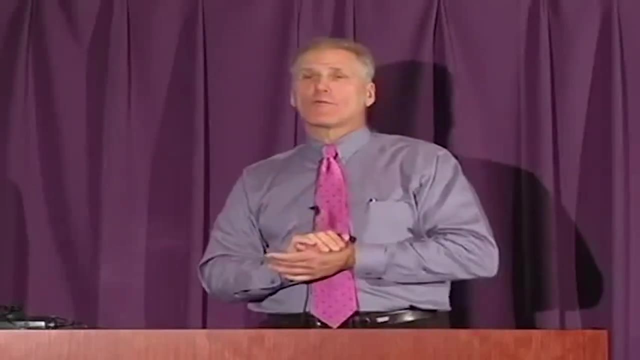 That way there. if you, If your system ingested a piece of plaster, we would show that the degradation in performance of the system because of a blocked line. So make sure you do maintenance on your thermal forming system to make sure that it hasn't. 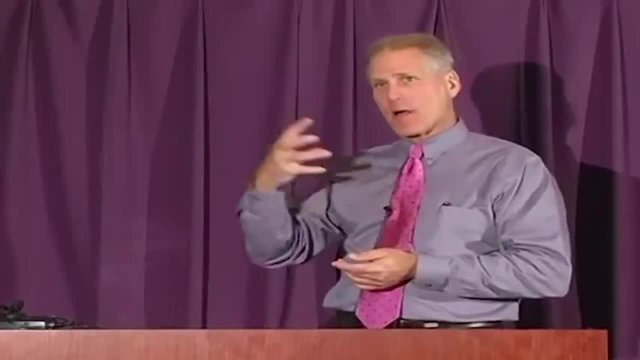 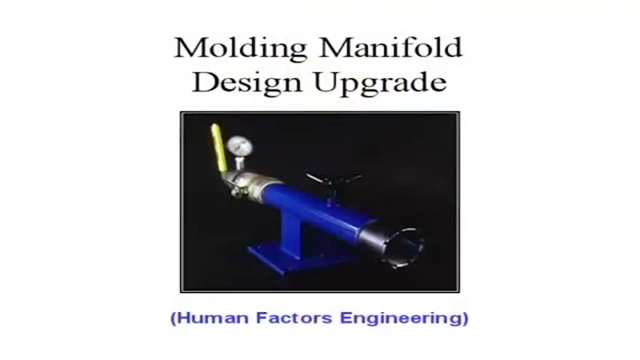 ingested a piece of plaster that has a remnant of a positive model and lodged itself within your system, choking it down. So we ran the full dynamic tests Once we got through the basic testing. then we started looking at manifold upgrades, how we could enhance that manifold. 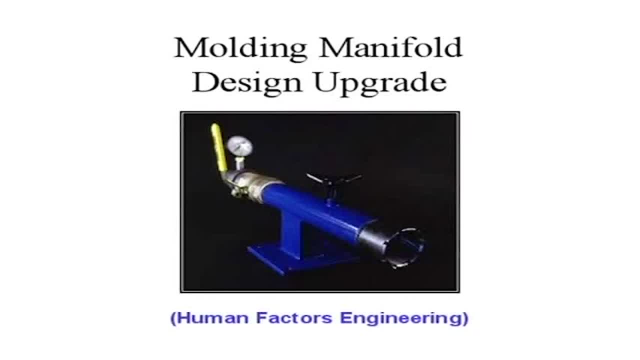 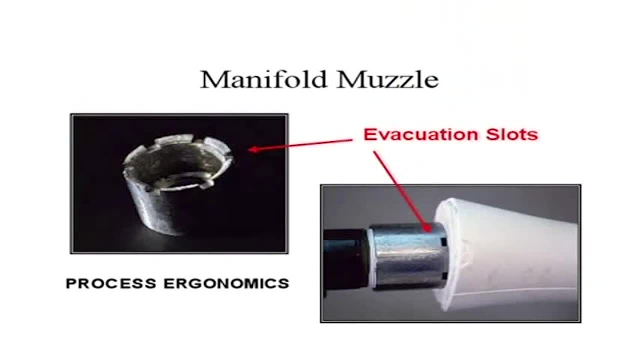 How we could make that manifold to help our technicians in terms of having repeatability and some process control. That goes into some of the human factors engineering. We put in a removable nozzle or a replaceable nozzle that had notches cut into the end. 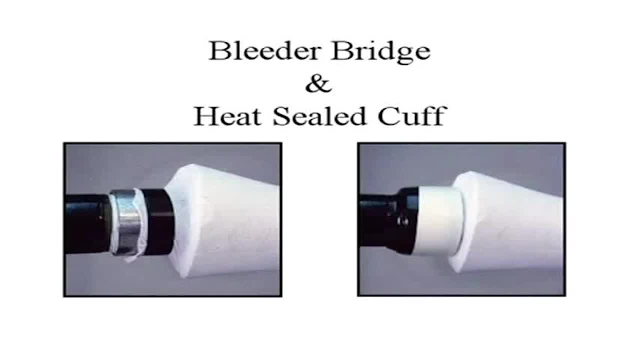 Those notches represented the same size volume as the line. We also use a foam cuff on the top. It's a polyethylene foam, which most of our foams are based on polyethylene. That Aliplast cup at the top Serves as a magnetic seal. 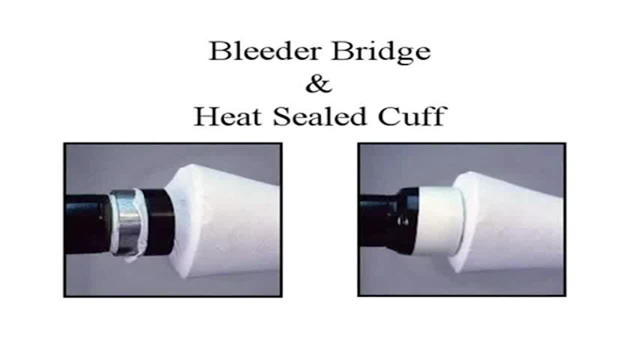 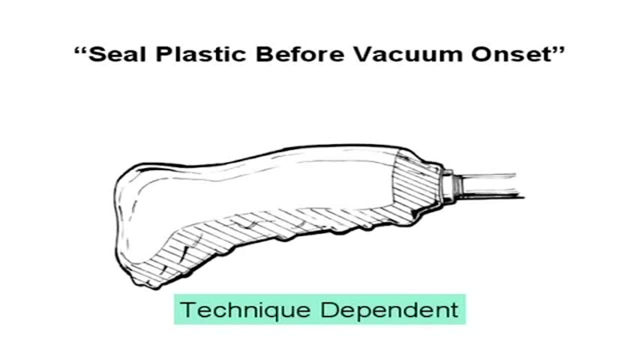 So when we seal our plastic to the top, the hot plastic seals to it, creates a perfect vacuum seal and prevents any leakage that could occur at that point in time. It also allows us to quickly remove the positive model from the manifold itself, because it's 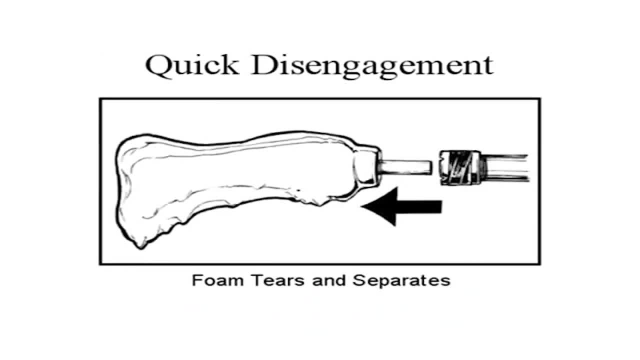 protected by that barrier foam. Loosen up your pipe vice, twist your model mandrel comes right off, because the foam will rip at that point and come right out. So it's very easy to remove it from your positive model. It doesn't get trapped. 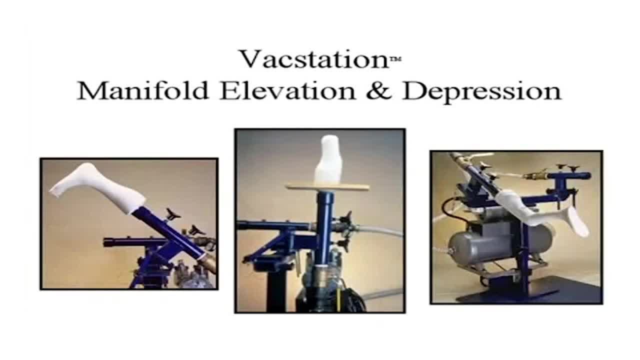 It's very easy to remove it from your positive model. It doesn't get trapped. It doesn't get trapped on the end of your molding manifold. This is our big system that we've sold for many, many years. One of the unique features of the system is that it's got a manifold that can change elevation. 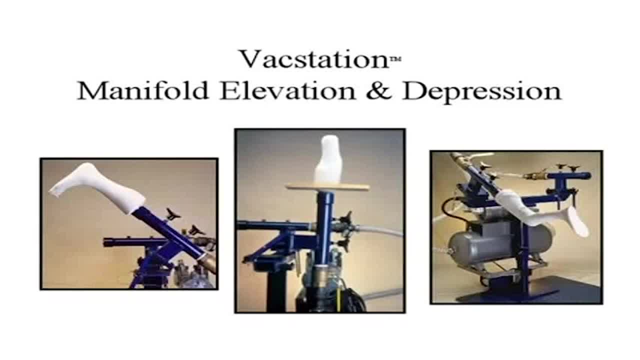 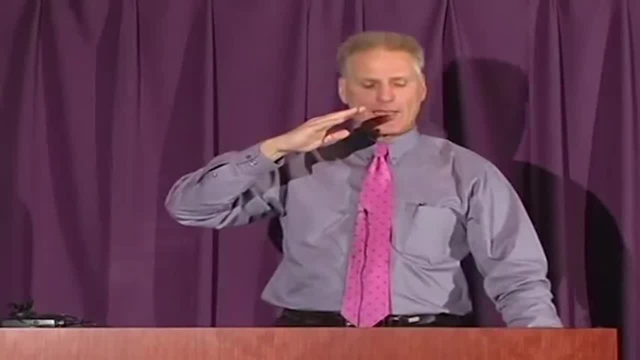 You can mold at a horizontal position. You can mold at a vertical position. for prosthetics, Some people like to mold their AFOs at an inclination. They say they get better control of the plastic draping around the ankle. And of course we can also depress the angulation. so if your vacuum foaming over a positive 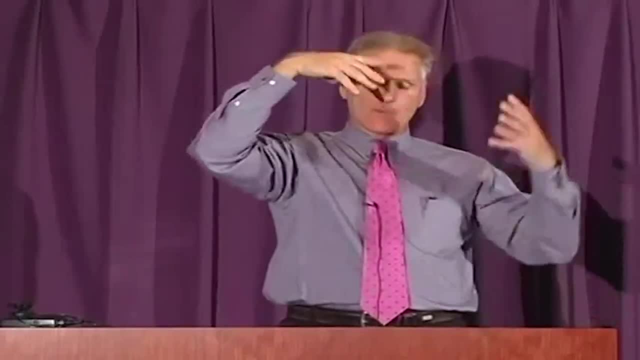 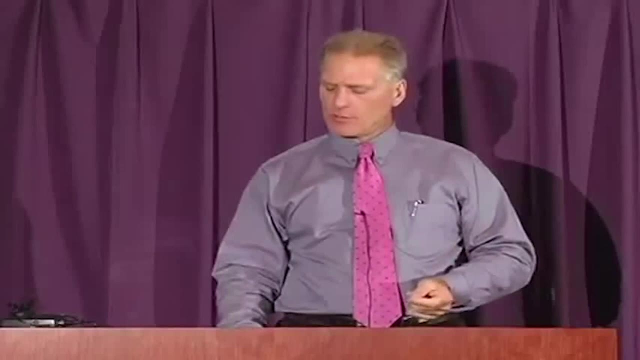 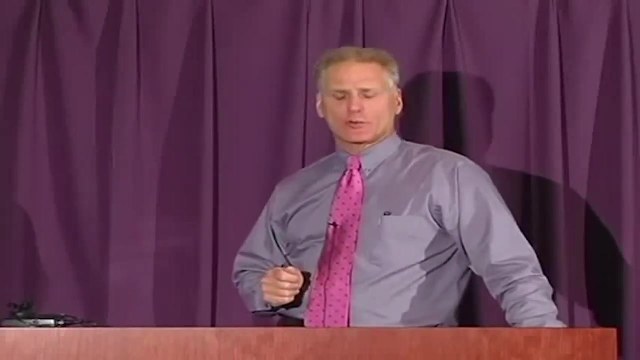 model has a knee flexion contracture. instead of having the foot in the air that might be at an unsafe working attitude, you can lower it down to a very safe attitude when you're manipulating that 300 plus degree hot plastic. As we made the system available, our international distributors indicated that the big system 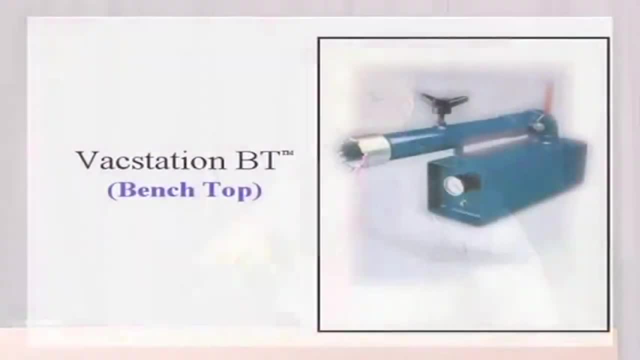 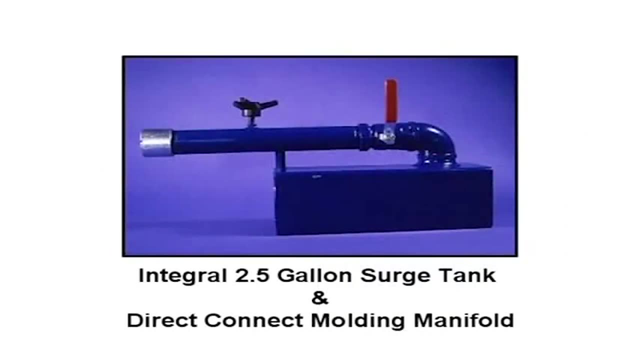 was too heavy to ship overseas, So I designed a bench top system, which really is my favorite system, primarily because it's a very small integrated unit. The surge tank serves as the base, The base of the molding manifold. you can mount that directly or bolt it directly to. 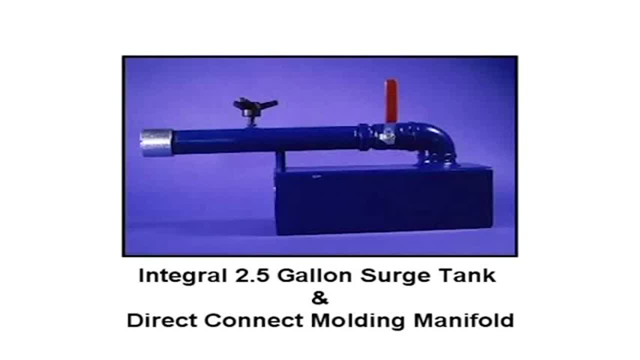 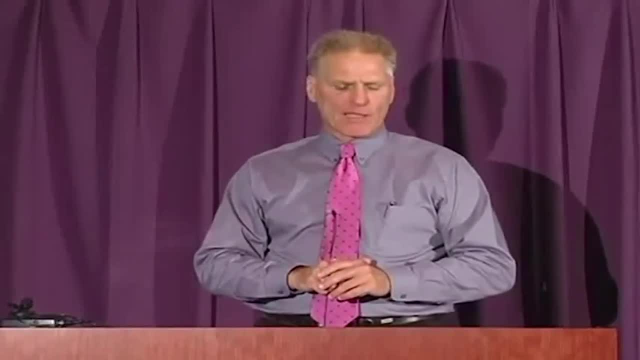 your workbench and then the molding manifold itself is directly connected to the surge tank. So we have a two and a half gallon surge tank. direct connection with the molding manifold itself makes for a very short draw to move the air from underneath the positive model. 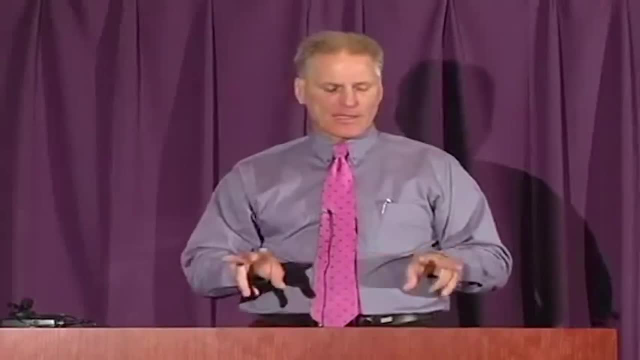 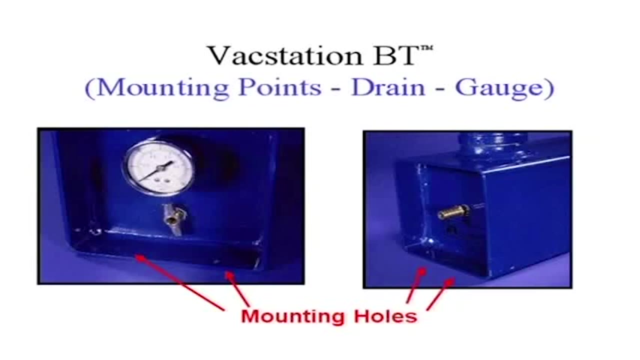 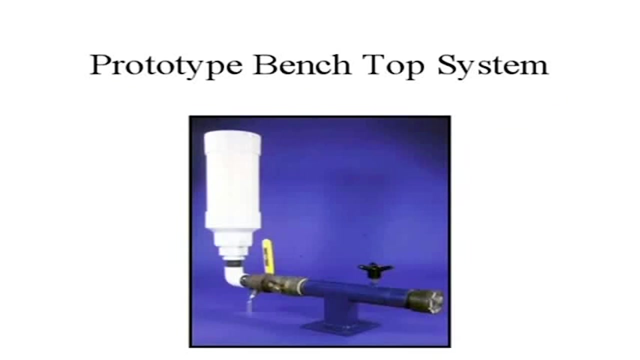 into the surge tank and it's a very, very quick acting system, Has mounting holes on the bottom, has its own vacuum gauge, has a clean out valve and also, obviously, an outlet for connecting your vacuum line to the system. That was just one of my prototypes in terms of working up the feasibility of having a 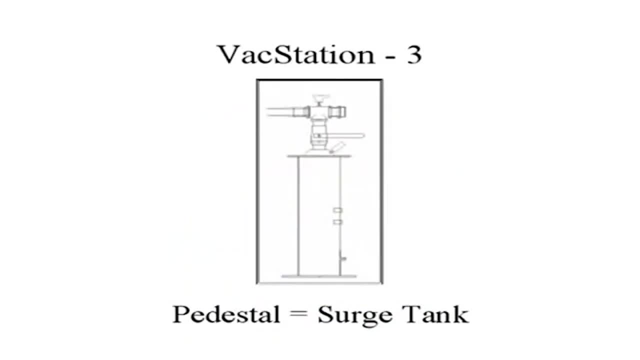 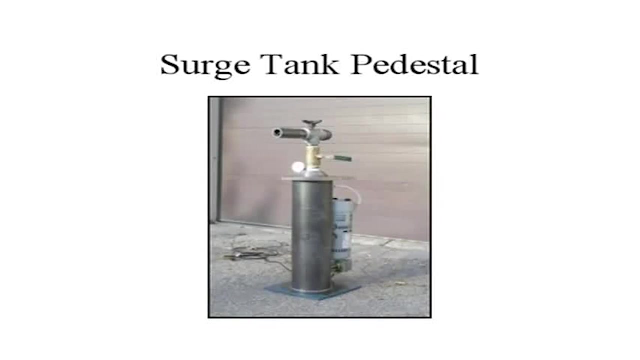 small integral surge tank. Recently, one of the engineers at Becker and myself went through a design exercise where we thought the concept of using the pedestal as a surge tank would create a very compact system, And so we did that. Here's our prototype. We haven't decided if we're going to bring this to market or not. 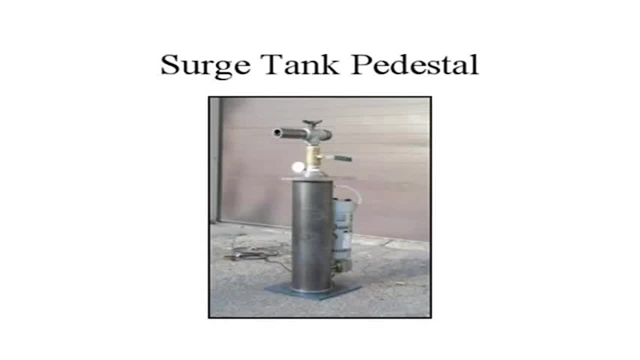 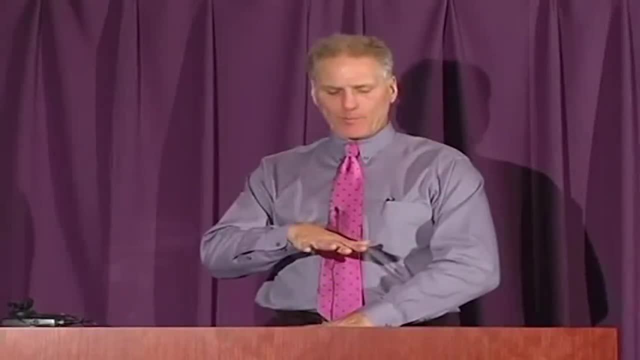 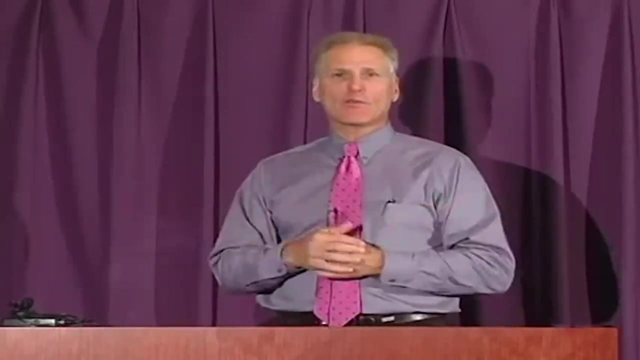 From simplicity in terms of space savings. this is going to be a methodology you're going to see more and more Using that steel tubing or square tubing, welded to a mounting base for the floor mount, and then a little tool platform at the top with putting your ball valve on top is going to. 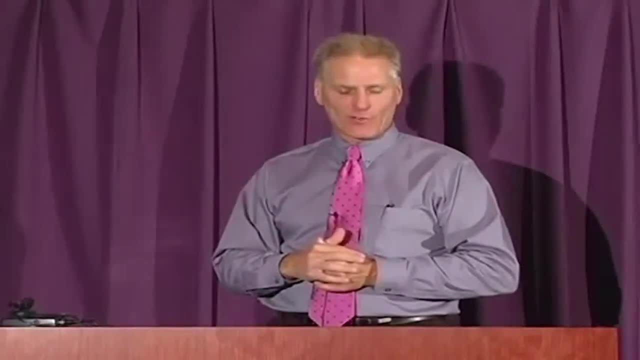 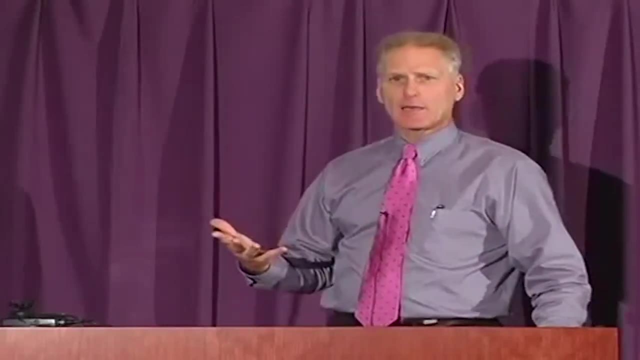 be a very adequate system. We use this- actually we use the prototypes in our lab for, at this point in time, for cream remolding helmets, but I think this is what you'll see more and more as being a very efficient and compact vacuum thermal formant system that's going to be very effective. 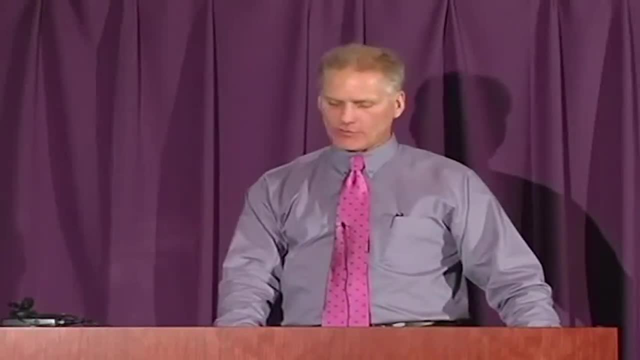 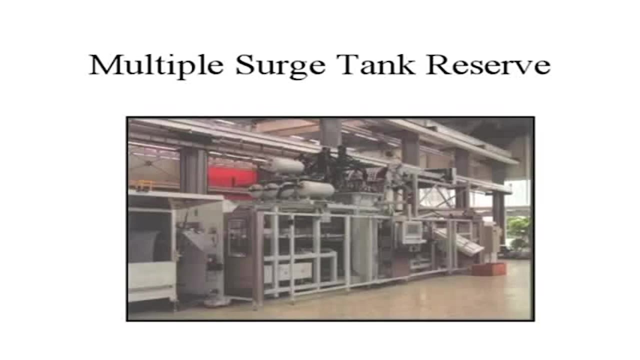 forming system that'll be used out in the field. so I have no doubt that you'll see it from a number of people. this is a very large go to the commercial side just to reinforce the aspect of how important surge tanks are. you can see on top of the this inline thermal forming machine that there's one. 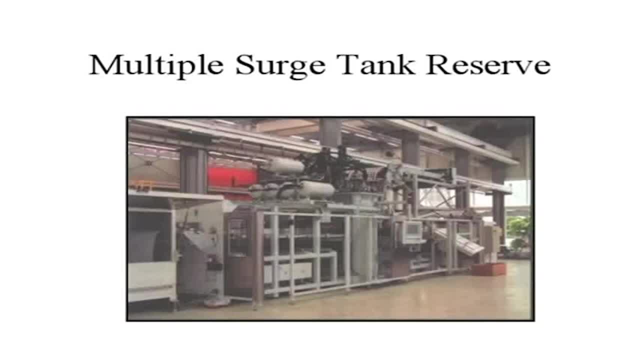 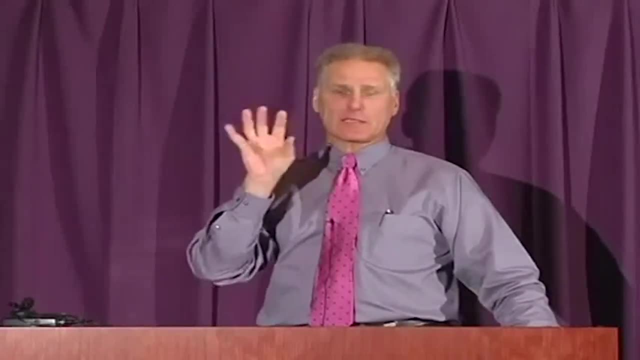 two, three, four, five large surge tanks and then also notice the size of the diameter of the lines connecting those tanks together: very, very large size. so that's all related to how much air you have to move from underneath the plastic that you've sealed on top of your positive model. so 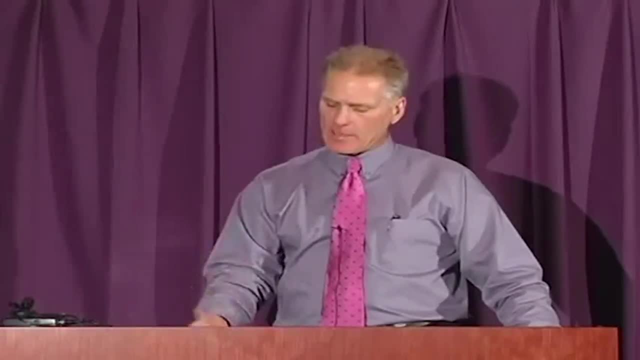 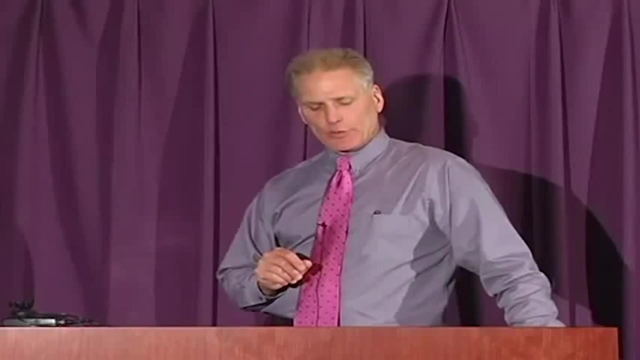 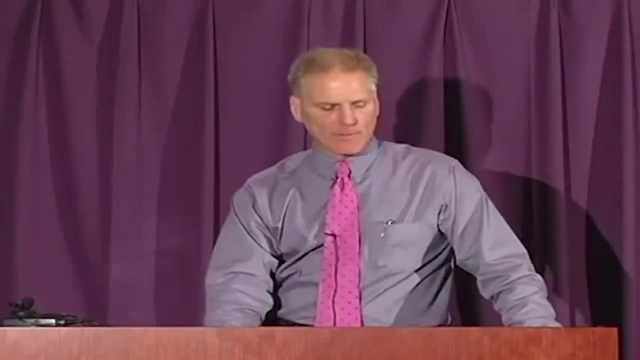 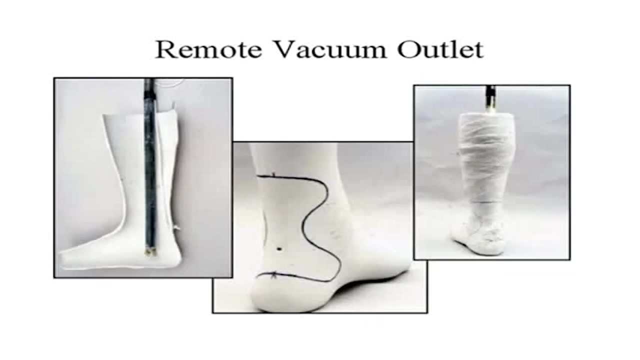 it's rather universal- of vacuum pump, surge tank, adequate evacuation lines. to give you one other little trick, this is something that I picked up out of a tooling handbook of how to make a vacuum outlet in a tool, especially plaster tooling. take a piece of vinyl coated clothes line and here I've got a bivalve cast to show that it's run. run it through a. 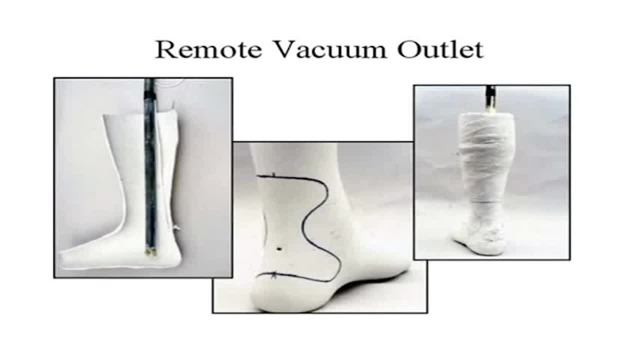 hole in your positive model where you want that at vacuum outlet. bring it up across your mandrel and tape it to your mandrel. fill it with plaster, just like you normally would, and when you strip your plaster away, cut the little knot. strip your plaster off and then, because it's made out of vinyl, it 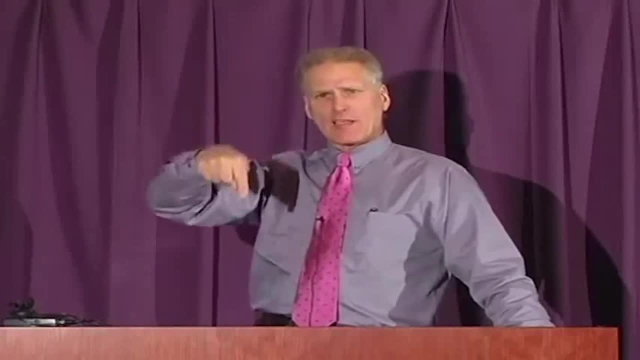 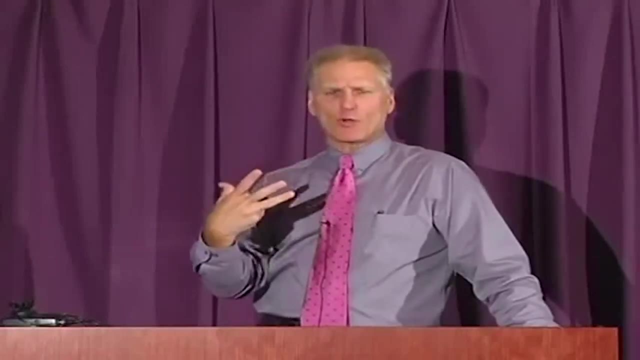 won't stick to the plaster, you pull it right out and basically you've now got a vacuum outlet all the way down to some specific point. in this particular exercise I was reinforcing this AFO with a layup of comp core right in the Achilles tendon area. I want a little bit more pull in that. 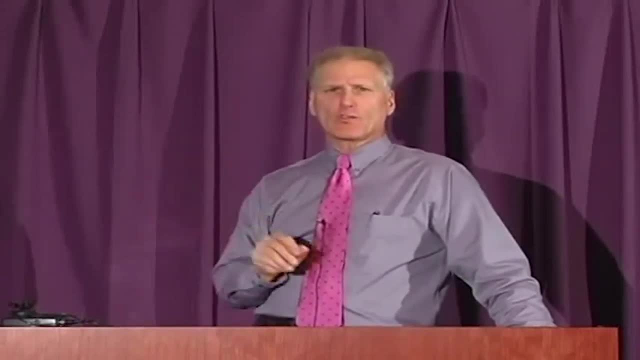 area. I think in prosthetics, if you're vacuum flowing with a valve in a thermoplastic liner that making sure that that valve is going to lock into the plastic, you could put this remote vacuum outlet there. so it's a lot easier than trying to drill down through your positive model, just put. 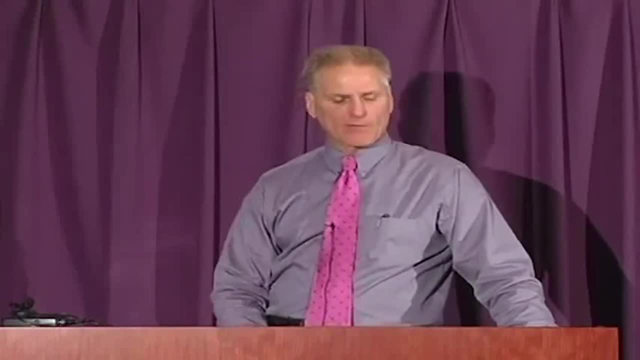 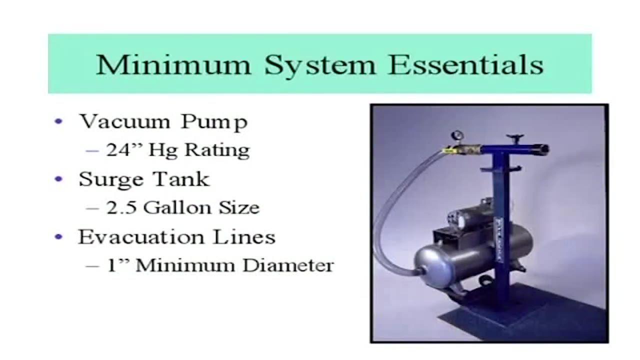 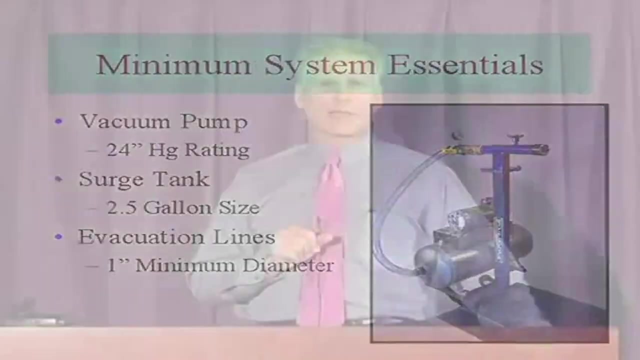 a piece of vinyl coated clothesline into your, into your plaster itself. so your minimum system essentials: vacuum pump with, I think, at least 24 inches of mercury rating, a surge tank at least two and a half gallons in size and evacuation lines at least one inch minimum. 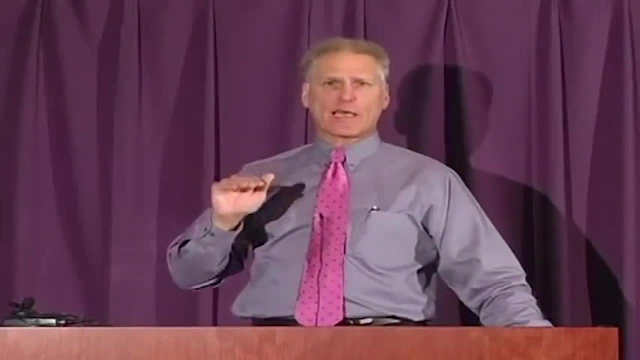 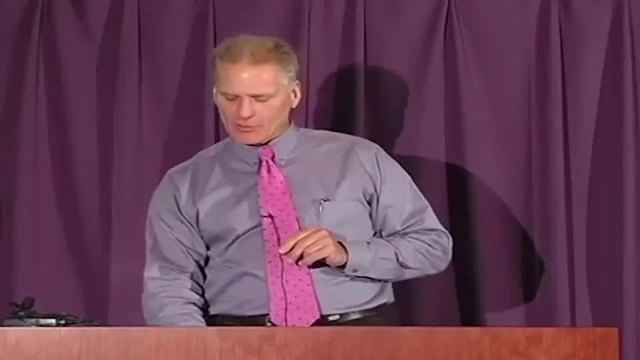 diameter. so that's the minimum system essentials to have a thermal forming system. remember I said a vacuum pump is just the heart of your system. it's not your complete system, so make sure you have all the other, do you two other essential components as well? so keywords in this surge. 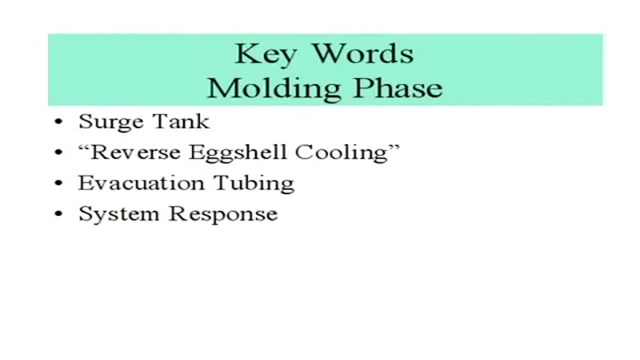 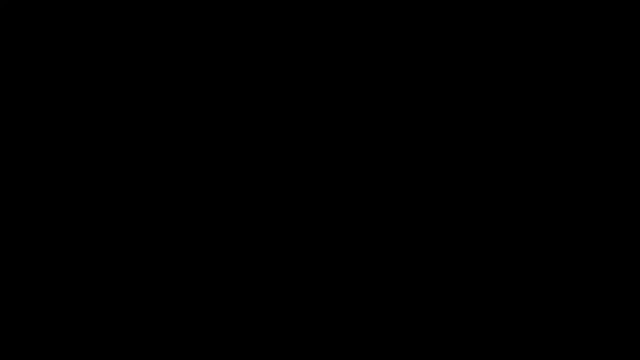 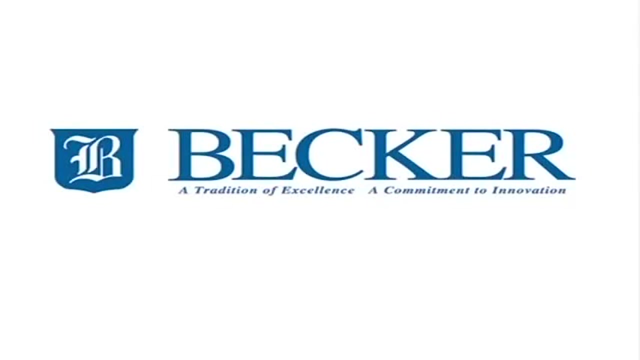 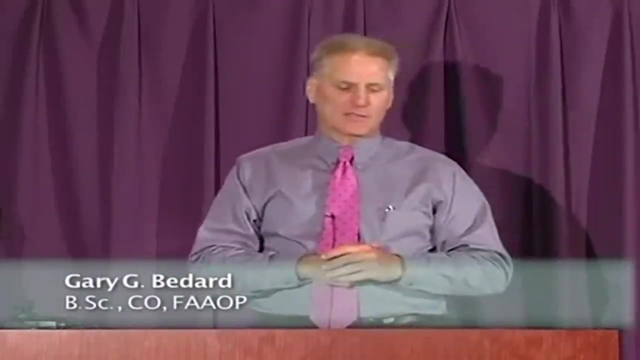 tank, reverse eggshell cooling, evacuation tubing and your system response- all key points that we made in the system. okay, now we'll move into the next video. Thank you to the next segment. Now that we've discussed the molding aspect of our process, we're going to go into what 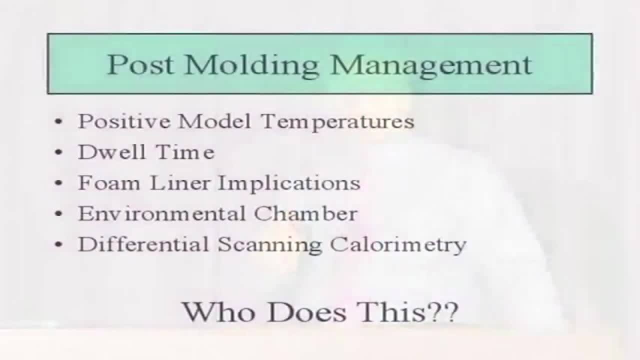 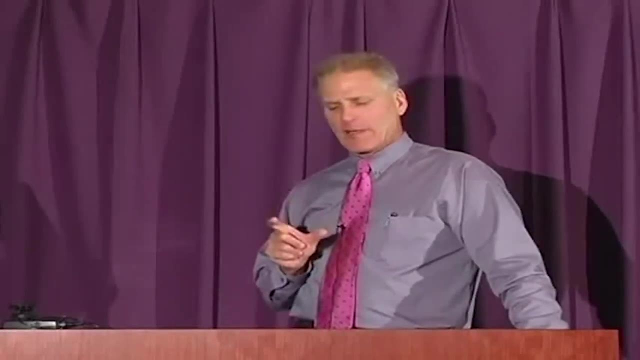 I call a pulse molding management. We'll look at positive model temperatures, dwell time, phone liner applications, environmental chamber and differential scanning climatry. Now, post-molding management, I think, is something that's very germane to what we do and not. 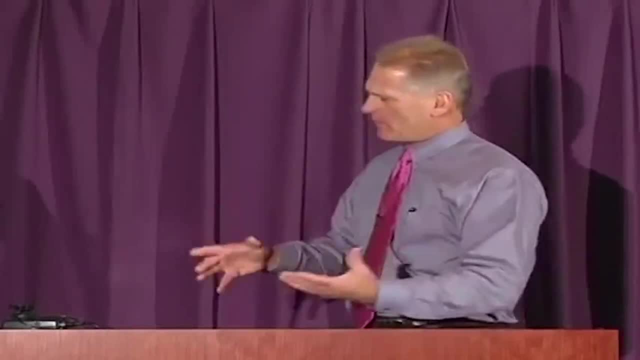 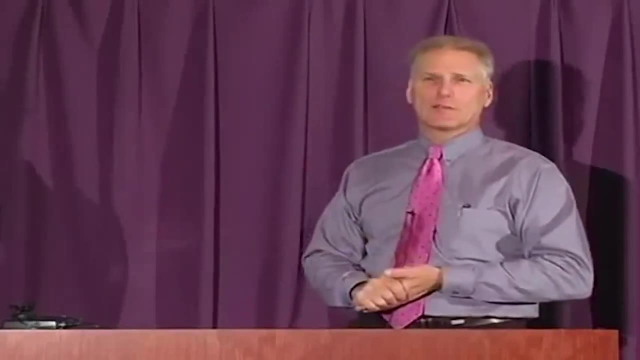 recognized by many people in our field, because typically when people wrap their plastic on a positive model and seal it up and trim it, they're done. They're done. They're just letting it cool and waiting until they can come back and trim it out. 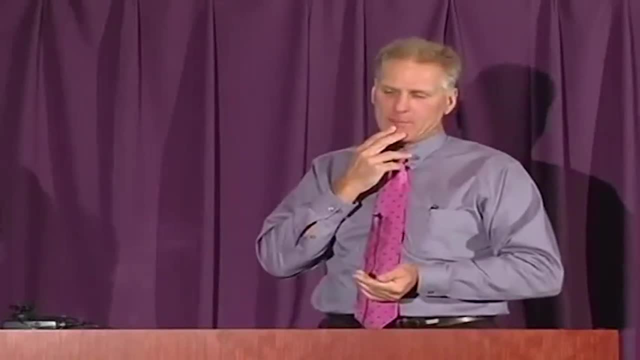 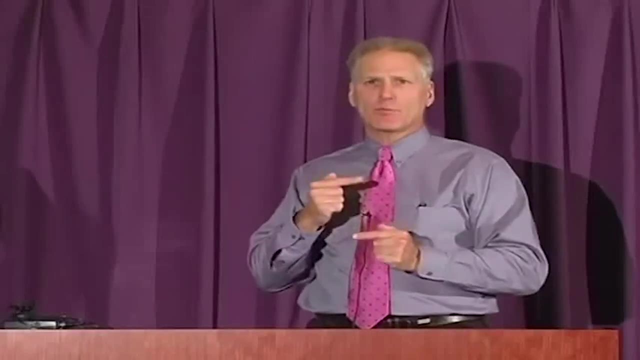 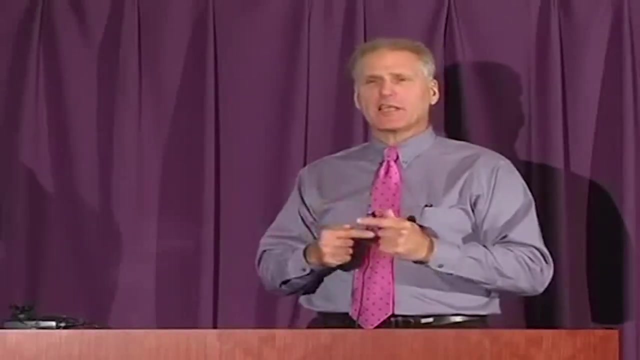 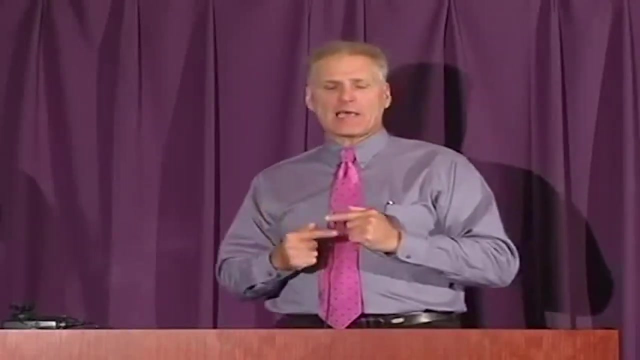 And remove that positive model from their molding manifold. But as we became more acclimated with the principles of industrial thermal foaming using thick gauge sheet and understanding the polymer chemistry, we came to realize that we did actually need to have a post-molding management segment. 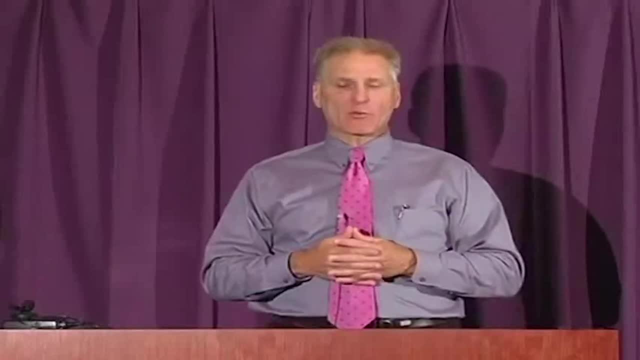 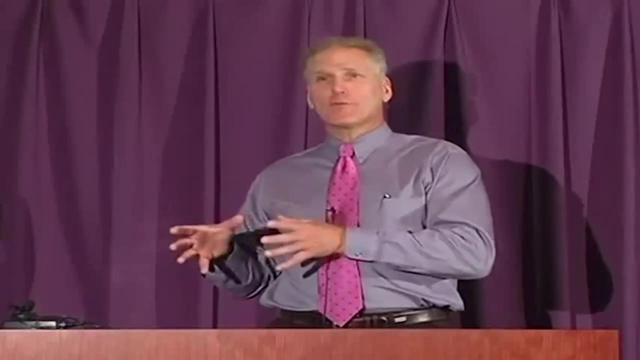 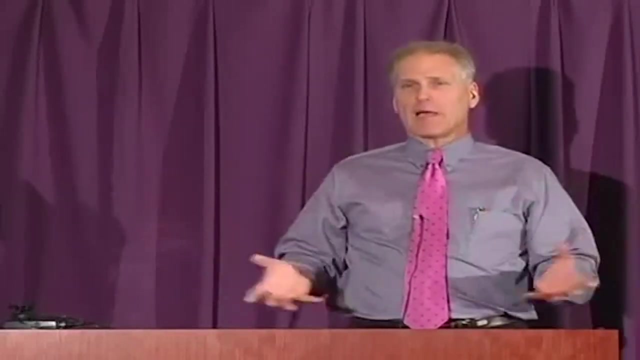 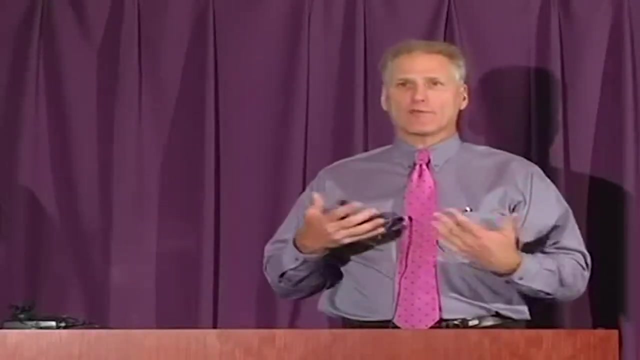 Post-molding, Post-molding, Post-molding, Post-molding management process, because it did directly influence the strength of our materials By the time we get through this segment. we're going to tie a lot of elements together and really make our look at industrial thermal foaming fairly sophisticated. 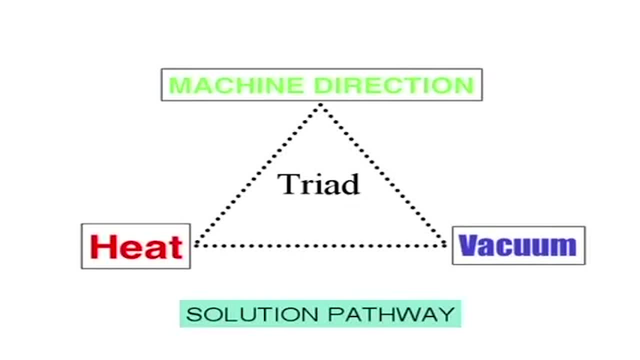 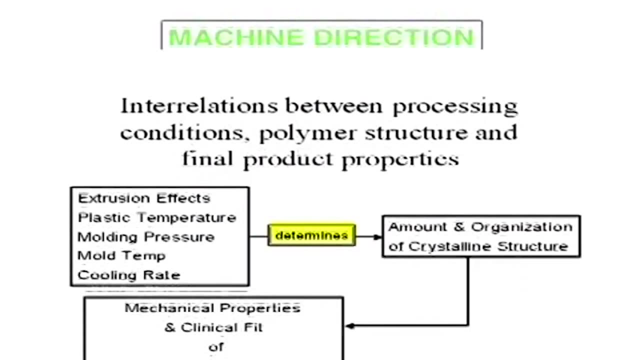 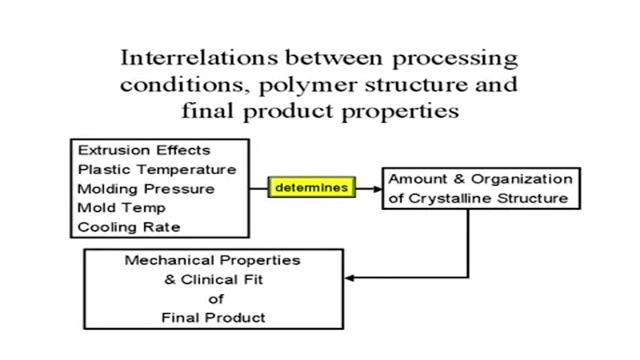 Again: Machine direction, heat and molding, And how we found our solution pathways to have a very disciplined process. This is our sophisticated look. The interrelations between processing conditions, polymer structure and final product properties are all geared to understanding the extrusion effects. plastic temperature, molding pressure, mold temperature. 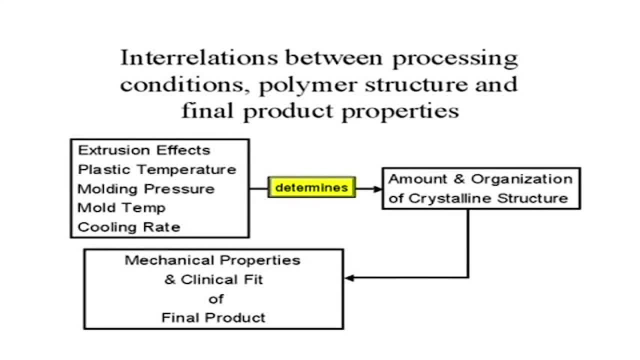 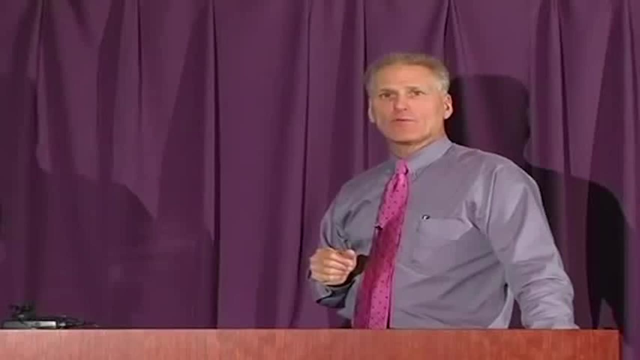 cooling rate, which determine the amount and organization of the crystalline structure of our thermoplastic material when it is made into a final product, which then determines the mechanical properties and clinical fit of that clinical device. So very sophisticated. look. We're pulling in all the information that we've reviewed within these multiple 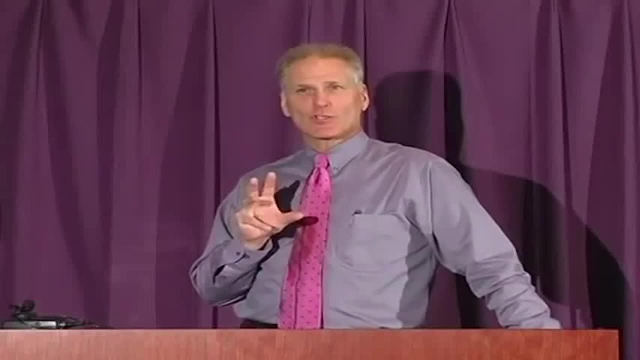 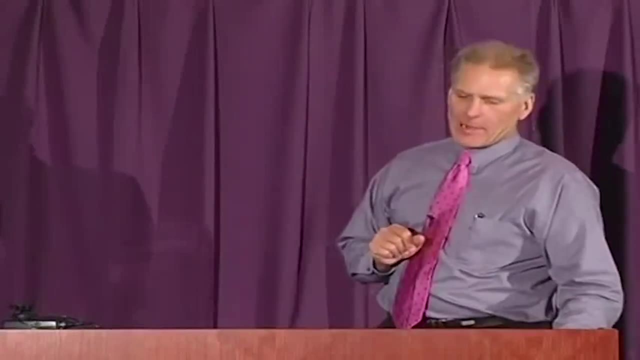 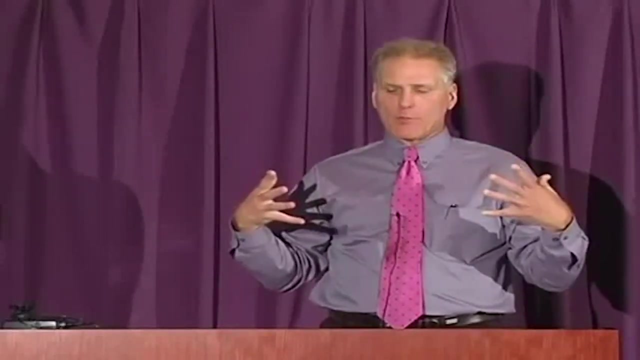 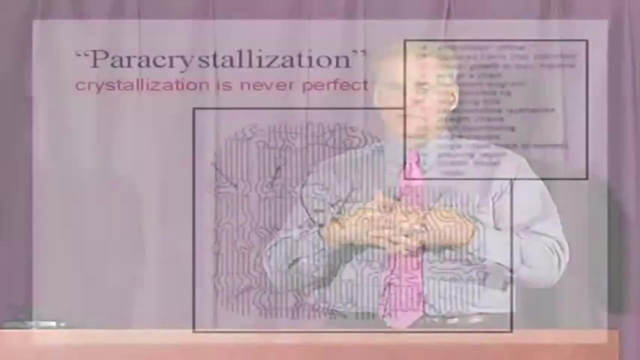 segments, to have this little bit more sophisticated approach to what we do. Paracrystallization is the term they give to the thermoplastic polymer chains when they reform into that amorphous and semicrystalline structure. It's not a benign event, It's a dynamic. 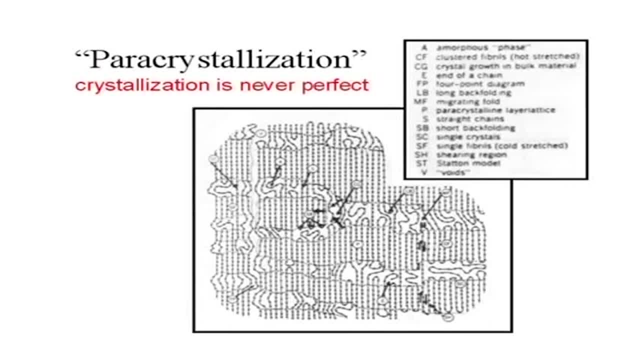 event, And there are many things that can interfere with the formation of that optimal bias or that optimal ratio of amorphous and semi-crystalline structure. The first thing that we're going to look at is the amorphous and crystalline area within. 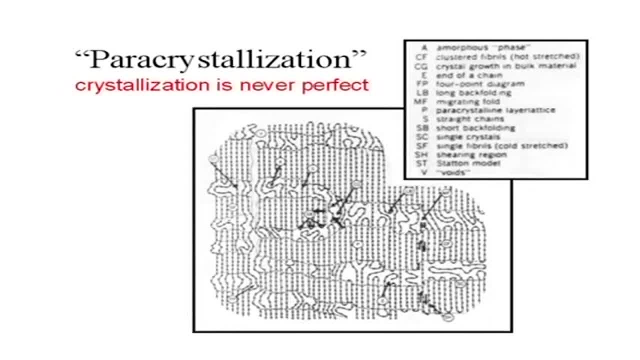 polyethylene and polypropylene- Here with the list that's given on your screen. amorphous phase clustered fibrils. four-point diagram: straight chain short back folding single crystals. these chains basically can take many different configurations, some good and 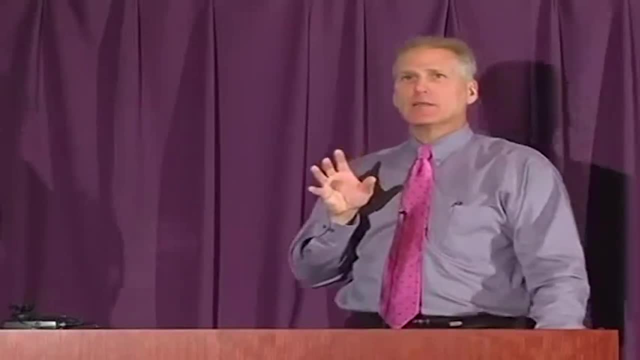 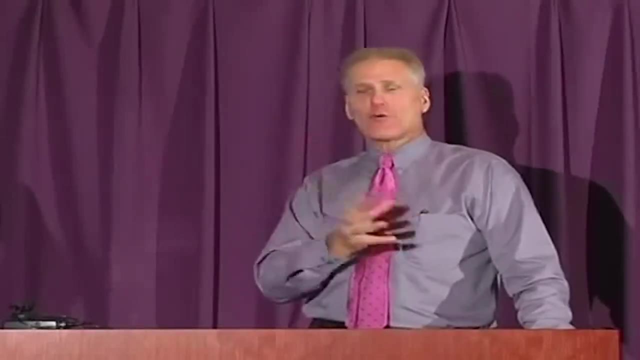 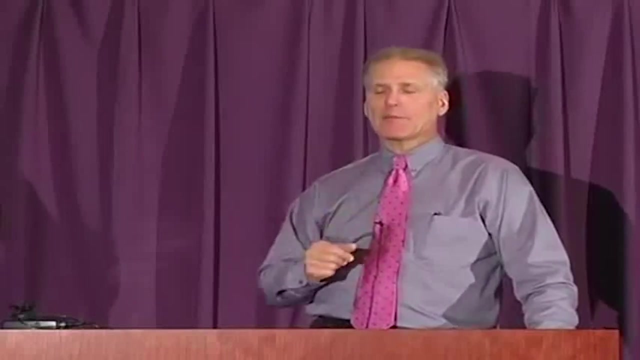 some bad. Some of you have probably taken a cast saw, put it onto cooled plastic around a vacuum foam. positive model: put that cast saw, made a notch in your plastic, had it crack all the way down. If you haven't, it'll probably happen to you at some point in time. 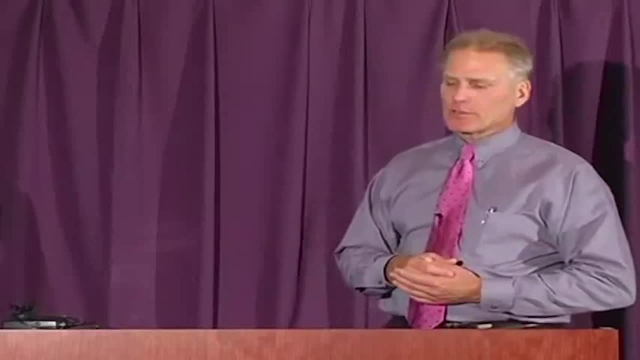 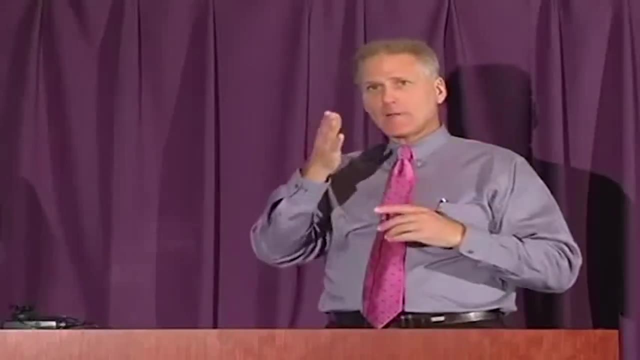 It's a very common occurrence. What has happened at that point in time is the plastic has become very notch-sensitive. The stresses within that structure are so high that as soon as you make a defect in that structure, it's a point of failure and it propagates in a 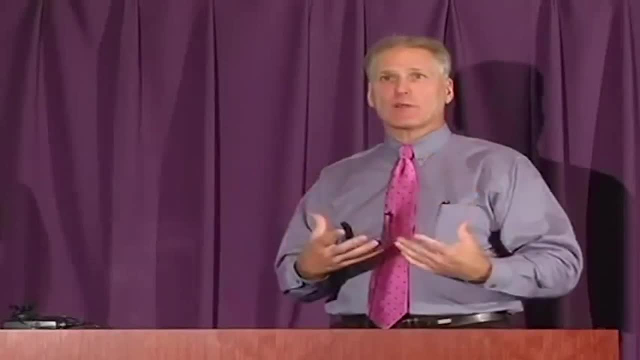 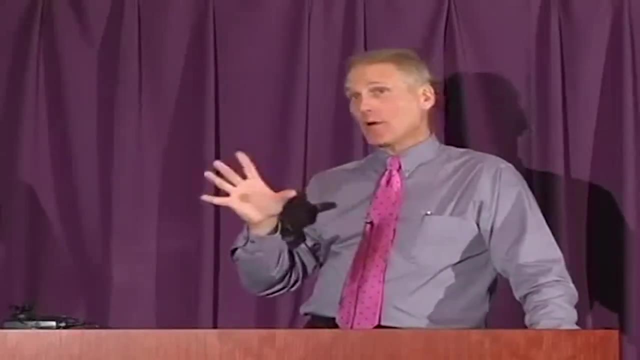 long crack. It's just a release of the forces. They've been trapped within that molecular structure. It happens quite often. It's because of this para-crystallization. It's not a benign event. We want to make it as a benign event. 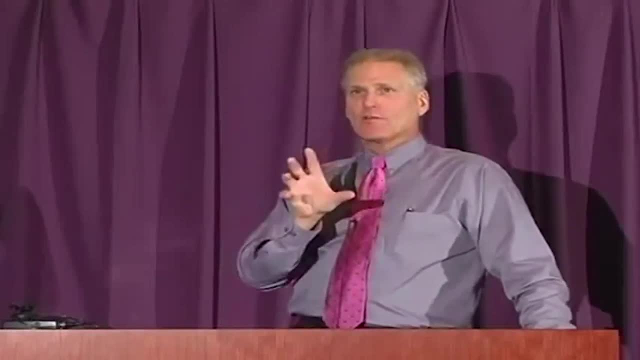 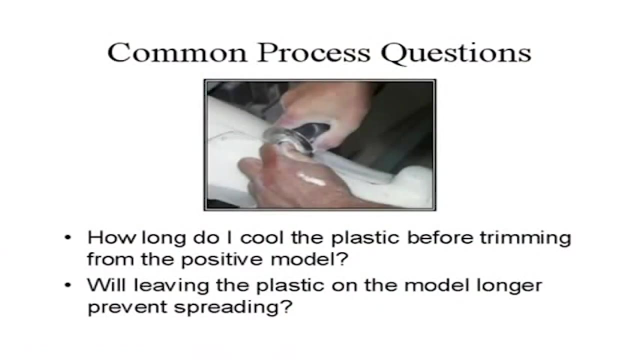 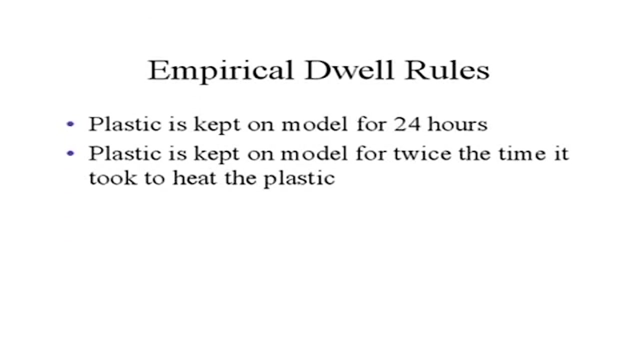 We want to make it so that semi-crystalline structure forms into its lowest energy state. Common process questions. How long do I cool the plastic before trimming from a positive model? Leaving the plastic on the model longer prevents spreading. We can look at our empirical 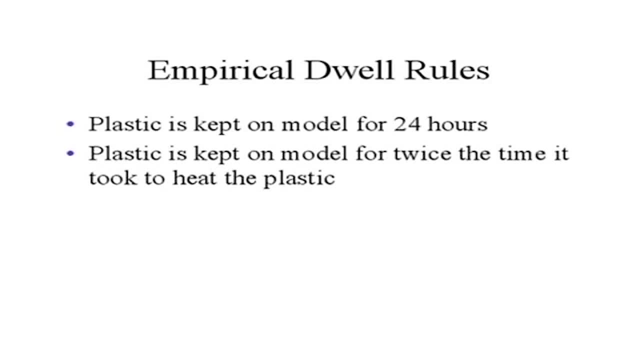 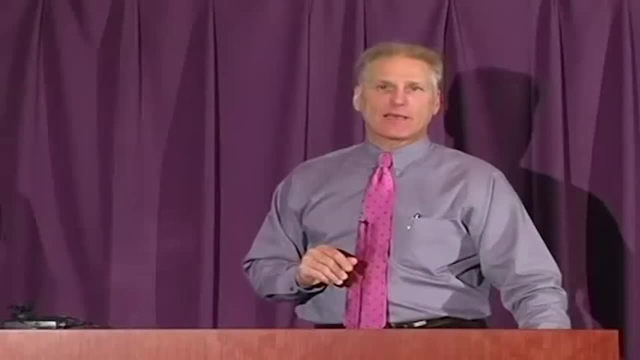 dwell lose. Plastic is kept on the model for a long period of time. The plastic is kept on the model for 24 hours. Plastic is kept on the model for twice the time it took the heat to plastic. These are very old rules not based on anything that is scientific- for the most part, Most. 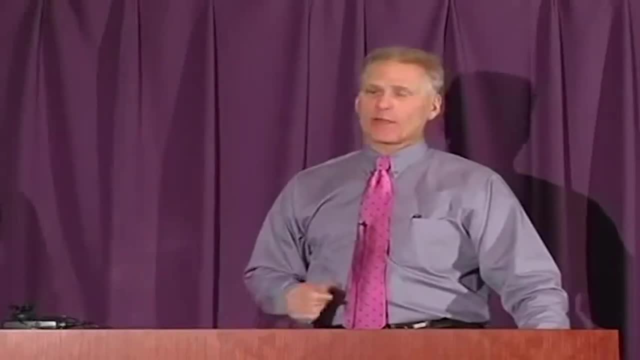 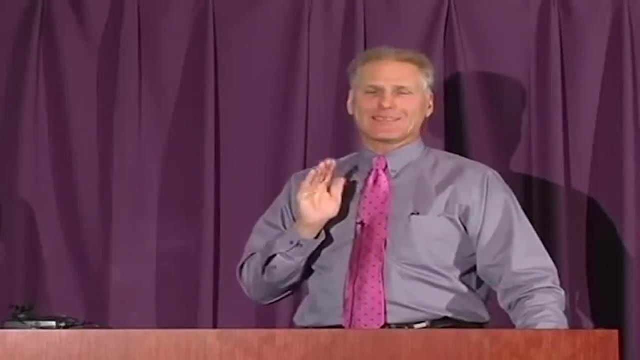 people believe if you leave it on for 24 hours it's not going to spread. That's not true. As soon as our materials hit their set temperature, they're frozen. They're not going to move. It's not a time-dependent equation. It's all based on managing that molecular structure. 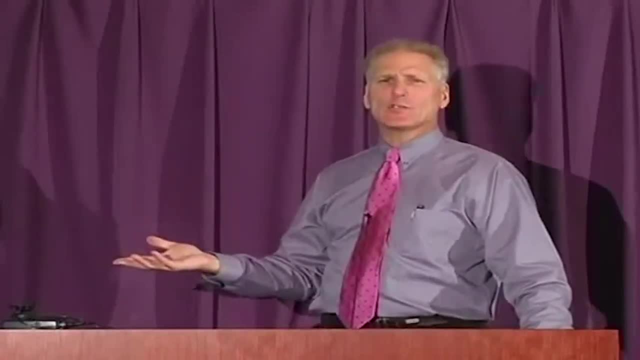 Plastic is kept on the model for twice the time it took the heat to move. It's not a time-dependent equation. It's all based on managing that molecular structure. Plastic is kept on the model for twice the time it took the heat to move. It's not a time- Berkeley. 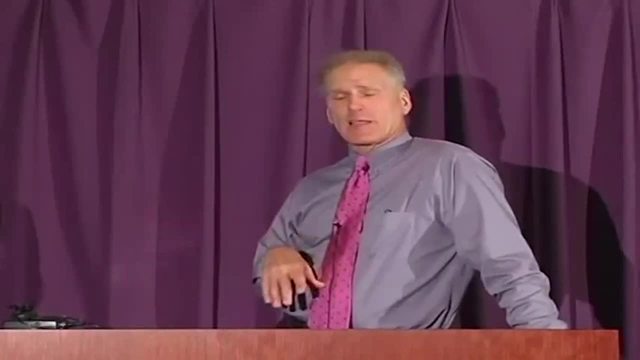 Well, in the old days you're using a convection oven and it took you 20 minutes to heat your plastic. That meant you left it on vacuum for 40 minutes. but all of a sudden I bought an infrared oven. Not only takes me 11 minutes, that means I could cut my plastic out in 22. 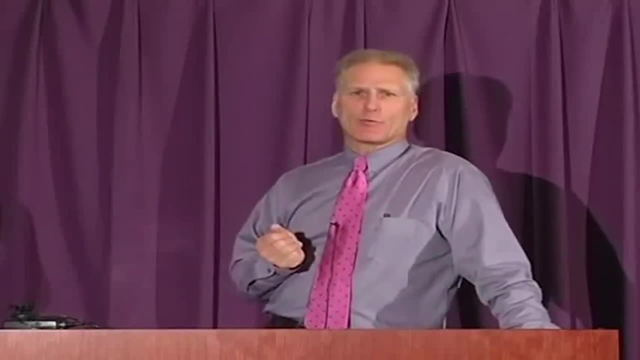 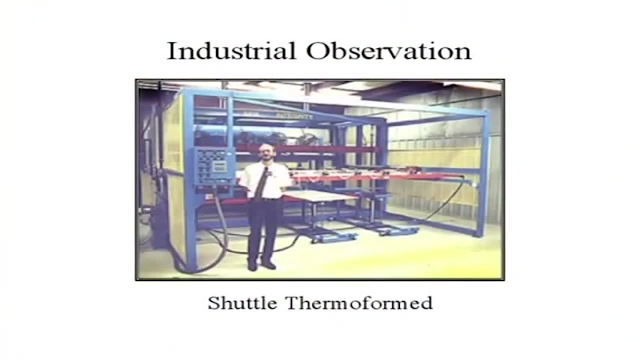 minutes. It had no correlation toyorsunic chemistry, It was all empirical rules and kind of those husband and wives' tales kind of thing. This first became apparent to me when I took one of my industrial courses. I was walking through a big lab. 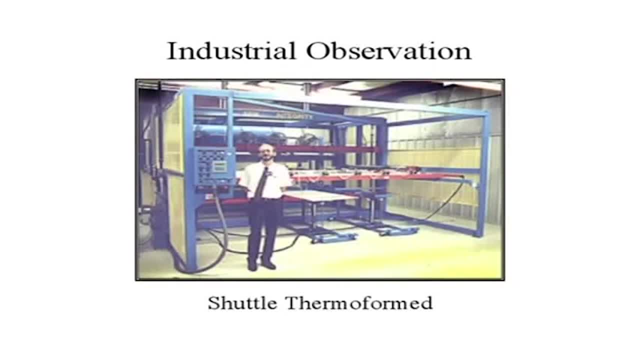 big industrial plant, thermal forming plant, outside of Milwaukee And they had these big shuttle formers like you see in this picture here. It would take a huge piece of plastic, I think 4 by 10 feet in that range, And the plastic was being formed into front end of NASCAR race cars. 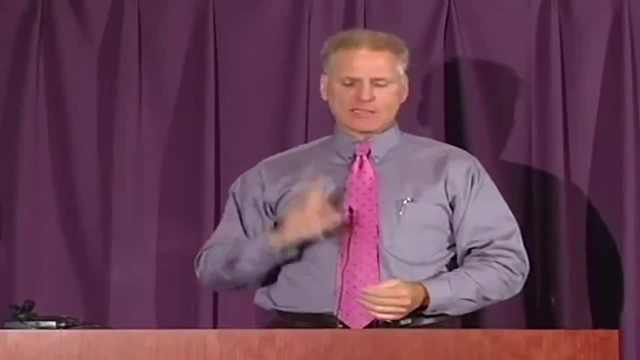 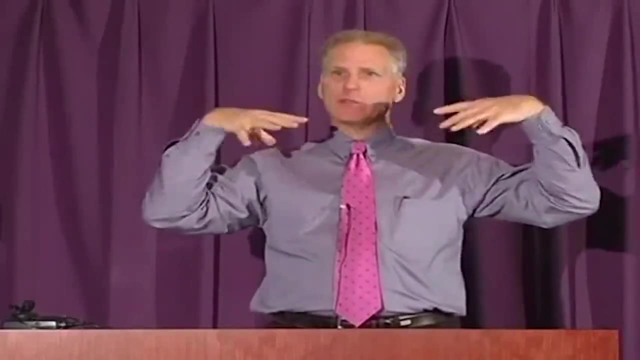 So a big industrial plant, right, big, big machine. And as I was walking through the plant very slowly, I noticed that the operators would load a piece of plastic, they would go in and heat form and within 10 minutes, 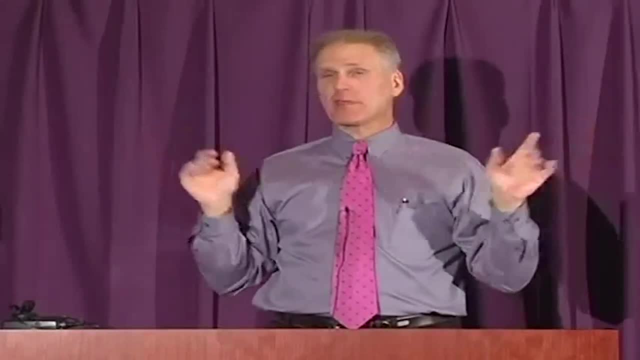 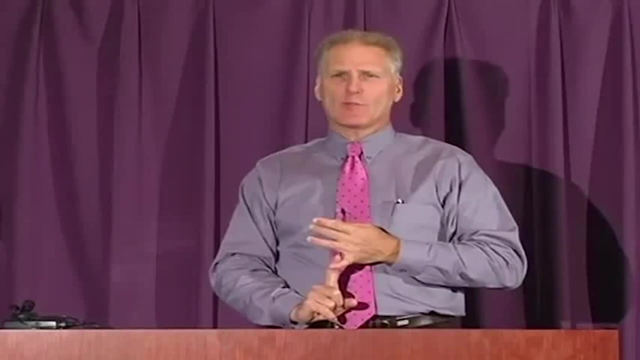 they were popping the plastic out of those molds And I'm thinking to myself: that's not as fast, We're not that fast. in our lab We were leaving our plastic on vacuum until it became room temperature, And then from there it went into a water bath for four hours. 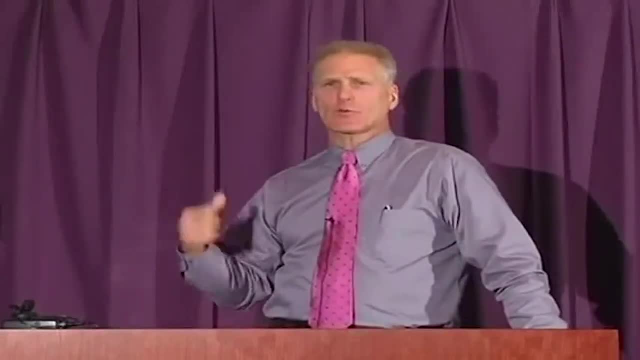 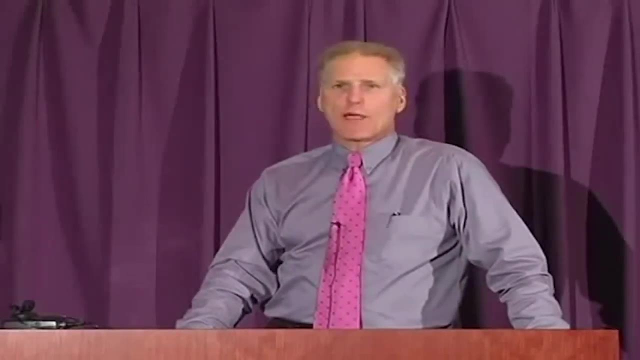 So basically four and a half hours before we would do a trim up, These folks were doing it in 15 minutes. So by being a student in one of those industrial courses opened my eyes to the vast difference between the industrial side and our side. 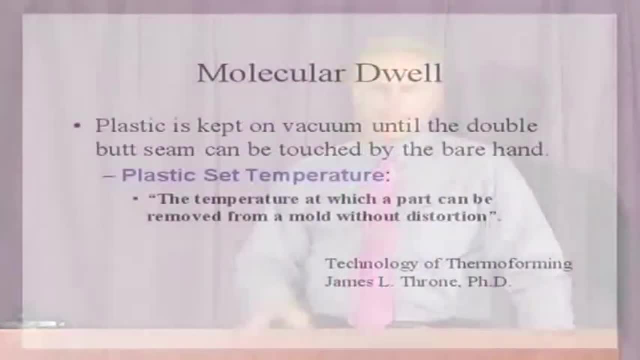 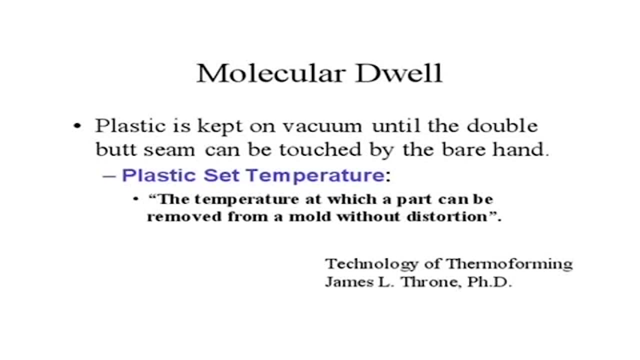 They were doing it basically. They were doing it basically in about 10 or 15 minutes. So they were following what's called a molecular dwell rule And this is based on the plastic temperature which, coming right out of Dr Throne's book, 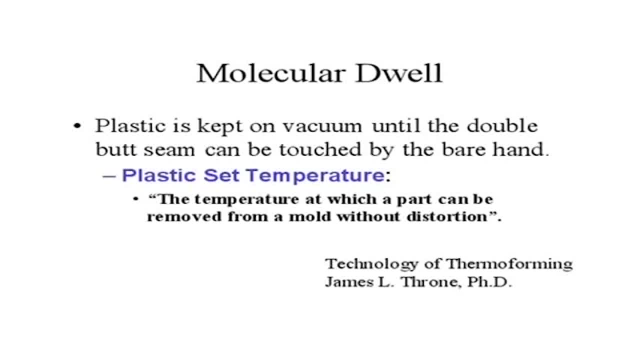 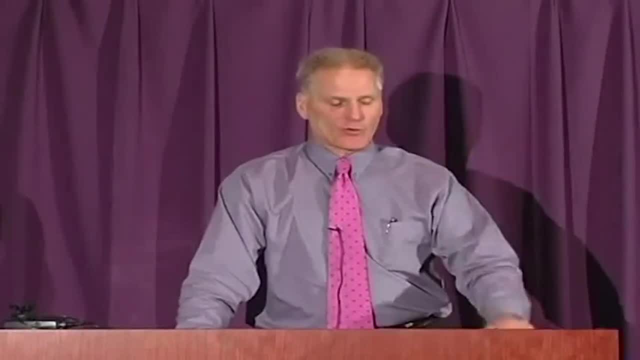 is the temperature at which a part can be removed from a mold without distortion. For polypropylene it's 190 degrees. Now we could cut off our plastic. 190 degrees- It's a little bit hard to handle with your hands. So our rule of thumb in our lab is we keep the plastic on the positive model under vacuum. 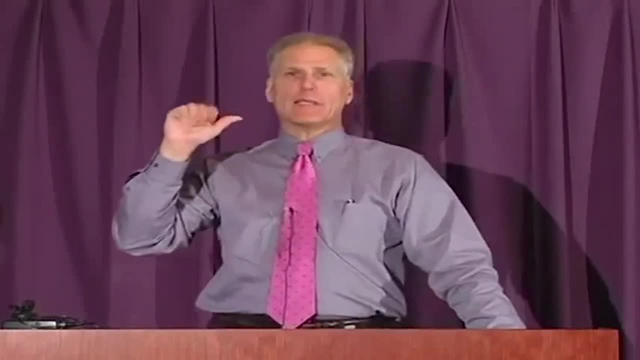 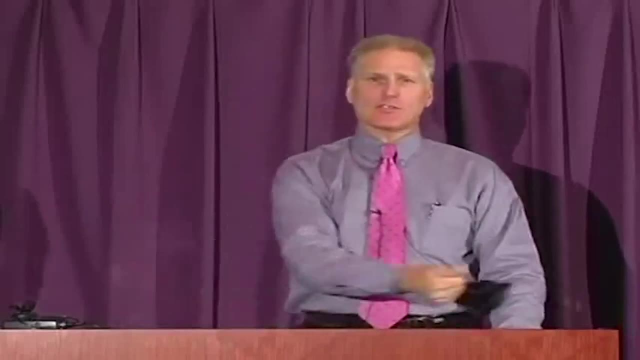 until the double butt seam can be touched with the bare hand, Because the bare hand can stand, heat up to about 125 degrees Fahrenheit and then becomes noxious, becomes painful. So it's very easy for my technicians to walk by, put their hand on the double butt seam. 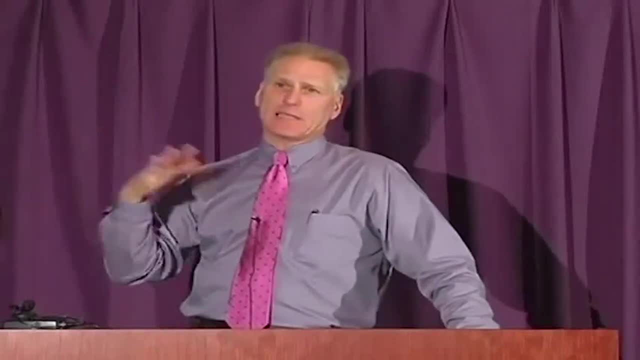 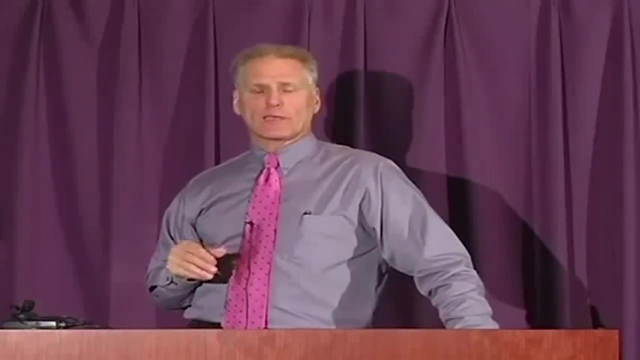 If it's too hot, take their hand off. it's not ready to cut off. If they can keep their hand on it, then they can cut it off, because 125 is obviously way below that 170 degree range for the set temperature of polypropylene. So it all comes down to where that temperature cools to, and understanding that polypropylene set temperature- it's temperature that it freezes at is 190 degrees Fahrenheit, Much quicker than the rules we followed in the past. Polyethylene: 180 degrees. polypropylene: 190 degrees. 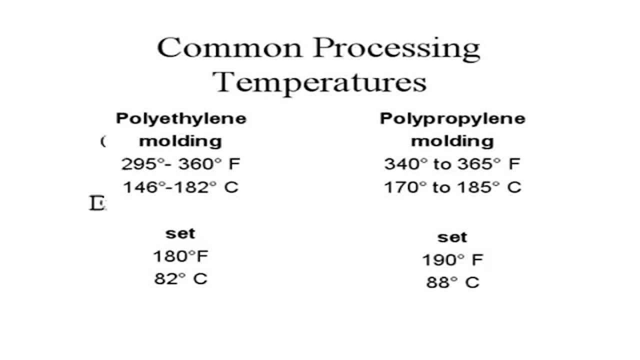 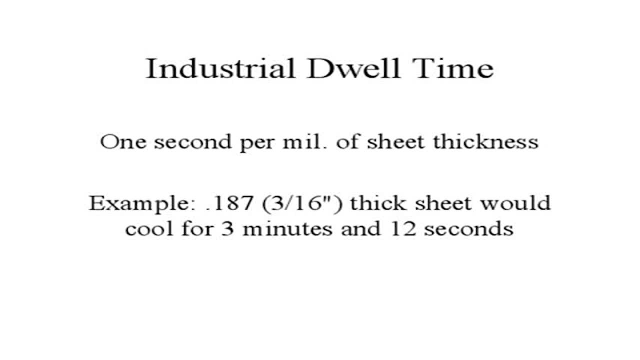 Once it hits that temperature, it's frozen. it's not going to change. Industrial dwell time: one second per mil of sheet thickness. If you had a piece of 3 16ths inch material that would cool in 3 minutes and 12 seconds. 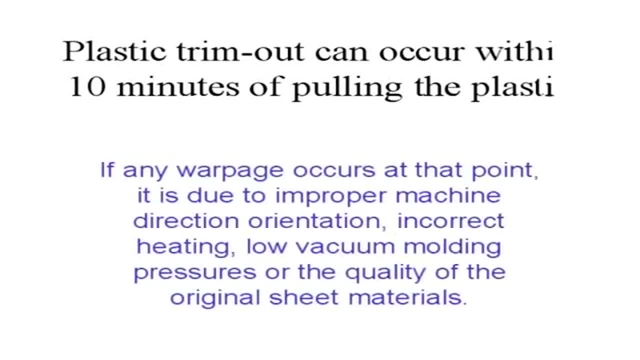 So there are some industrial rules as well. Plastic trim out can occur within 10 minutes of pulling the plastic. If any warpage occurs at that point, it's due to improper machine direction, orientation, incorrect heating, low vacuum molding pressure, all the quality of the original sheet materials. 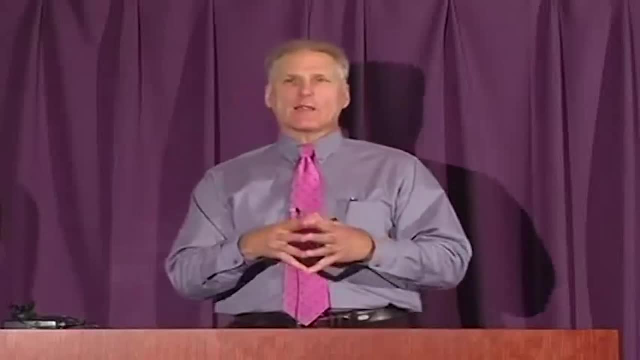 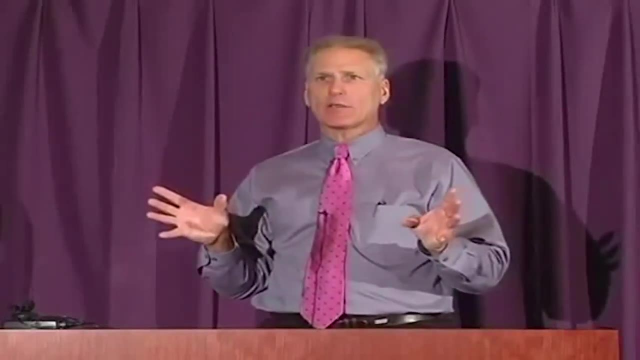 So it's not a single event or a single element that creates that warping or that shrinkage or that orientation. It's the multiple factors that we talked about here today. It's controlling that whole process, controlling that whole triad, controlling your machine direction. 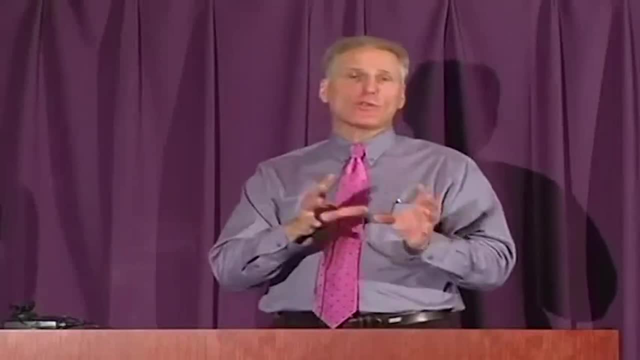 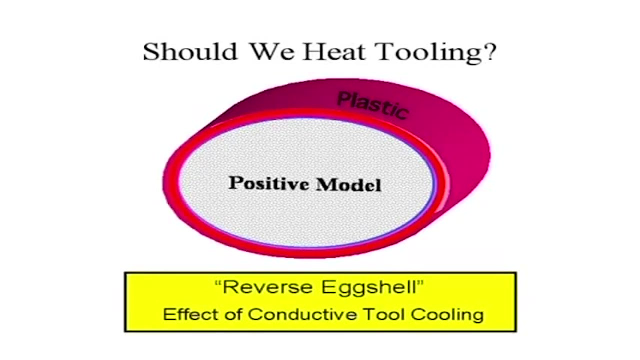 Not just how long you leave it on the positive model. It's all the elements and you have to balance all of them. Should we heat our tooling? We've talked about this several times- that reverse egg shell. A common fabrication technique in our field is to use a foam liner. 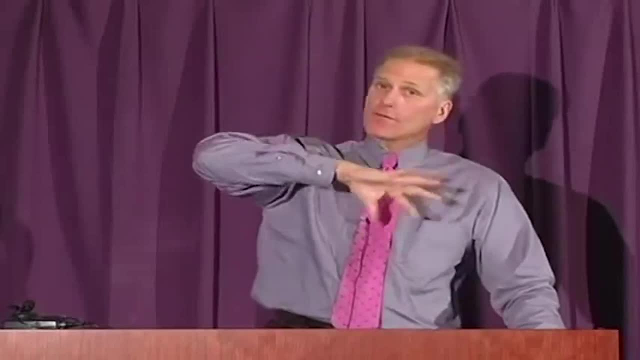 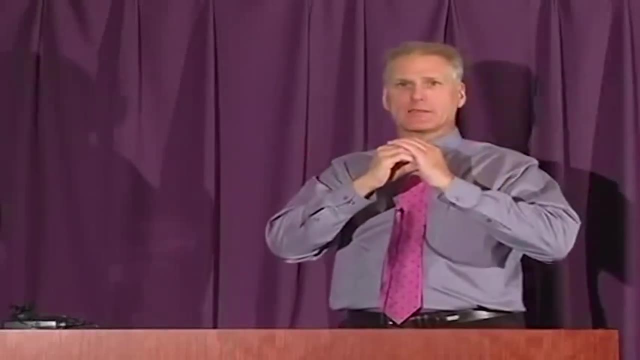 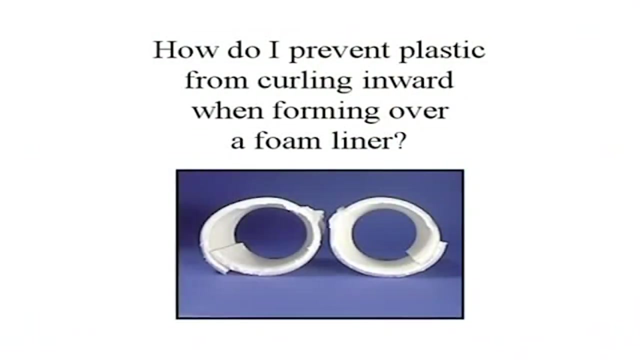 And that necessitates us vacuum foaming over the foam, that's, over the positive model. What we've always seen is a curl into the plastic, Very hard to eradicate. So what can we do to eliminate that? This is a very practical type application of using the chemistry of thermoplastics. 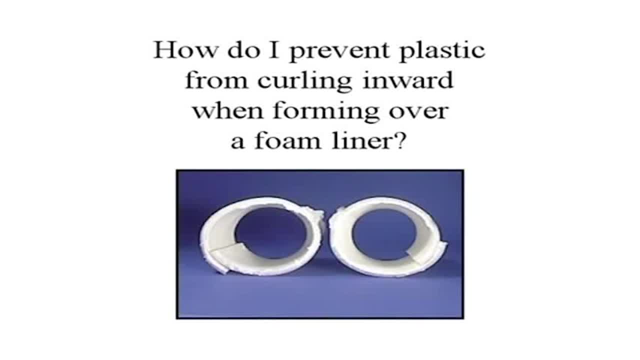 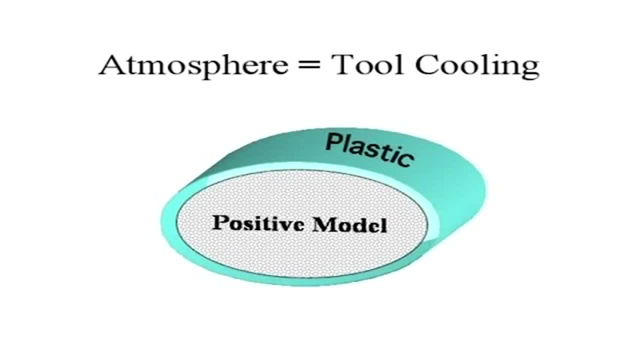 to take care of a problem that's been common for many years. The problem is an unbalanced cooling effect on the molecular structure. When we put our hot plastic on a positive model and let it cool, we more or less believe that it cools at the same rate on the inside and the outside. 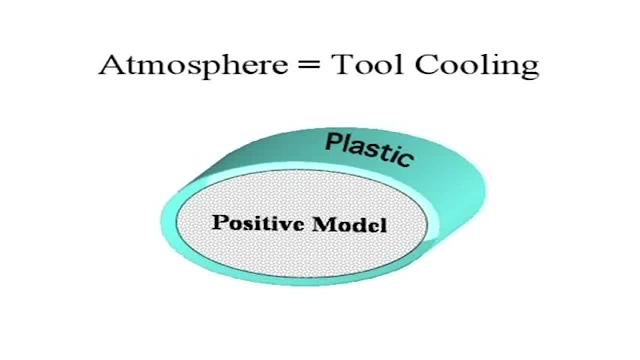 It really doesn't, because once convective cooling, which is the outside, which is much slower, on the inside it's conductive cooling because the plastic is in direct contact with the positive model. That's much quicker. But we kind of bastardize the system and say it's even and it works okay. 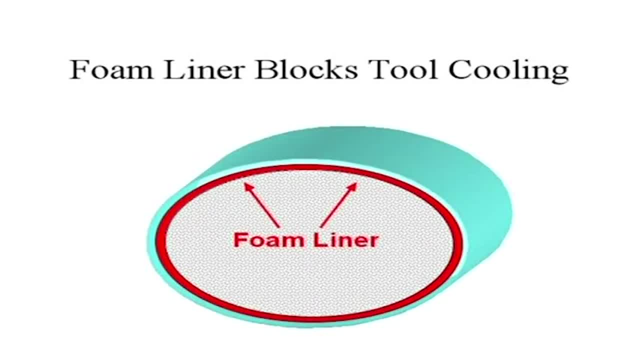 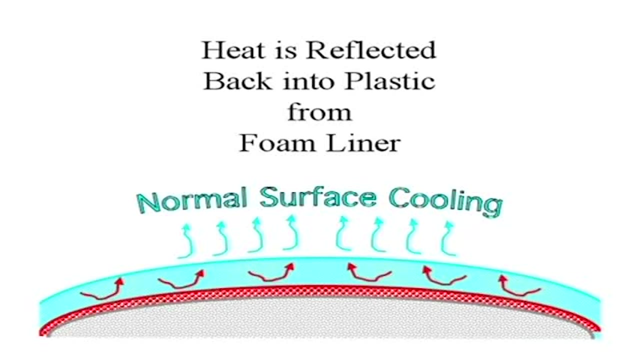 But when we put a foam liner on top of the positive model, the foam liner acts as an insulator, So that plastic on the inside doesn't have quick cooling. Now the only way it cools is through the surface. That foam liner blocks the cooling of the inner plastic. 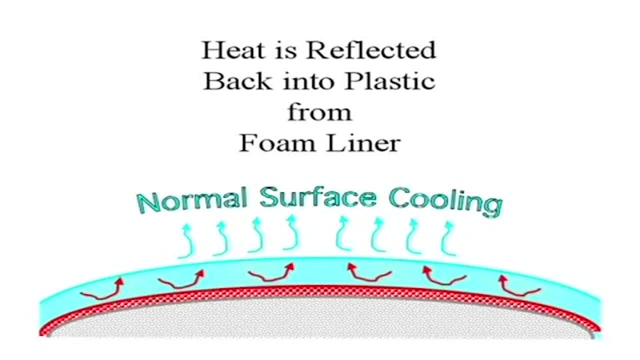 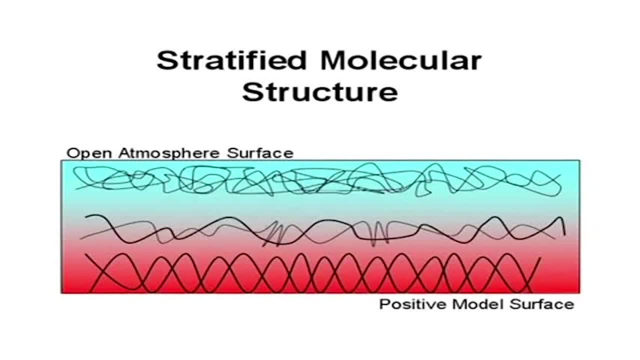 So the only way that heat can dissipate is through the surface. So, consequently, what happens is that she cools is the inner surface against the foam liner. has a longer period of time in order to cool. has a longer period of time to form into a crystalline structure. 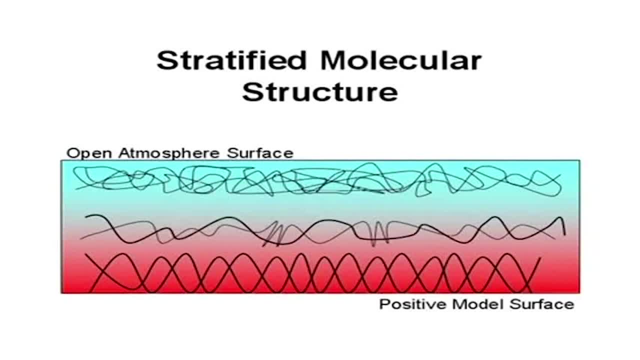 The plastic on the outside cools quicker because it's the only way heat can dissipate it from that piece of plastic And the upper surface. this is made a little bit more amorphous in structure, So the crystalline component on the bottom shrinks a little bit more. 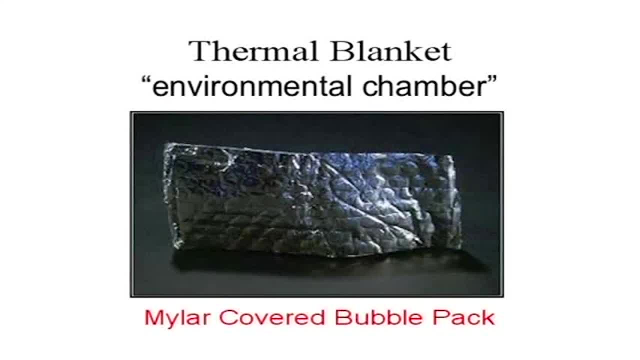 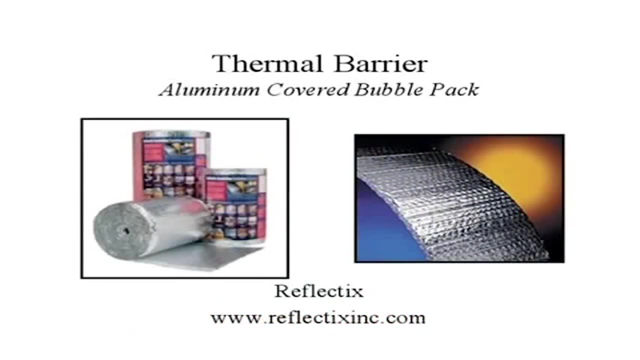 has a higher tensile value and just makes that plastic curl in like a potato chip. What we do? we cover the entire thermoform piece with a piece of insulation. This is insulation that's used in the air conditioning and heating industry. It's a double layer of bubble pack covered by an aluminum film. 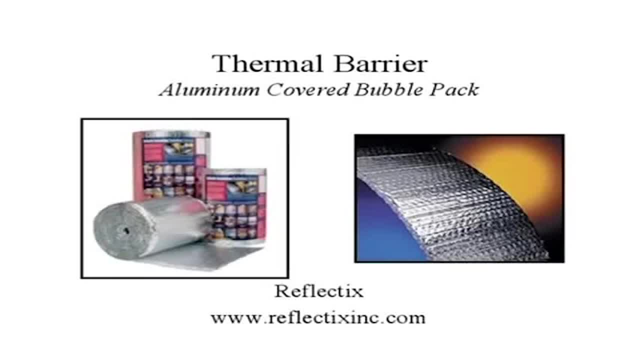 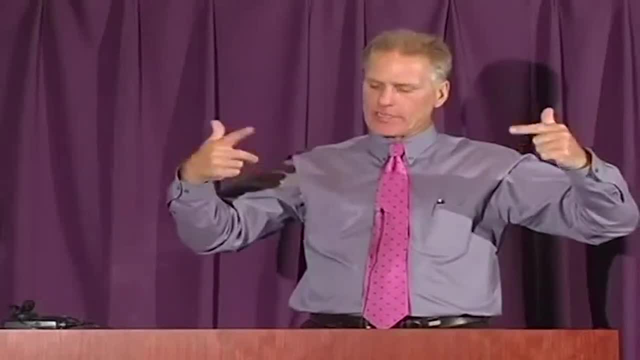 Very inexpensive. Most hardware stores cover it. It's called Reflectex is the name of the company and that's their website. We either take a big sheet and just wrap it and seal it like a tootsie roll with using ace wraps above the top and the bottom for a big TLSO. 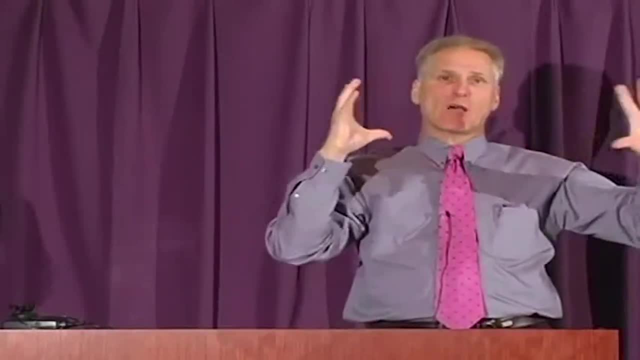 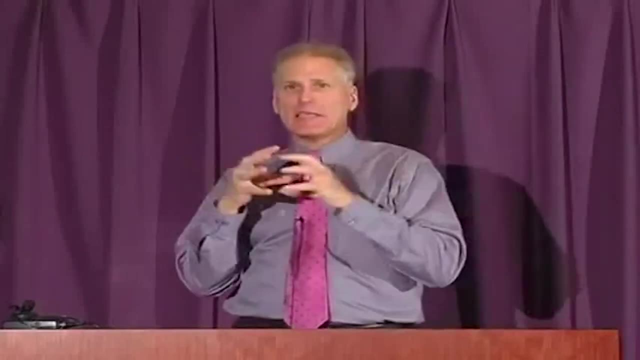 For an AFO. you can actually sew this material and make a big sock like a Christmas sock and just bring it up over your AFOs or KAFOs and seal it, And that will retain the heat. This is the environmental chamber, as I call it. 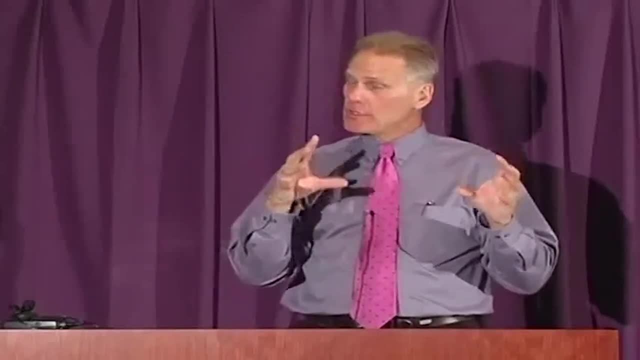 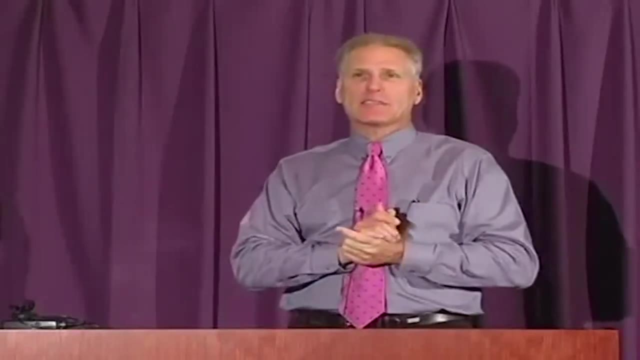 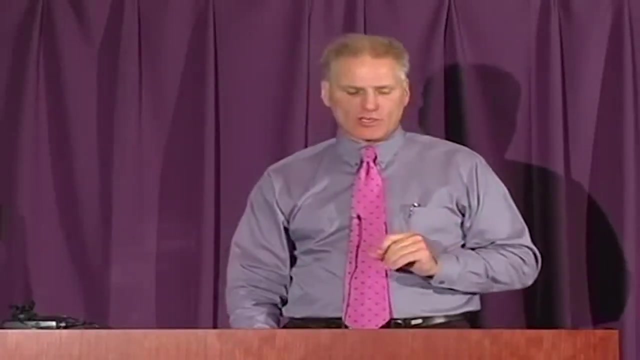 This retains the heat on the plastic, slows the heating, slows the heating down. Then you say: well, you know, I don't want to slow down my process. It adds maybe about 10 minutes to the time, but if it changes the dimension or it makes you manage the dimensions of your sheet, 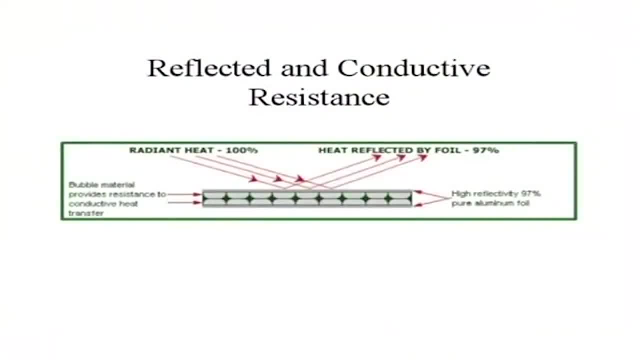 it works much better. And that double bubble pack basically has the ability to both be conductive and reflective in its insulating quality, So it's actually a pretty good material for this kind of side type of application other than insulation in the heating industry. 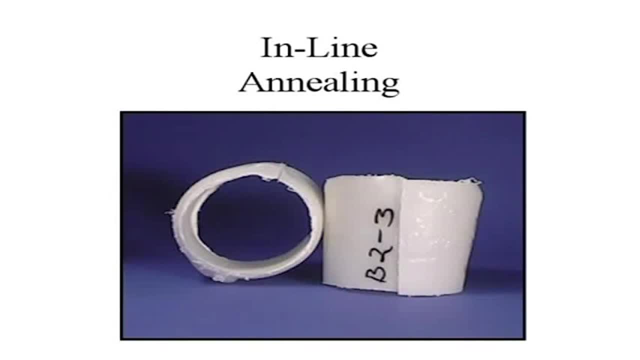 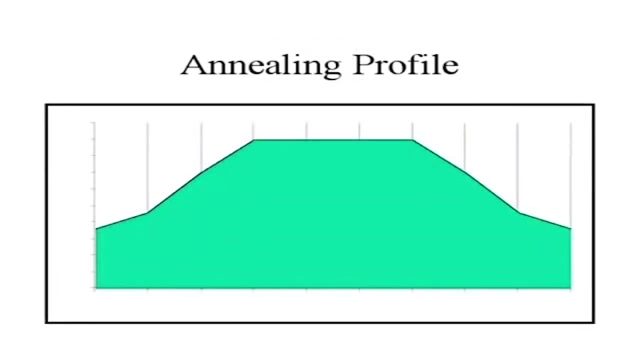 So when we do this type of wrapping, in essence what we're doing is in-line annealing. Now, normal annealing is where you take a product that's at room temperature, bring it up to just below its set temperature to let the stresses within the molecular structure dissipate. 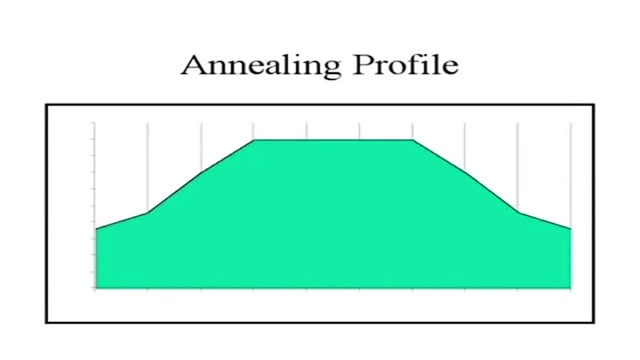 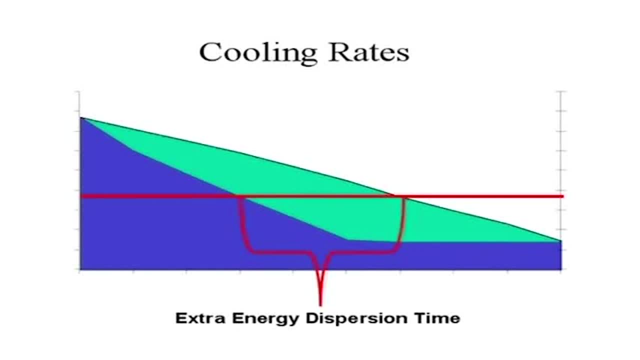 and then ramp it back down to room temperature. Well, in our process we're doing it in an in-line fashion. What we're doing is in this first line, the dark blue, with the steep slope, we're going from the melt temperature polypropylene rapidly cooling down to that set temperature. 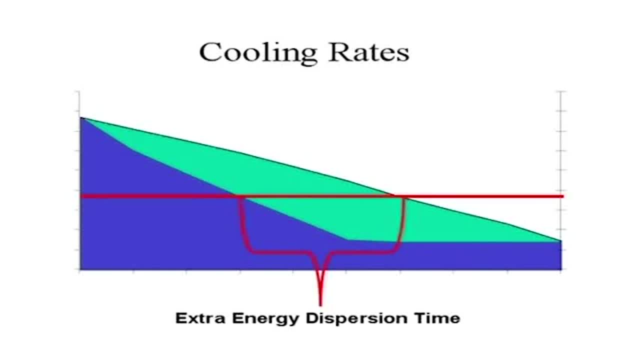 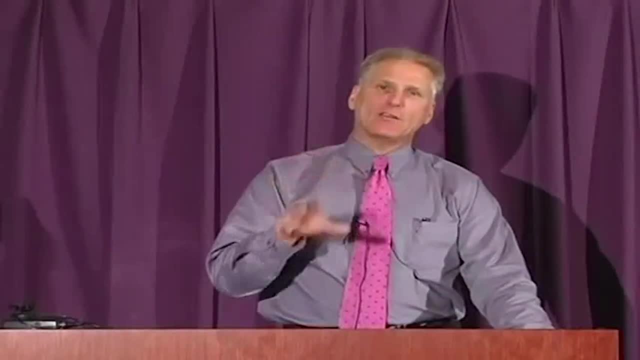 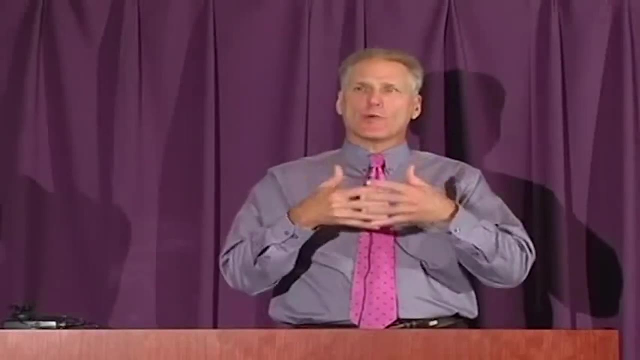 By slowing it down we basically decrease the slope and we gain all this extra time right here in order to have that energy disperse within the molecular structure and for those polymer chains to come into the optimal ratio of crystalline and amorphous segments. 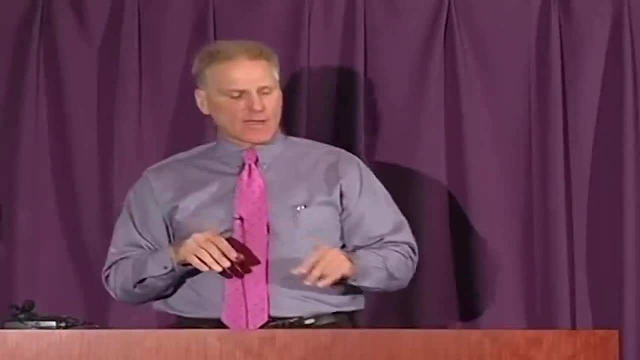 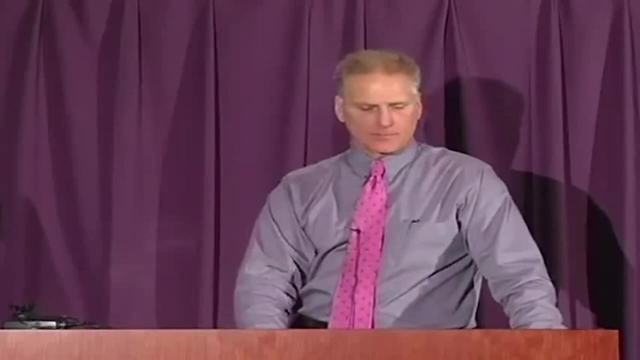 So we're at its lowest energy state, which we've talked about several times today. So, in essence, this is in-line annealing rather than doing it as a separate process. This fits right into the specifications of the plastic, primarily because one of the interesting things about thermoplastics 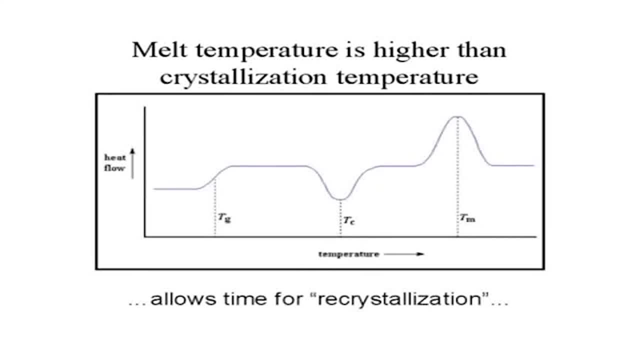 is that the melt temperature we can see here represented on this temperature graph, is much lower than the temperature of crystalline. So it takes more energy to separate or lower the Van der Waals forces so the individual polymer chains can move independently And then for them to come back into that semi-crystalline. 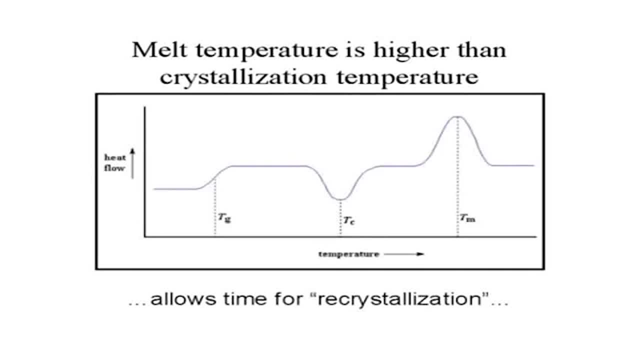 and become rigid again. that temperature is much lower temperature crystallization: Usually it can be as high as 100 degrees centigrade difference in terms of melt temperature to temperature crystallization. So it's within that spectrum that we let the plastic cool just enough. 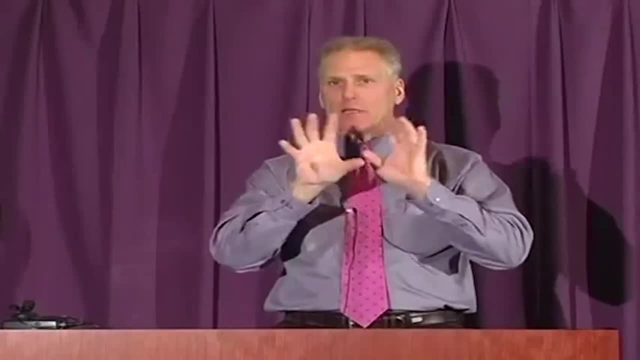 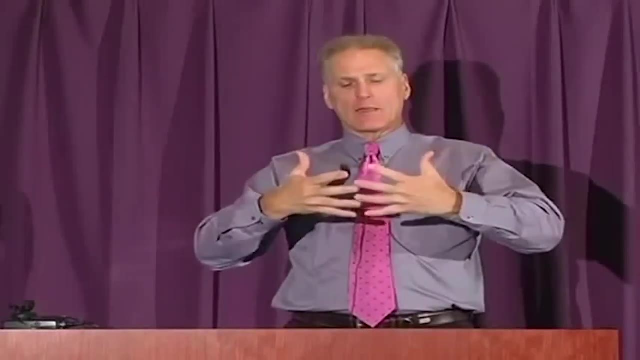 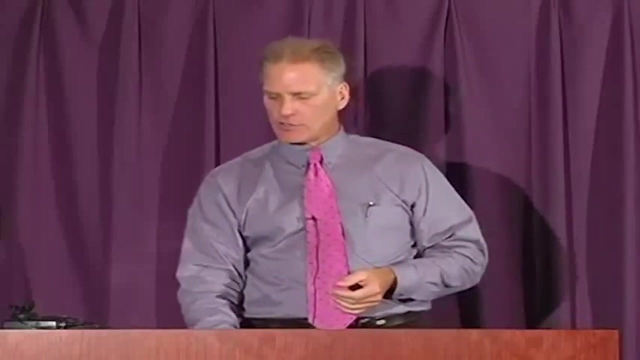 so we can overwrap it without marring the cosmetic surface of the plastic and yet retaining enough heat. so it slows down that recrystallization and allows the recrystallization to have more time in order to come to its lowest energy state. 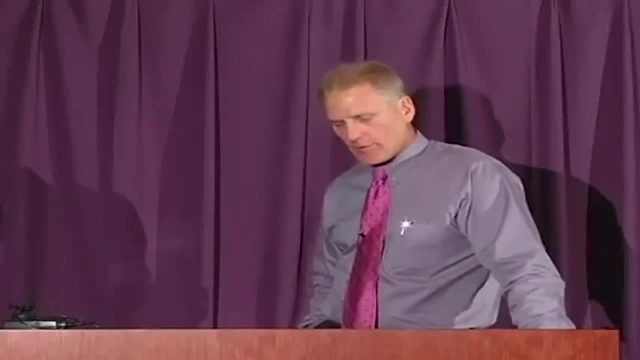 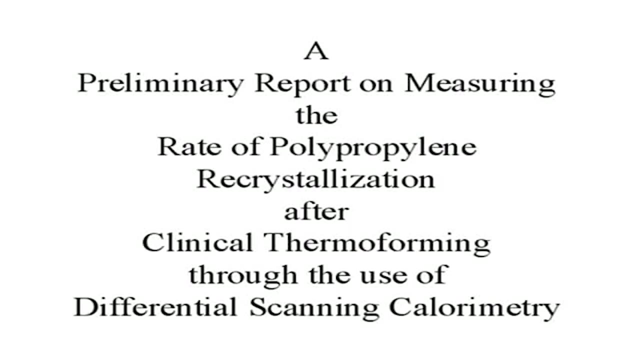 Once we got to this point of understanding of our thermoforming process, I did a paper at our National Academy meeting, which was a preliminary report, on measuring the rate of polypropylene recrystallization after clinical thermoforming through the use of differential scanning collimetry. 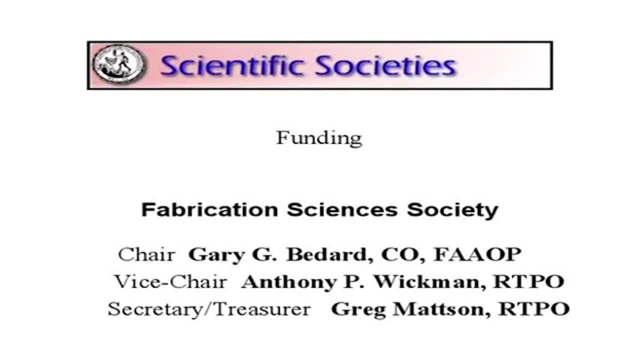 Now, I did this from a grant from the Fabrication Sciences Society, because I was the founding chairman of the society and used the money from the Academy in order to conduct this test, And my founding chair was Anthony Wickman, and then my secretary of treasurer was 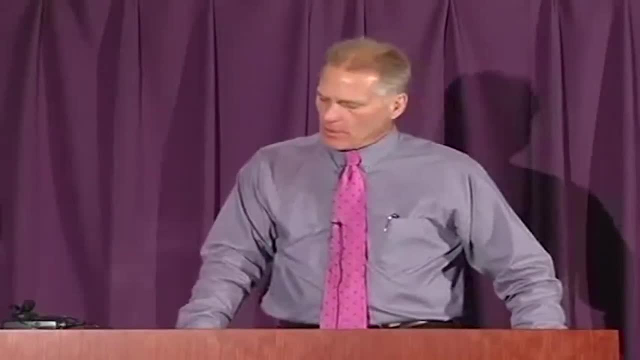 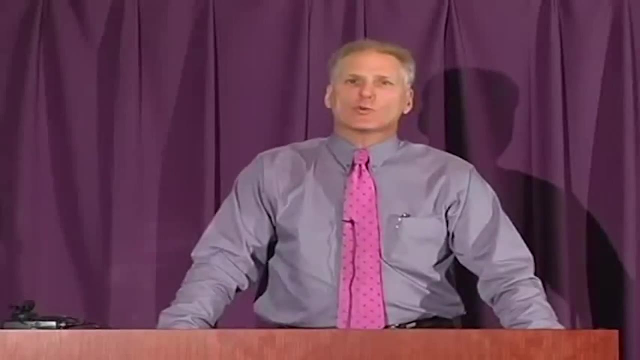 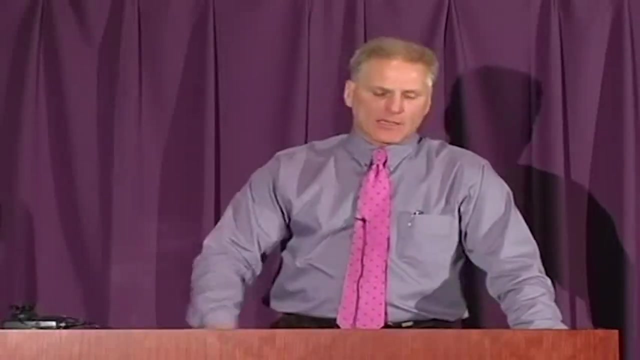 Tony Mattson. Tony and I had talked for a while. We both had independently thought up the idea of having some type of body of individuals that were very interested in fabrication sciences. so that's why we put together this Fabrication Sciences Society. Again, it goes back to that processing cycle effects. 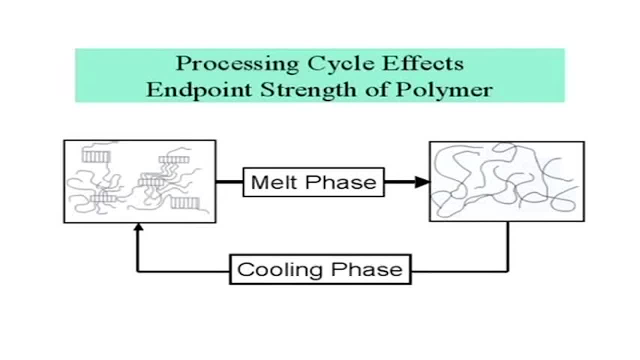 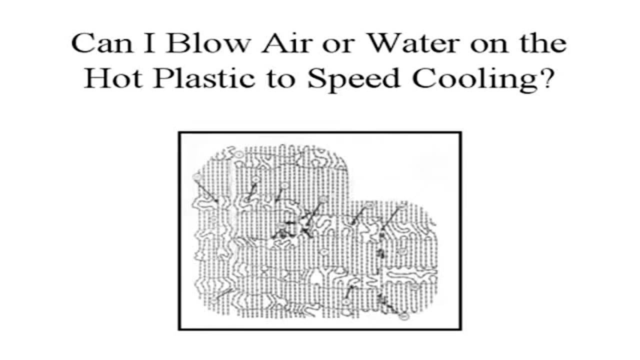 on our end point: strength of the polymer, making sure that, as it goes through the melt phase and then through the cooling phase, that we're bringing it back to its original state of specification. Wanted to tell people, from a practical standpoint, that you do not blow air or water on hot plastic. 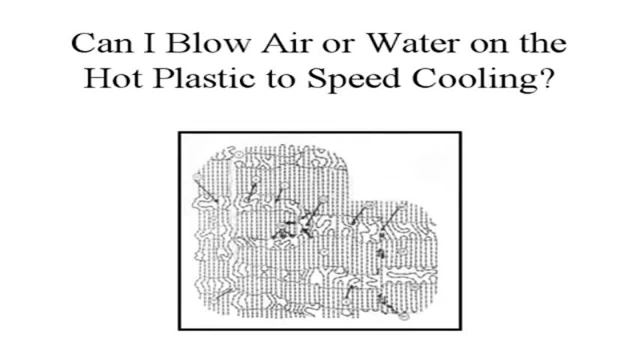 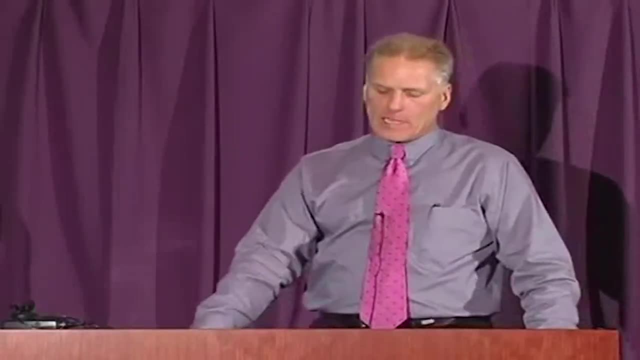 to speed the cooling. This will be detrimental to your process. We wanted to have some very practical outcome from this, but also based on using a scientific test that comes right out of the plastic industry. The other force that was pushing us in this direction was the realization. 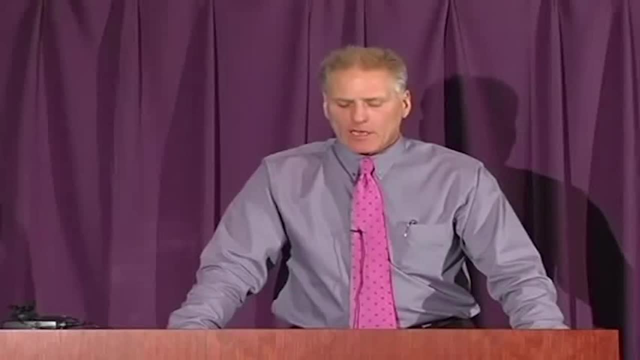 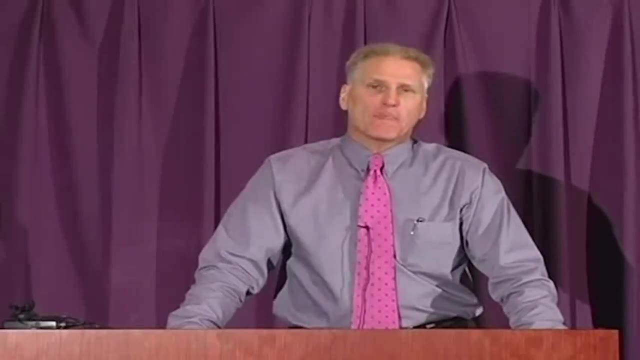 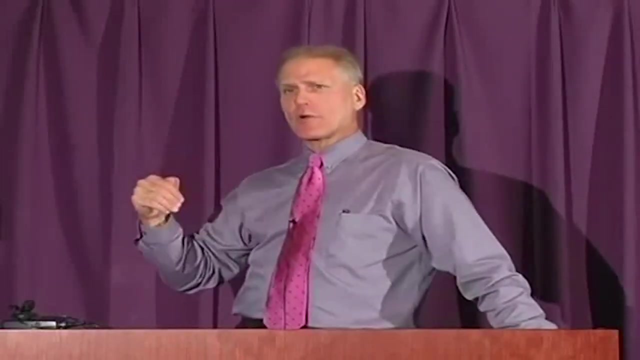 that if we accelerated the cooling of our thermoplastic materials after we vacuum foam, that we could possibly be weakening that structure. and because thermoplastics, in comparison to thermosets, are much weaker, we did not want to degrade the strength specifications of our thermoplastic materials. 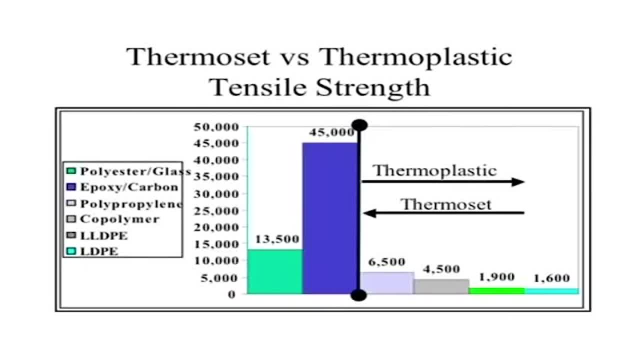 In this graph we can look at the strength differentials between thermoplastics which are to the right of the black line and thermosets which are to the left. On the right hand side, at tensile strength of 1600 PSI, is low density polyethylene. 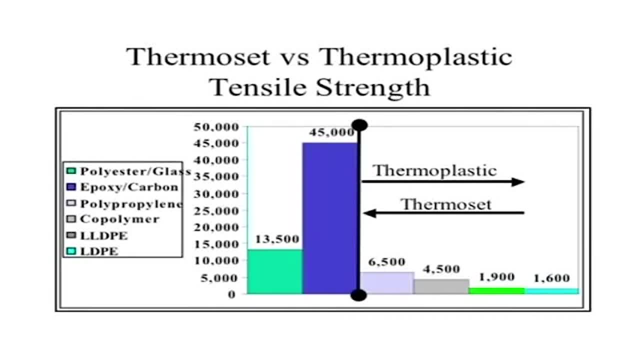 Then we have linear low density polyethylene which jumps up to 1900 PSI tensile strength, and then 4500 PSI tensile strength of the coal polymer and then 6500 PSI is book value tensile strength of polypropylene Right. 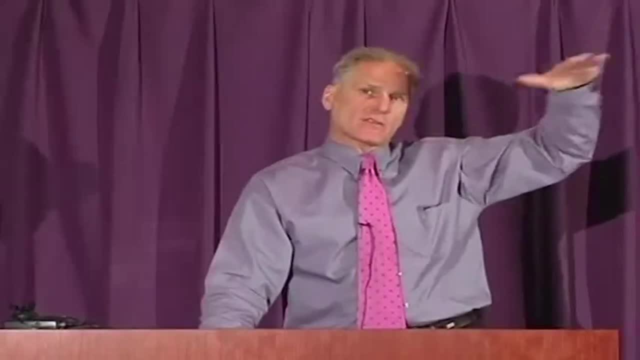 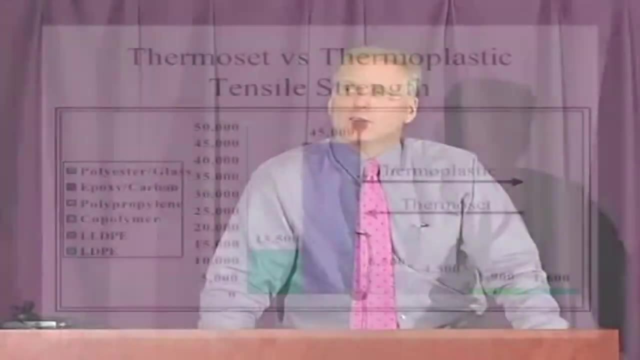 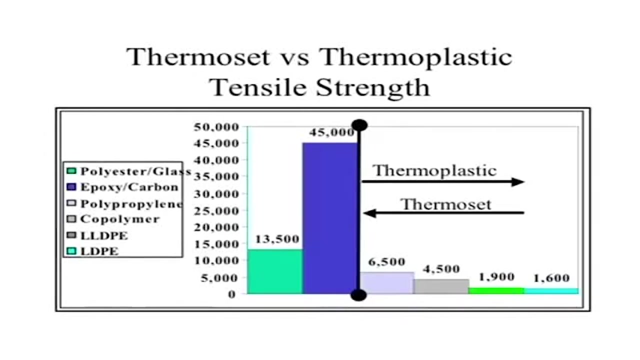 Overall you can see the gradiation of strengths of very common thermoplastic sheet materials. in our field, To the left of the black line we have the strength of an epoxy carbon fiber layout, 45000 PSI tensile strength, and then the thermoset layout. 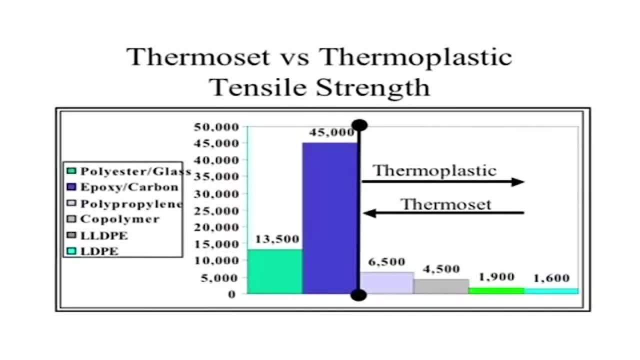 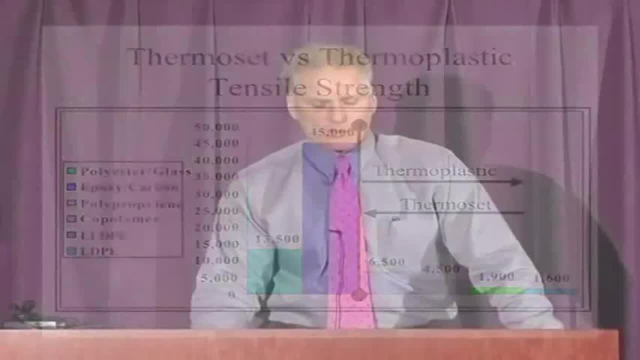 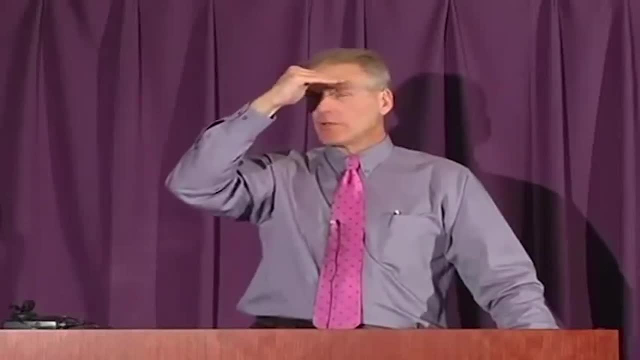 of polyester resin and fiberglass, much weaker, which is not used that widely anymore but nonetheless has been a standard lamination for many, many years. So you can see that huge differential between thermoplastics and thermosets. and so, since there was a huge differential, as a practitioner, 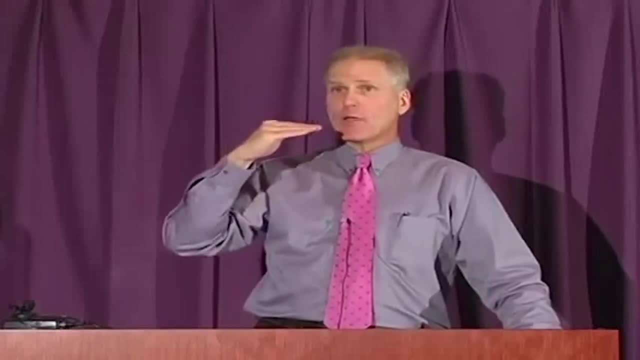 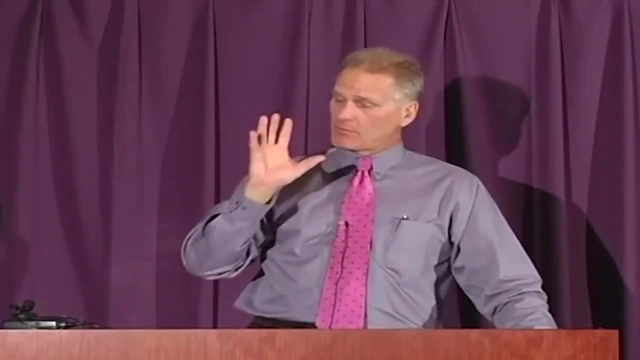 if you elected to use thermoplastics, you wanted to make sure that you had the full strength coming out of that sheet material that you had bought, so that you didn't degrade the strength of material because it's much weaker to begin with. Again looking at the difference, 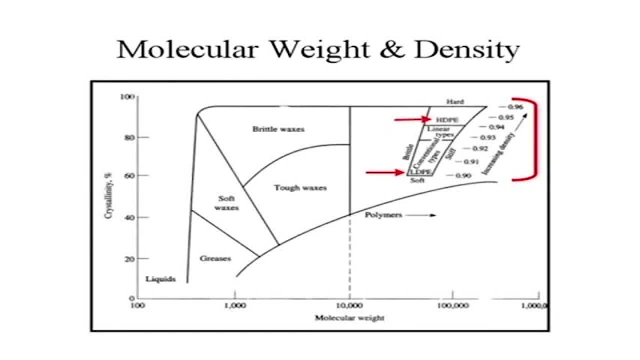 in the crystallinity of material. A very small change makes a big impact in strength. If you look at this one: low density polyethylene has a percentage of crystallinity of about 90%. high density polyethylene has a crystallinity of about 95%. 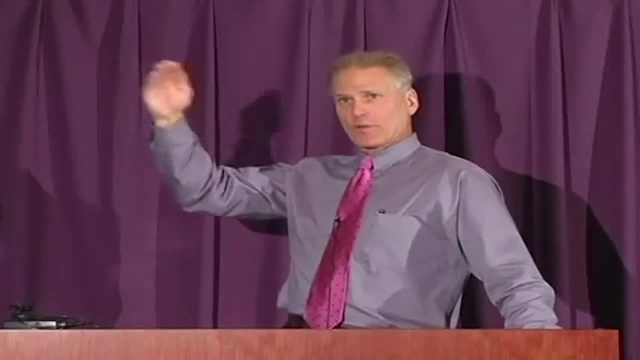 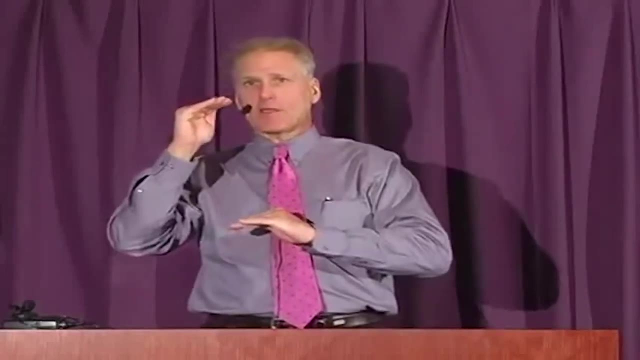 Only a 5% difference in crystallinity. So if we slow down the recrystallization of our materials, even a short or small differential in crystallinity can have a big effect on the physical characteristics of that polymer structure. So differential scanning collimetry 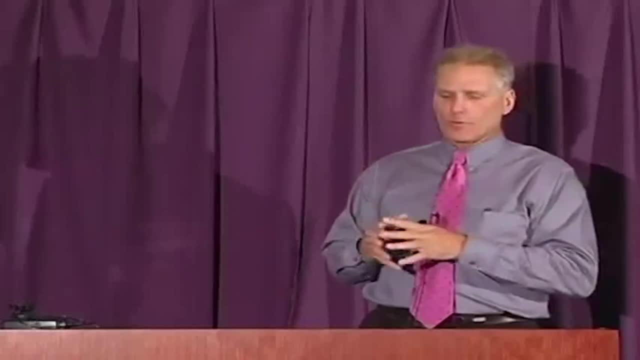 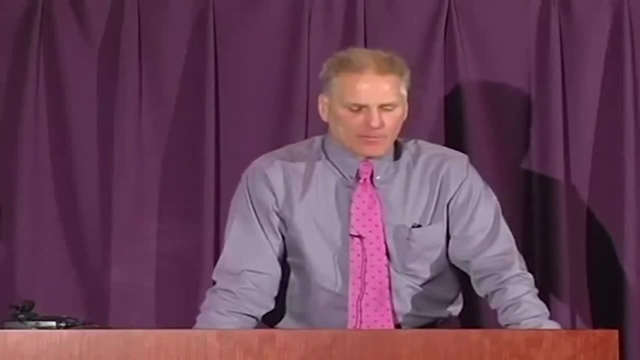 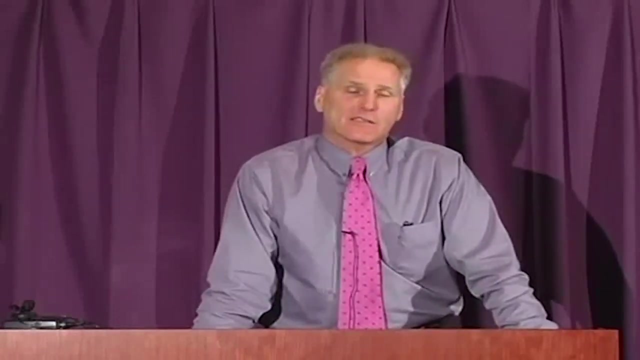 as I said, is a standard industry tool And the gentleman that did the actual testing for me writes a column for the Injection Molding Magazine, Mike Seppi. he published an article just about every month in Injection Molding Magazine called the Material Analysis And he looks at: 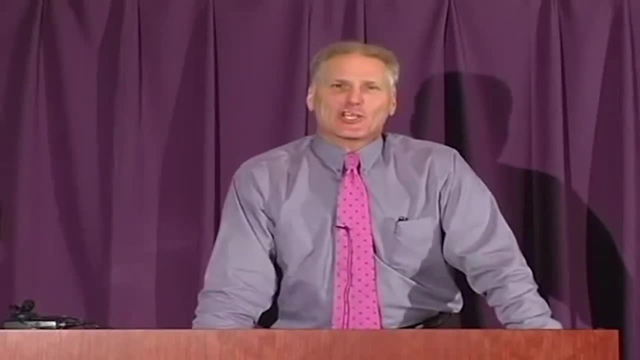 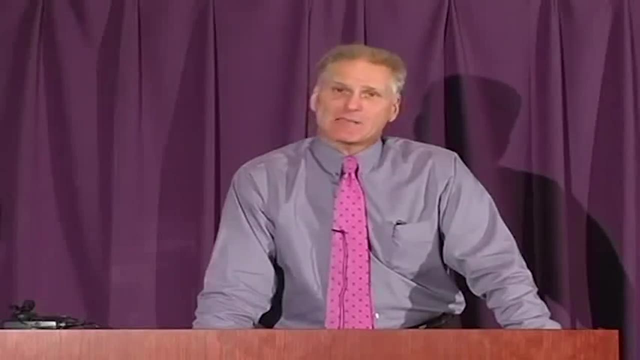 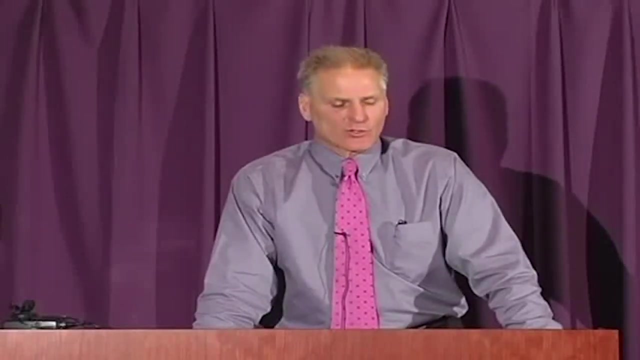 he's basically like a forensic plastics engineer: He looks at how products fail and then uses standard plastic industry testing methodology as a more or less a detective to find out why they did fail. So it always produces an interesting column, if you like that kind of thing. 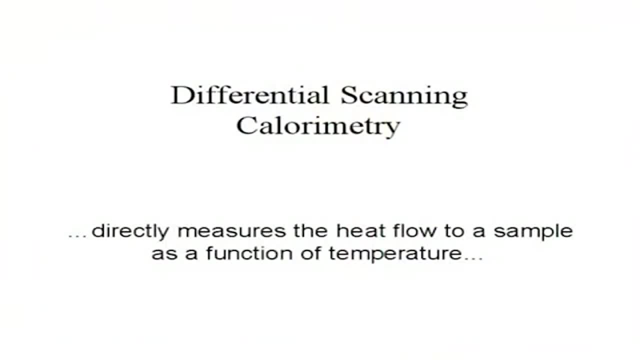 I know it's rather arcane but nonetheless it's rather interesting. But differential scanning collimetry directly measures the heat flow to a sample as a function of temperature. That's one of those again definitions that don't give much clarity What it does or what this apparatus is. 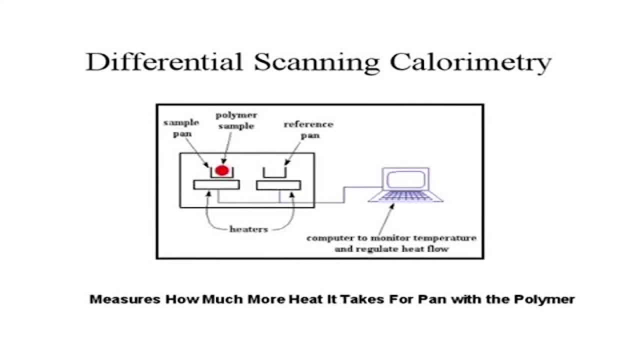 is a very sophisticated two burner stove. Two burner stove controlled by a computer. Two burner stove, two pans on top. One pan is empty. One pan has your sample of plastic. Turn the machine on. The machine heats both pans at the same rate. 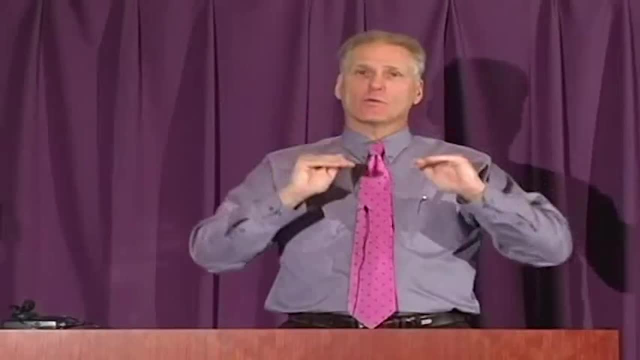 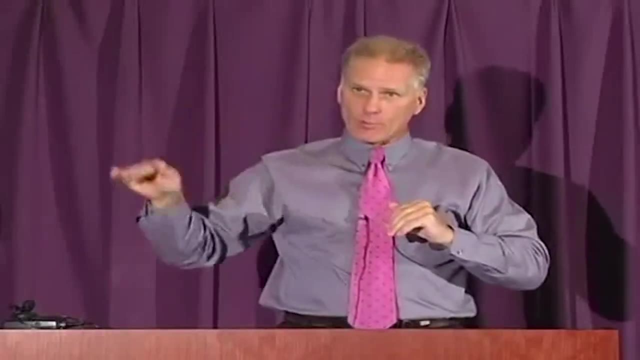 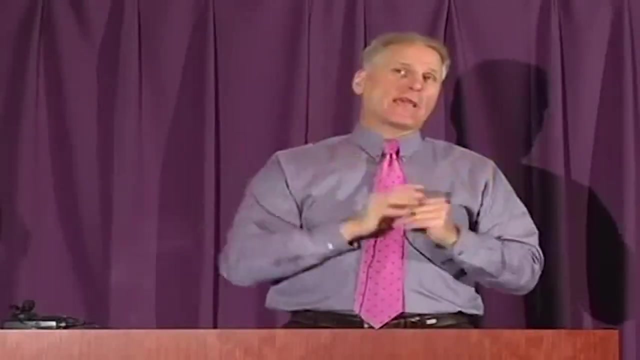 of temperature increase. Well, obviously the empty pan would want to raise much quicker than the pan with the sample in it. So the computer has to basically regulate and allow more heat flow into the pan that has your sample in it, But they both raise at the same time. 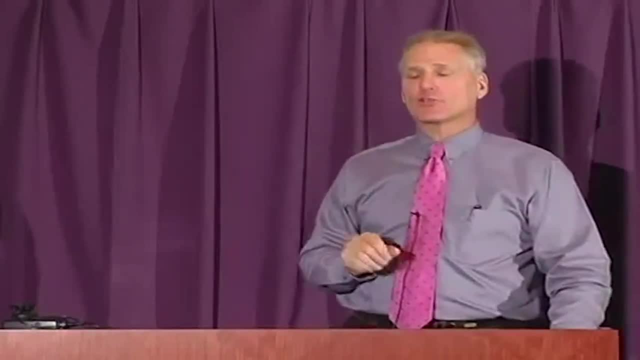 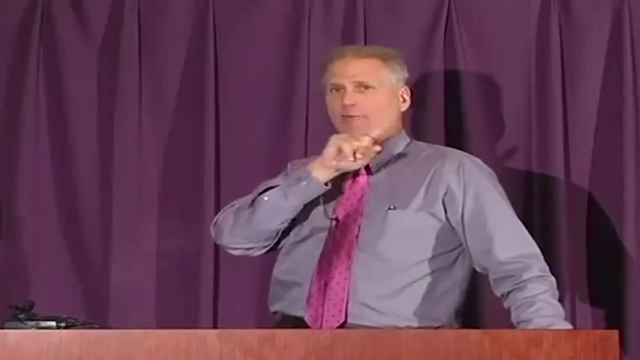 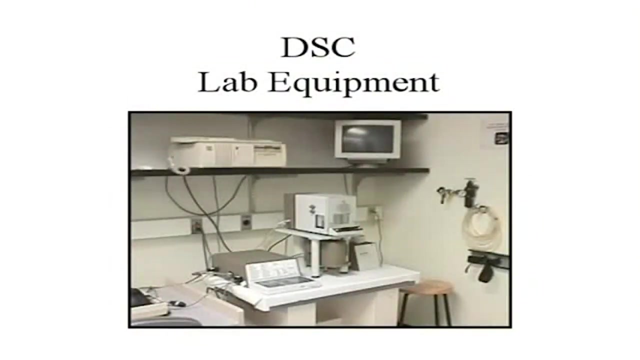 but they can measure the rate, the differential in that rate flow. So by looking at that differential we can determine quite a few characteristics of the material that's being tested. They always call them black blocks apparatus. I don't know why. It seems like they're always beige. 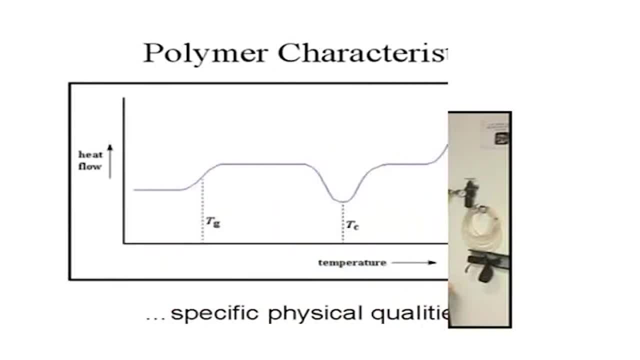 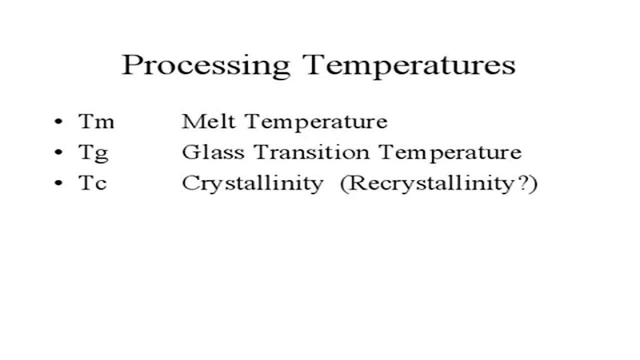 but nonetheless, this is what a DSC sample looks like And it'll give you rings of graphs, but it'll give you specific physical qualities of that specific resin. It'll give you the glass transition temperature, the temperature of crystallization and also your melt temperature. 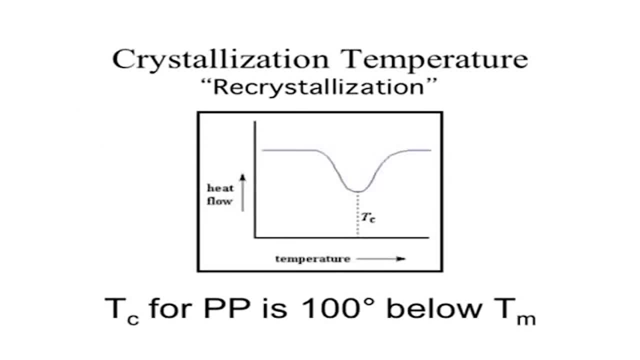 as we talked about The temperature of crystallization, which I like to think of it more along the lines for clarity of recrystallization, because you're going from, of course, you're going from crystal to melt, back to crystal. So it's in my mind, 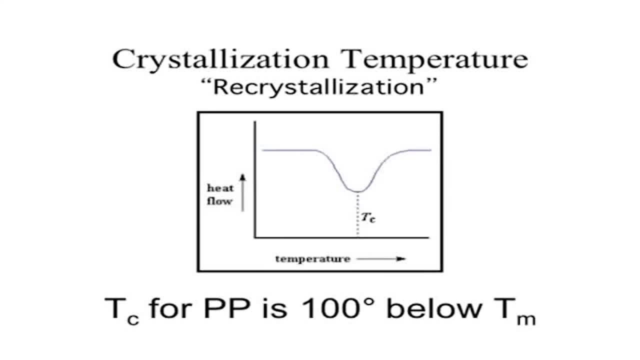 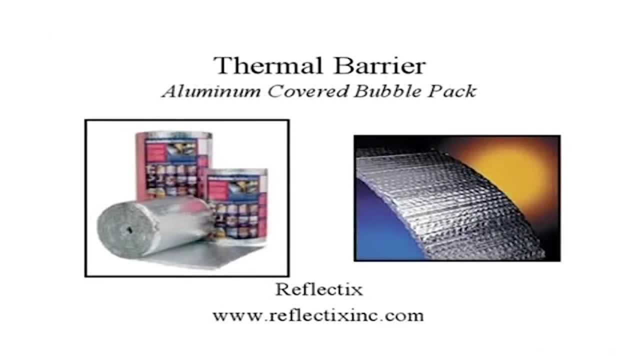 it's just clear when I think of it as recrystallization, but they call it TC. It's typically about 100 degrees centigrade below your melt temperature. As I said, this reflective material slows that process down because there is that differential. 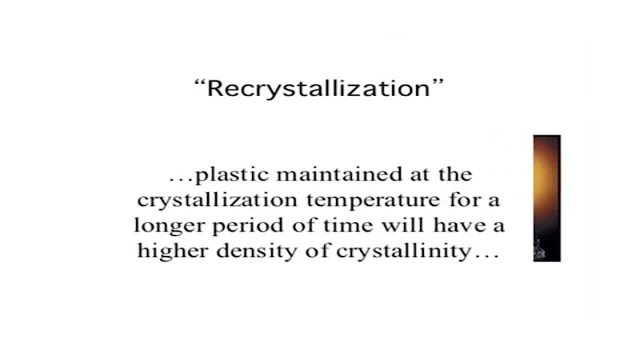 It works with us basically So in that recrystallization, as I call it, plastic maintained at the crystallization temperature for a longer period of time will have a higher density of crystallinity. That's our goal. Keep it above the set temperature. 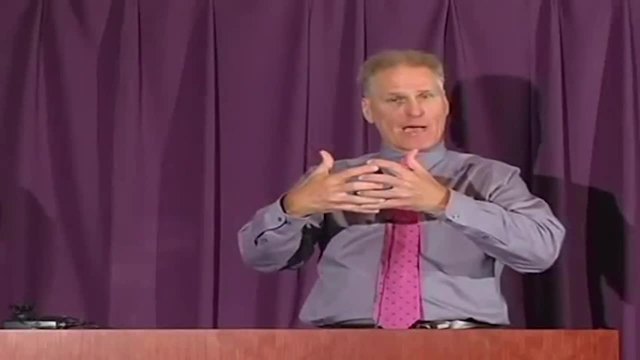 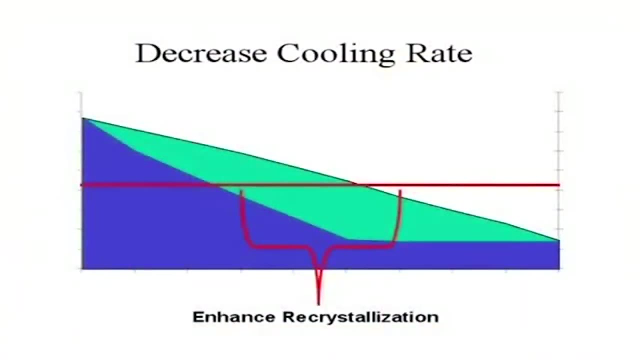 for a little bit longer period of time just allows for that polymer chains to flow. Remember it's a slow, viscous, fluid type of flow into that optimal ratio of amorphous and crystalline content. Gives us that time. We talked about that already. 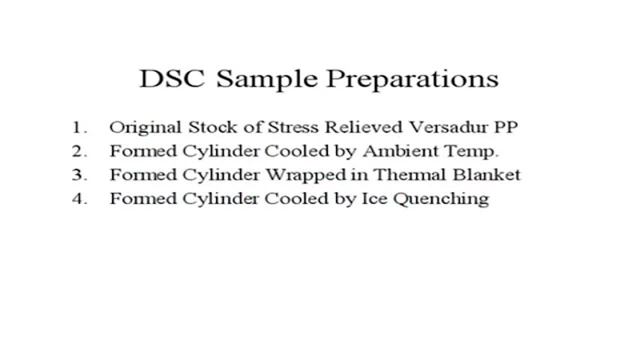 So we did four tests, Had enough funding through the small grant I received through the academy that we were able to test the percentage of crystallinity in the original large sheet of plastic that we bought. And then we did three thermal forming events. We formed on a cylinder. 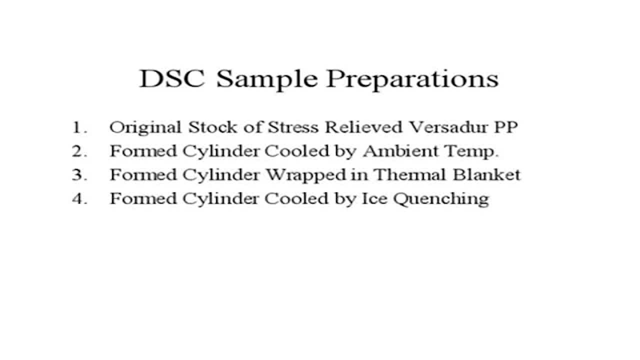 and let it cool by ambient temperature. In other words, we just vacuum, formed it, let it sit there, didn't put a fan on it, didn't put any water spritzer on it, just let it cool within our normal process. Then we formed a cylinder. thermal formed a cylinder. 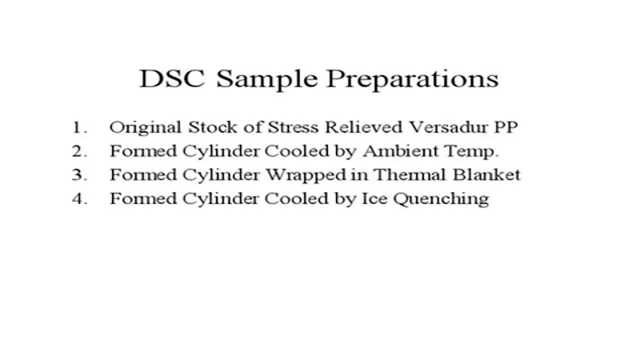 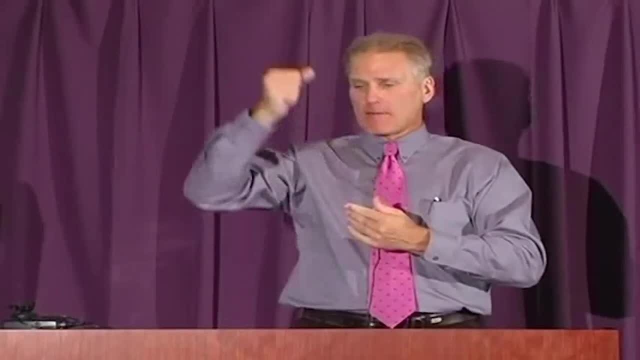 and wrapped it with a thermal blanket to slow down the cooling. And then the last one: we ice quenched it, because there are some literature citings, citations about people taking hot plastic and, boom, immediately putting it into a barrel of ice water, Quenching it. 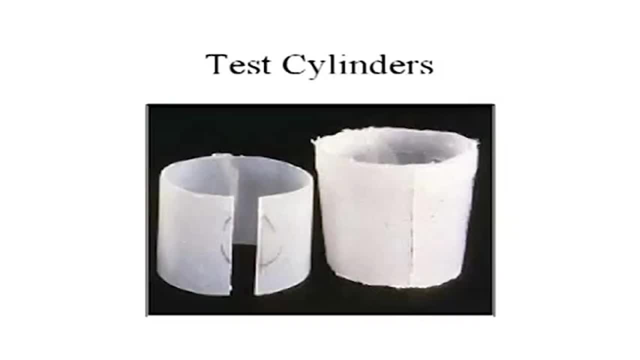 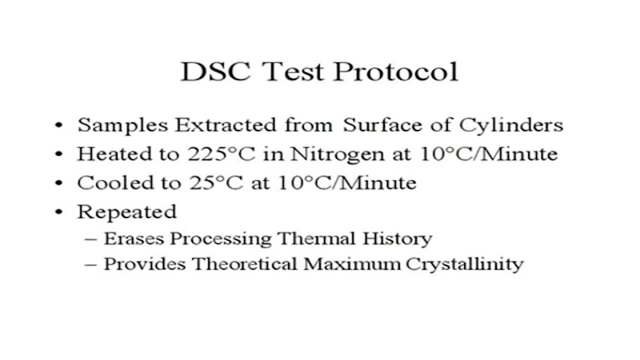 Ice quenching it. So we wanted to show that differential as well. Test cylinders. I always like to use test cylinders. The protocol of course, samples extracted from the surface of the cylinders, heated nitrogen gas, et cetera, et cetera. it just goes into. 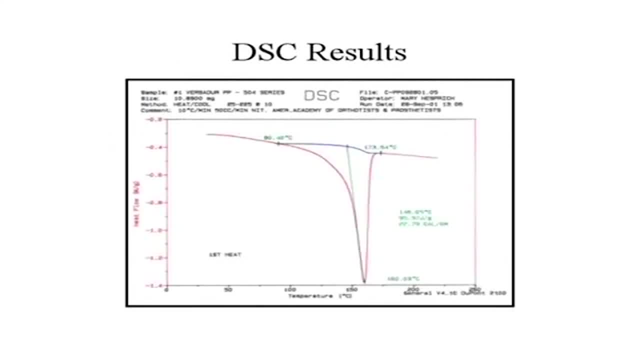 the idiosyncrasy of the test itself. We got reams of this type of readouts from the apparatus itself And then we found from a statistical standpoint that there was that the original sample had a crystallinity rate of 95.3%. 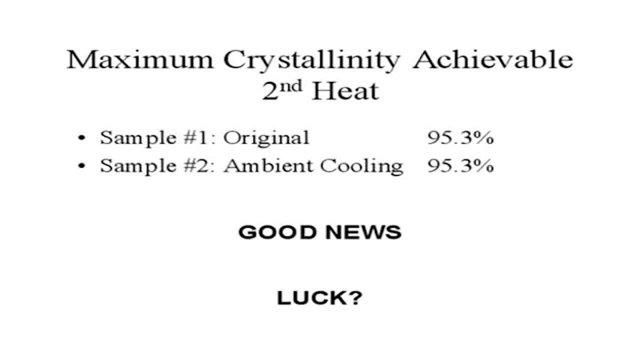 That was a coupon, just a sheet of material, Virgin seeded material. bought it from the distributor, cut a full sample, sent out for testing. 95.3% crystallinity In sample number two. we allowed that to have ambient cooling, In other words vacuformed it. 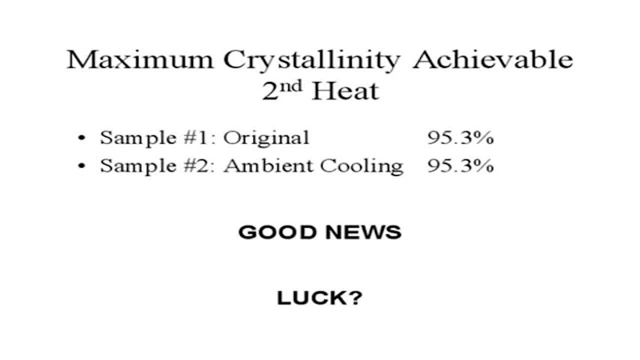 and just let it cool. It also had a crystallinity rate of 95.3.. That was a good thing, Absolutely Good news. But it wasn't luck because we knew not to speed up or accelerate the cooling of that plastic. So we did have. 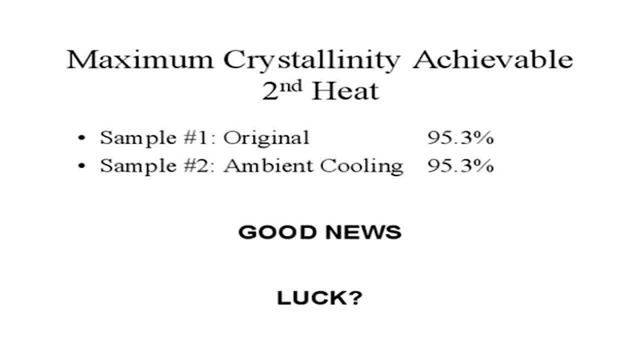 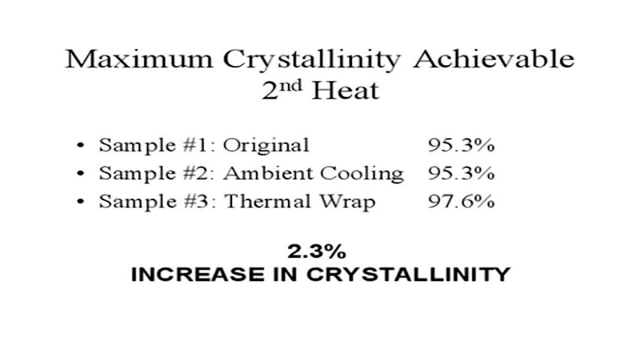 some controls in place. This wasn't an ad hoc or type of process. When we put the thermal wrap on the model and had that material tested by the DSC's, we found that we increased the crystallinity by 2.3%. Now, unfortunately, 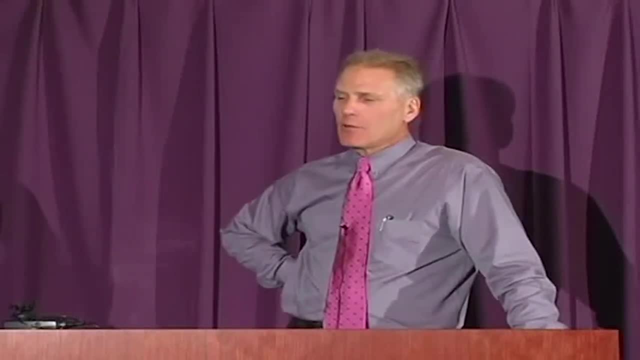 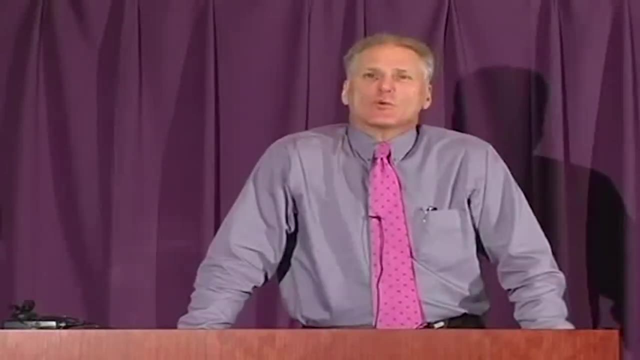 we were a little blindsided by this. When we set up the rules of our experiment, you always have a design for the experiment that you want to run. We actually were a little short-sighted. This surprised us and it shouldn't have, but it did. 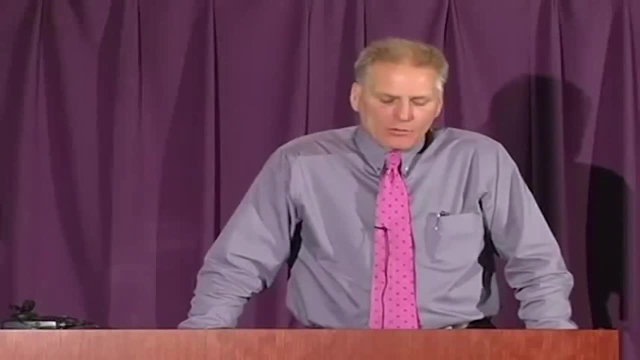 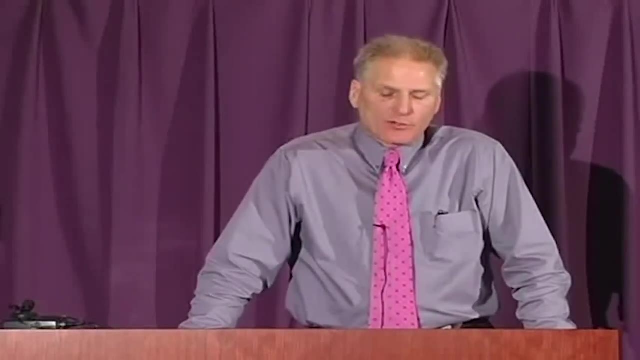 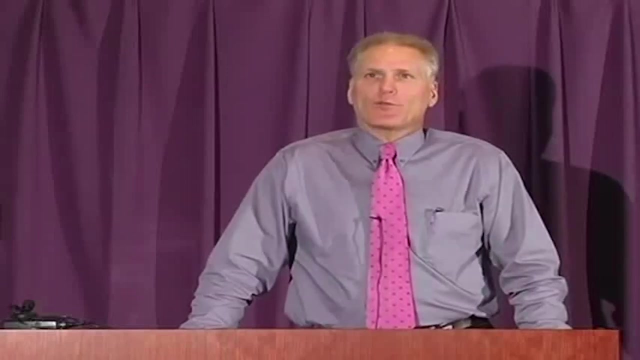 And the reason I say that is: how could we end up with an increase in crystallinity compared to the original sheet that we didn't thermoform. We had bought it from the distributor, came right from the extruder And yet it was 2.3% higher. 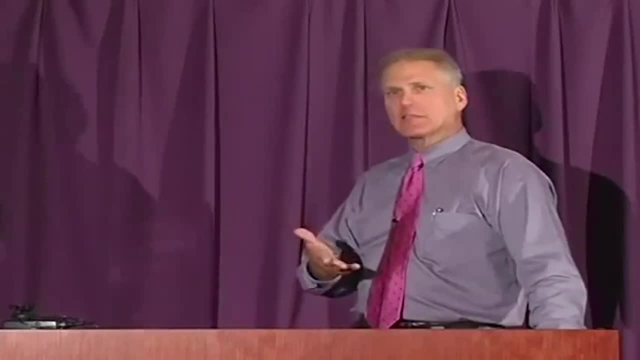 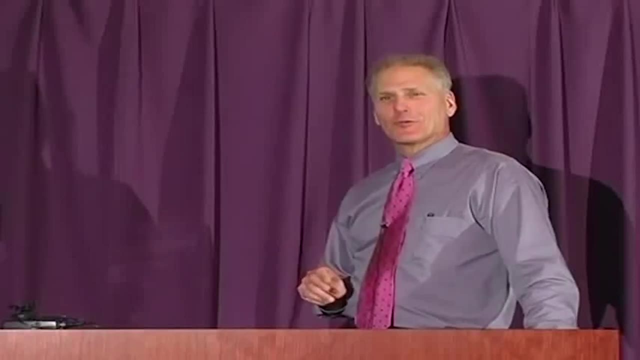 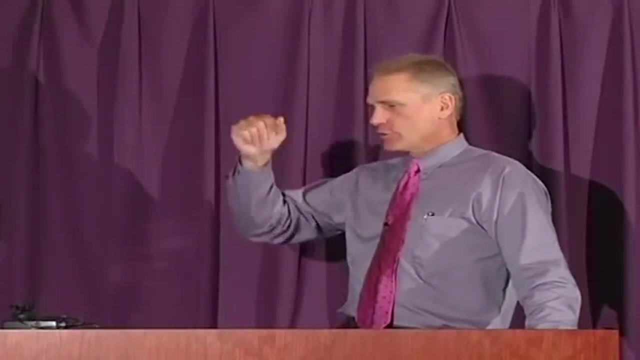 That means that was that thermoformed plastic in that cylinder was stronger than the original sheet material. And soon as we saw those figures we realized what had happened. Whatever company extruded that sheet material, took those little plastic beads, forced it through the machine and made it into a sheet. 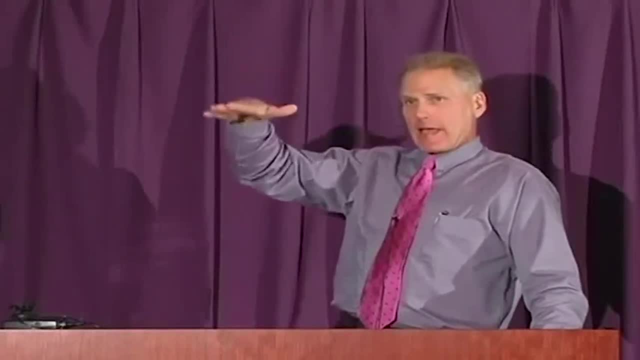 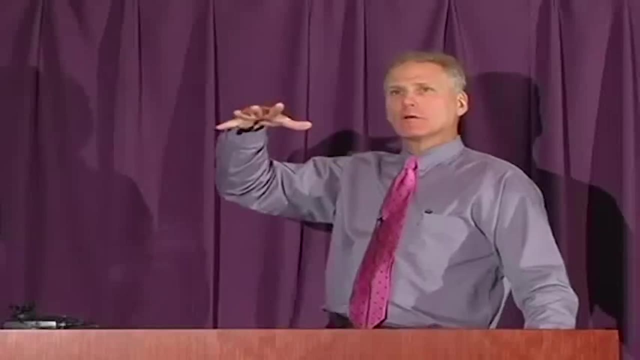 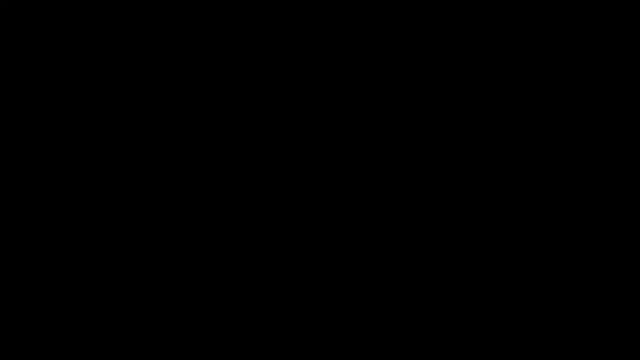 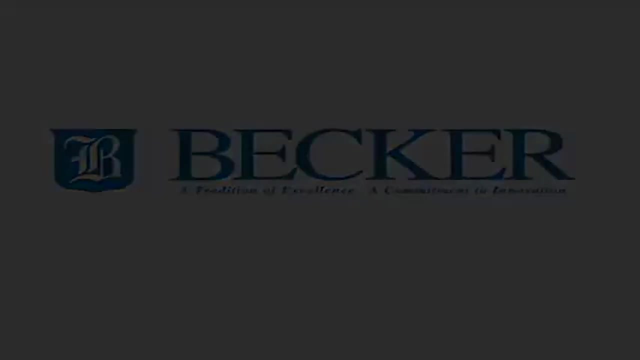 They pushed it through so fast and cooled it so quick that they actually cooled the material before it crystallized into its optimal amorphous and crystalline content. They made it weaker. They made it weaker. Now we're going to come to the last segment. 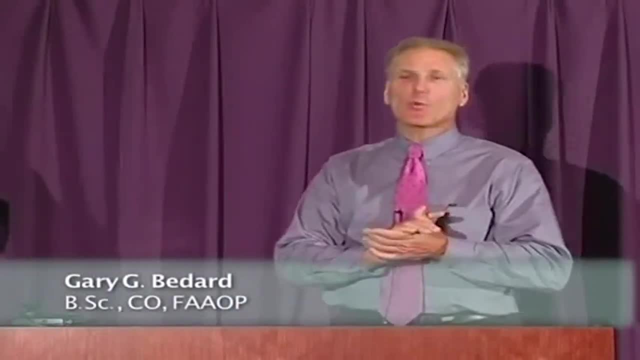 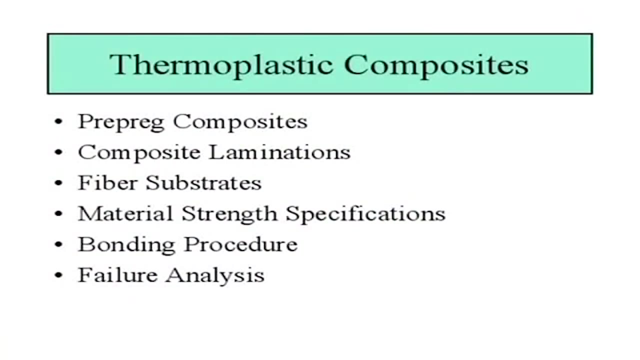 of this program. We're going to discuss thermoplastic composites, So we'll look at the meaning of pre-preg composites. We'll look at composite laminations. We'll look at fiber substrates. Material strength specifications, Bonding procedure. 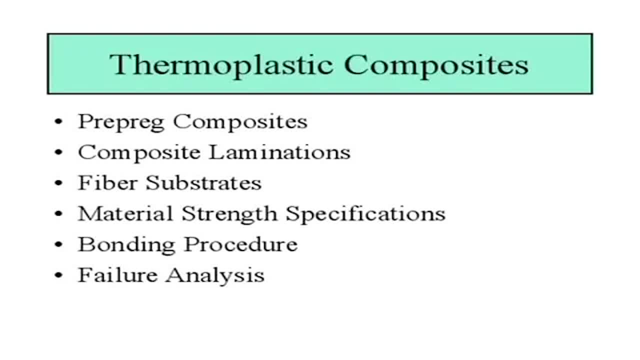 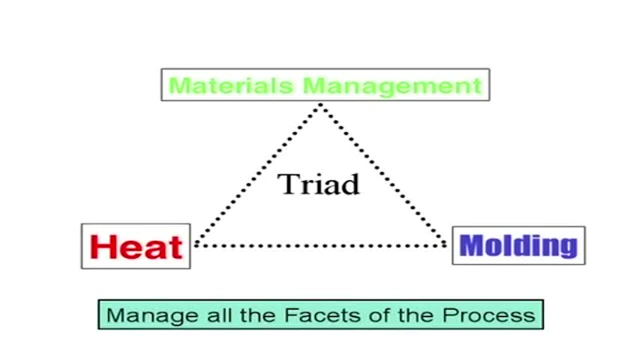 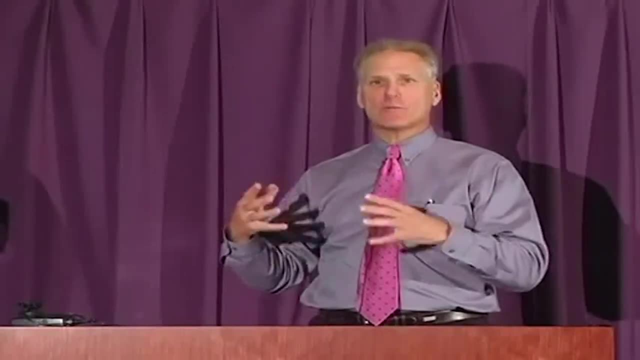 And then some failure analysis when using thermoplastic composites. This really could be thought of as advanced materials management, because we truly are moving beyond the simple thermoplastic homopolymer sheet materials into the realm of thermoplastic composites which, in looking at the world, 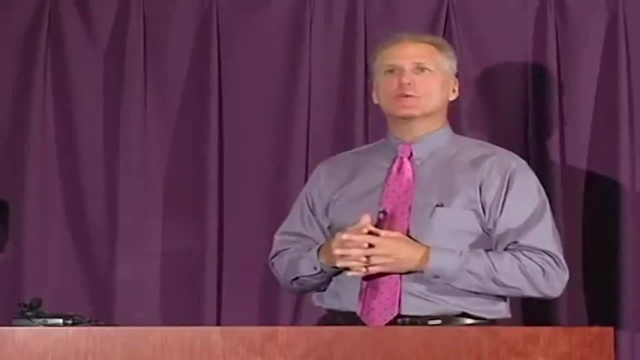 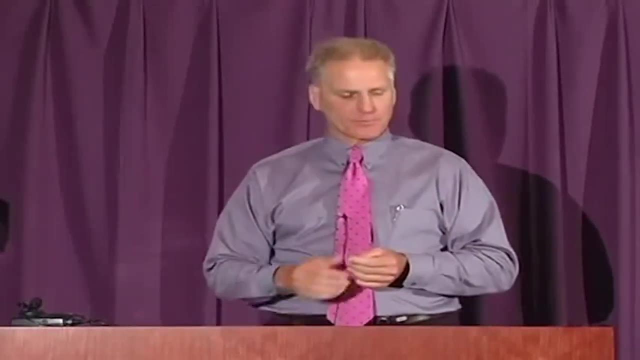 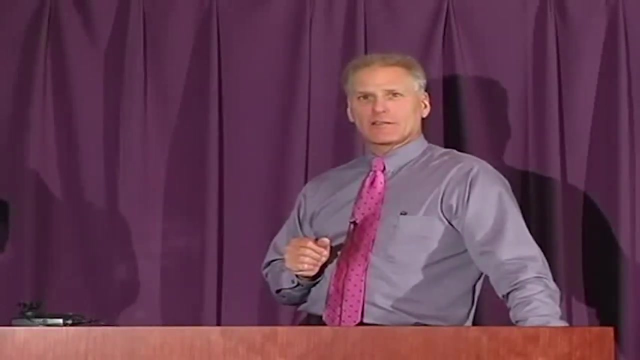 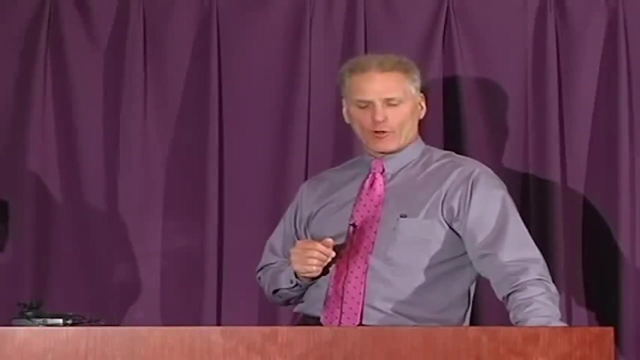 of composites. that's some of the newest technology that has been developed and is used within that field of material development. The way that I started, I should say the- I guess the incident that gave me the impetus to start this program on clinical thermoforming. 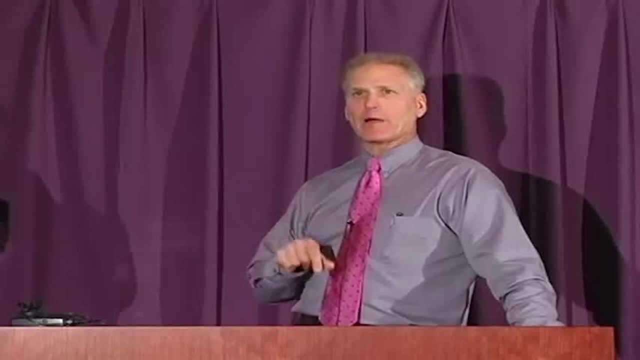 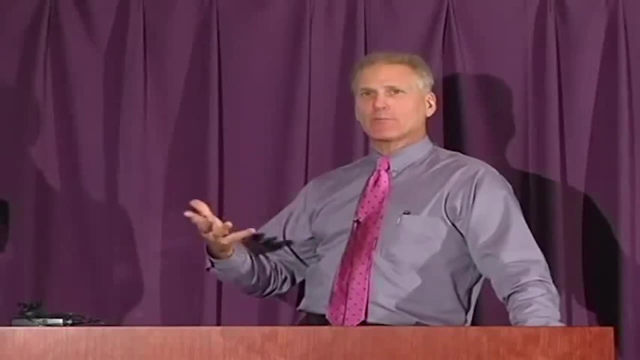 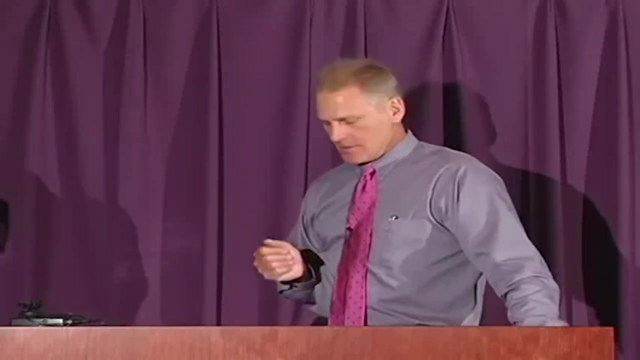 was germinated by a question from a composite engineer at the company that was providing me with my precursor- pre-preg thermoplastic tapes that I was using in the development of Comcor, And after having a conversation with this engineer, who I knew quite well. 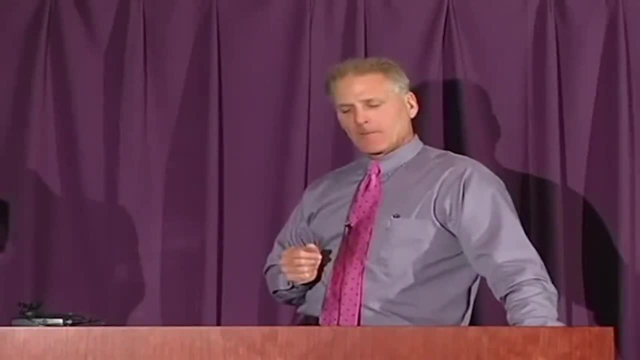 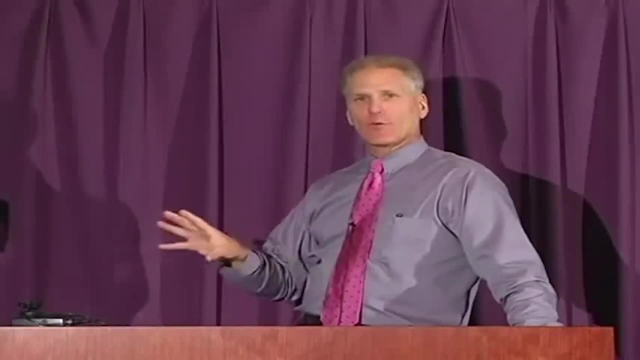 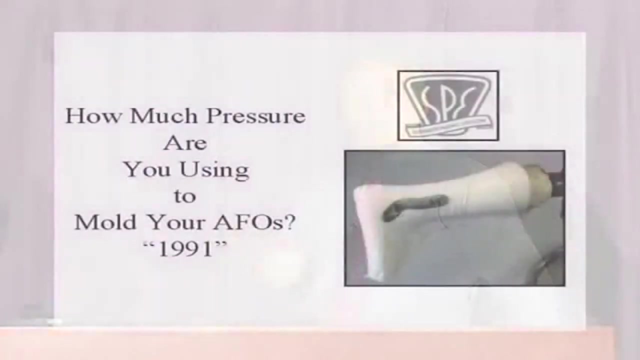 through a series of projects. I was describing to him a week of failures, of trying to do a specific layup to reinforce solid ankle AFOs or just reinforce a thermoplastic device And at one point in our conversation he said: how much pressure are you using? 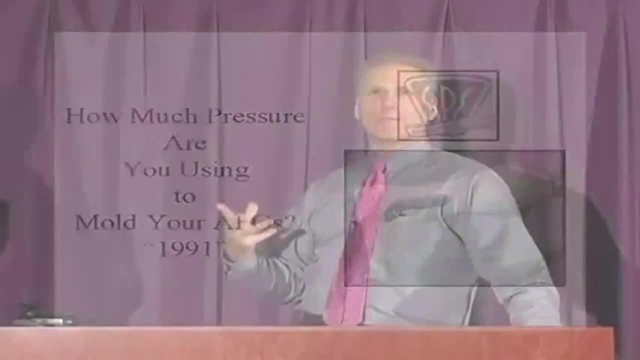 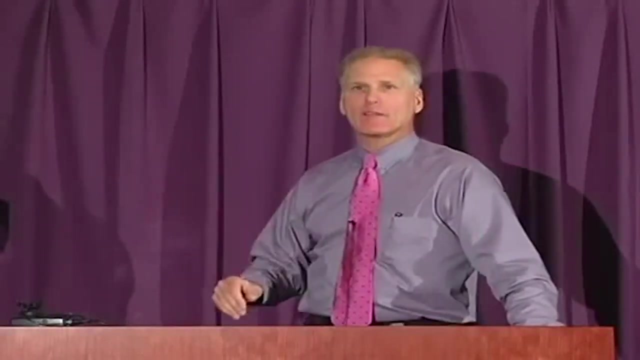 to mold your AFOs. This was back in 1991.. And at that point in time I had no frame of context in terms of how to respond to him. I had gone through the program at the University of Washington in orthotics and prosthetics. 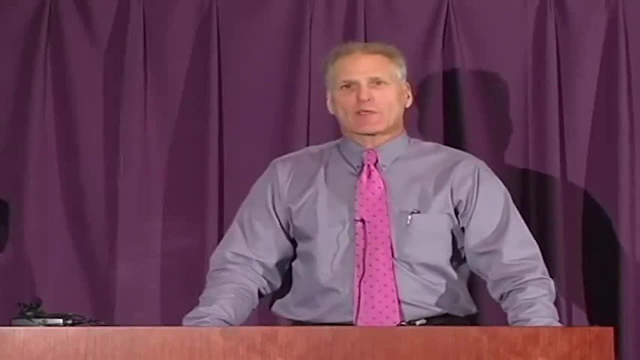 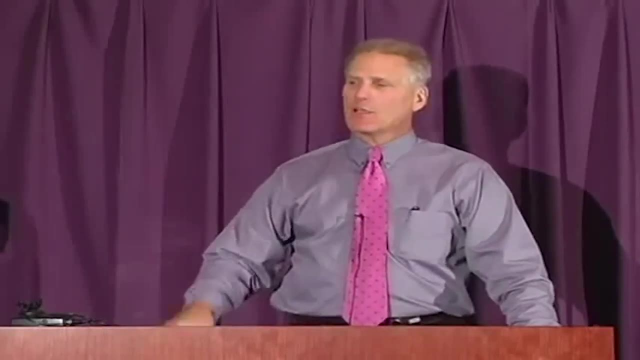 never heard anybody talk about process pressures in order to fabricate an AFO. I had been in the field many years, both institutionally at Stanford Private Practice and SCOPE in San Diego. I was manufacturing knee braces for a few years and then went on. 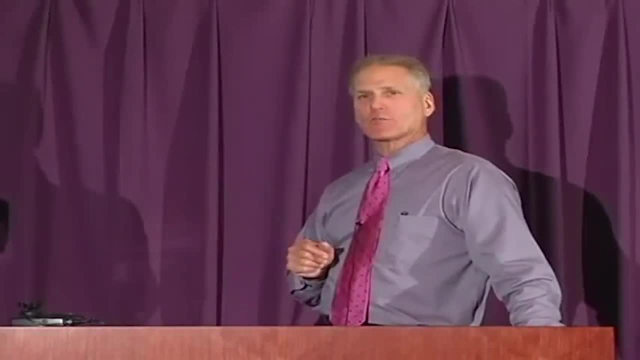 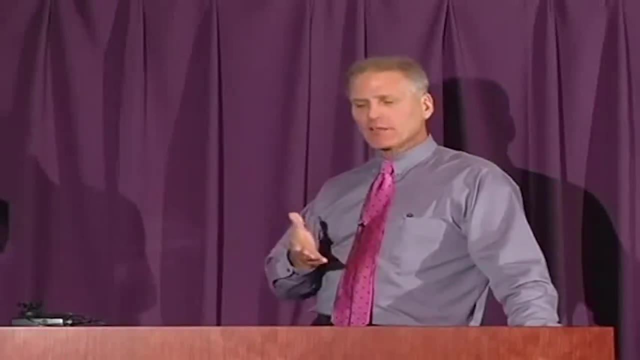 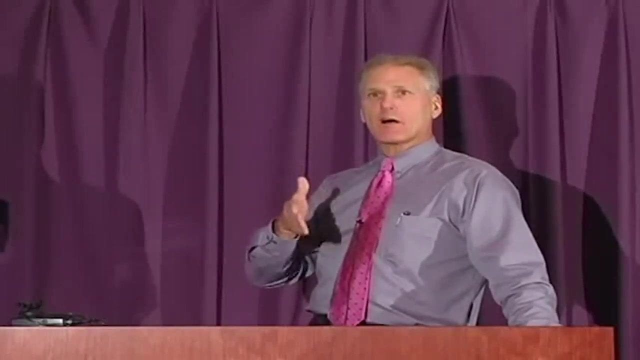 with Becker Orthopedic Never heard anybody talk about process parameters when it specifically came down to our clinical thermoforming. So it was at that point in time that internally at Becker Orthopedic we stopped our development of Comcor and basically started on this discovery pathway. 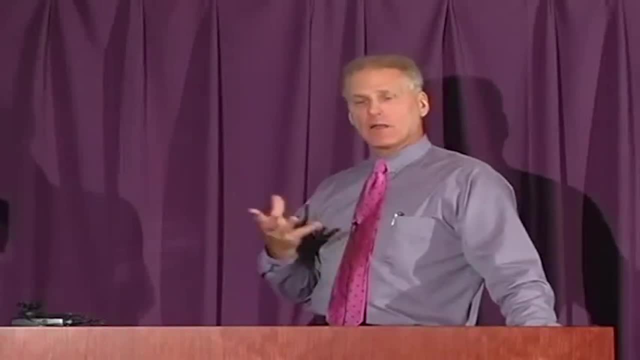 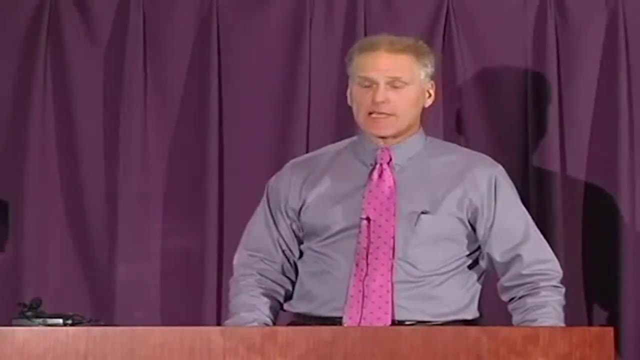 to find a solution to bringing our O&P lab processes up to an industrial level. So that's where it all started and that's when I joined the Society of Plastics Engineers At the University of Washington. I have to admit, I learned the thermoforming procedure. 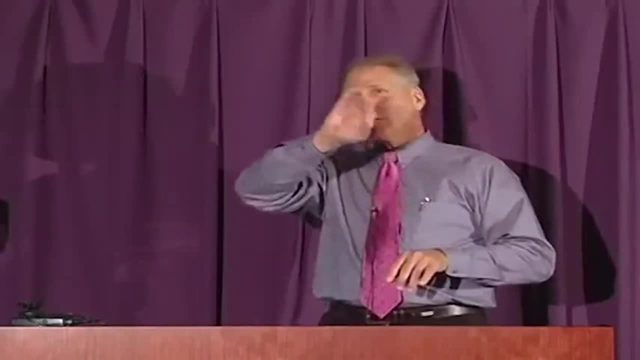 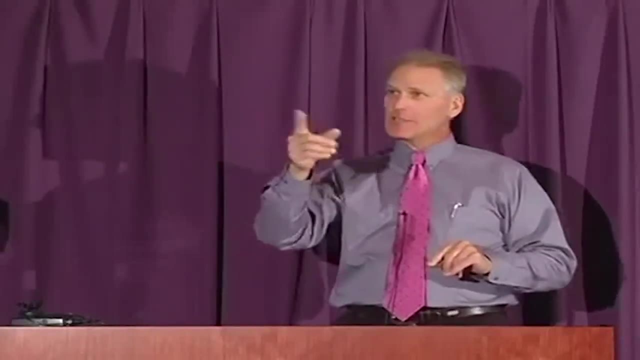 much like everybody else. We had a simple vacuum pump, braided- not vacuum line but braided ear line running directly from the vacuum pump, as you can see in this illustration, going to the inside of the pipe. mandrel for the AFO, You would seal that off. 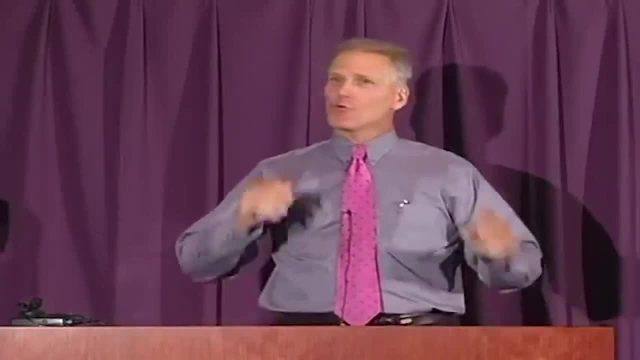 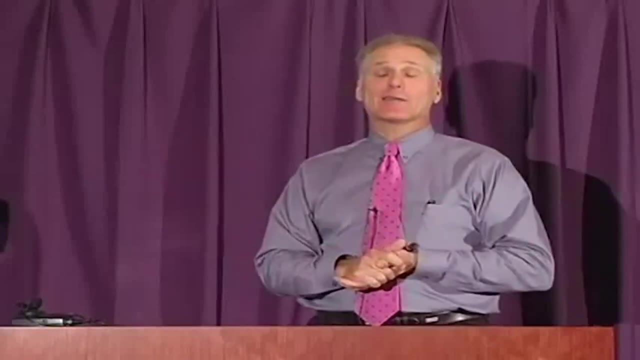 drill a little hole in your mandrel itself. put the piece of plastic in the oven. it would turn clear. somebody would turn on that machine. that made the sucking noise. wrap plastic on it and that's how I learned how to vacuum form, Very empirical in nature. 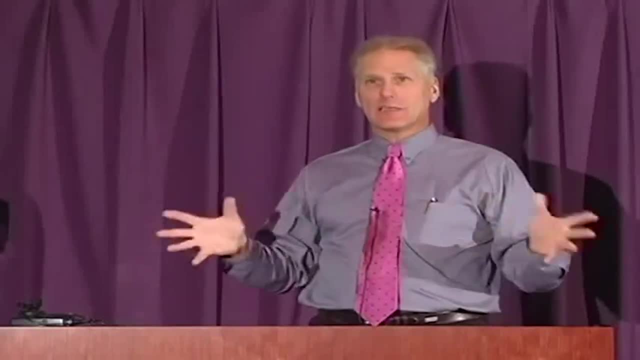 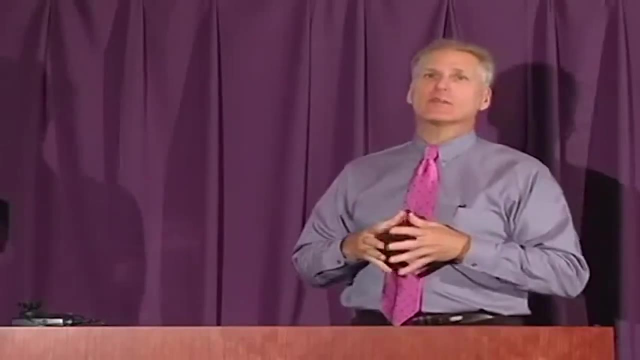 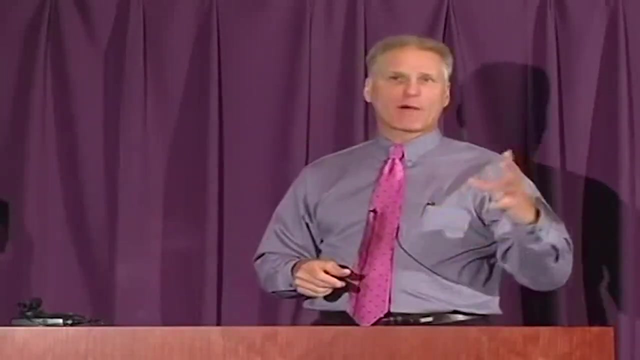 very easy to learn. Thermoforming is a very simple process. When it comes down to understanding the science of it, it can be as sophisticated as any other manufacturing process, whether you're using thermoplastic materials, composites or metals. Comcor is what we'll talk a little bit. 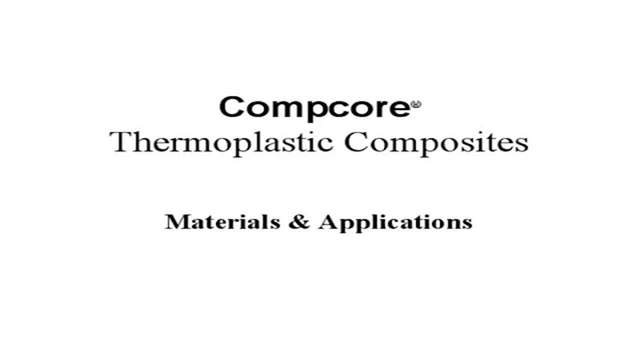 about in this segment. The first time I presented a paper on this was at an AOPA combined regional meeting back in 1992 in Reno, Nevada. It is a thermoplastic prepreg composite, the first polypropylene based thermoplastic composite used in our field. 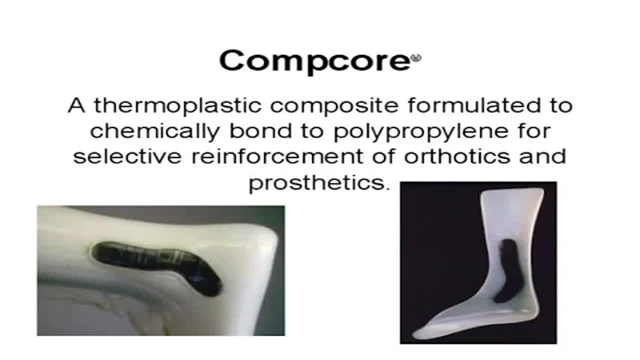 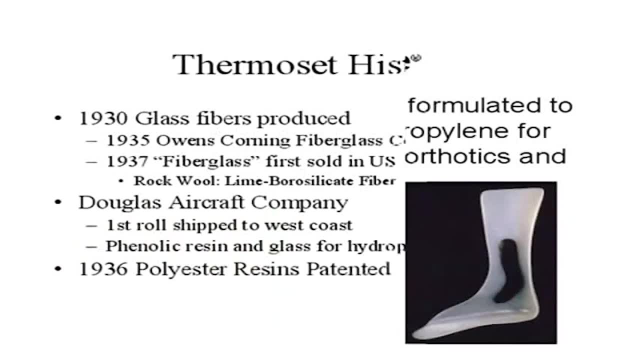 Comcor is a thermoplastic composite that is formulated to chemically bond to polypropylene for selective reinforcement of orthotics and prosthetics. To get away from that, though, I always like to go through a little bit of history of composites. Glass fibers were first produced. in 1935 at the Owens Corning Fiberglass Company. That was a combination of two different companies coming together in a conglomerate. Fiberglass, itself as a trade name, was first sold in the United States in 1937.. Ironically, the story within the aircraft industry is their west coast salesman walked into the Douglas Aircraft Company. If you know- DC-3s and some of the war planes, C-47s and then all the commercial airliners that came after the war- a lot of them were Douglas aircraft. 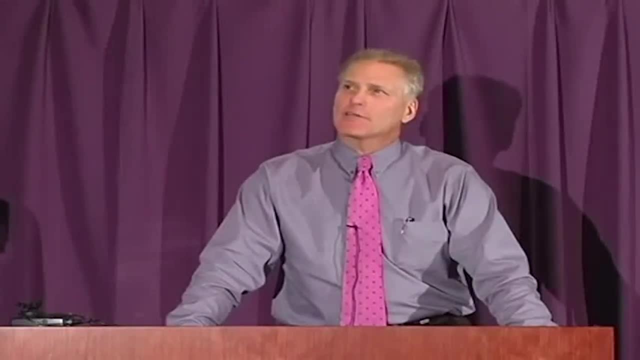 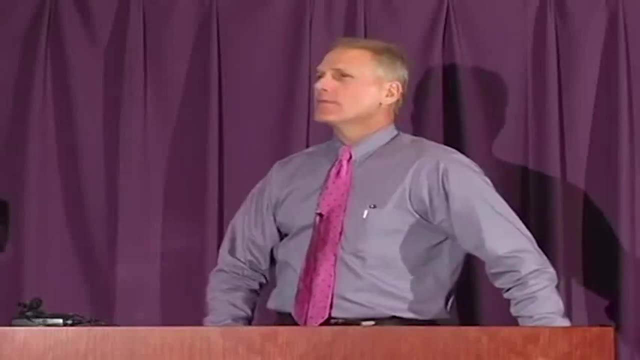 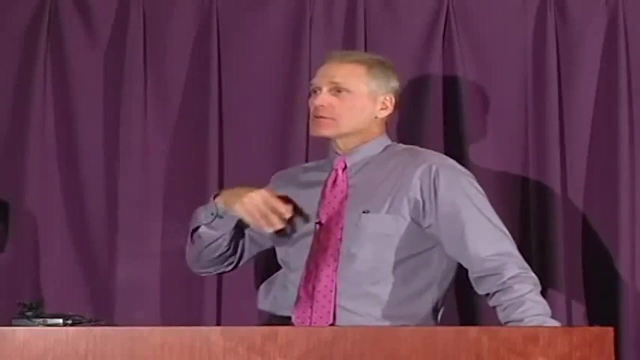 Apparently, this west coast sales representative walked into the Douglas Aircraft Company with this roll of fiberglass And the engineers looked at this material and thought that they could take some of their phenolic resin, mix it in with the fiberglass glass fibers and make molds for their hydro presses. 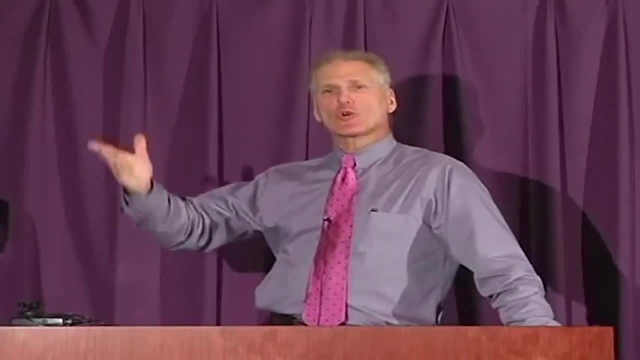 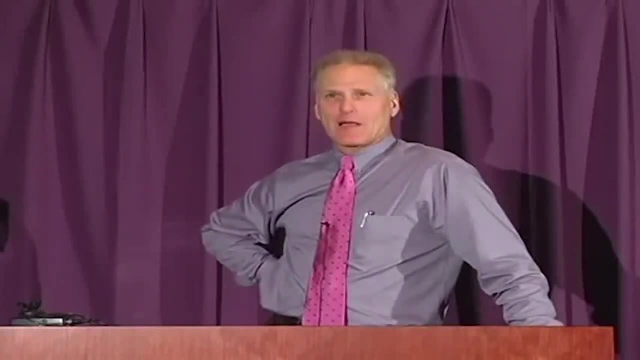 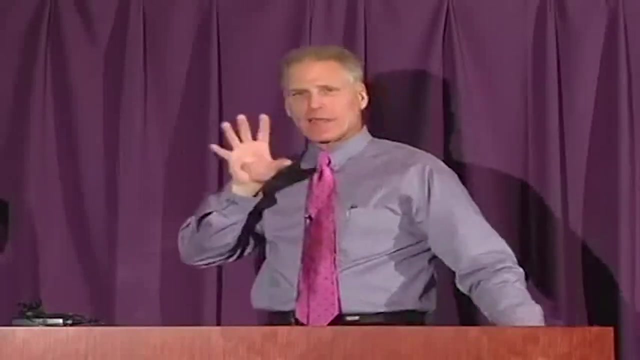 in order to form the compound curves of the aluminum skin for aircraft fuselages. So to this day fiberglass is more or less the generic term for fiber reinforced plastic. So as earlier I talked about that, you know different use in semantics or lingo within various fields. 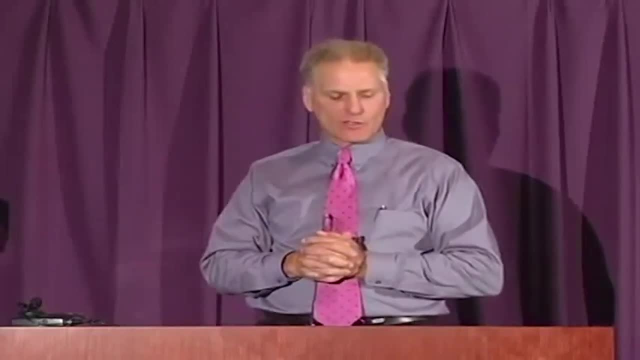 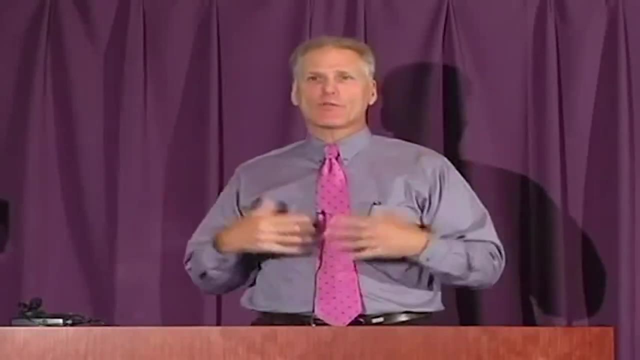 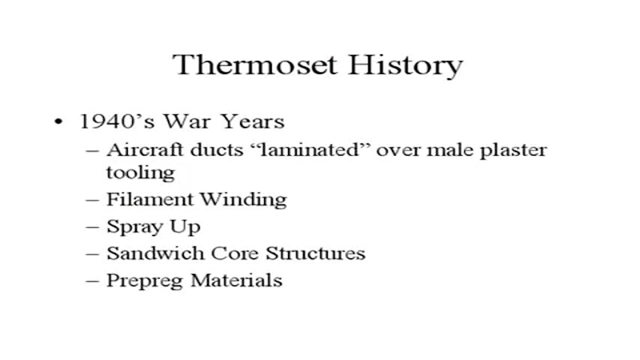 how it's not always translates directly across the board. Polyester resin was only developed in 1936. So really that was the birth of our thermal set composites. at that point in time, During the war years, they were using a- they called it a laminated method. 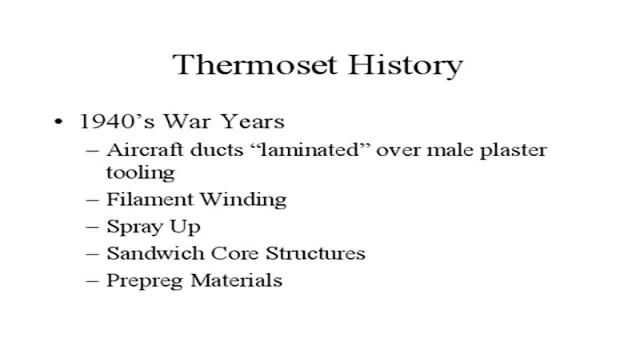 of forming thermal sets over plaster tooling to make the long, convoluted cooling ducts for fighter aircraft. So our technique of using a positive model from a residual limb comes directly from that aerospace technology. at that point in time I should even call it. 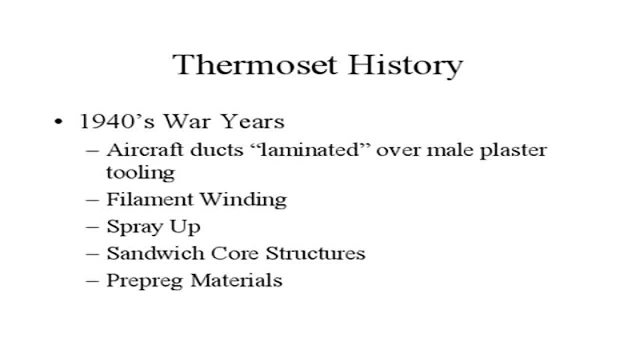 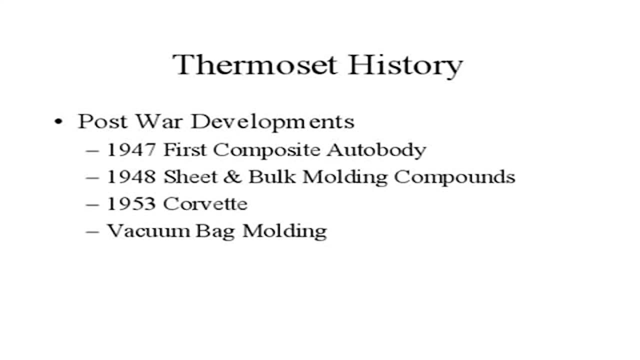 aerospace aircraft industry at that point in time In the war years. they also developed the means for filament winding. They developed means for spray layups, Sandwich core structures and, of course, the beginning of prepreg materials. Post war we had the first composite automobile bodies completed. 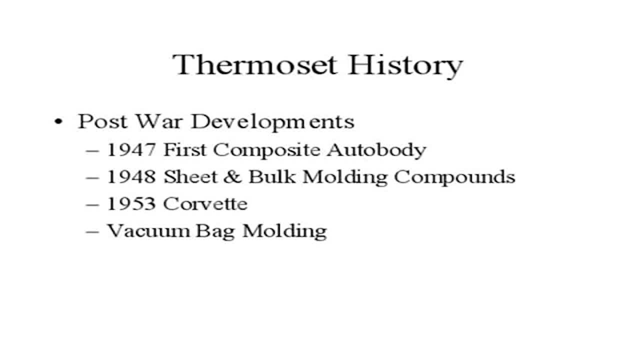 They had sheet molding compounds that are still used to this day to form into the body panels for automobiles. The corvette, which has always been a composite body on a metal frame, was first introduced to the public in 1953. And then, of course, vacuum molding. 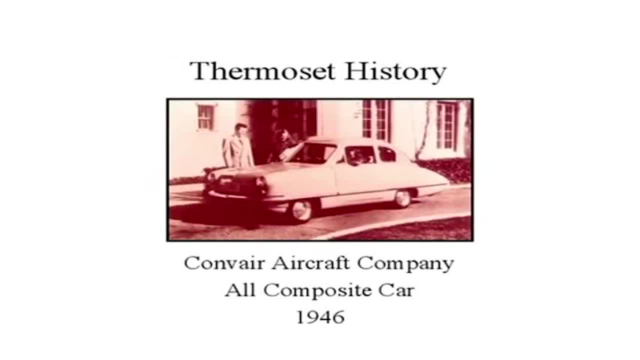 was also developed back then. The Convair Aircraft Company at one point in time had a research project in house where they produced an all composite automobile. Even down to the wheels themselves were all composites. And this was in the post war years when of course they were looking. 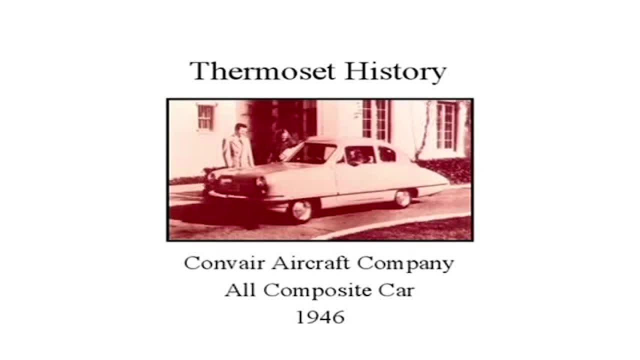 to augment their sales because there was no longer the defense department type of manufacturing for the war effort. They were looking to produce some civilian products And they thought all the pilots coming being discharged from the Air Force and the Navy and the Marines following World War II. 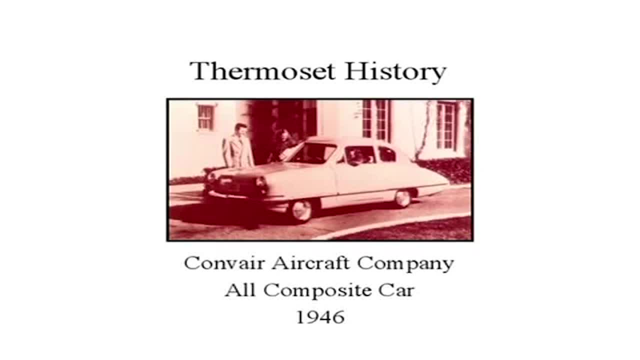 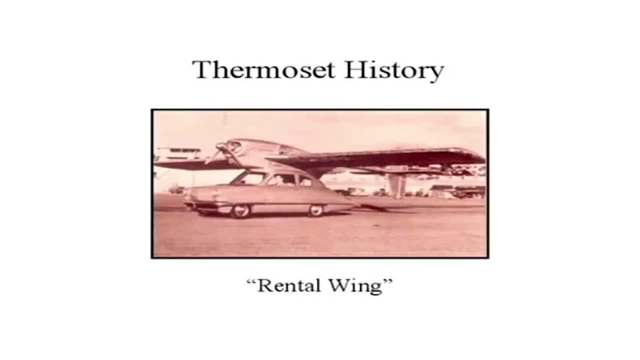 would possibly like to be able to take their family on vacation and, rather than driving the complete distance to be on vacation, that they would rent this wing and motor kind of apparatus that would strap to the top of the car, have a rudder, wings, motor. 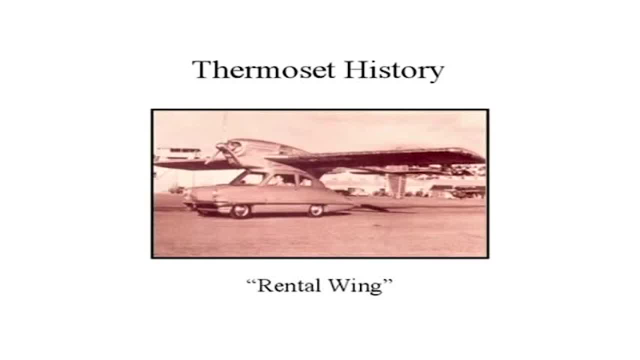 and then fly to a destination, drop off the rings at their local Hertz, rent the wings and go on vacation with their family. come back to the rental agency, strap the wings back on, fly back home and drop off the wings at the Hertz rental agency. 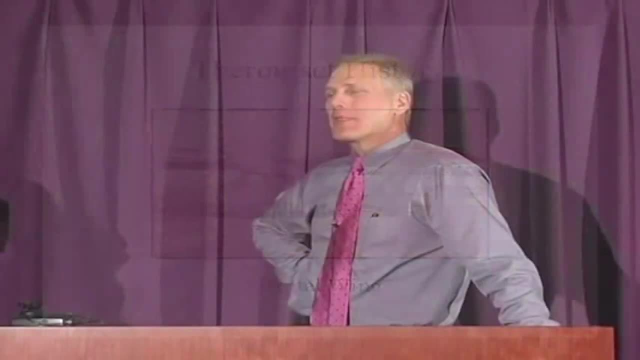 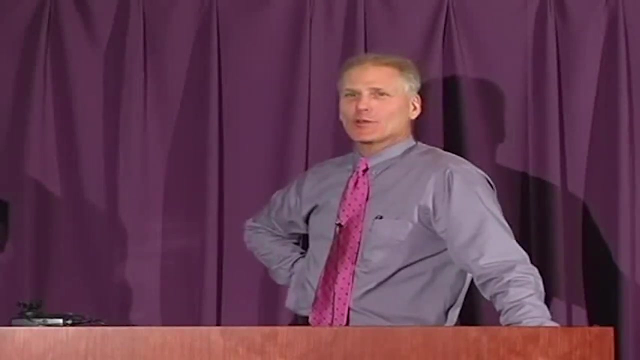 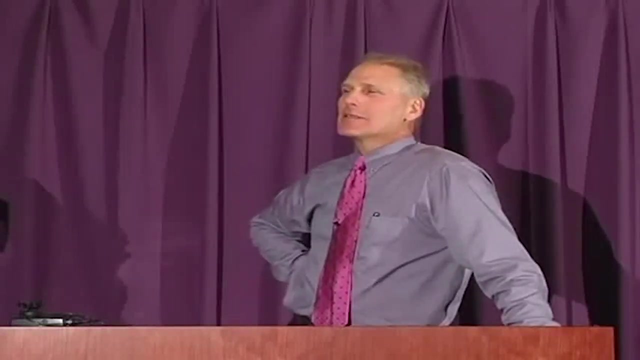 I'm just using Hertz as a fictional. obviously, This was actually an FAA certified aircraft, Never went into mainstream production, but was flown by pilots on this kind of convertible car. I'm actually kind of happy that this did not come to be, because I can just imagine. 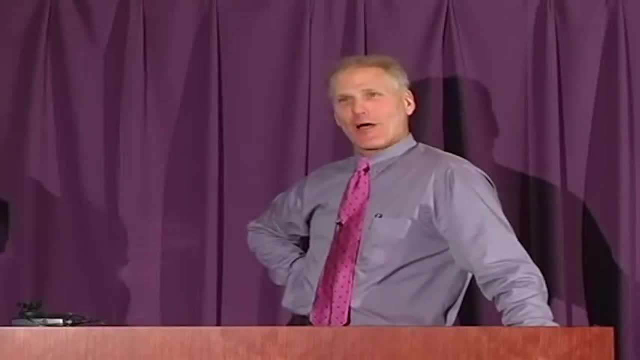 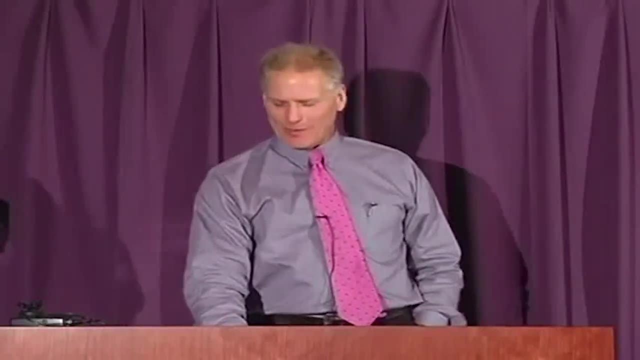 all the SUV drivers that are on the road being up in the air flying and, as a pilot, myself not wanting to be with that type of driver, so to speak. So it was an interesting tidbit, I think, to the composite industry In our 1960s. 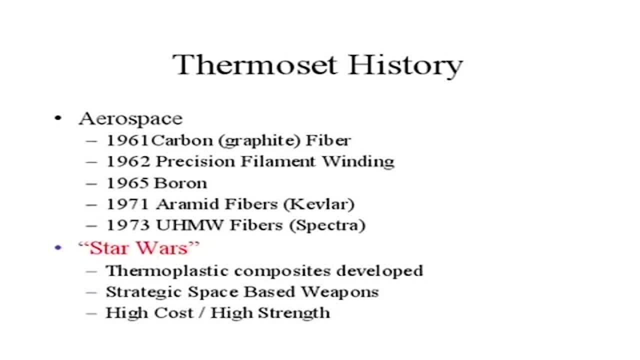 more along our aerospace development. our carbon was developed in 1961.. Precision filament winding: 1962.. Boron as a fiber. 65.. Kevlar, which is an aramid fiber, 1971.. Spectra, which is an ultra high molecular weight. 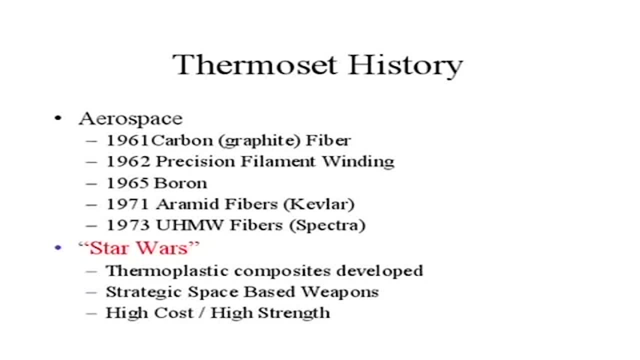 polyethylene fiber 1973.. And, of course, in the early 80s, when Ronald Reagan put all the money into our defense department to try to drive the evil empire out of existence, came up with Star Wars or a space defense initiative. That's when thermoplastic composites were developed. 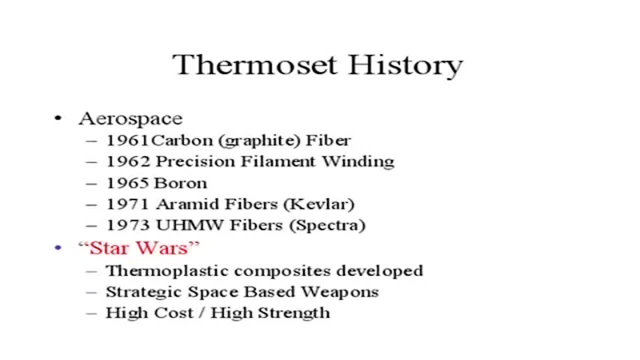 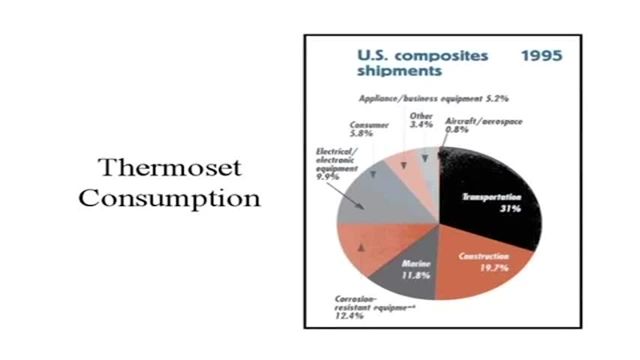 So they've been the newest part of our composite development. as we look at the history of composites In terms of utilization, again there's very specific areas where there's high use: Transportation, maritime use, construction- all high end uses of composites. 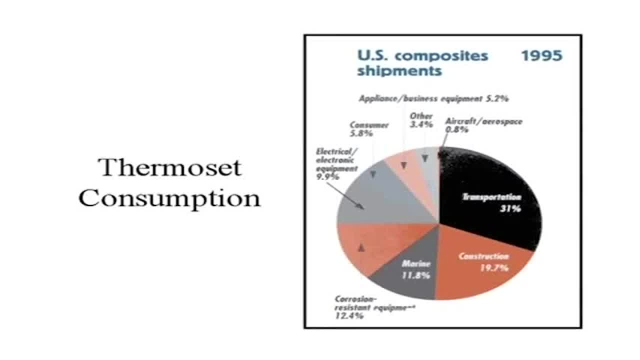 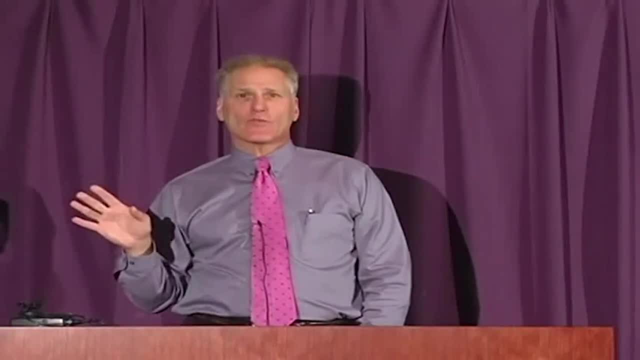 As you can see, we don't even- we're not even- a blip on that usage because we're such a small field. I particularly watch the marine industry because they're about the same size as the orthotics and prosthetics business in the United States. About 22 to 2300 boat builders in the United States. On average they have about 25 employees, never more than about 75, but they use 11% of all composites here in the United States. So to see how they're regulated. 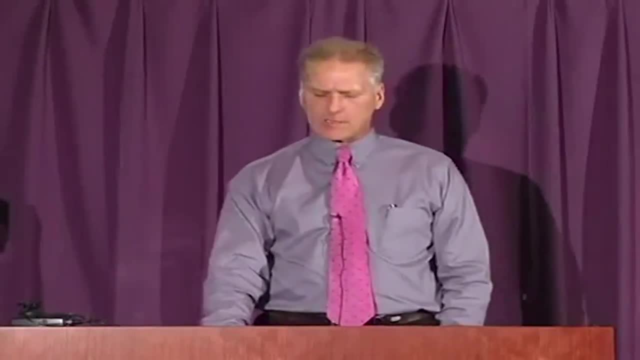 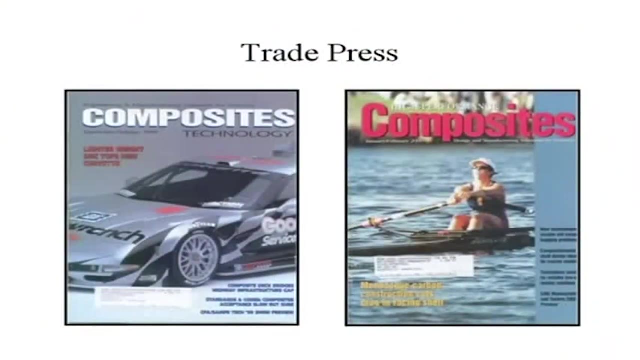 is very interesting in terms of how they conduct their composite manufacturing. There's trade magazines, just like in our field for composites, As you can see, composites technology, high performance composites- Usually these come across my desk every month and there's always some article in there. 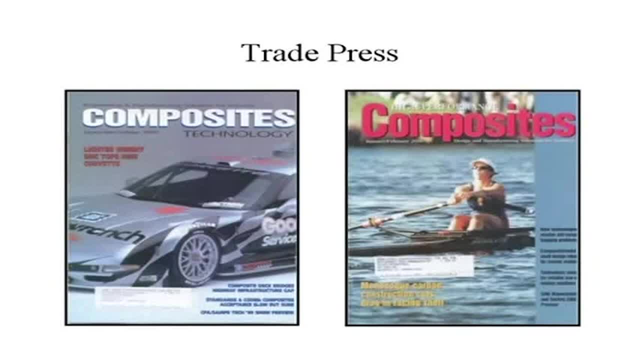 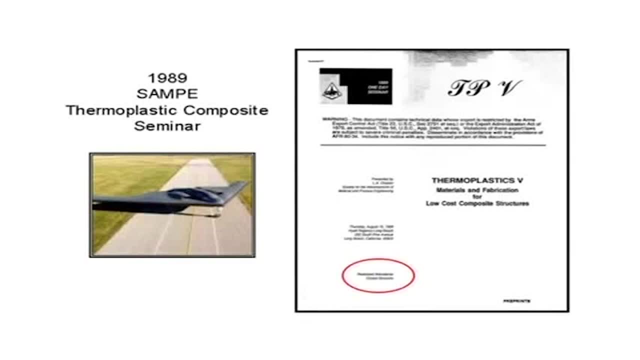 that I find interesting. that I find has some relationship to what we do For myself. my education in thermoplastic composites started in the late 80s when I was manufacturing knee braces. I was the charter vice president of Townsend Design, So I was investigating thermoplastic composites. 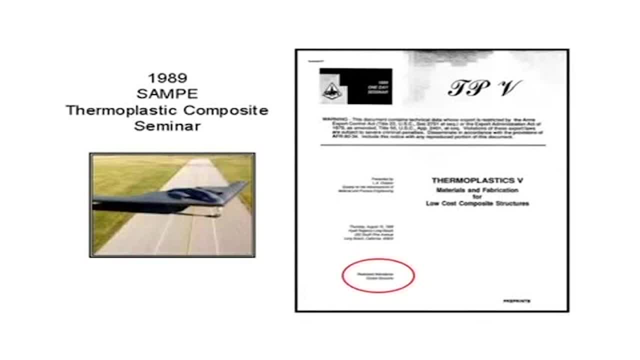 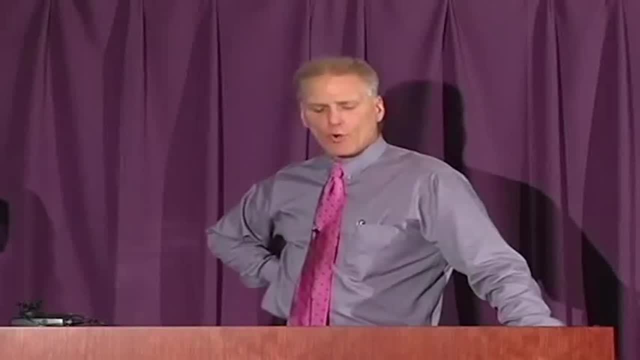 as being an alternative means of making knee bracing. So I attended this program back in 1989.. It was a thermoplastic composites seminars on supposedly low cost thermoplastic composites. That was somewhat of a misnomer because this was all geared 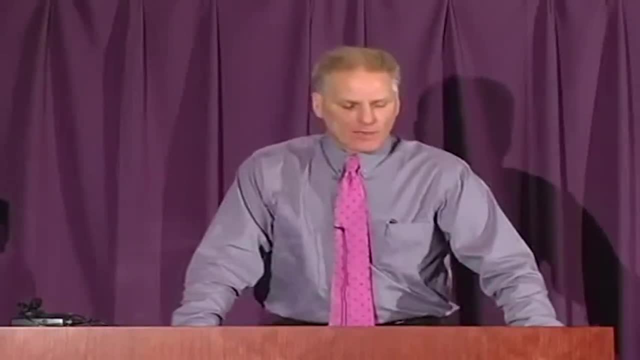 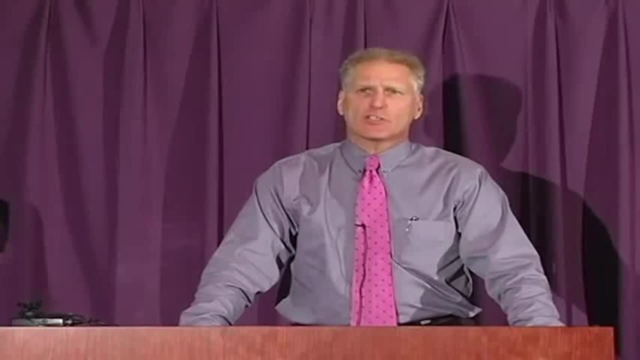 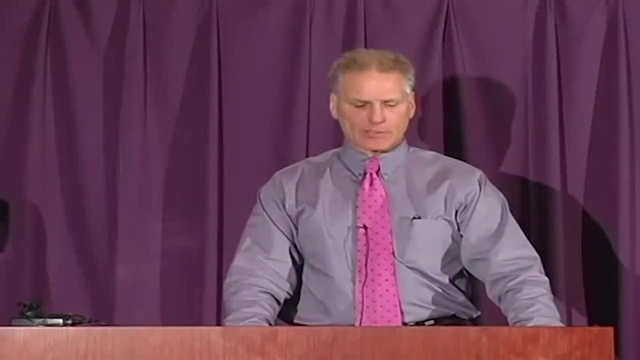 for the Department of Defense, because this was in the era when all the B-1 bomber and the stealth fighters were all basically starting their engineering cycle. So everybody at this conference was from the defense industry. There was certainly nobody from O&P at that point in time. 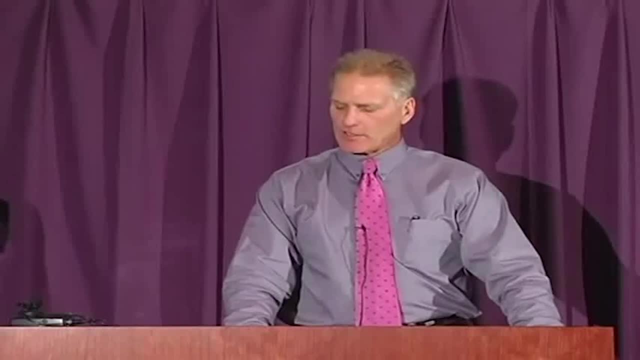 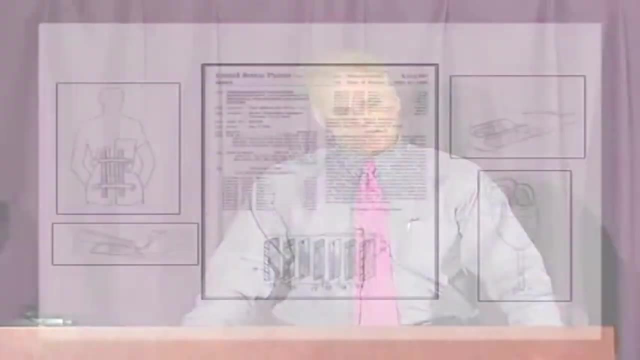 But it was the start of my educational process on thermoplastic composites- and I still deal with some people that I dealt with back then up to this point in time- And it did allow me to actually have a patent awarded for this application of this polypropylene based. 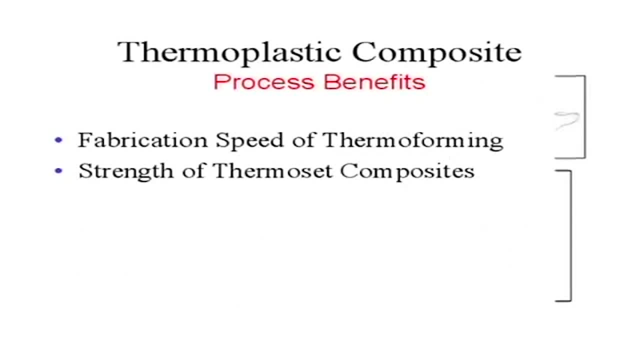 thermoplastic composite- prepreg composite. Now the process benefits of a thermoplastic composite versus a thermoset is we keep the fabrication speed of thermoforming because we're heating the resin and letting it cool because they're thermoplastic resins. 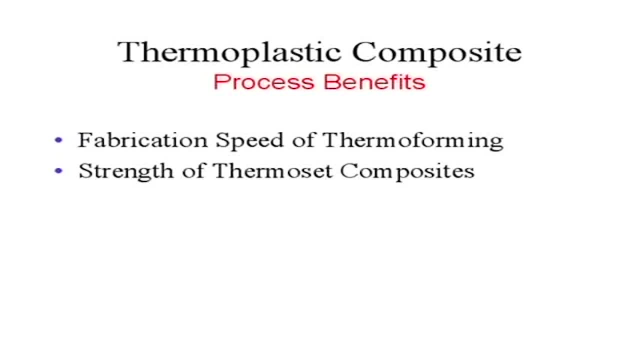 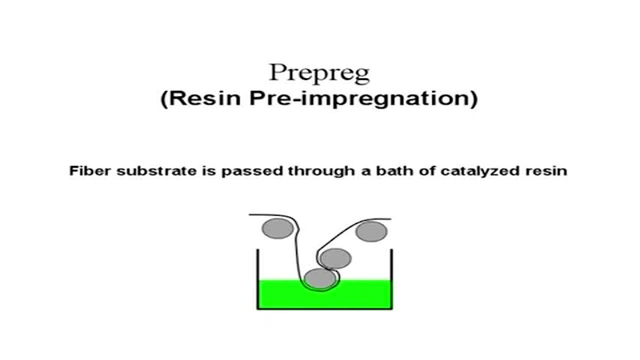 and we attain the strength of a thermoset composite. So speed and strength are the two factors. Now a prepreg for those of you who have never run across that term before. it really means pre-impregnation. We take the fibers. 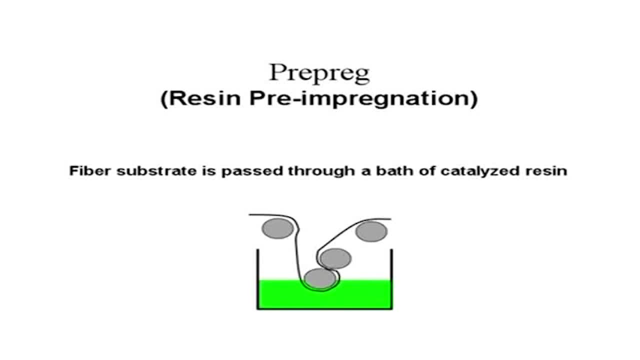 our reinforcement fibers and bring them through a bath of resin in order to coat the fibers with whatever resin choice we have. Prepregs, as you know, can occur both on the thermoset side and on the thermoplastic side, On one side. 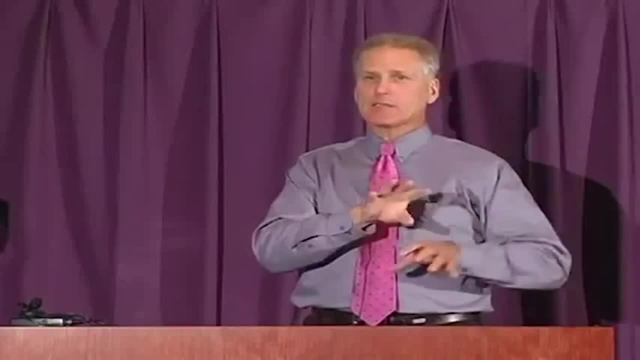 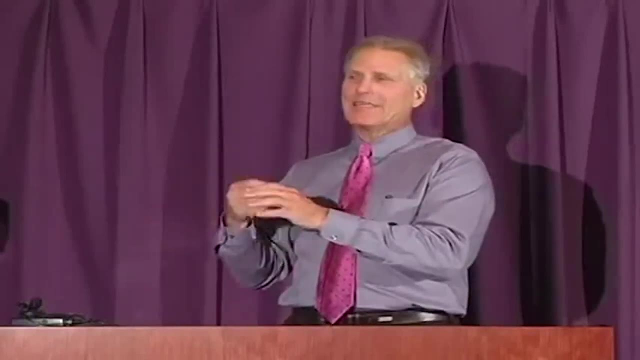 the resin is polymerized by mixing your catalyst and your resin. thermoset side, Thermoplastic side. there's various means of heating the material or introducing the thermoplastics to the fiber itself And I won't go into that. but there's some proprietary. 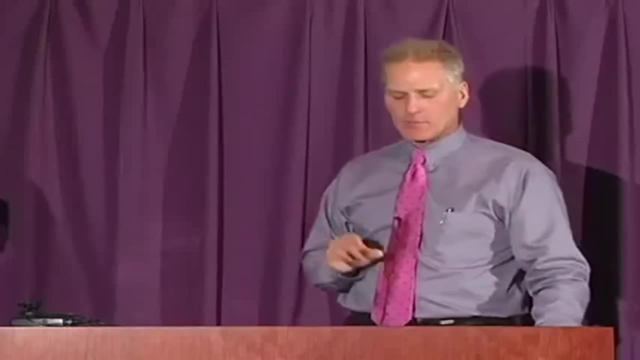 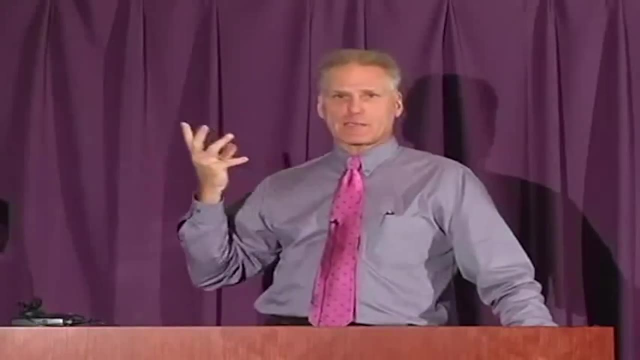 means of doing it. Some use dust, some heat it. There's different mechanisms that are kind of complicated, because at room temperature it's all solid, So they have to find a way that they can coat the fibers with the thermoplastic and make it flexible enough. 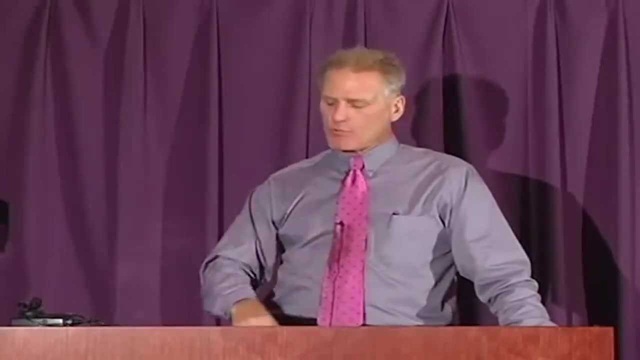 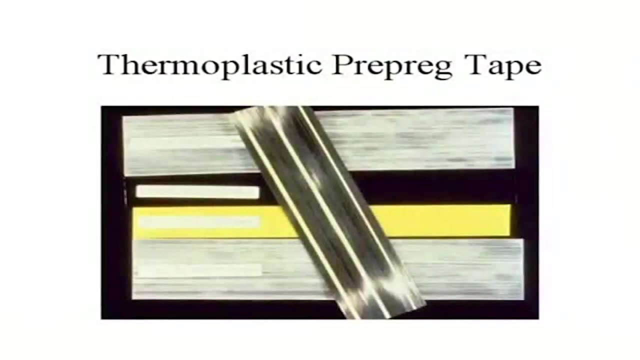 or in a usable form that we can then post-mold with heat and pressure into a composite shape. So prepreg pre-impregnation. In CompCore we use a prepreg tape. In other words, this is a tape of. 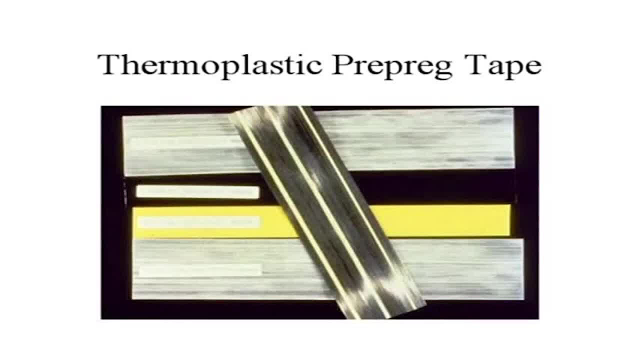 here you have examples of a fiberglass, carbon fiber, Kevlar, and then a combination of such That are coated with polypropylene, And these tapes are pre-made, pre-coated with the polypropylene tapes of these various materials. 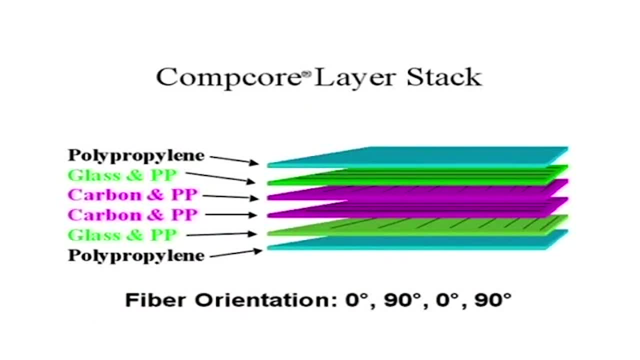 And then we take them and we put them into a stack, So it's glass and polypropylene, carbon and polypropylene, and then of course just polypropylene on the top and the bottom as a surface layer. That is all then consolidated. 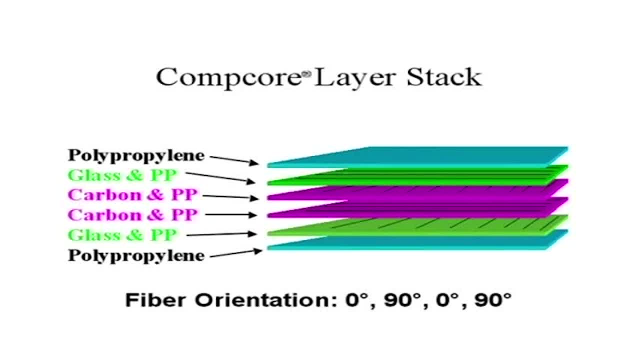 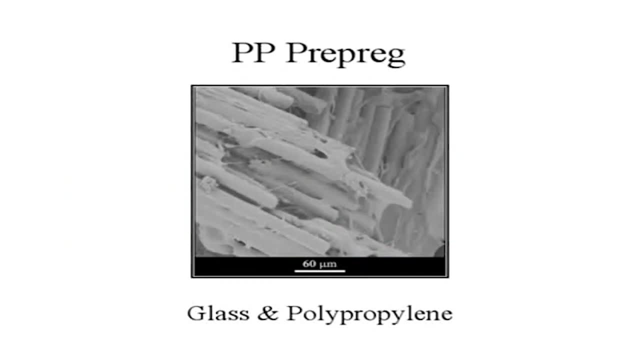 under heat and pressure. so you have a consolidated structure with your fibers running at zero and 90 in the layer. And, of course, if you looked at this through an electron microscope, you would see the polypropylene completely covering the glass fibers. So it all becomes. 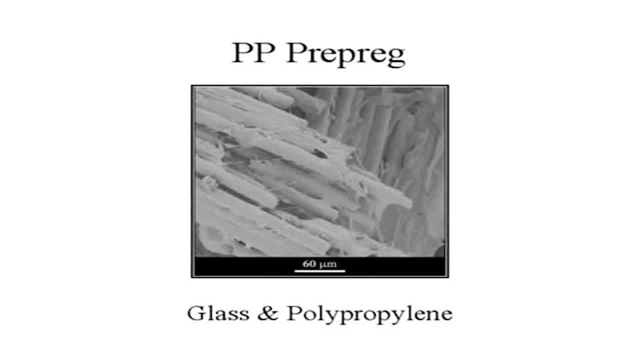 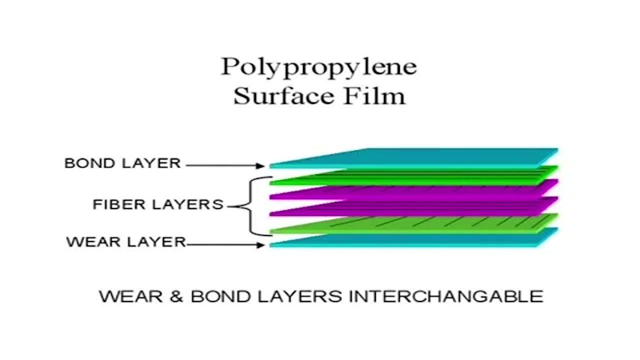 much like a composite, as if it was a thermoset composite, but it's thermoplastic. The top layers are flooded, And what I mean by that is that the tape layers have an optimal ratio of resin to fiber, But that's a very dry type of ratio. 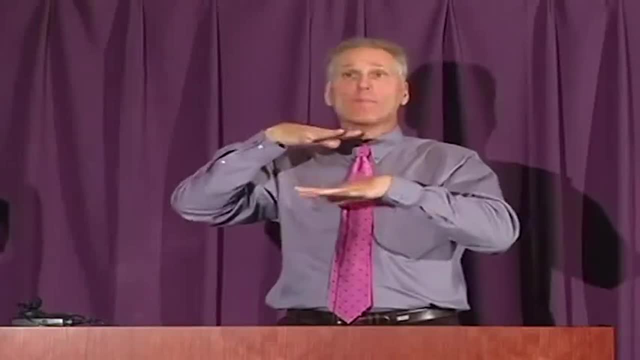 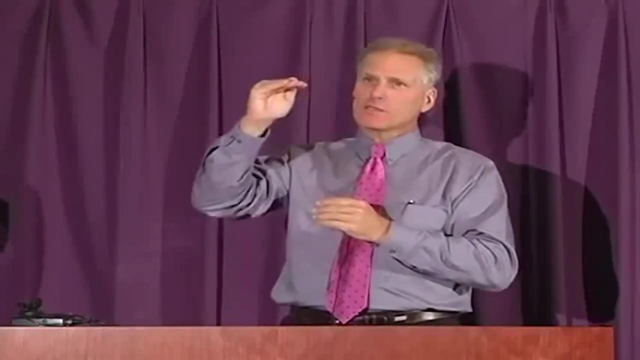 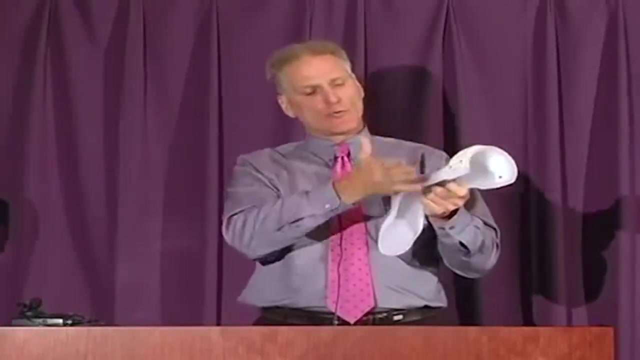 So my concern was having enough raw polypropylene on both surfaces to act for two different reasons. On one side you would have a layer on top of your composite, so when you wrap your polypropylene over it, there'd be a flood of polypropylene. 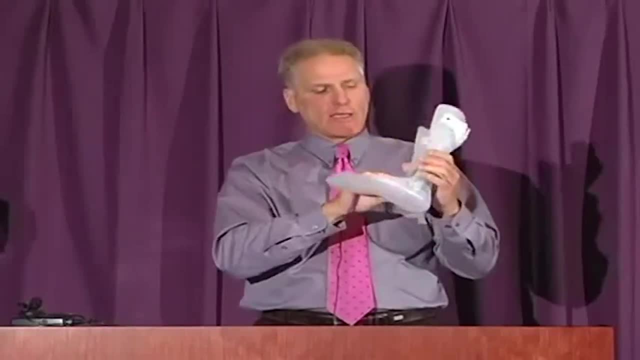 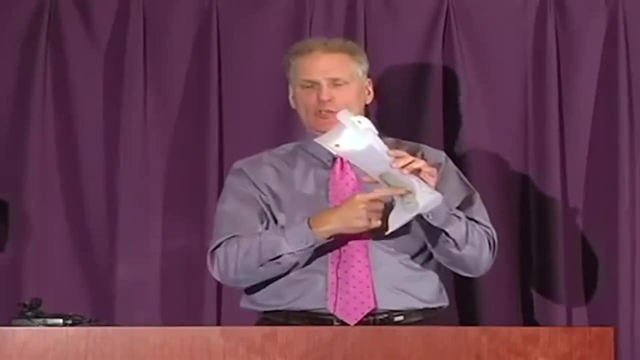 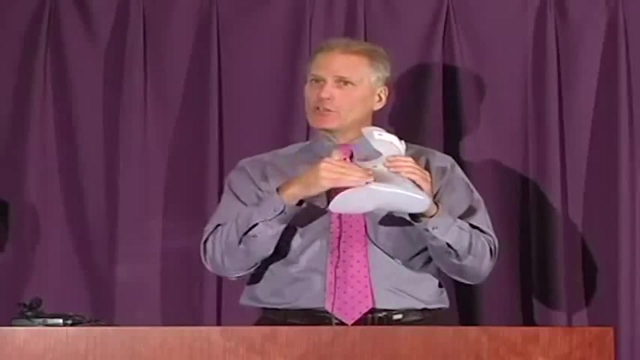 to act as a bonding layer between your host sheet and then your comp core reinforcement itself On the inside layer, where it would be exposed to the patient. I wanted that to be a flooded surface as well to act as a wear layer, So that way the patient 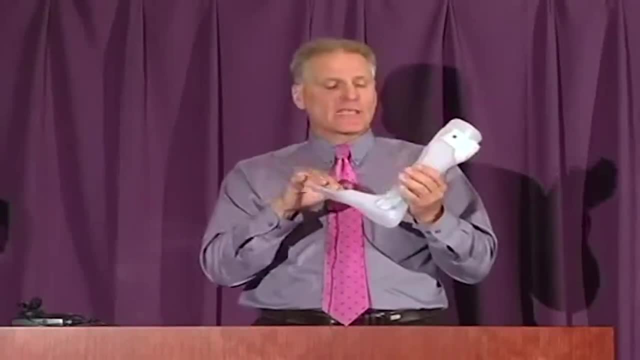 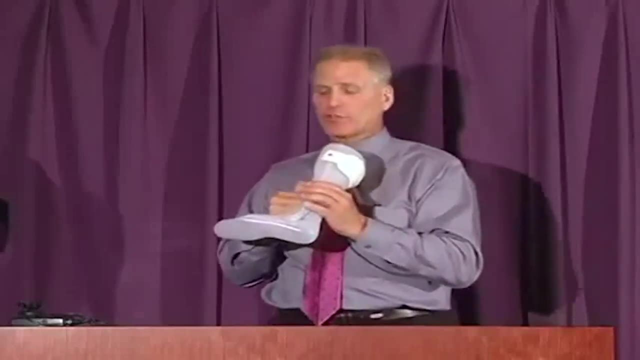 with a little bit of abrasive wear from socks or skin wouldn't be wearing right into the fibers itself. They would have to wear through a layer of polypropylene which, as you know, polypropylene is a little bit more durable than skin. 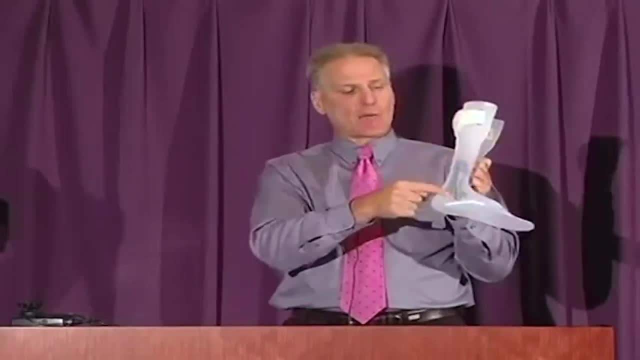 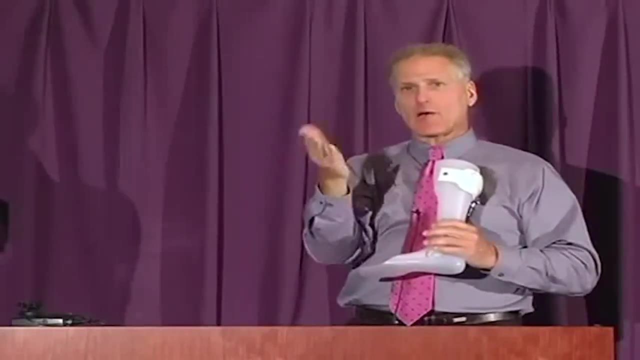 It's very rare that that ever occurs when you've got it completely encapsulated by polypropylene. It doesn't matter which way you lay up the material, basically it's just in name itself. One's a bond layer, one's a barrier layer. 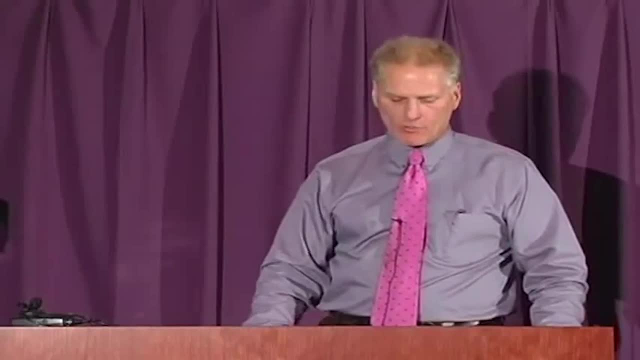 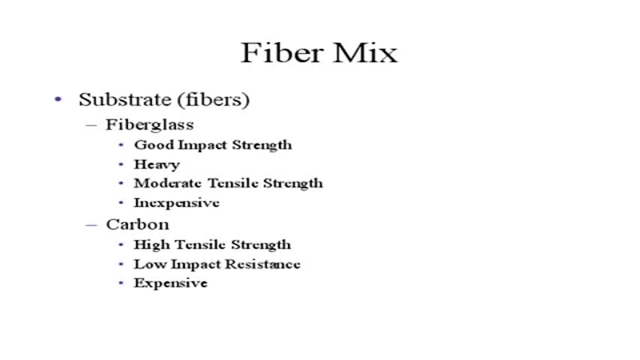 So it all depends how you just put it on your model. In terms of the fiber mix, I like to use both fiberglass and carbon. It's a great mix. Everybody thinks carbon is sexy and absolutely it is. It's the Elvis Presley of fibers. 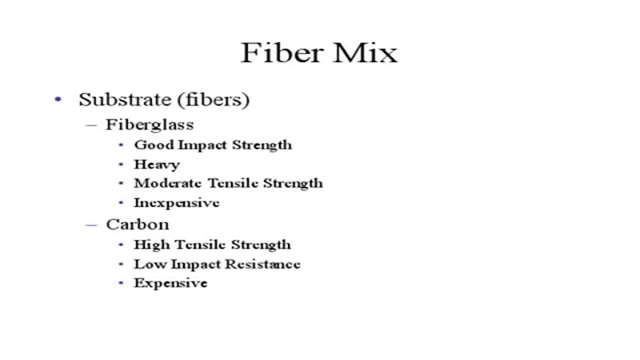 Everybody thinks it's cool because it has such high tensile strength, but, on the other side, expensive, as you know, and has a tendency of having catastrophic failure. Glass, on the other hand, it's the Barry Manilow of composites. 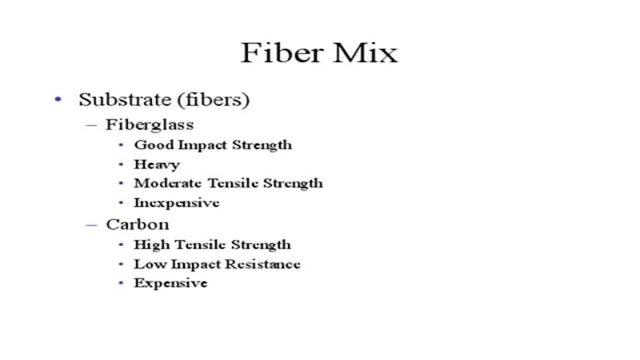 It's basically been around. It's inexpensive, It's somewhat heavy, It only has moderate tensile strength, but it has exceedingly good impact strength. So consequently, if you put a mix of both fibers in your prepreg composite, it can basically have. 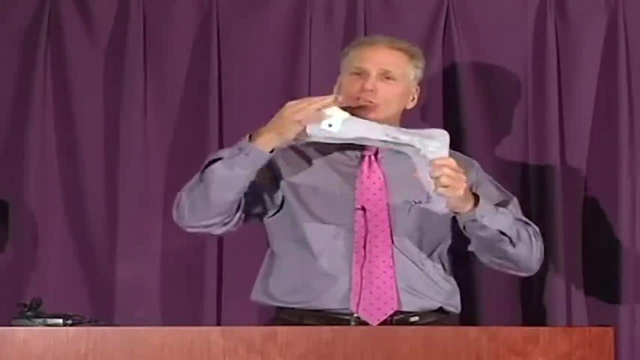 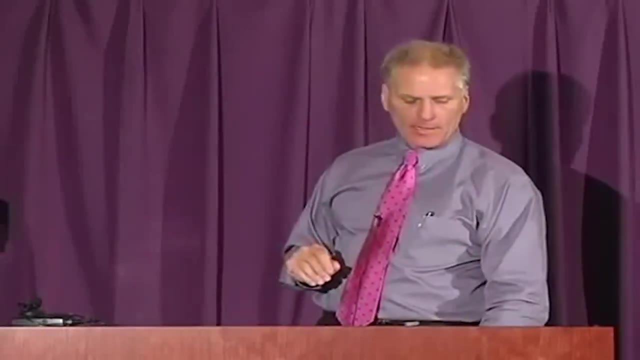 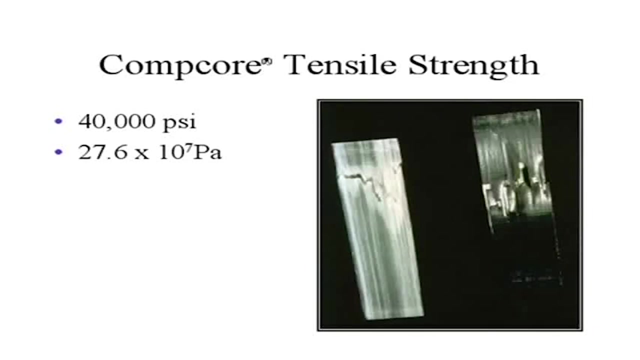 real, good impact, strength and yet good structure. So it's a great combination of fibers within any type of composite layer. In terms of strength, Comcor, from a tensile standpoint, is at 40,000 PSI. In terms of the bond interface, 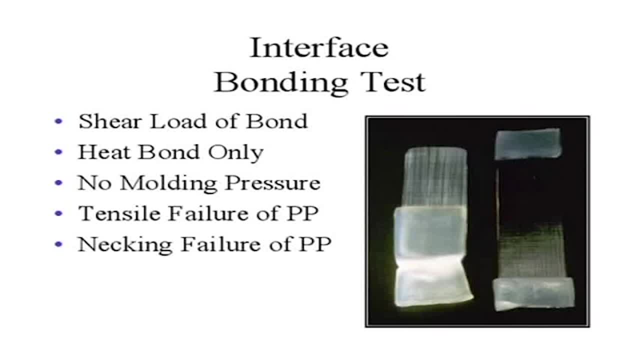 where the polypropylene bonds to the polypropylene. it is as strong as the polypropylene because it's just bringing two polypropylene materials or resin surfaces together and bonding them together. So it's exceedingly strong. So it's exceedingly strong. 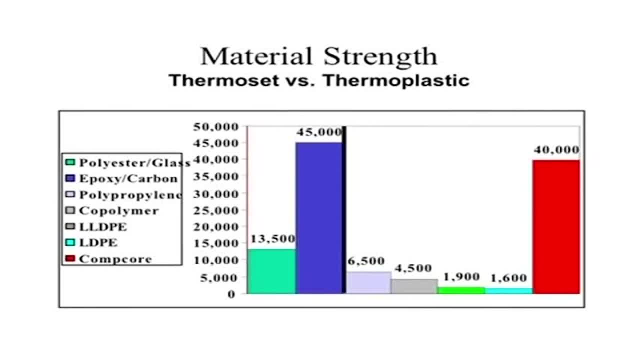 Going back to that very similar chart we looked at earlier, to the right of the black line: polypropylene, copolymer, linear, low density. low density polyethylene, very weak Carbon fiber and epoxy. Here's Comcor, which is polypropylene. 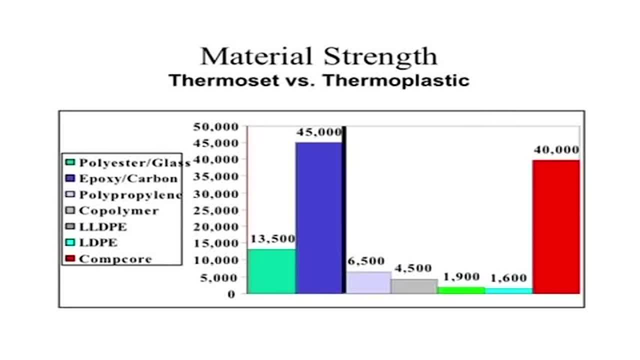 carbon fiber. You can see, by mixing a piece of carbon fiber into your polypropylene, it's going to bridge this huge gap that exists between your thermoset epoxy and carbon fiber layup compared to just your straight polypropylene. 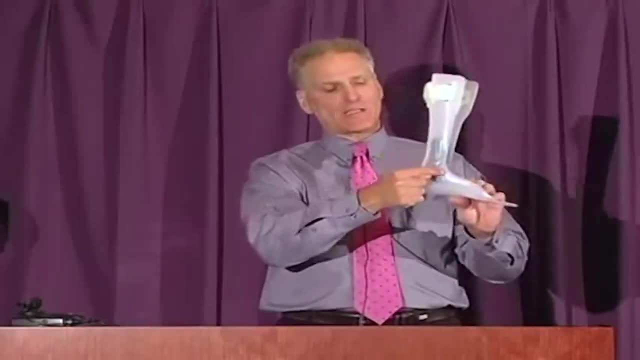 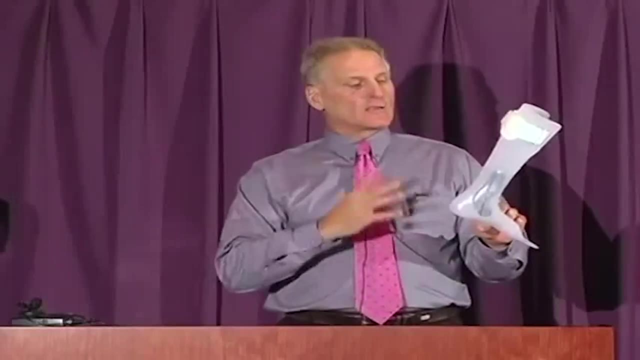 So that's why we looked at it as being a means of selectively reinforcing thermoplastic devices with this polypropylene prepreg. Tom Lunsford, who's retired now, but at one point in time was president of our academy. He was also. 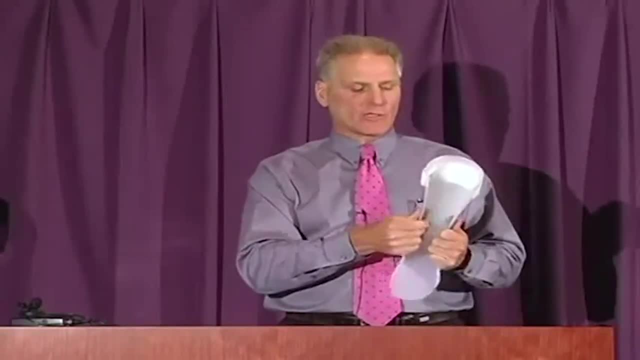 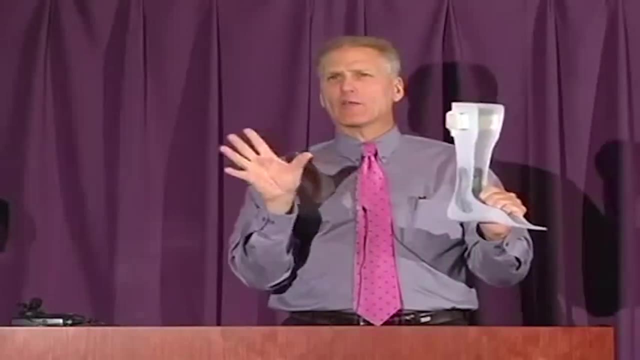 the research director at Rancho Los Amigos in the OMP department. there I made a series of AFOs that were reinforced and unreinforced. Tom had a great AFO testing machine that would test the sagittal plane stiffness of an AFO. 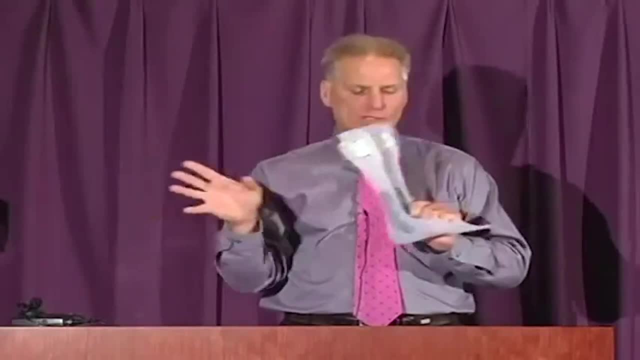 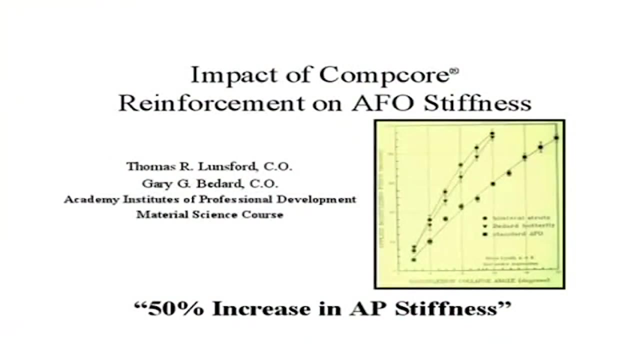 When he basically put my AFOs into his machine, did his testing, we found out that we improved the AP stiffness of a solid ankle AFO by 50%. So that's a considerable margin of increase in stiffness just by including a little. basically. 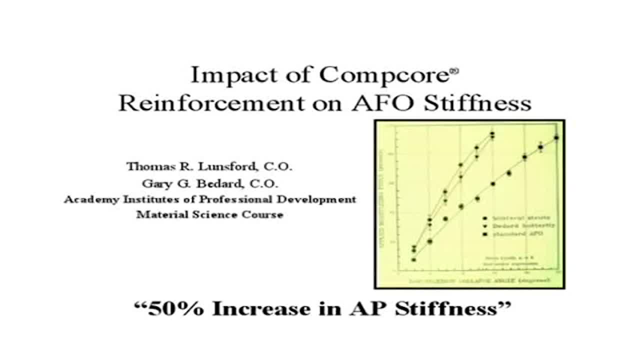 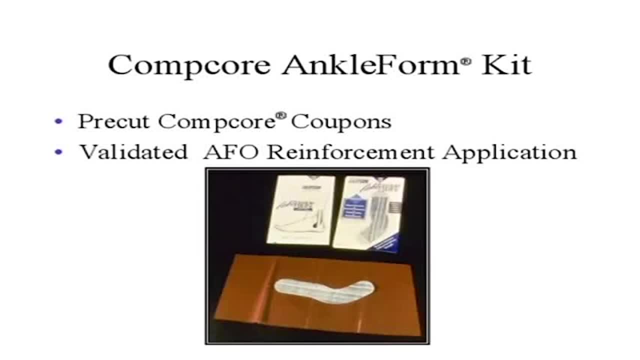 coupon of material. So once we did that initial testing, I took that information back to Becker Orthopedic. We then elected to make a kit for a specific size reinforcement coupon that you could vacuum form directly into your model. We cut these on a water jet. 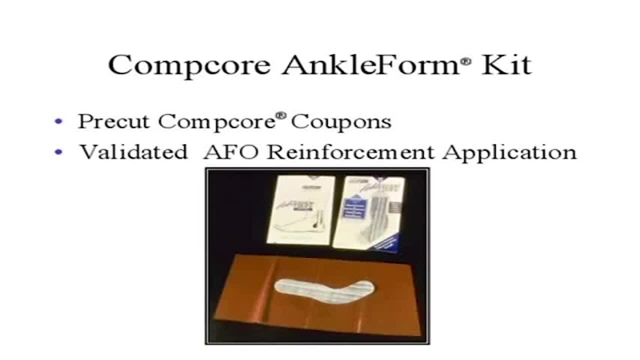 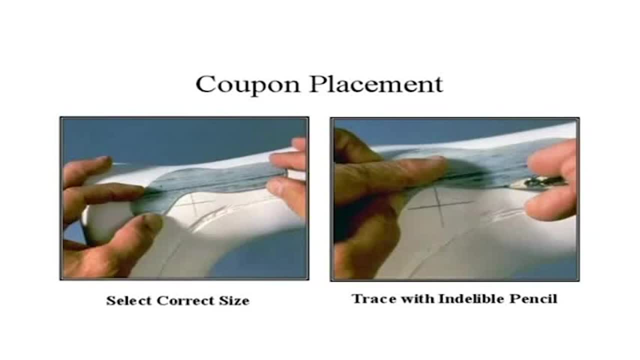 They're a validated shape. It comes in a kit that you come in several different sizes. The way that you apply this in your manufacturing process, in your lab, is to take that coupon, draw the outline on your positive model, then cover that model with a, of course. 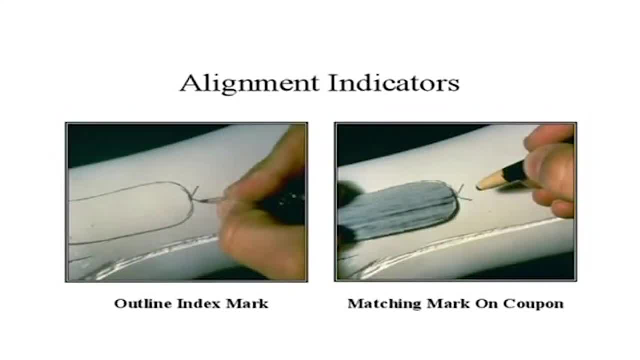 your evacuation layer. make some indexing marks for aiming for proper alignment, because it has to be all done within that 25 seconds of thermoforming. Make sure you have a clean environment. Clean your surfaces of your materials because of that blooming effect. 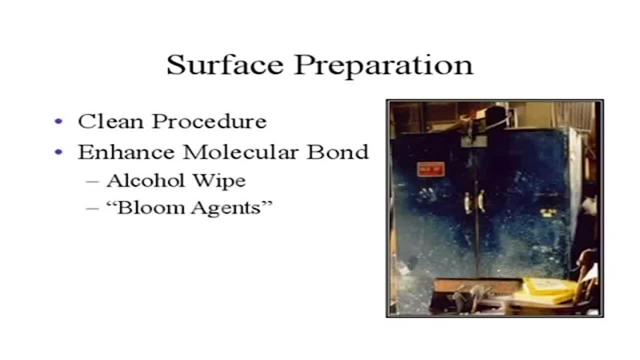 that we already talked about Those agents that might come to the surface, that might interrupt with the bonding of the one poly hot polypropylene surface coming to another hot polypropylene surface. It comes with a piece of Teflon film that you lay in your oven. 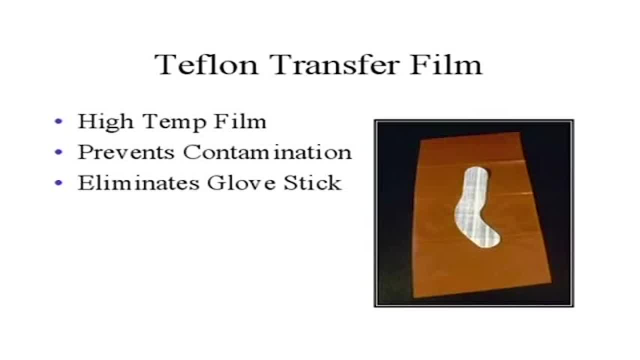 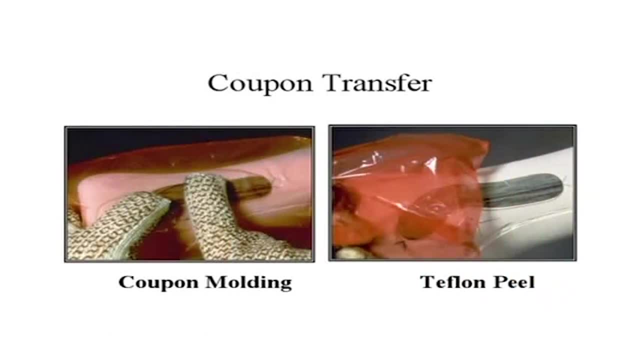 that keeps that piece of prepreg polypropylene from sticking to the oven tray. You can pick it up with your gloves. Once you pick it up with your gloves, use that Teflon film to mold it onto the evacuation layer of your AFO. 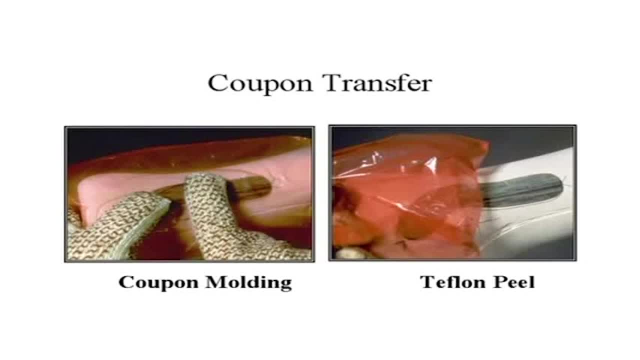 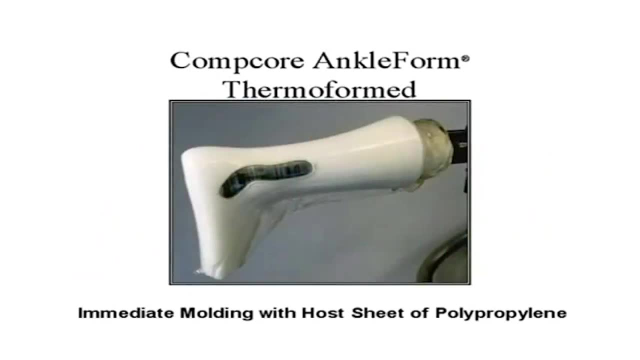 Sometimes I might put a little 77-3M spray on there to hold the composite in place and then immediately vacu-form with your hot polypropylene. It all has to be hot because polypropylene when it's at melt temperature. 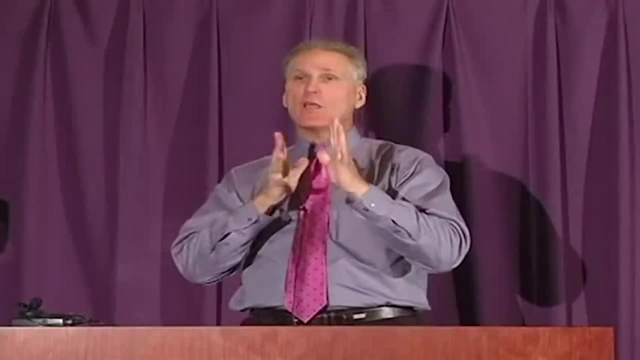 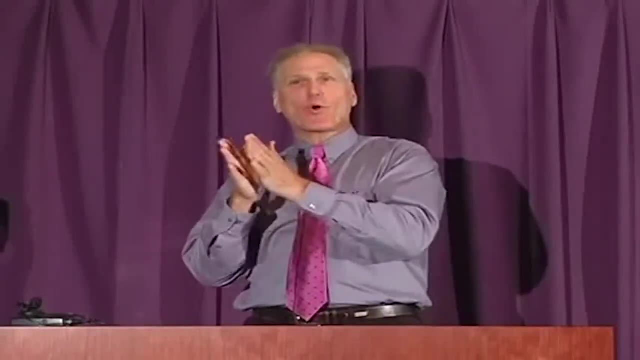 it's going to be hot, and it's going to be hot when it's at melt temperature and comes in contact with each other, as you know, will bond to itself. So by using a polypropylene prepreg at melt temperature. 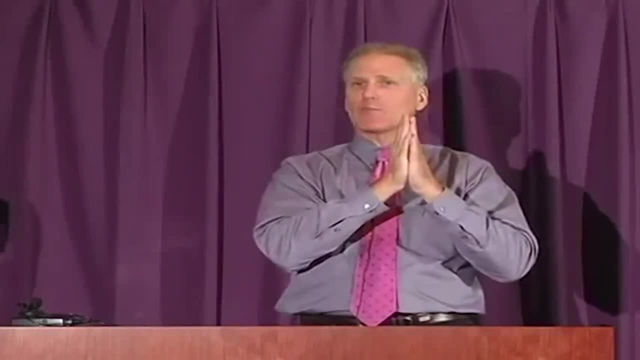 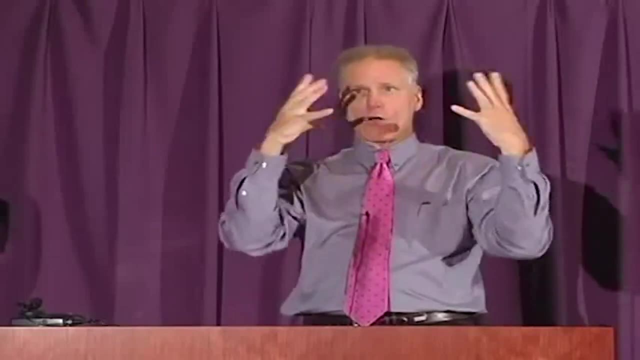 matched up against the whole sheet of polypropylene at melt temperature that you're using to form your clinical device, it basically all becomes integrated. It all basically ties in together through those Van default's force without using any kind of adhesive. It's all chemical bonding. 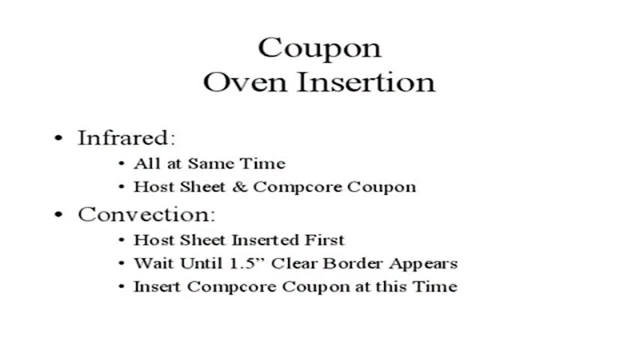 at that point in time, Coupons in the oven, If you else would like. If it's an infrared oven, I put everything in at the same time. If you're still using a convection oven, I put the whole sheet of polypropylene in first. 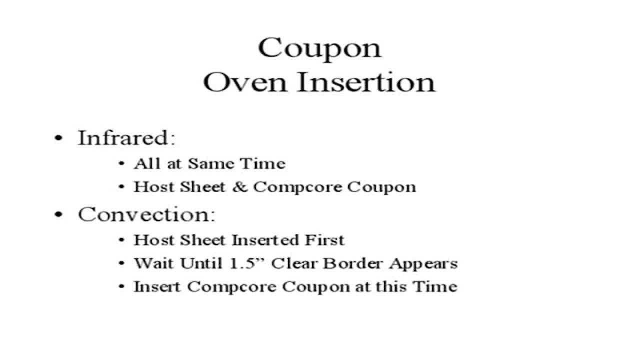 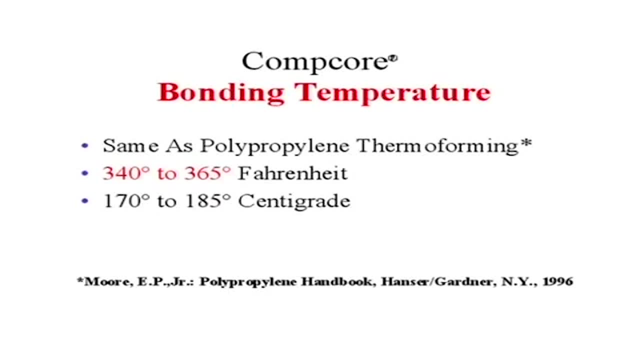 weight to the edges, have about an inch of clarity all the way around. then I stick in my prepreg coupons at that point in time. That way there I don't overheat my prepreg coupons. It all bonds at the same temperature of polypropylene, because it all is polypropylene. 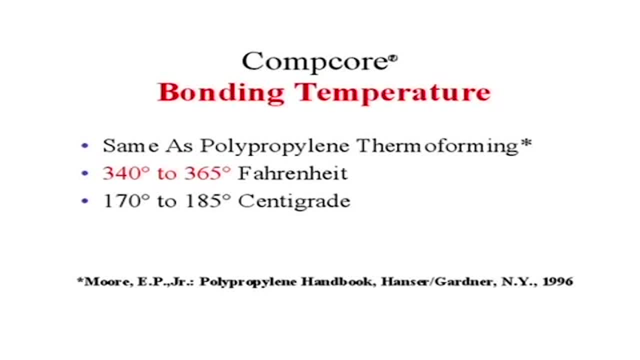 We've just introduced some carbon fiber and glass fibers into the polypropylene to make that prepreg coupon Kind of simple in concept. but when we first did the engineering nobody was doing this stuff. That's why we got a patent on it. 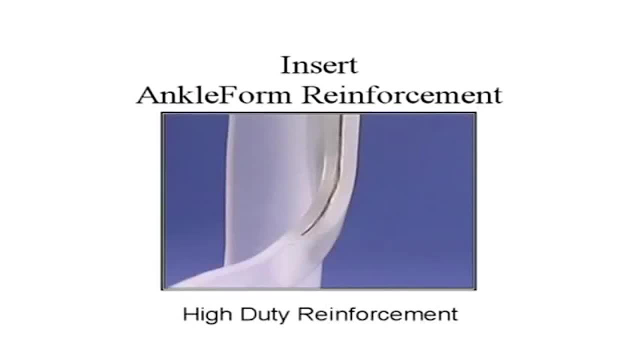 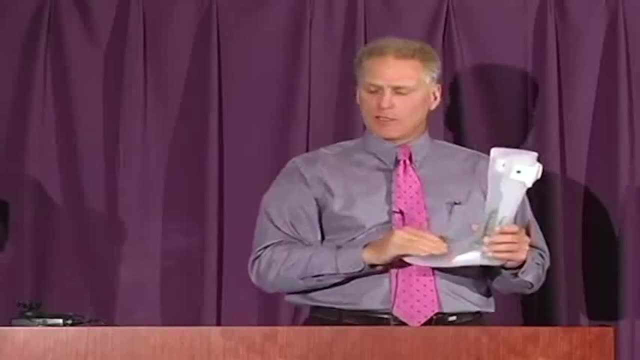 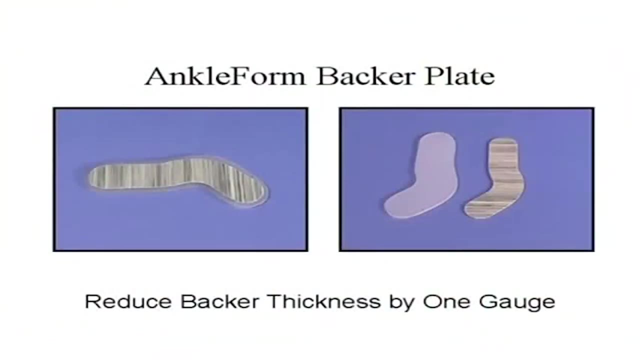 How do you reinforce large patients? I like to do an insert bonding. In other words, instead of just having the Compcor laying on the inside of that polypropylene sheet, we'll make a stacked layer. By that what I'll mean is we'll take one of the coupons, cut a backer plate of polypropylene. 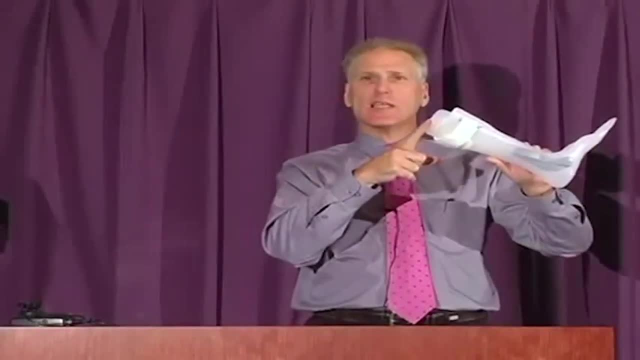 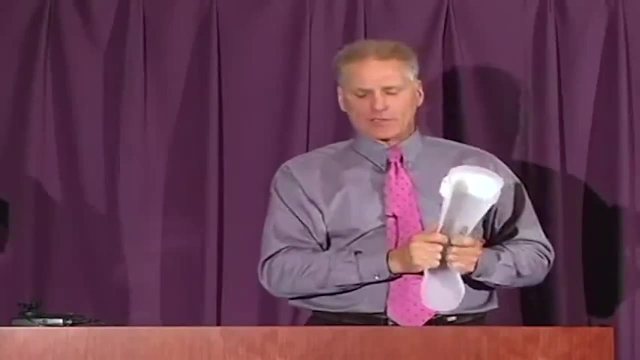 typically one gauge. If this is 3- 16ths, I'll use 1- 8th inch. If I'm using 1- 8th inch for my host material, I'll use 1- 16th inch. I always bring it down. one thickness down just keeps down on the bulk. 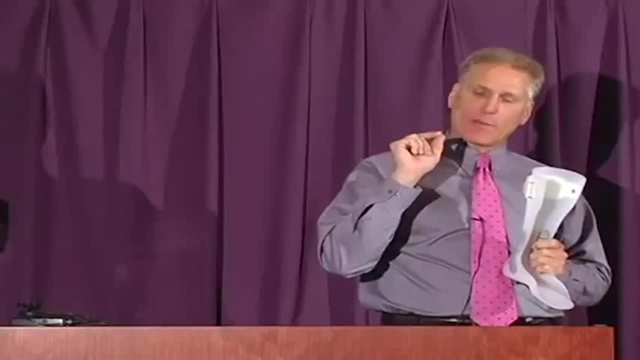 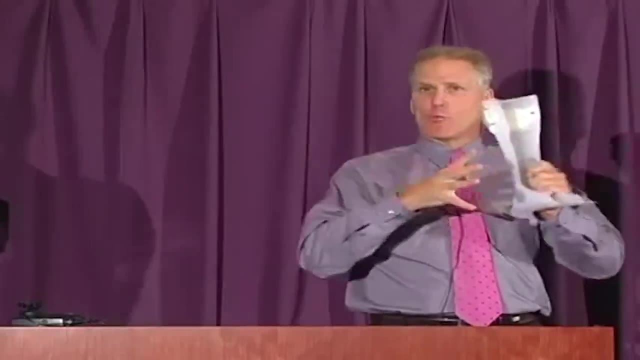 I will make that inner coupon of homo-polymer polypropylene about 25% bigger than the actual coupon of Compcor because, as you know, plastics at that temperature will change shape. You want to make sure it doesn't change shape and doesn't completely act as a component. 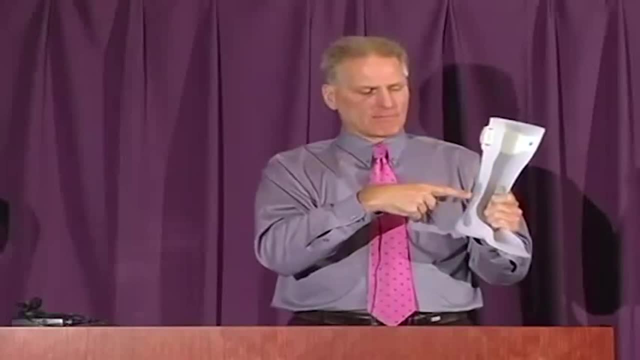 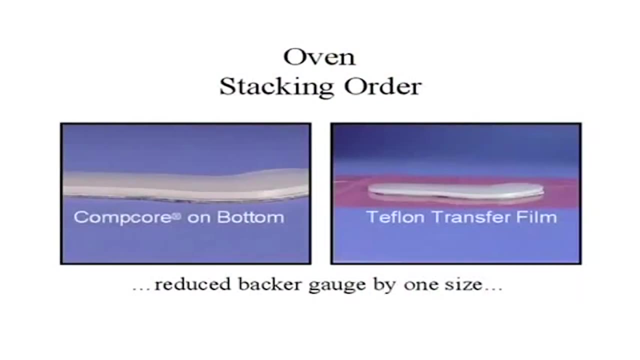 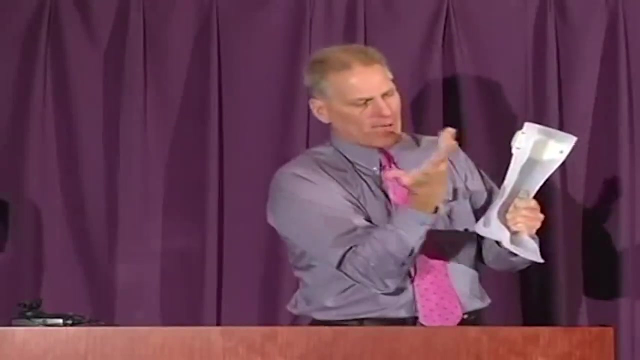 That's what I do. I make sure that it completely covers your prepreg coupon. All that's placed in the oven on a Teflon sheet. The composite is on the bottom. When you pick it up and then mold it against your positive model. the polypropylene is. 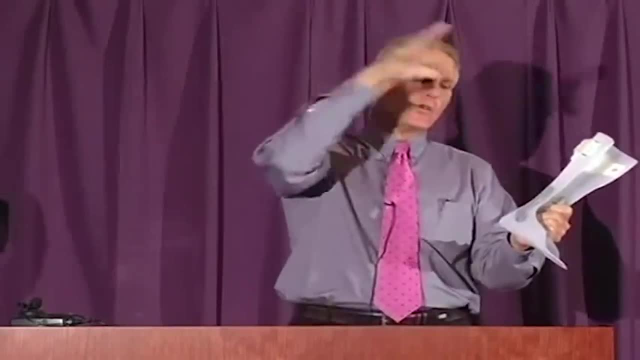 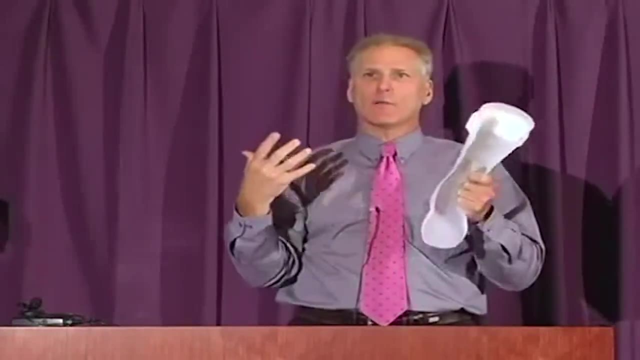 against the positive model. Then you have your Compcor, Then you overmold it with your host sheet of material. That way there the Compcor is sandwiched between two pieces of polypropylene. It makes a very, very big difference. 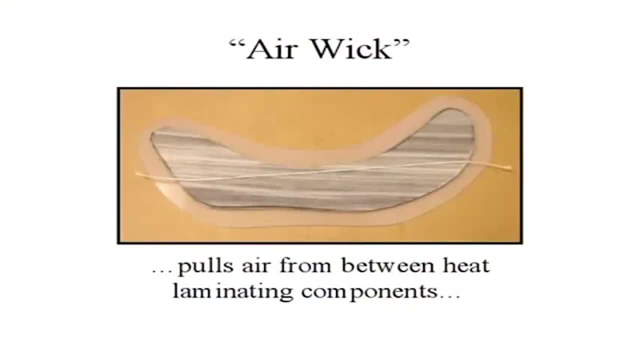 It's a very strong structure. We also use what I like to call an ear wick. This technique is used by many people in the field. A very light piece of cotton string run across that doubler. When you lay it up, the string act as an ear wick. 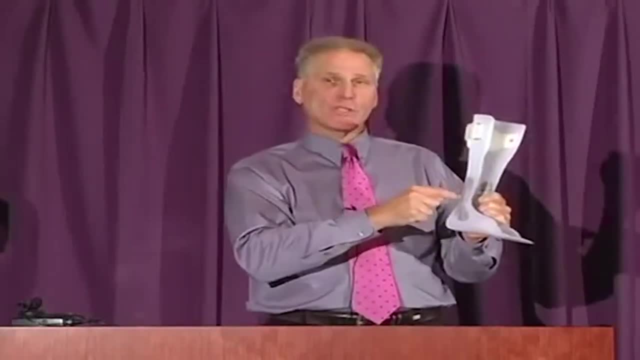 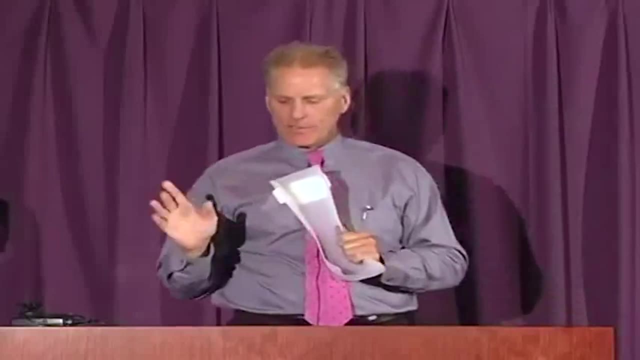 It will pull any ear that's trapped between those layers out of that encapsulation so that you have complete bonding between those two layers. You use an ear wick- Very simple techniques. We use it any time we want to do a doubler. 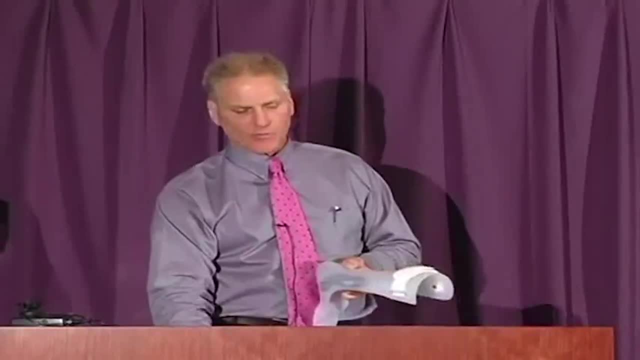 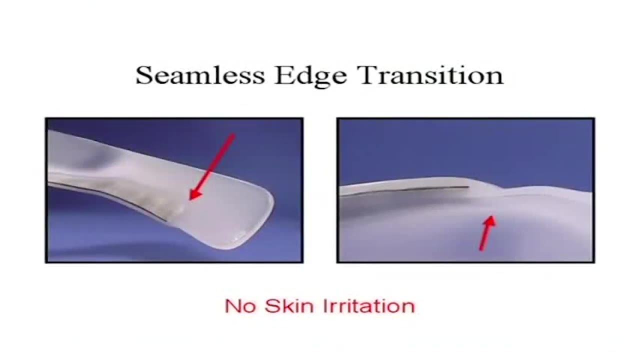 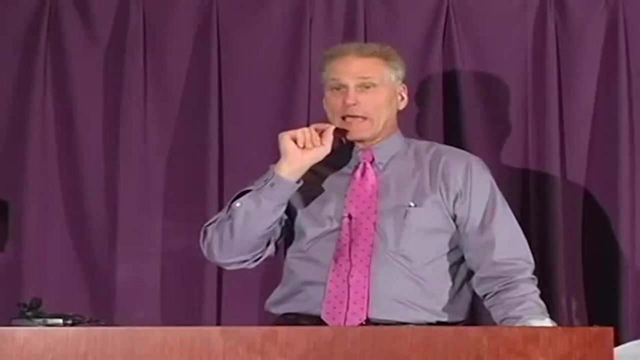 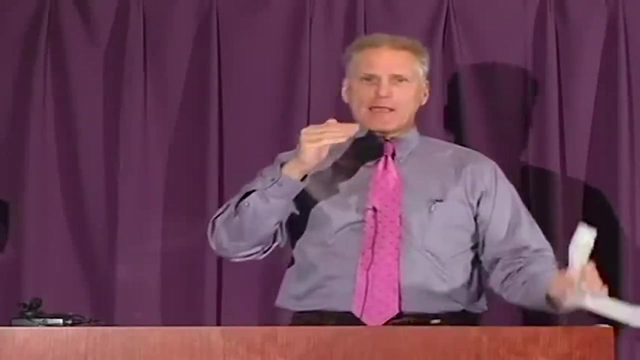 Even on small pieces, Even on small ankle blocks, making a range of motion stops for our AFOs. Here's a cutaway look in terms of having that layup on the inside. It's also a seamless transition If you control, have good process control and your temperature's at the right temperature. 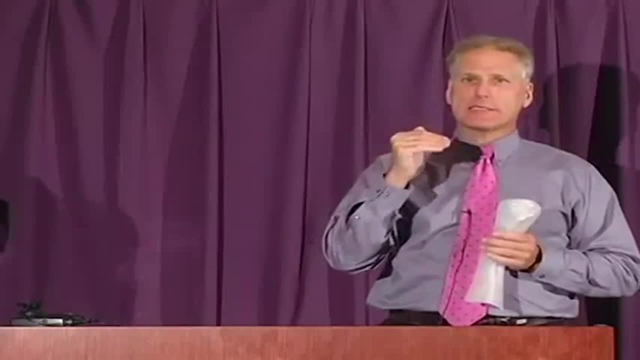 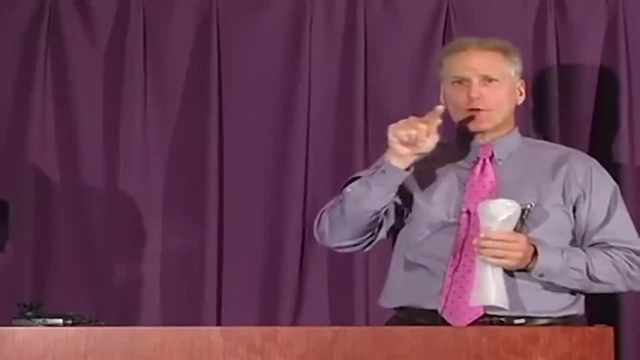 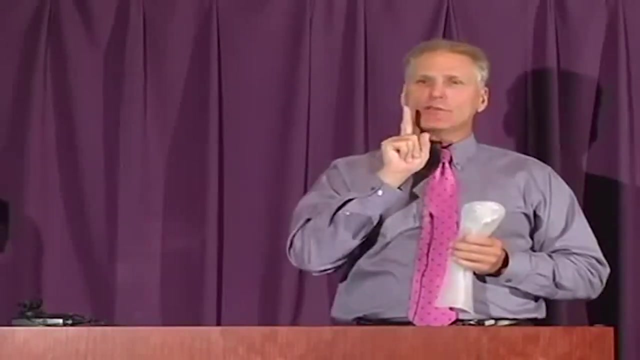 that bond line on the inside is completely seamless, Completely seamless. There should be no groove around that doubling at that point in time. If there's a groove around it, then you have a problem in your thermo forming process And that's a visual cue you can use whenever you do any thermo forming. 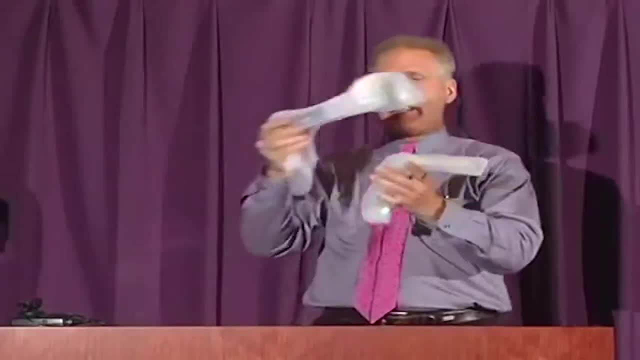 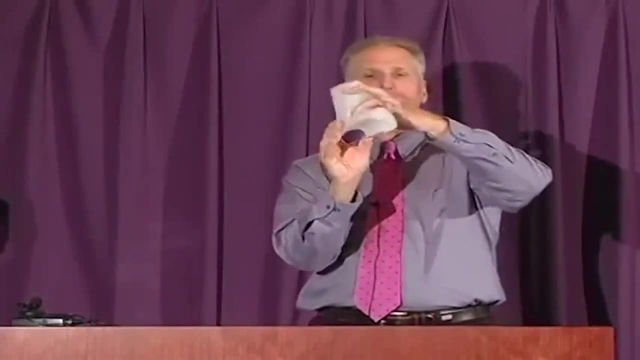 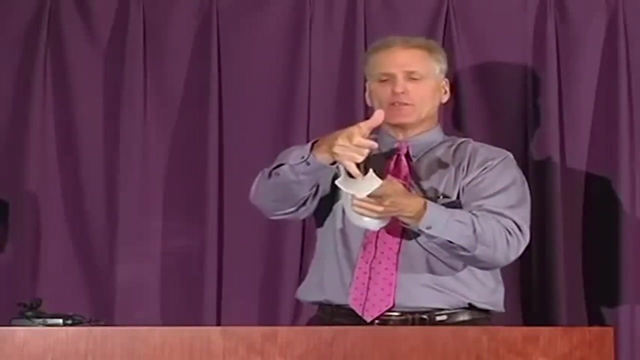 When you trim that piece of plastic out from any device and you pull it off and then you look on the inside of where this bond line comes together. Subtitles by the Amaraorg community. if there is a line on the inside, a groove, I should say if there's a groove. 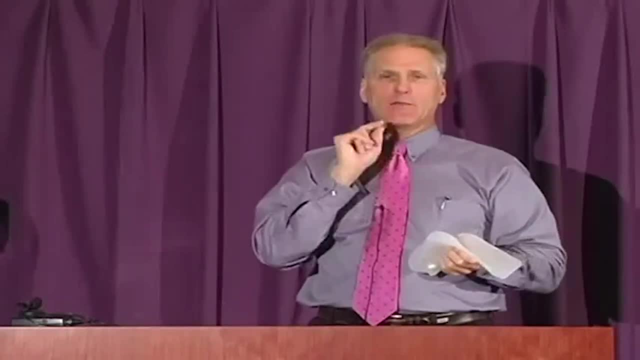 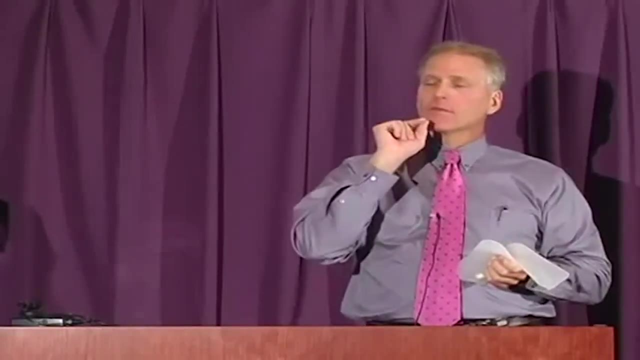 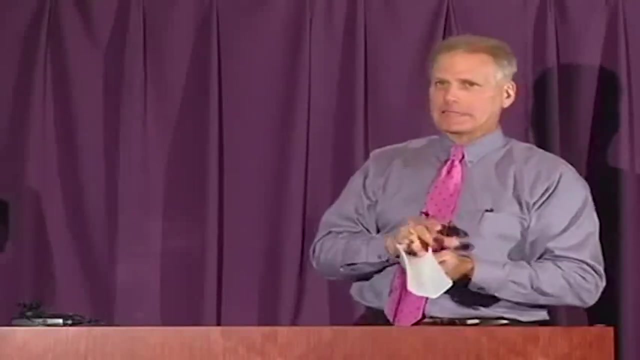 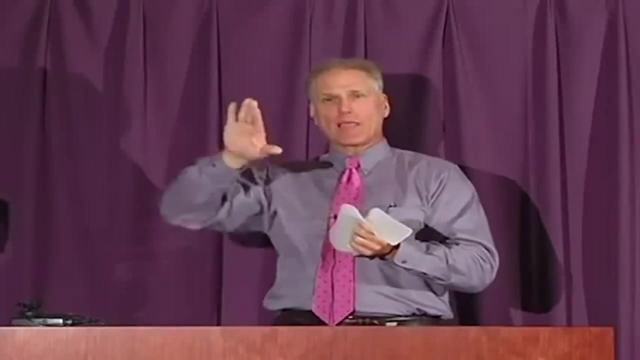 on the inside. that indicates to me that you are not controlling your temperature or your pressure and that you have an adequate process. if there's a groove on the inside, you've probably pulled that plastic at too low, or temperature or the onset of your vacuum forces are slow. slow that you get that reverse eggshell. 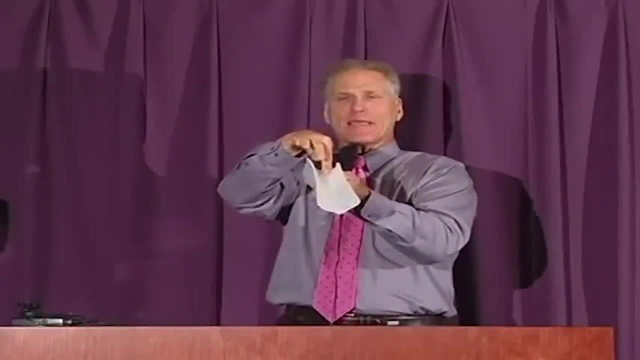 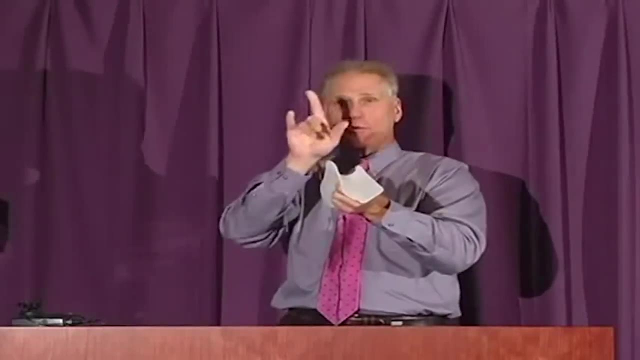 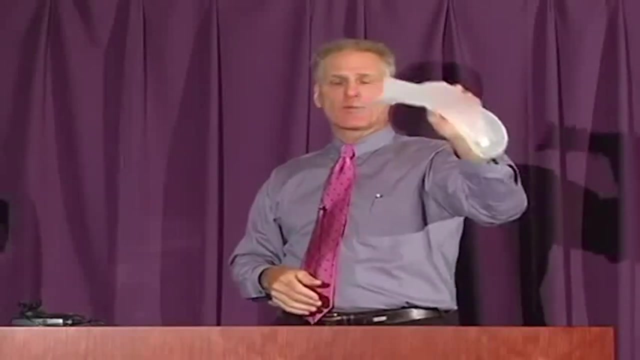 and it prevents the flow of your plastic so that you have a seamless bond line on the inside. there's no demarcation, it becomes completely smooth. right, good test. if there's a groove, you've got something wrong. anytime you trim off on an AFO, look on the inside. it's perfect test to see your staffers, your 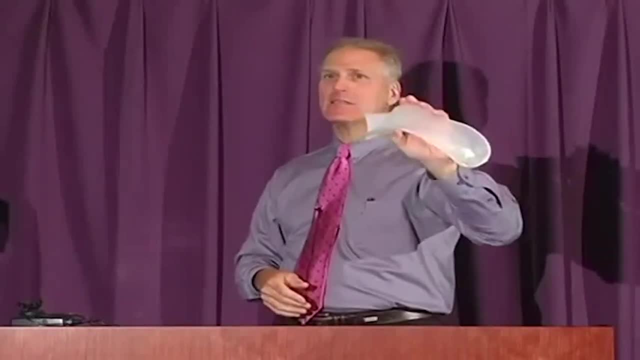 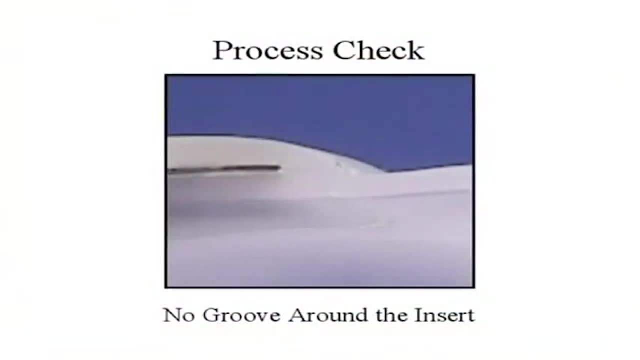 technicians if they're controlling the process. if they're getting lazy or they're trying to rush the process and there's a groove, they're doing something wrong. Visual cue: Anytime you make any product in your lab, you can use that visual cue. 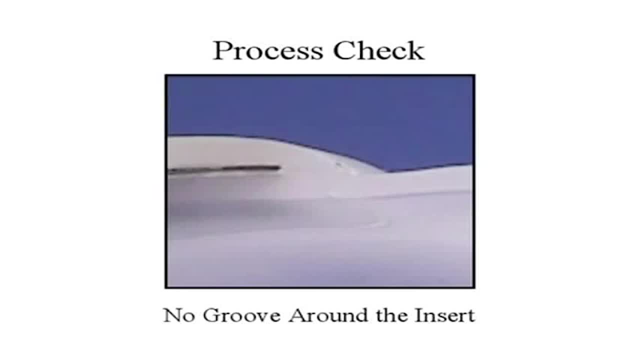 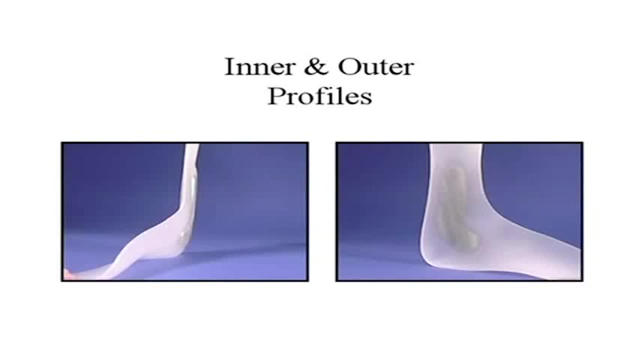 So there should be a seamless edge on the inside. That's a process check Here you can see it. this little groove- or there should be no groove here- That should be seamless where that overlap bond line comes together. So that was just a little close-up to show you that differential. 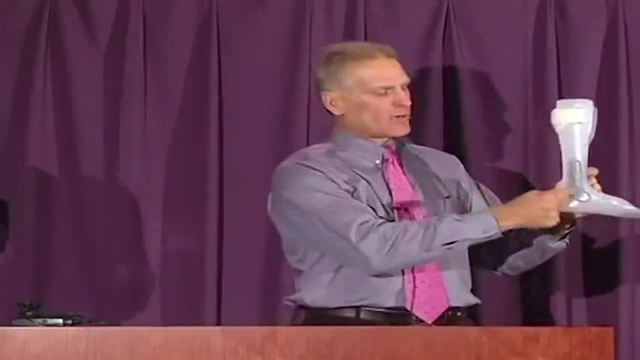 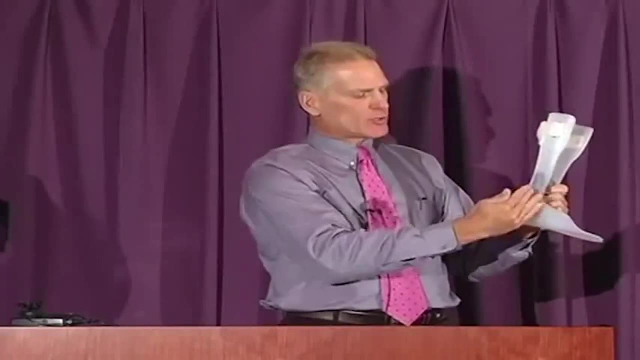 Now, in terms of the trim line, never cut into the composite. You want to isolate that from the patient, So you want to make sure, when you lay these up, that they're posterior to your anterior trim line so that you have a nice smooth edge. that's just homopolymer polypropylene. 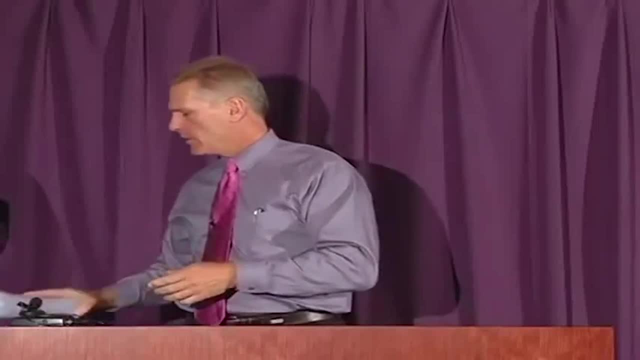 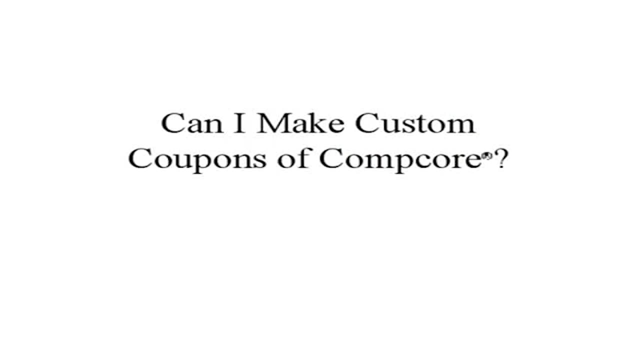 You do not want to expose that carbon fiber, if you can help it at all on the inside, just to make that smooth edge. How do you make a custom coupon? We sell pre-made ones. custom one: very easy: Draw the outline. indelible pencil. 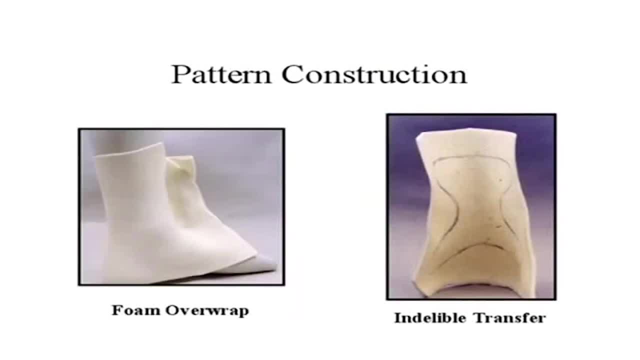 On a green cast, over-wrap it with a heated piece of Adliplast. that indelible outline transfers. You put it on your piece of stock Comcor, trace it out with a wax pencil. You want to flatten it out, obviously. 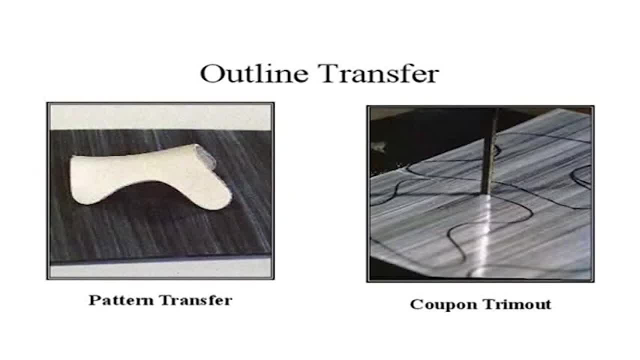 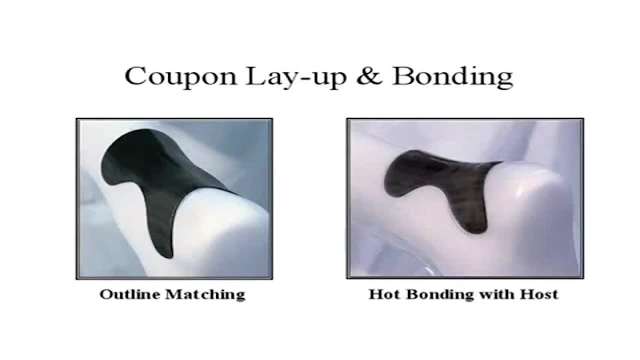 It's a three-dimensional pattern. at that point in time, Cut it out, put it in the oven, just smooth up the edges. They don't have to be tapered, They just have to be smoothed out. When you heat it, it will drop in exactly to whatever outline you have. 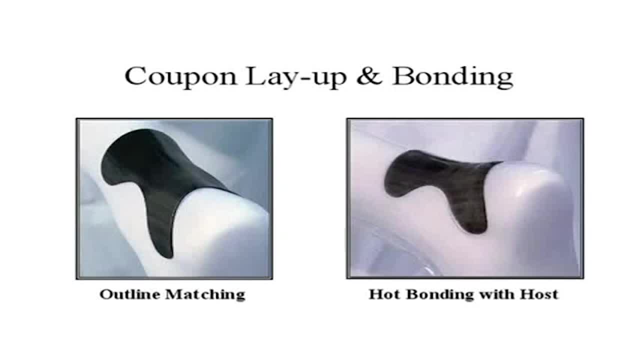 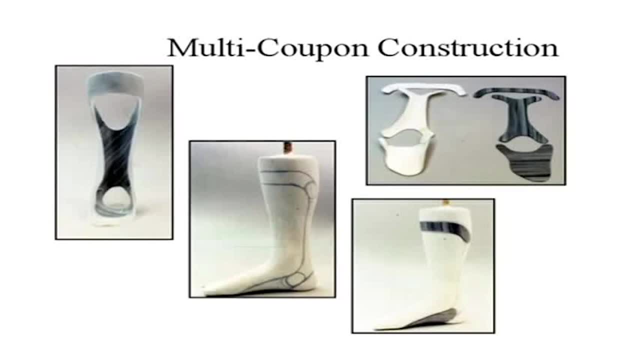 And by using this technique you can make some pretty sophisticated, complicated composite products. Everybody loves ground reaction AFOs that are laminated. This is a way to do it, basically with a thermoplastic composite. In this fashion, you draw where your composite skeleton is going to be. 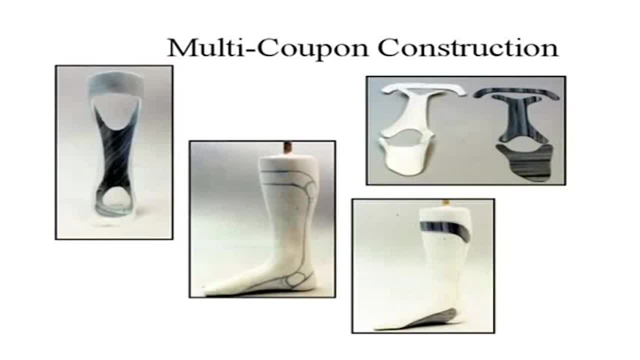 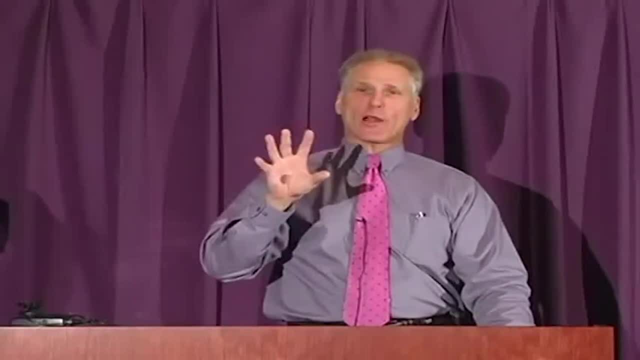 Here we have three overlying patterns. We take those three patterns, cut out our three pieces of material When we do our layout come out of the oven. it's four steps: choreograph: Boom, boom, boom, boom. Overlay with a whole sheet. 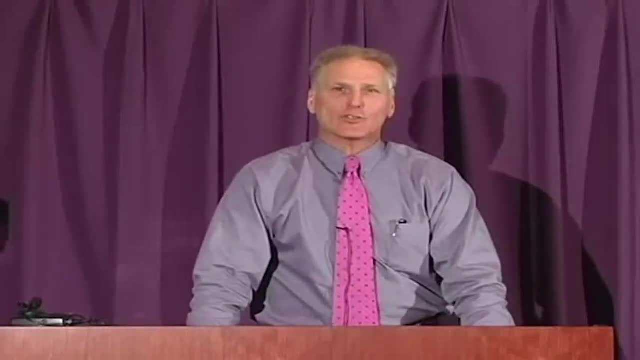 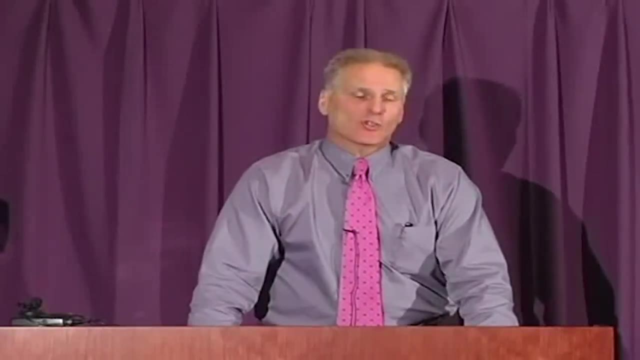 All vacuum form. Basically less than 25 seconds. Takes two guys to do it. You can be very quick but in the same amount of time that you can do a solid ankle AFO in just homopolyproplene by cutting out the coupons. now you've got a laminated AFO. 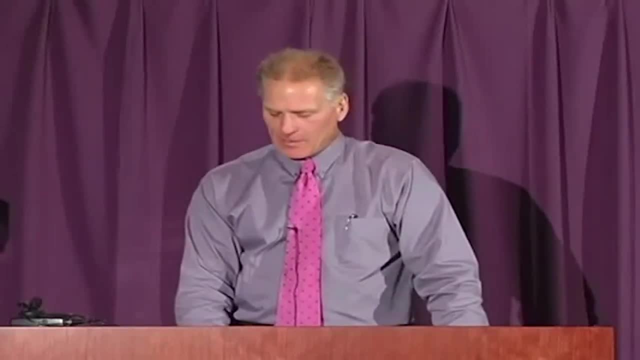 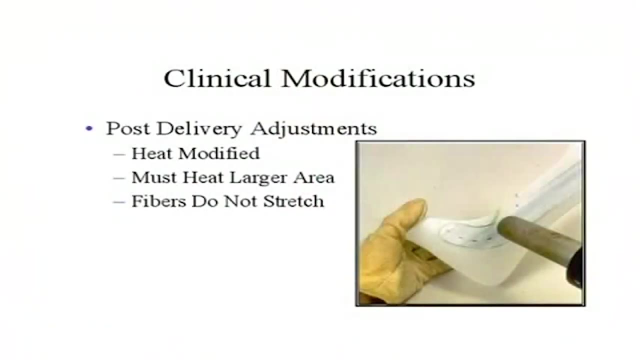 Very quick to do. it All done with Compcor. So depending on how sophisticated you want to get with the material, it'll basically allow you to do whatever you want: Clinical modifications: because it is a thermoplastic, you can recontour that device. 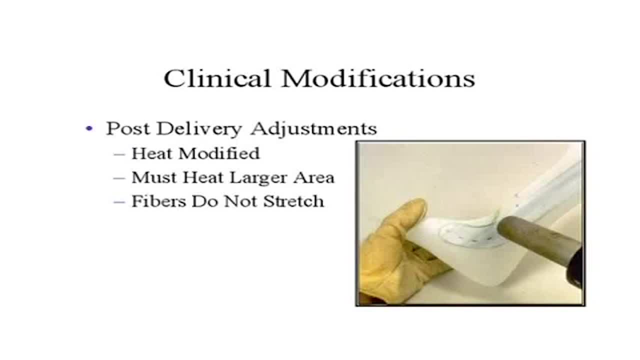 Now you have to typically heat a larger area, primarily because you're also moving the fibers. You're not getting stretch, you're just moving the fibers. So you have to heat a little bit of area. be very slow in that heating process. 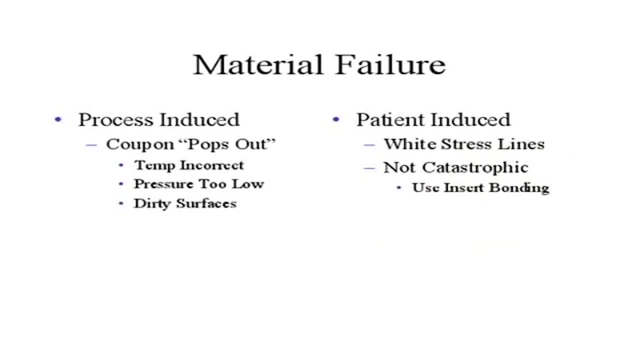 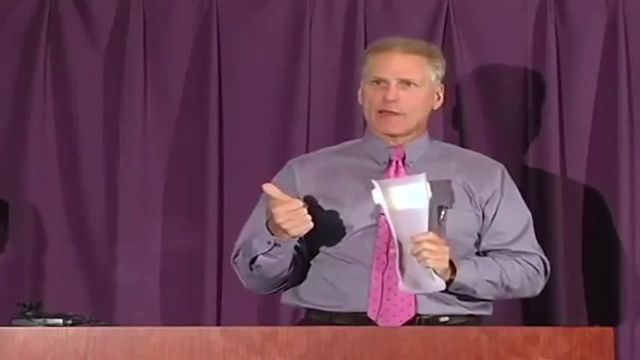 In terms of failure, we do see it like anything else, but here's the way that I determine whether it's process induced or patient induced. If the coupon pops out, in other words this whole coupon separates and pops out of the host device, then your temperatures were incorrect. 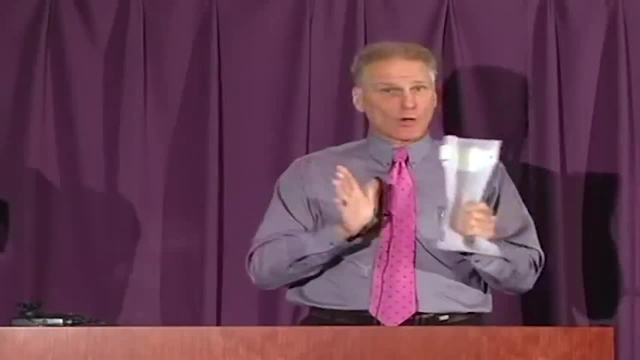 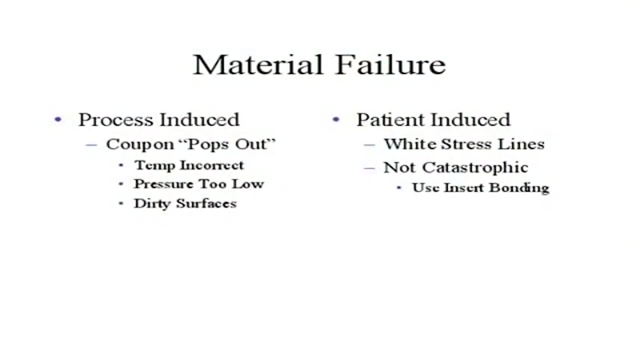 Didn't have enough temperature to allow the polypropylene to bond. The pressure was too low to bring everything together or you had dirty surfaces. You had that blooming effect that made a dirty surface. If it's patient induced, I might see white stress lines. 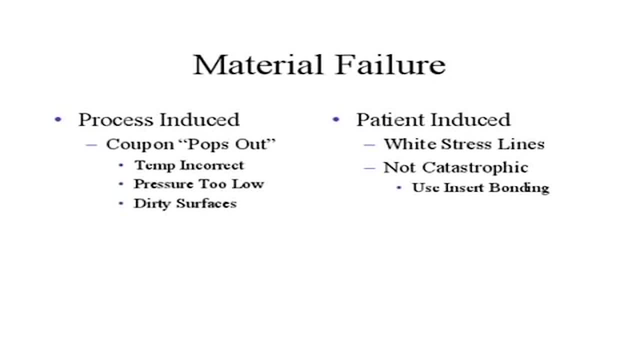 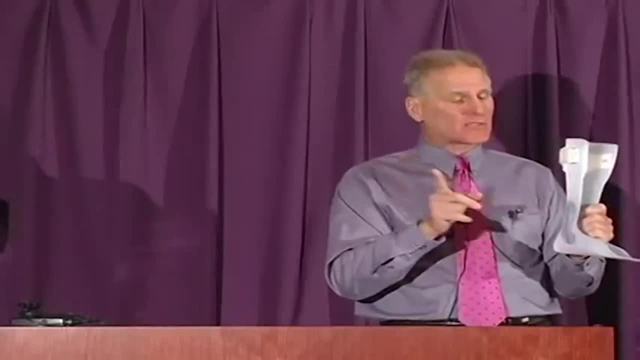 That's not a catastrophic failure. that's showing me that the glass fibers are starting to fail. Now the glass fibers would fail at a much lower level than the carbon fiber, obviously, So typically that's not a situation of risk at the patient, For the patient. 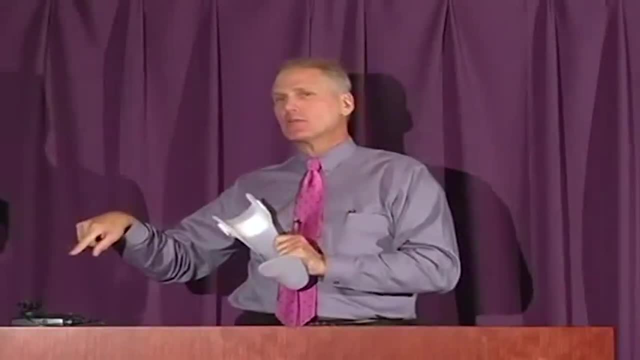 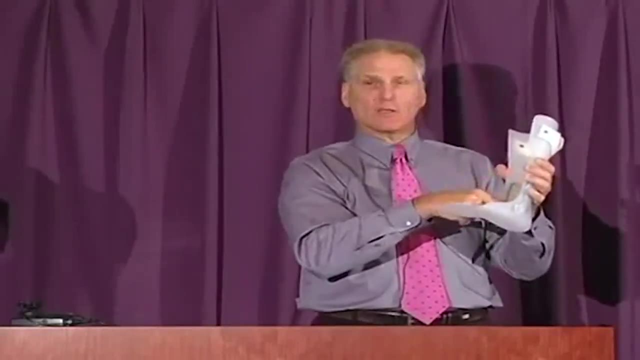 But what it will tell me is when I want to do a replacement AFO for that patient, I'm probably going to now want to do my double lamination Rather than just doing a single lamination. I'm going to want to do that embedding technique. 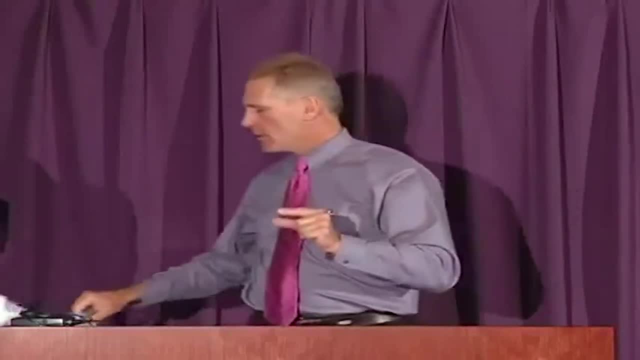 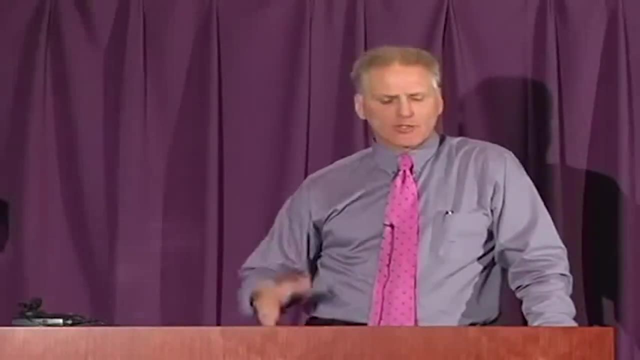 that we just talked about. So it all depends how we do it. Or you use the very thick layer of comp core, that six layer stick, rather than just doing four layers of prepreg tape. So to end this segment on thermoplastic composites, 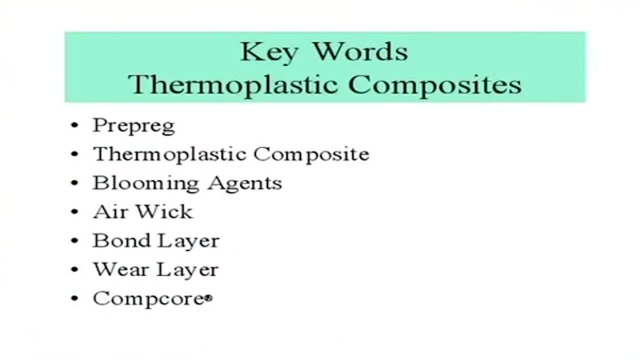 We described what a prepreg was, what a thermoplastic composite was, the blooming agents, again, the ear wick, the bond layer, the wear layer of comp core and then, of course, just the general term of what comp core is. 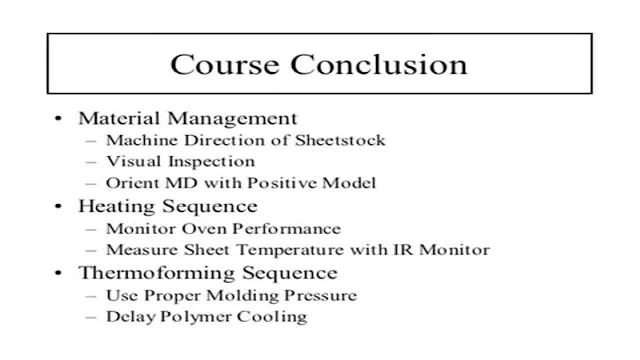 In terms of bringing this course to a conclusion, I do want to just hit a couple high points In terms of materials management. know your machine direction. Do the visual inspection of your sheets coming into your lab. No ripples, No pressure contracts. 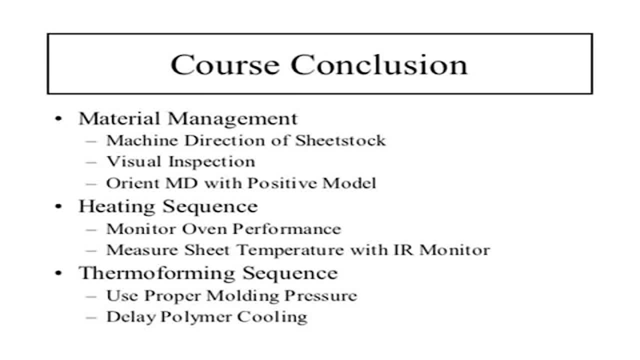 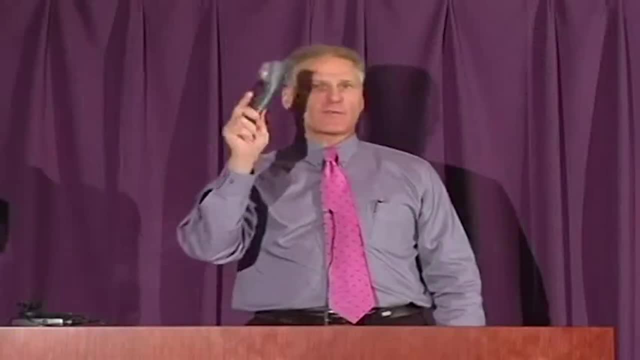 And then orient that machine direction with your positive model. When you get to the heating sequence, monitor your oven performance, Make sure it's the clean tubes, Make sure the regulator is working at the level it should be, And then measure your seat temperature with that handheld infrared thermometer. 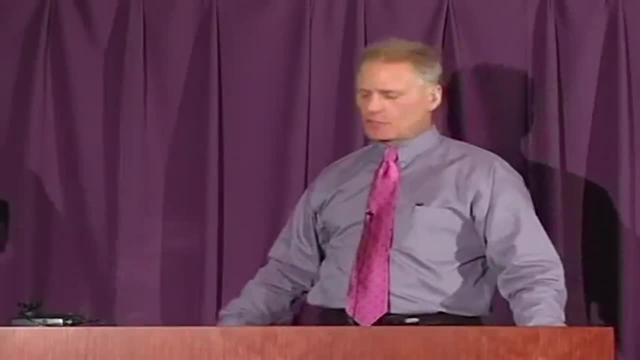 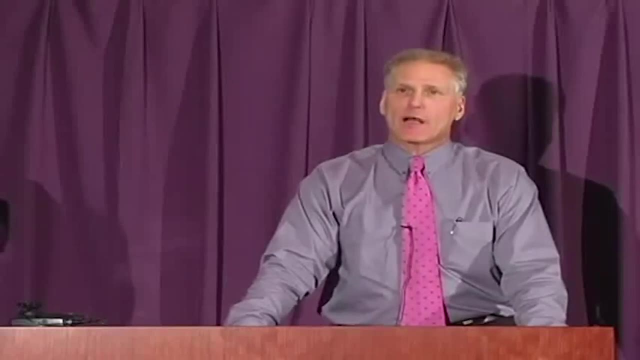 For 50 bucks. this is very sophisticated, cheap technology at this point in time. If you want to really be disciplined in your lab, do have a process record for every item you make. You don't have to do it right now. I firmly believe that one of the regulating agencies is going to come along at some point. 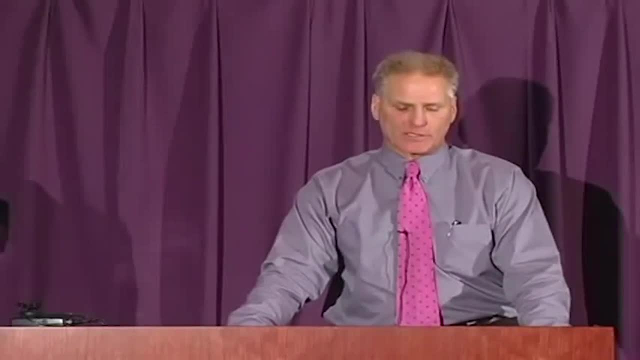 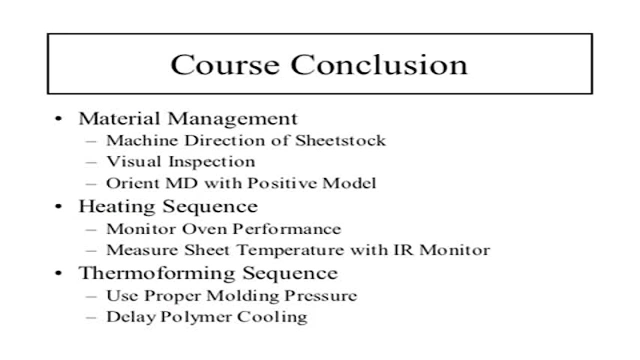 in time and make us do that. So it's an easy habit to put in place at this point in time. In terms of your molding sequence, do use proper molding pressure. Make sure your system is more. your vacuum molding system is more than a vacuum pump. 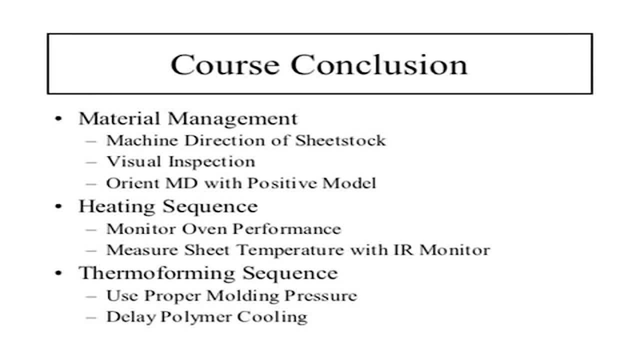 It has to be. That's just the heart of the system, It's not the whole system- And delay your polymer cooling. That will just allow your material to go into that Lowest energy state and have its highest strength capability. Those are all the processes that you want to put into place in terms of this course. 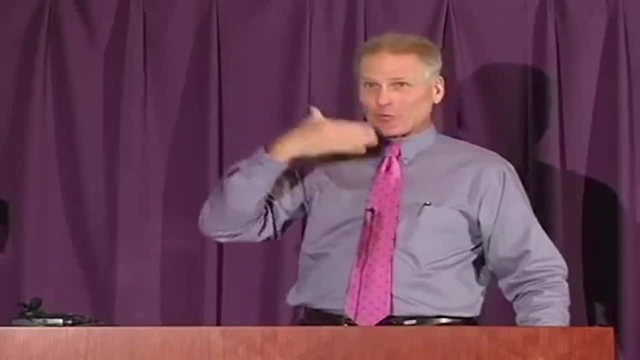 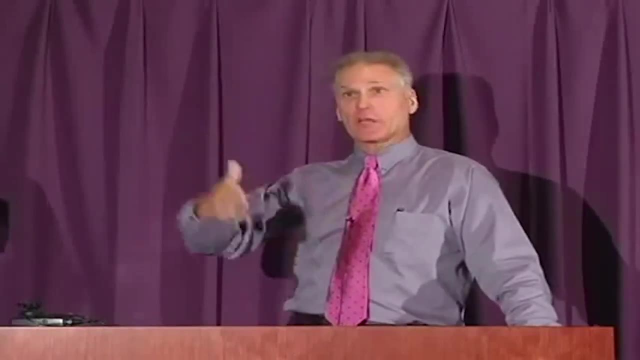 It's been a long time for you, I'm sure at this point in time if you've gone through this whole program all at once, But it took us basically about eight years to go through all this in our lab, in this discovery pathway. 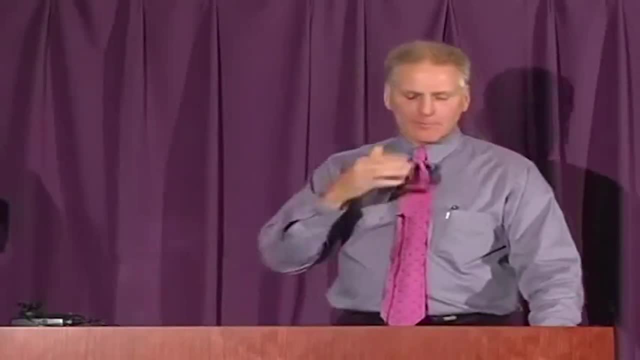 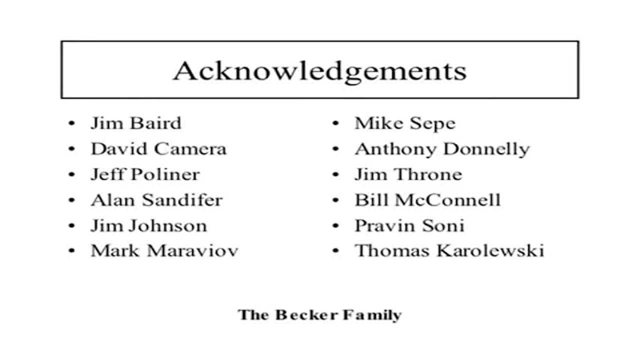 And finally, we use these techniques all the time. So, if you stayed with me at this point in time, There's a number of people I'd like to acknowledge with this list of people. They've all helped me along the way. They've given me insights. 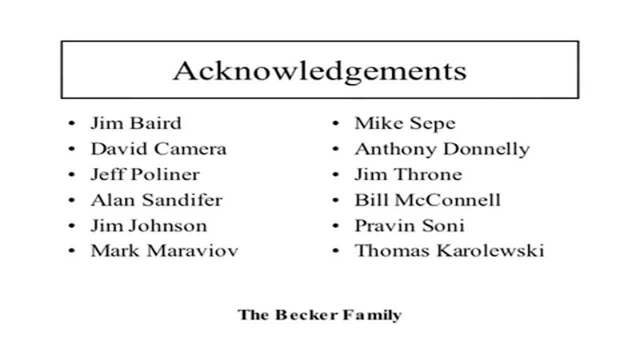 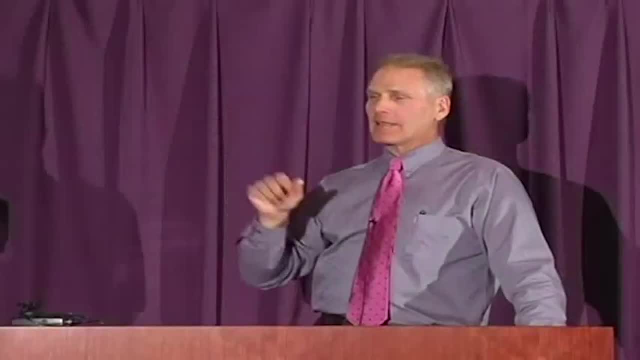 They've been mentors, They've given me feedback, And none of the projects of this magnitude ever happened with just one person going all the way through. I'd like to thank the Becker family, of course, because they've always supported me as an 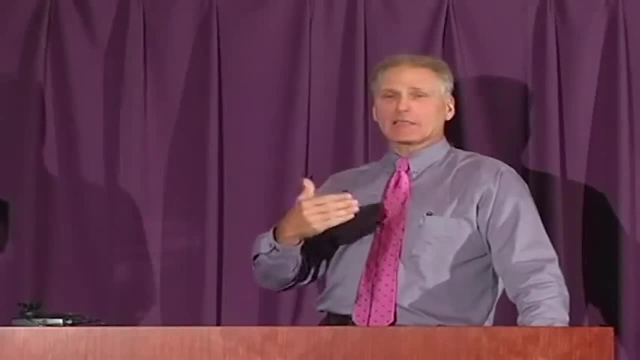 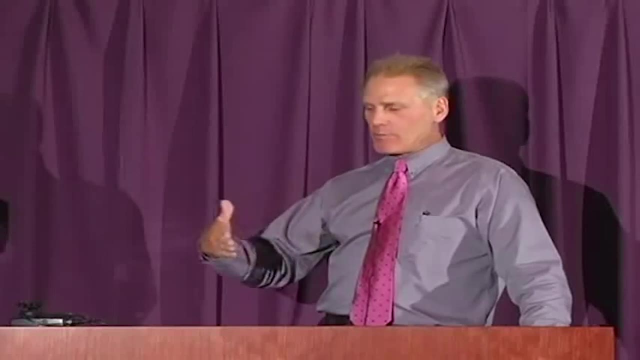 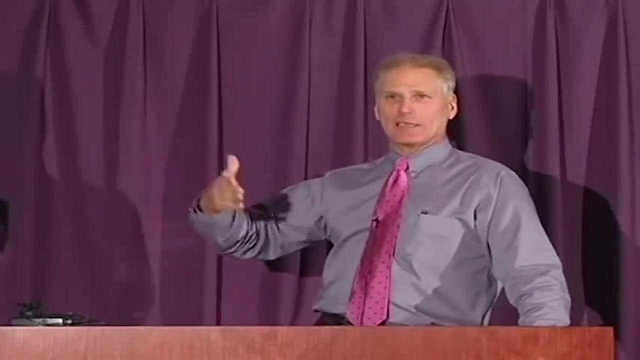 employee through all these years Employed basically supported me with my communication with the schools. When I started this program I thought that this would be probably a 14 to 18 month process. I never thought that I would be doing this year in and year out through 30 plus countries. 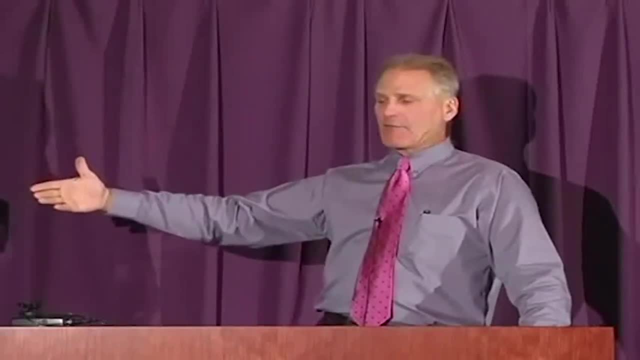 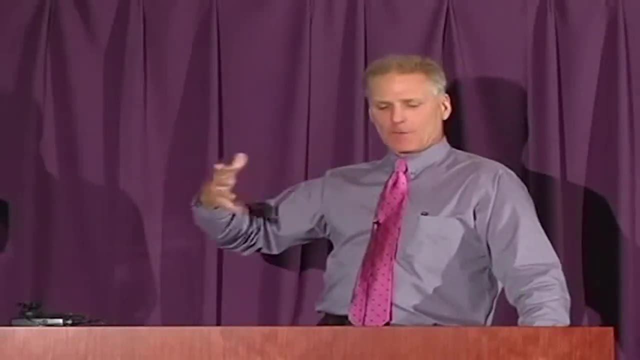 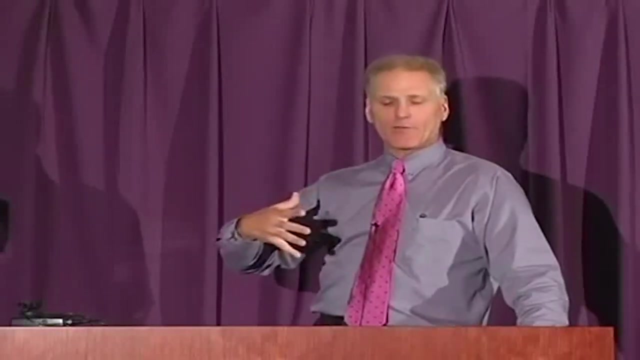 But the basic course has grown to have that level of appreciation from the field. And then for myself, you stay with a subject this long and you have to be somewhat introspective of what drives you to have the interest. And for myself It comes a little bit, I think genetically. you know, our upbringing is always somewhat. 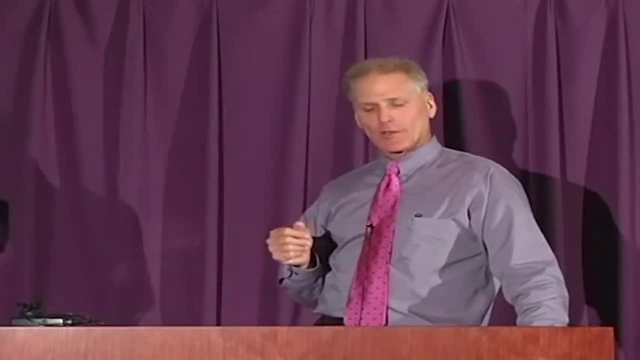 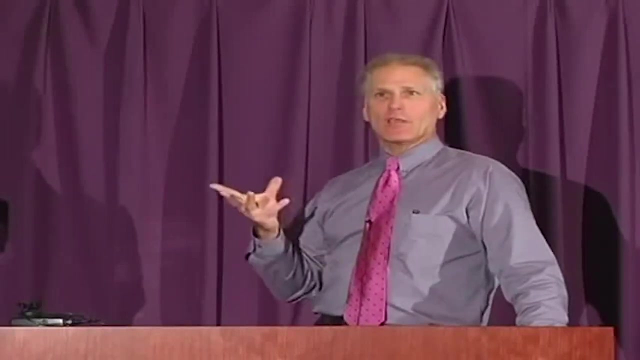 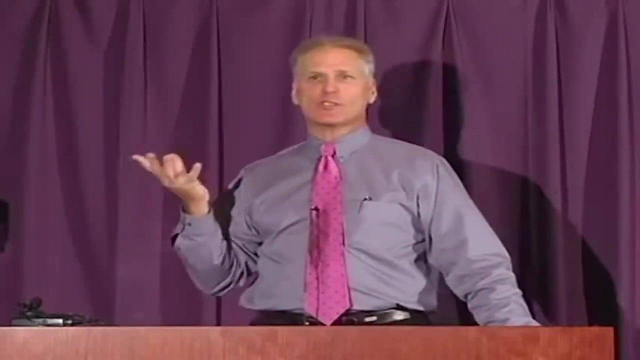 environmentally controlled and genetically controlled. And ironically my great grandfather had a company back in the textile mill I grew up in in Woonsocket, Rhode Island that he was one of the earliest users of composite materials. He had a company where they would take acetate saturated cardboard and pressure steam form. 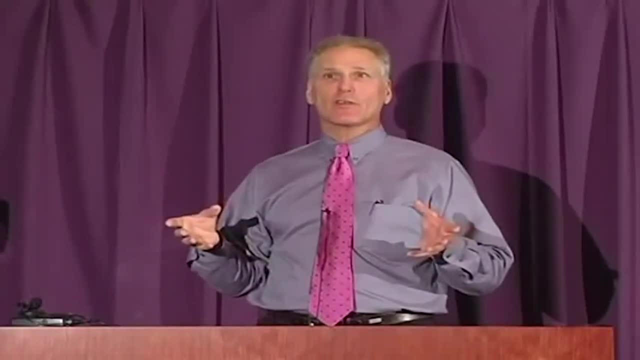 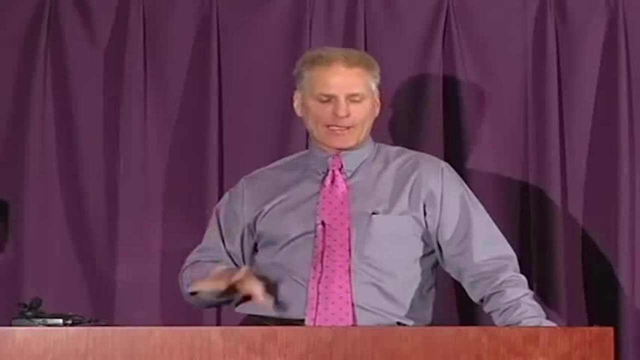 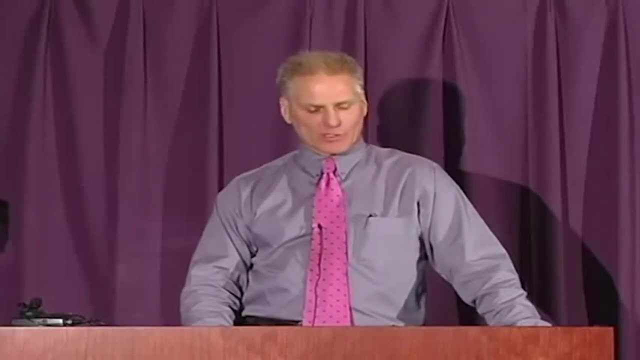 them into bobbins for the textile industry. Unfortunately, he went out of business just before World War II. He died at an early age. My great uncle couldn't run the business and we lost the business, But on the Blackstone River, which was the site of our earliest industrial revolution. 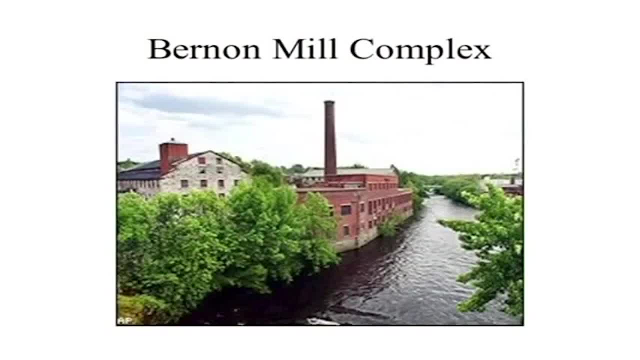 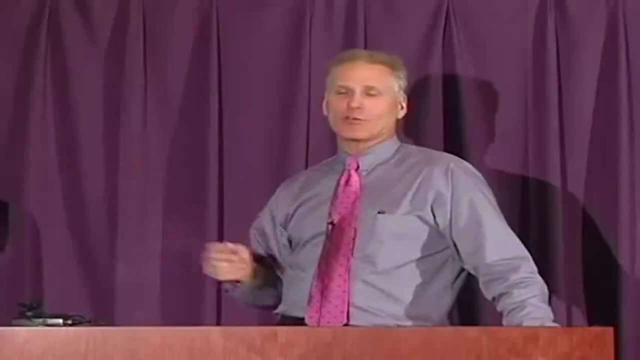 these were all textile mills as I was growing up, And in this old granite building was where my great grandfather had his business, And today they're nice condominiums. So it's kind of ironic how we've seen that evolution of outsourcing jobs. All those textile jobs in the New England went to the South and of course, as you know, 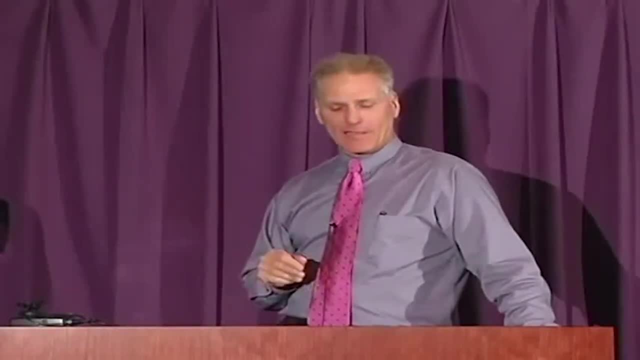 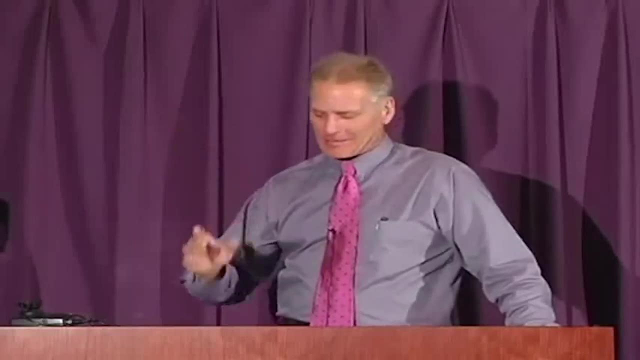 they've all gone out of the country at this point in time, But I think that certainly my interest in it comes from it genetically, because how could it ever last this long at this point in time? So I do want to thank you. I'm always available. 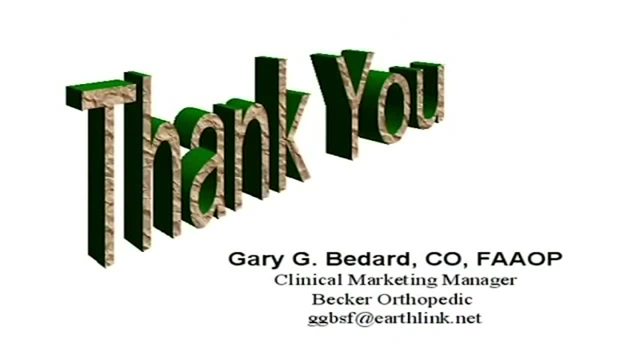 There's my email address. that's on here. You can either contact me through my email address, Call me directly through Becker Orthopedics. I'm always more than willing to answer questions on the topic of clinical thermoforming. Thank you very much. 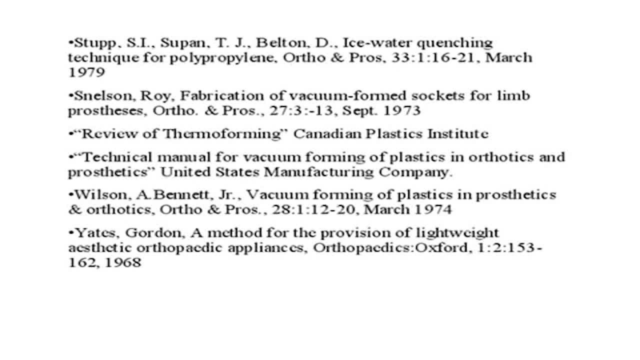 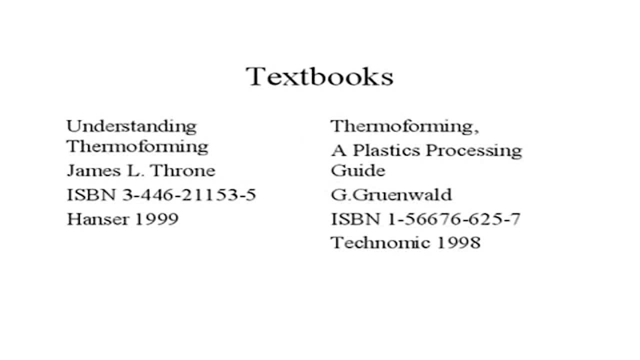 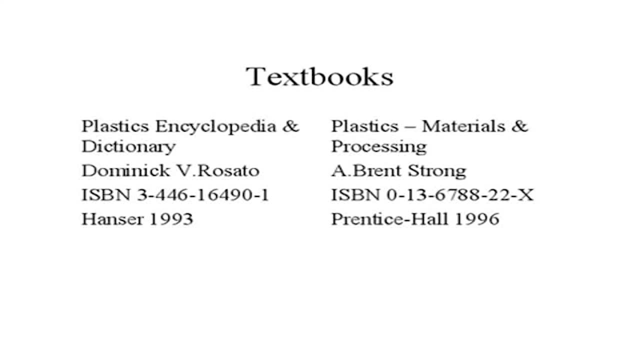 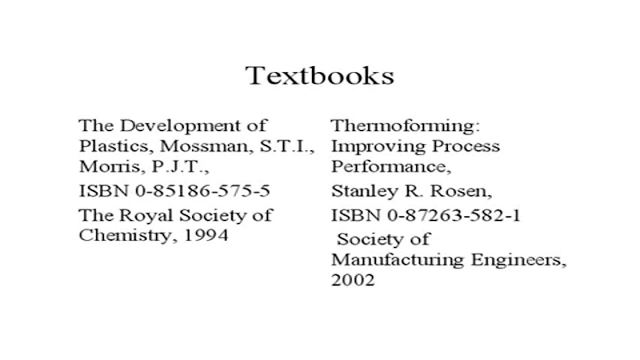 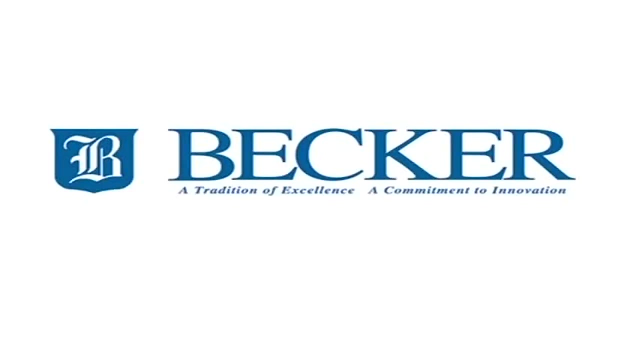 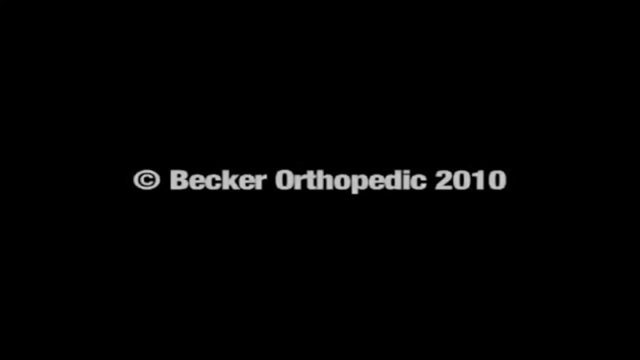 Thank you. Thanks for watching.